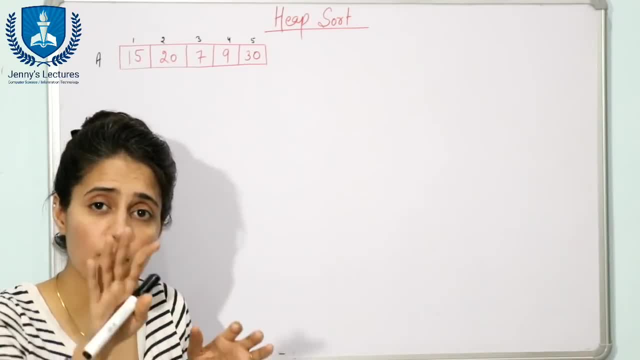 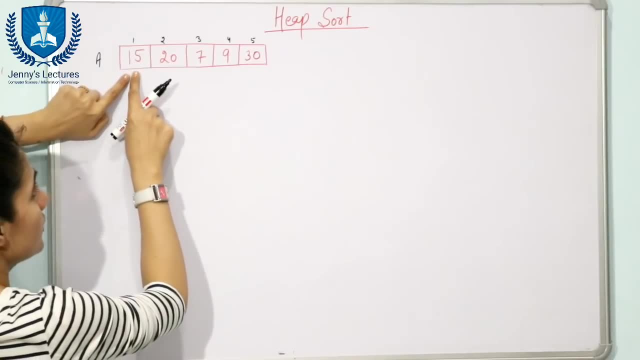 to build a max heap. how data is to be inserted in max heap, That processor I have already discussed in the previous video. You can check out that link in the description box. Now see first. first element is 15.. So in the tree we have only one element that is 15.. So it is a max heap by default. 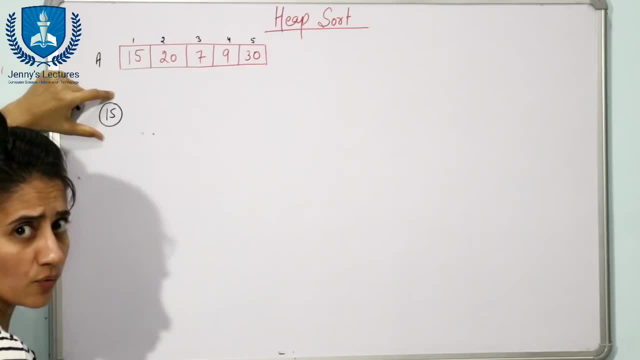 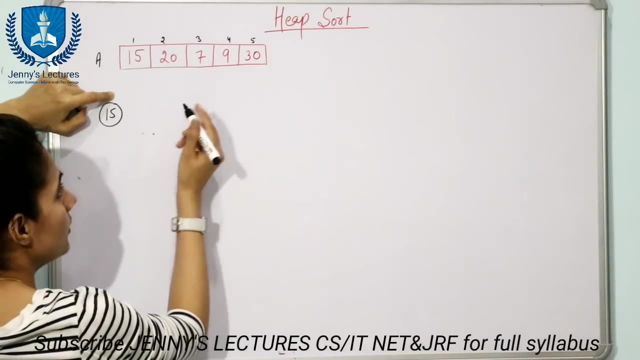 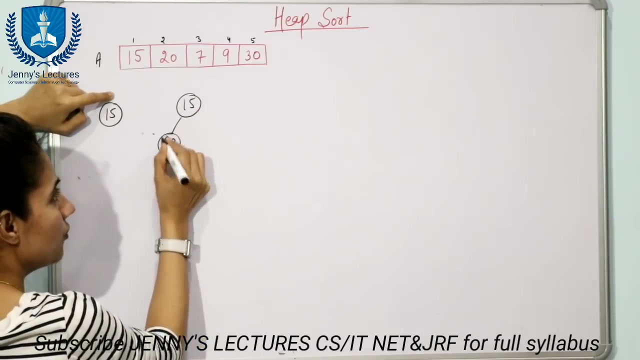 because no child element would be there. Only one element is there, Then obviously it is a max heap Fine. Next element is 20.. Now where the data is to be inserted. We have 15.. Now where 20 to be inserted To the left of this 15, because, see, this heap tree is a almost complete binary tree. Okay, 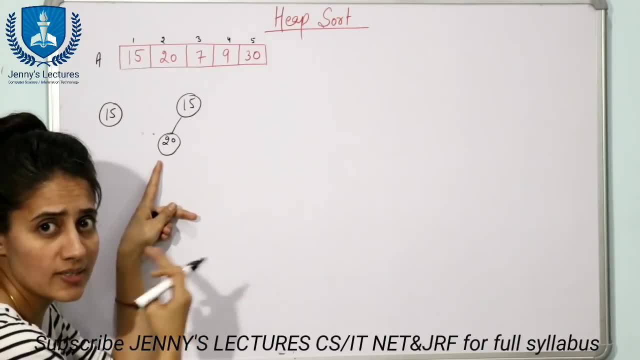 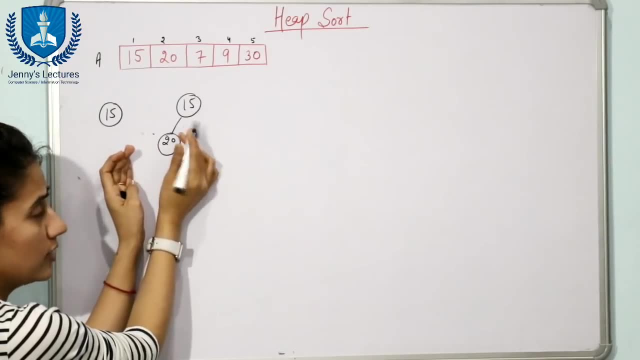 And the data in the complete binary tree in the last level data should be as left as possible. So we are going to insert to the left of this 15, not to the right of this 20, because we cannot leave this place empty. We have, we are supposed, we are going to. 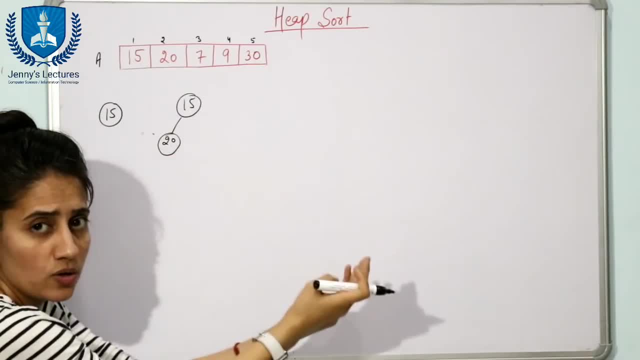 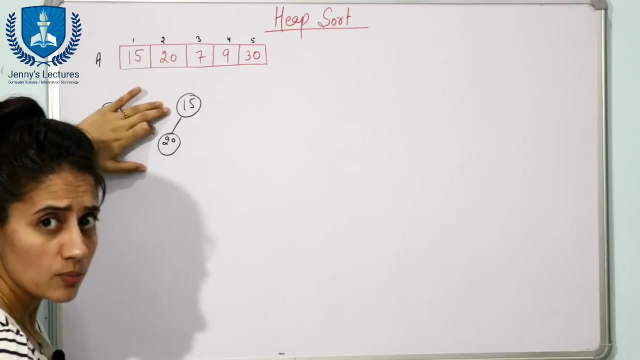 we are supposed to fill this left side first. After that you can fill right side. So now, after insertion of 20, this is the tree. Now you have to check: is it satisfying the max heap property? Because after each insertion you are going to check is it still a max heap or not. Have to. 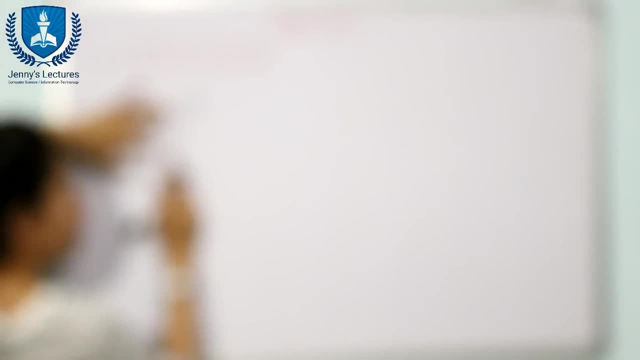 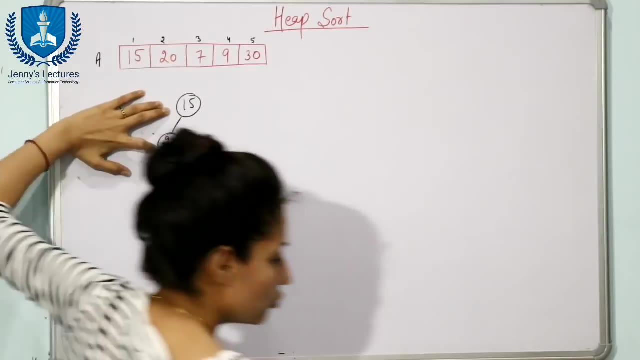 check. the data to be inserted is 20.. Now find out: parent of this 20, parent of 20 is 15 and 15 is less than 20, and that is not possible in max heap. So we are going to swap, because in max heap 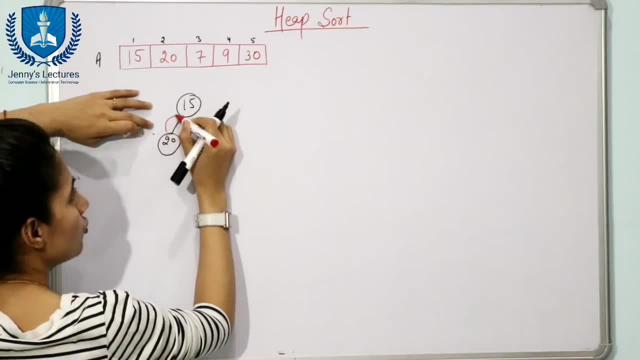 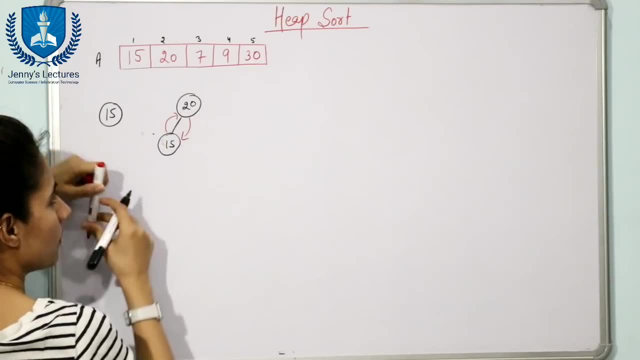 parent would be always greater than or equal to its child. So here swapping would be done. So here we will write 20, and here we will write 15.. Now it is max heap. Next element is seven. Now where seven is to be inserted, Here we: 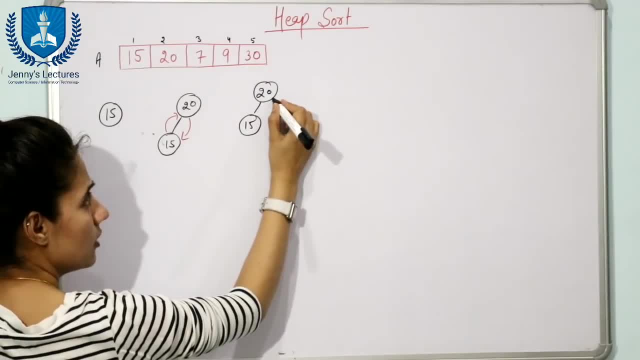 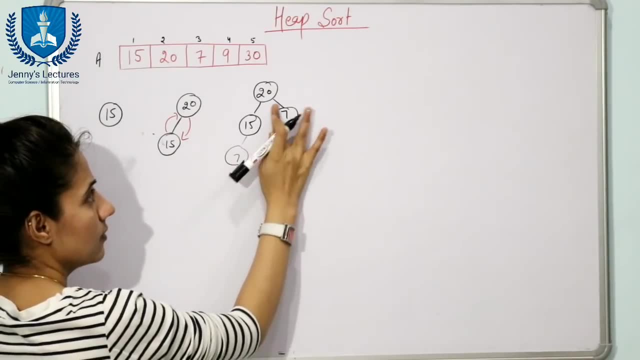 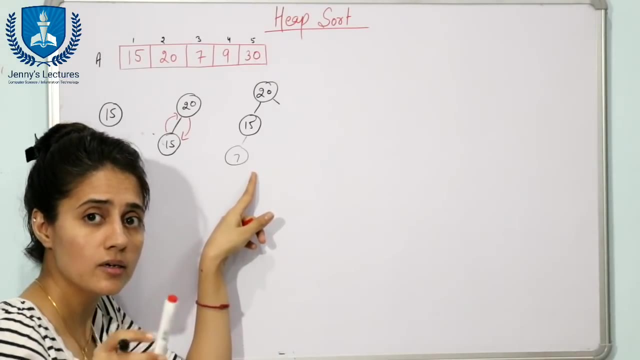 have 20,, 15,, seven would be inserted first of all to the right of this 20.. Fine, See, we cannot insert seven here. Why so? Because is it this? this heap tree is also a almost complete binary tree, And in complete binary tree all the levels except possibly the. 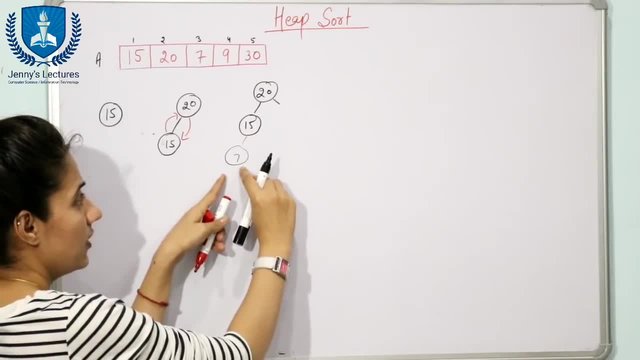 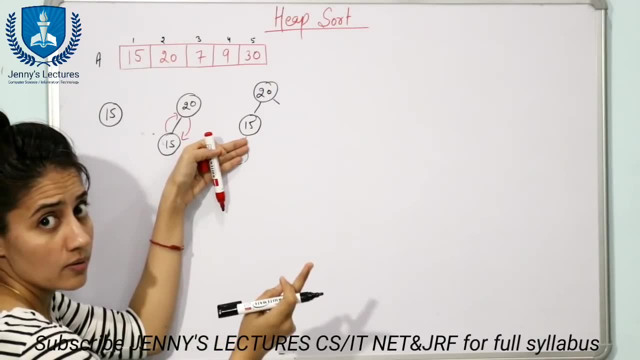 last level should be completely filled. So if you insert seven here, so this is the last level, So these levels should be completely filled, but this level is not completely filled. This is this is having only one child here. right child should be there. So first of all, 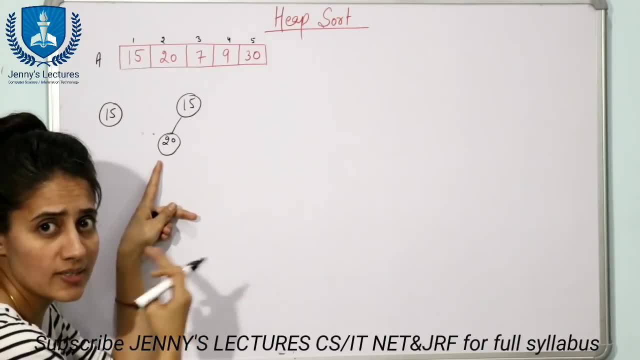 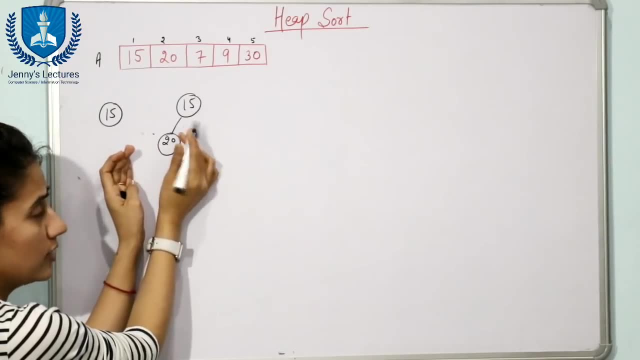 And the data in the complete binary tree in the last level data should be as left as possible. So we are going to insert to the left of this 15, not to the right of this 20, because we cannot leave this place empty. We have, we are supposed, we are going to. 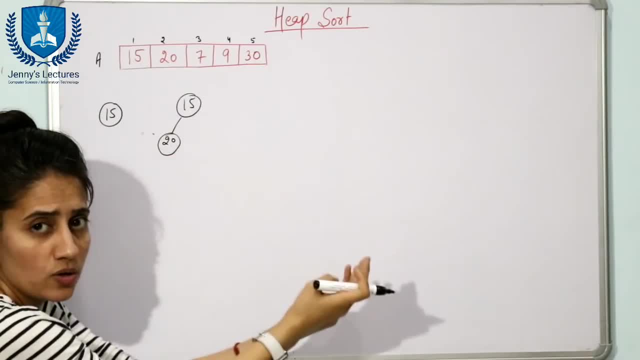 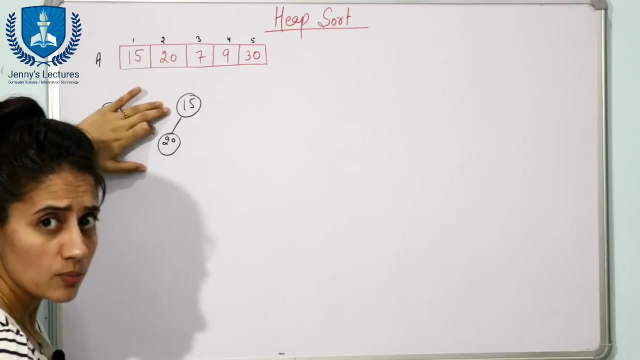 we are supposed to fill this left side first. After that you can fill right side. So now, after insertion of 20, this is the tree. Now you have to check: is it satisfying the max heap property? Because after each insertion you are going to check is it still a max heap or not. Have to. 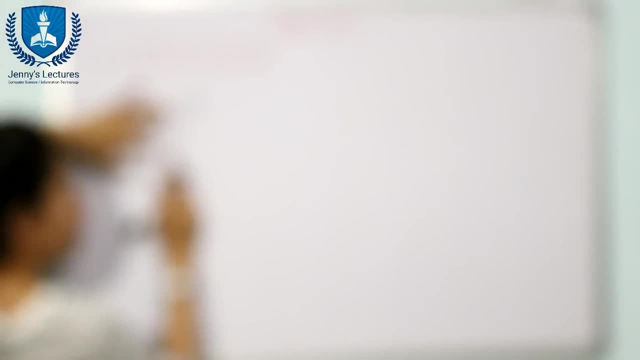 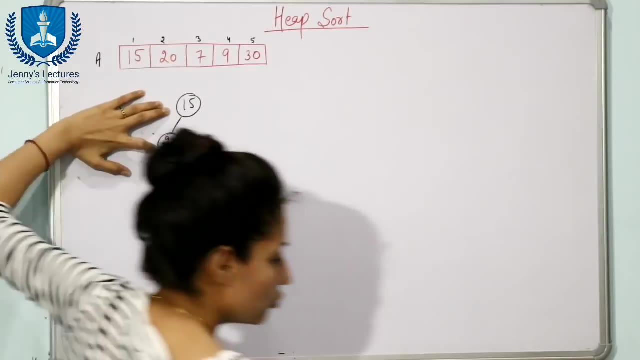 check. the data to be inserted is 20.. Now find out: parent of this 20, parent of 20 is 15 and 15 is less than 20, and that is not possible in max heap. So we are going to swap, because in max heap 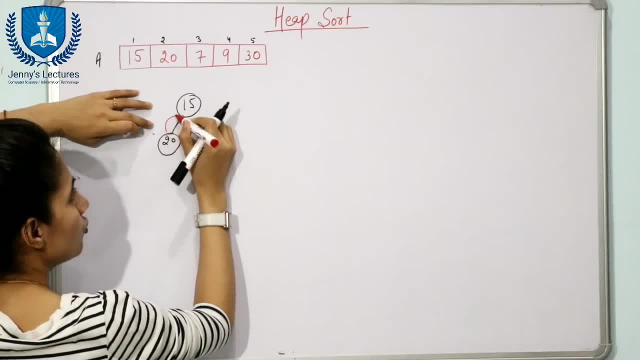 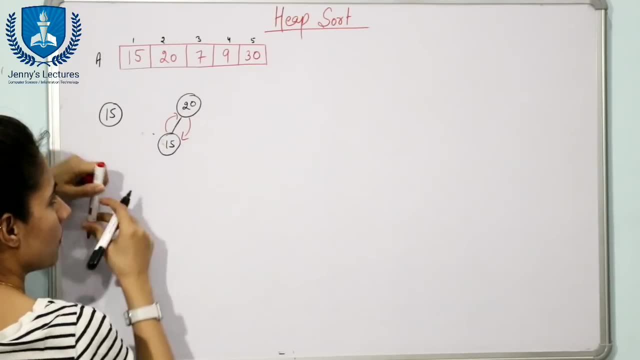 parent would be always greater than or equal to 20.. So we are going to swap, because in max heap parent would be always greater than or equal to its child. So here swapping would be done. So here we will write 20 and here we will write 15.. Now it is max heap. Next element is 7.. Now where 7? 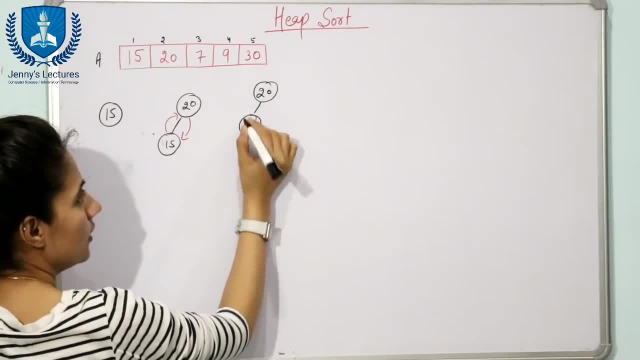 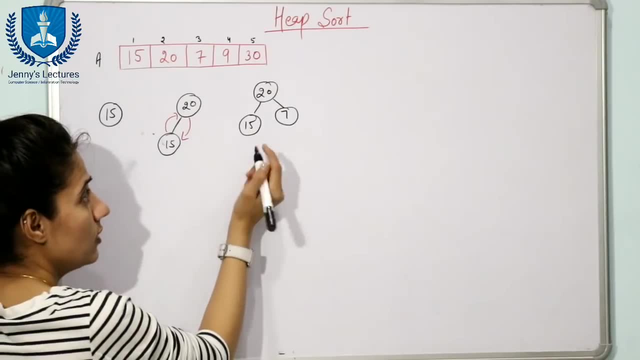 is to be inserted here. we have 20, 15.. 7 would be inserted first of all, to the right of this 20.. Fine, See, we cannot insert 7 here. Why so? Because is it this? this heap tree is also a. 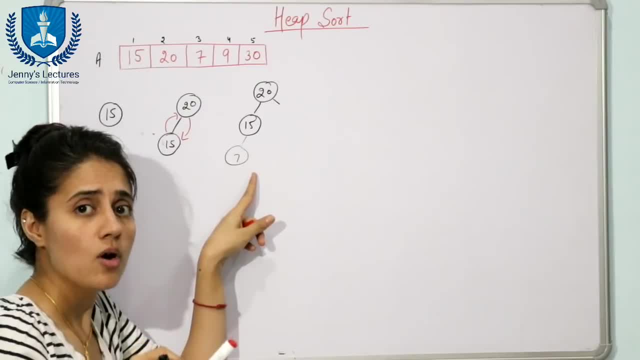 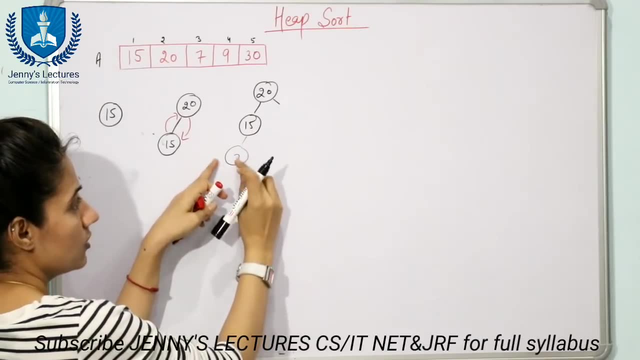 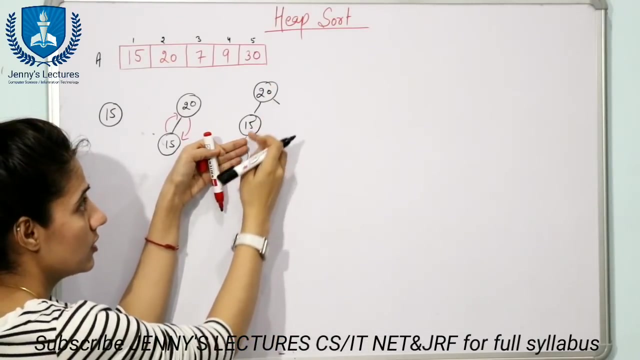 almost complete binary tree and in complete binary tree, all the levels, except possibly the last level, should be completely filled. so if you insert 7 here, so this is the last level, so these levels should be completely filled, but this level is not completely filled. this is this is having only one. 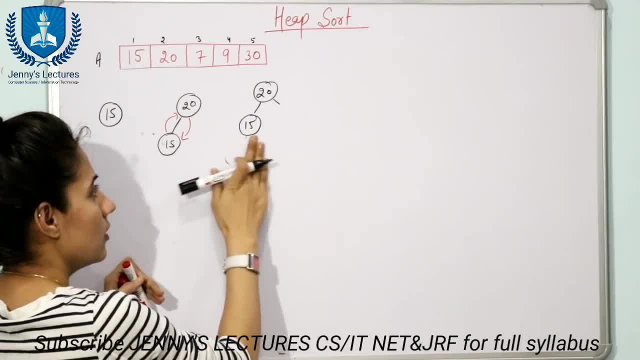 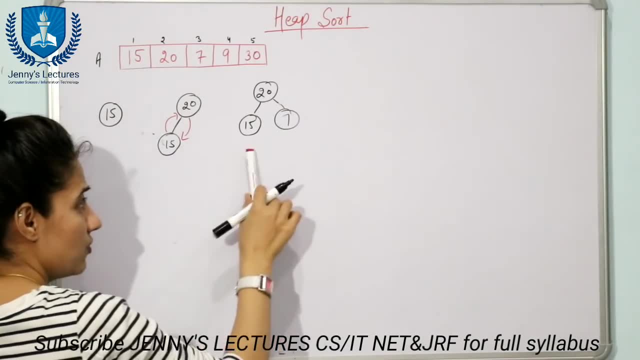 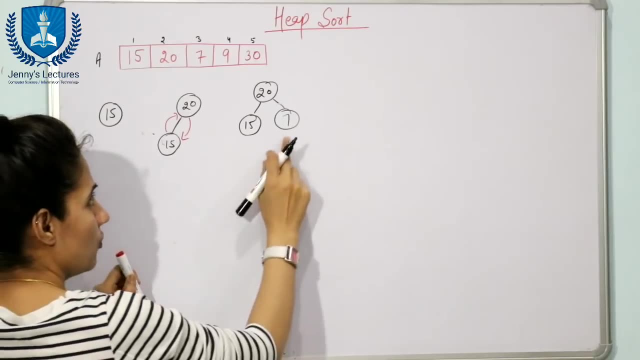 child here? right child should be there. so first of all, so we cannot insert 7 here, we have to insert 7 at this place. fine, now check: is it still satisfying maxi property? after inserting 7, find out the parent of 7. that is 20. 20 is greater than 7. fine, no swapping would be done. it is maxi. 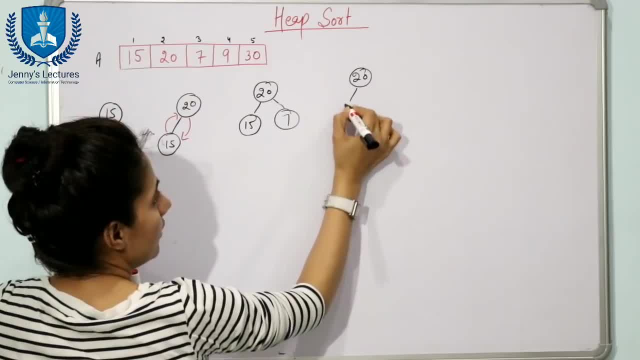 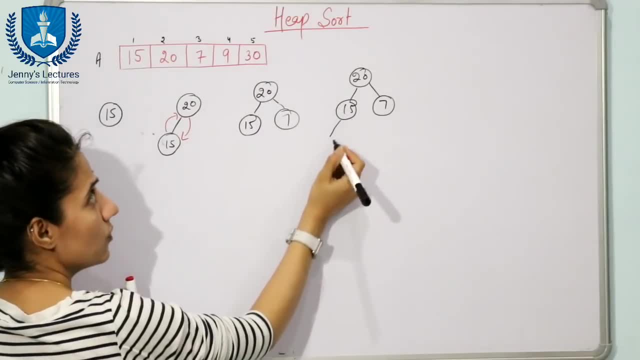 insert 9, 20, 15. here we have 7, so this level is completely filled. now 9 would be inserted to the left of this 15. here we will insert 9. now check out parent of this. 9 is. after every insertion you have to insert 9. and after every insertion you have to insert 9. and after every insertion. 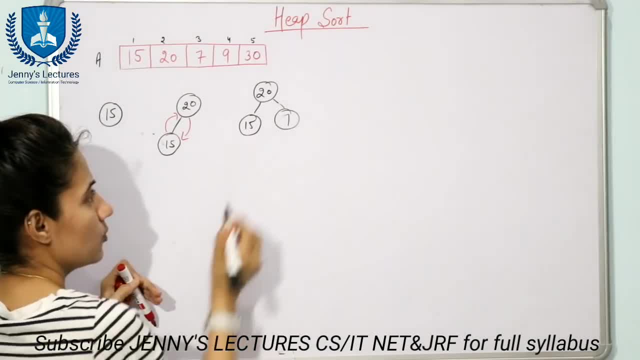 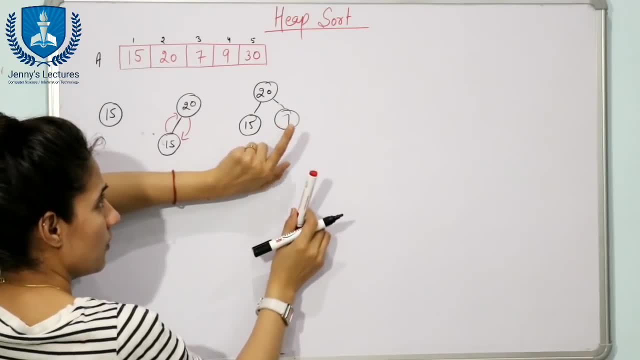 so we cannot insert seven here. We have to insert seven at this place. Fine, Now check: is it still satisfying max heap property? So after inserting seven, find out the parent of seven. that is 20,. 20 is greater than seven, Fine. 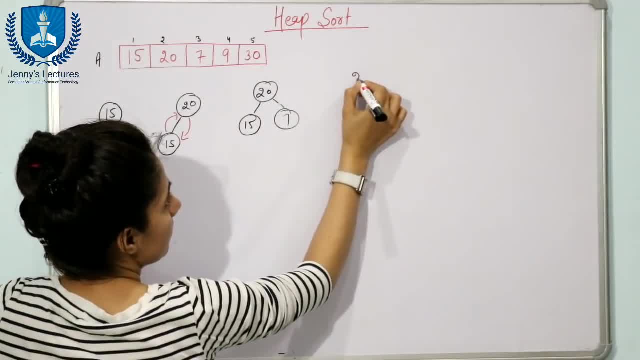 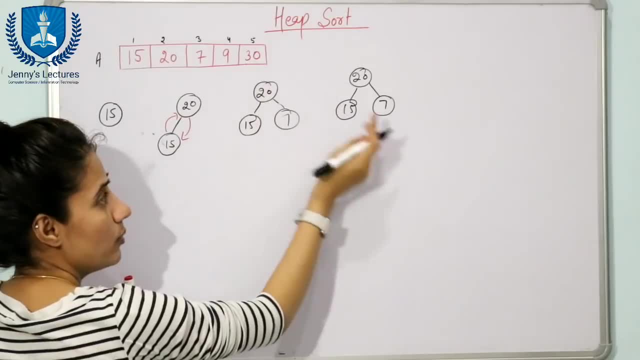 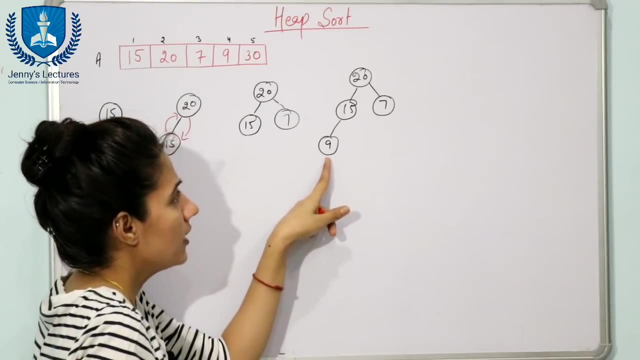 No, swapping would be done. It is max heap, Insert nine, 20,, 15.. Here we have seven, So this level is completely filled. Now nine would be inserted to the left of this 15.. Here we will insert nine. Now check out. parent of this nine is after every insertion you have to check. 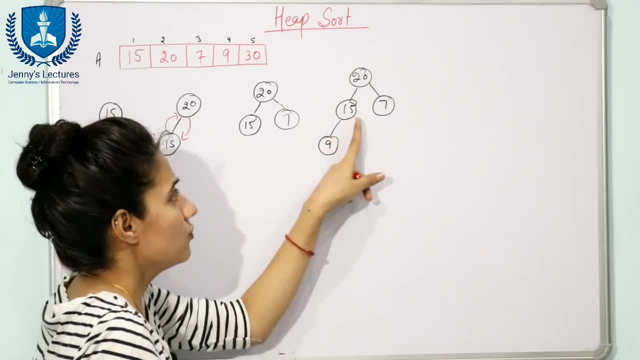 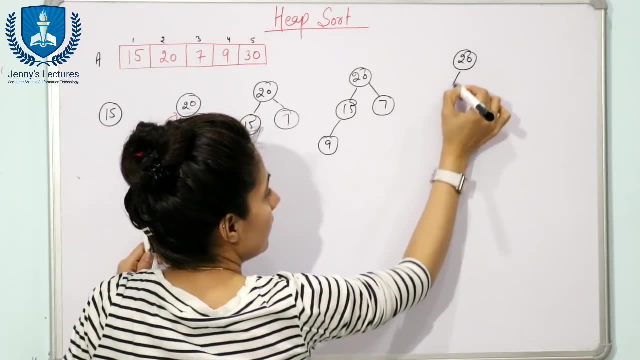 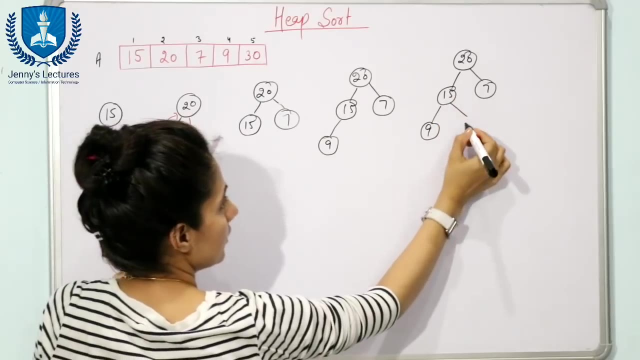 Is it still satisfying the max heap property or not? Parent of nine is 15 and two is greater than nine, So it is a max heap. no need to do any swapping. Next is 30. Here we have 20,, 15,, 7, and 9.. Now where this 30 would be inserted to the right child of this 15? Here. 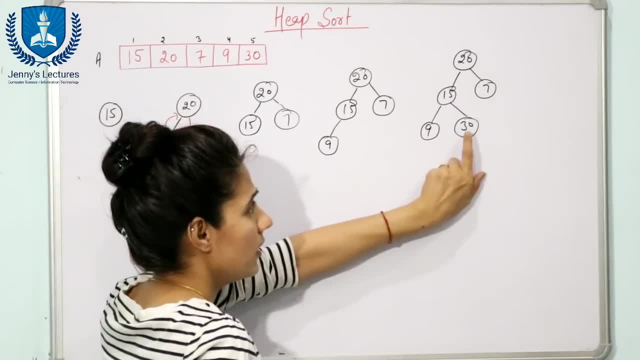 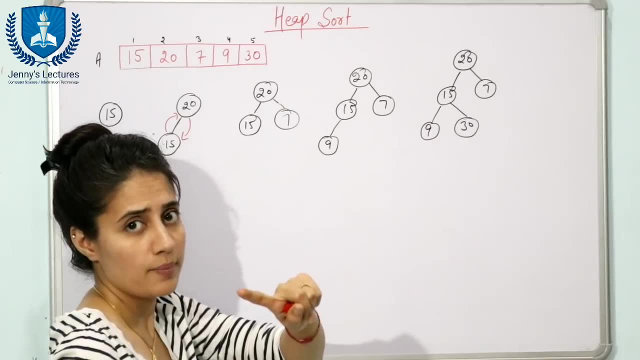 we have 30. Now again check, Find out The parent of this 30. parent of 30 is 15 and 15 is less than 30 and that is not possible in max heap. Now you have to do what Swapping 30 would go up. So here. 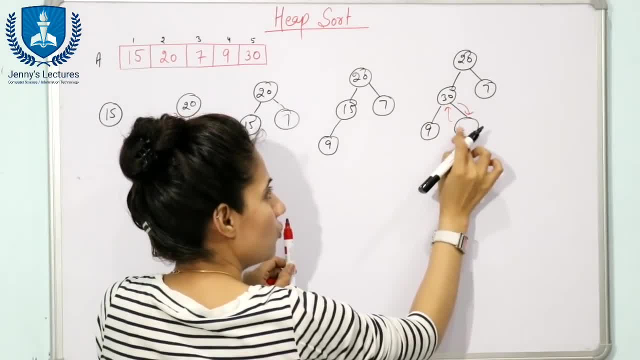 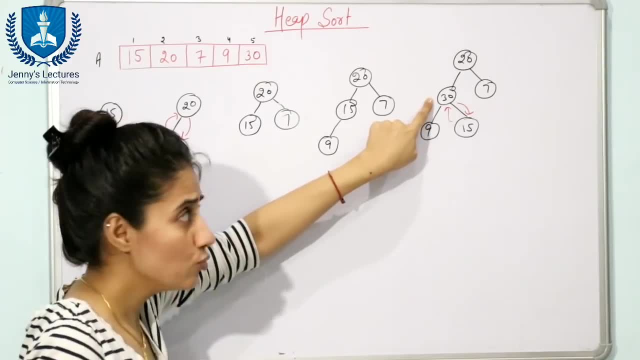 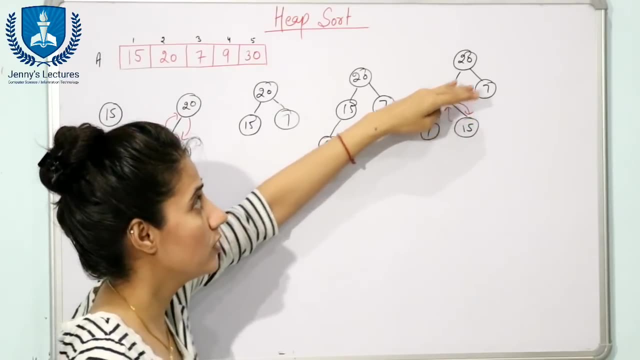 you will write 30 and 15 would go down here. you will write 15 now, 30 is here. now you are not done with this. you are you are supposed to check this with its parent. we will keep on. we will keep on checking this inserted element with its parent till we reach to the root element. fine, we have. 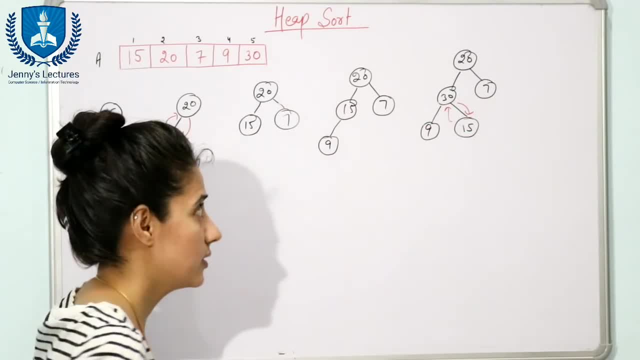 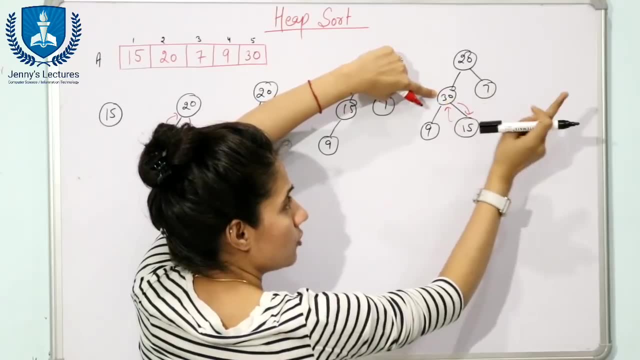 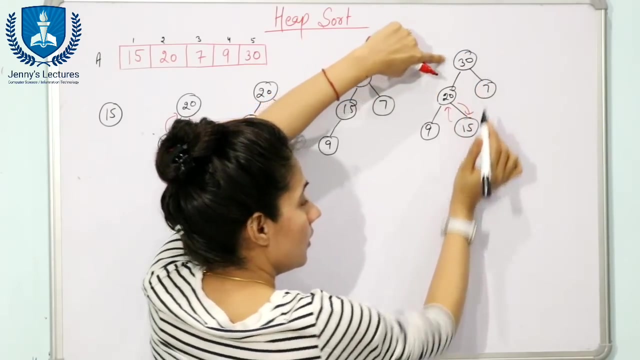 already discussed this concept in when we were discussing max heap insertion. now again find out: parent of 30. now parent of 30 is 20 and 20 is less than 30. so that is not possible again. we will do it swapping. so here 20 would be there and here 30 would be now. 30 is the root element now. 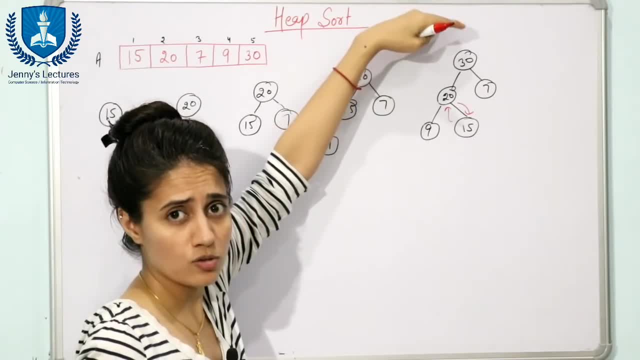 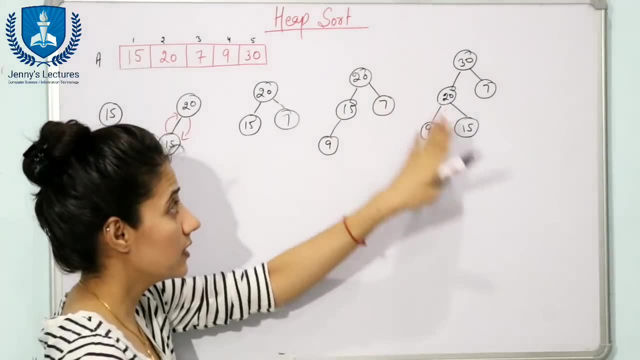 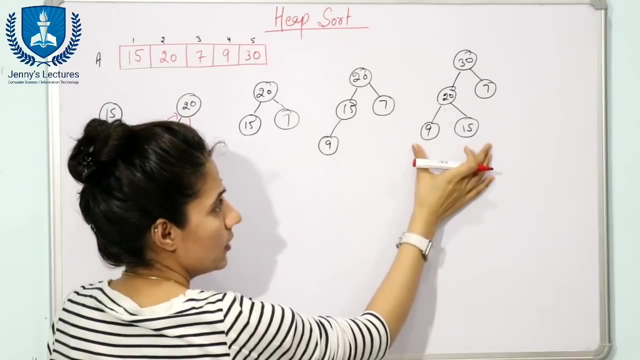 we are going to stop this comparison, because 30 is 30 is not having any parent node. now, fine, so this is now our max heap after inserting this data. now, this is our max heap now. now that array would be. this array has been updated. now array would be something like this: 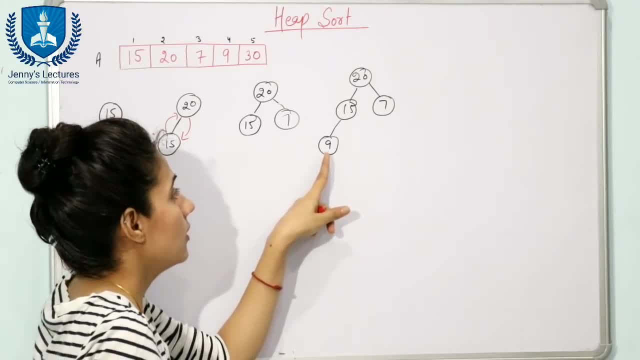 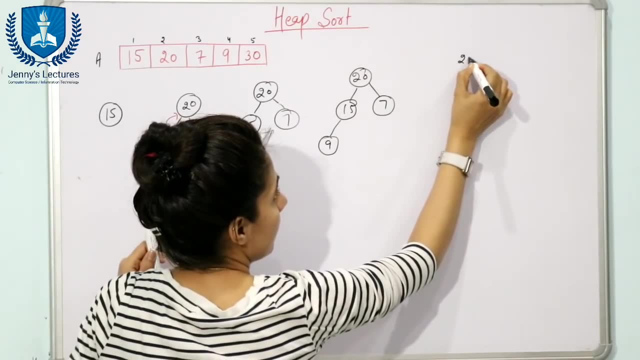 to check is it still satisfying the maxi property or not. parent of 9 is 15 and 15 is greater than 9, so it is a maxi. no need to do any swapping. next is 30. here we have 20, 15, 7 and 9. now where this? 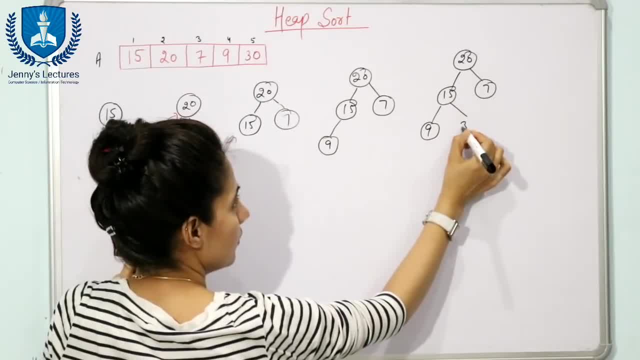 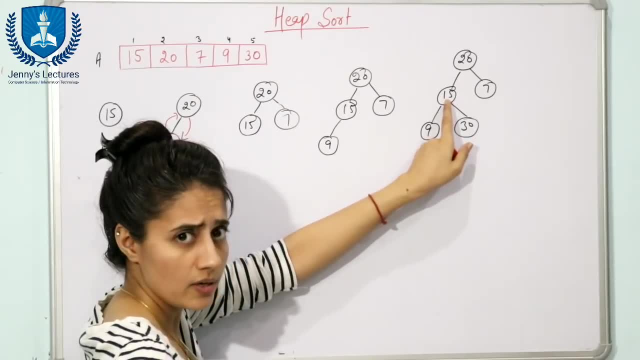 30 would be inserted to the right child of this 15. here we have 30. now again, check, find out. the parent of this 30. parent of 30 is 15 and 15 is less than 30 and that is not possible in maxi. 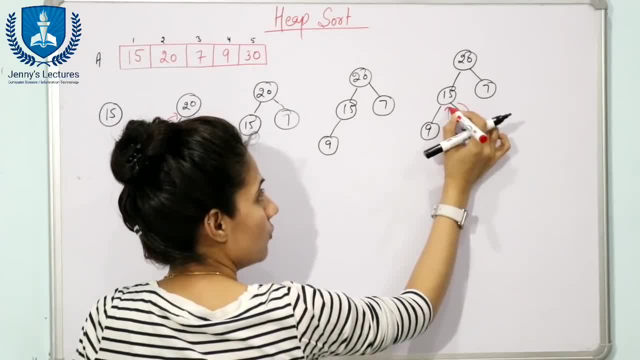 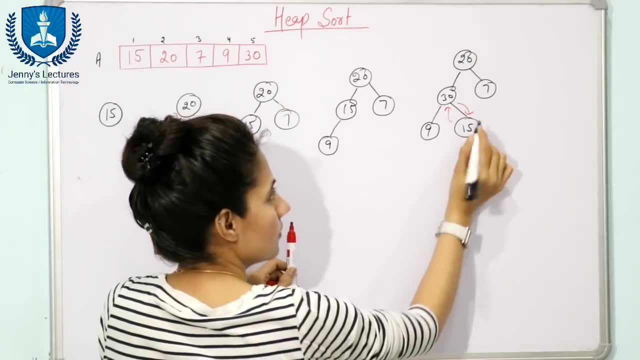 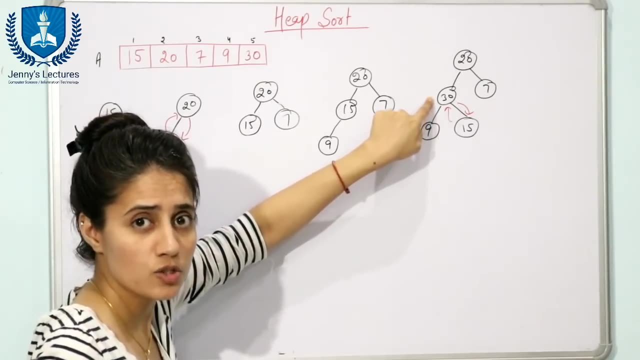 now you have to do what swapping: 30 would go up, so here you will write 30 and 15 would go down. here you will write 15. now 30 is here. now, you are not done with this. you are. you are supposed to check this with its parent. we will keep on. we will keep on checking this inserted element with its parent. 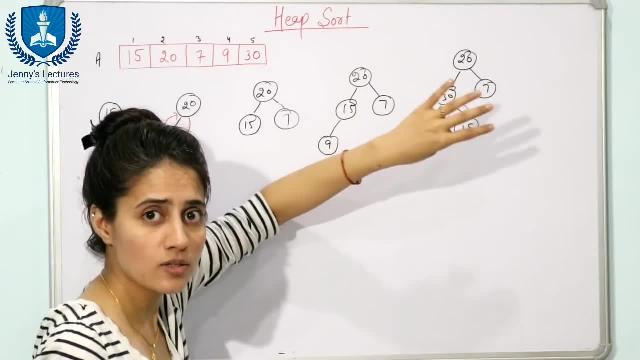 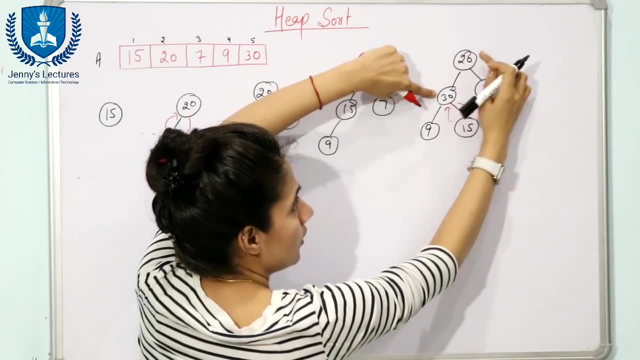 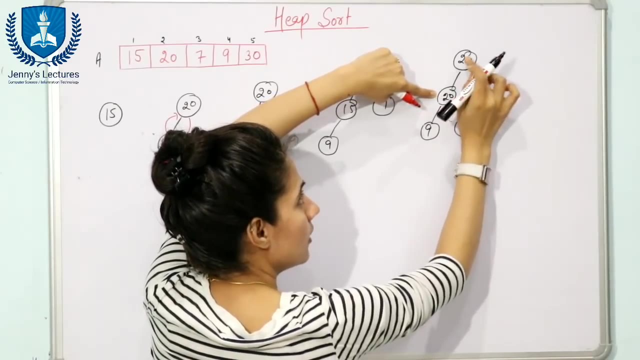 till we reach to the root element. fine, we have already discussed this concept in when we were discussing maxi pencil insertion. now again, find out: parent of 30, now parent of 30, is 20 and 20 is less than 30. so that is not possible. again, we will do what swapping, so here 20 would be there and here 30 would be. 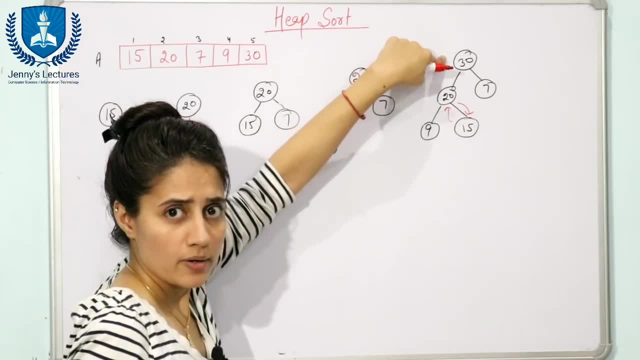 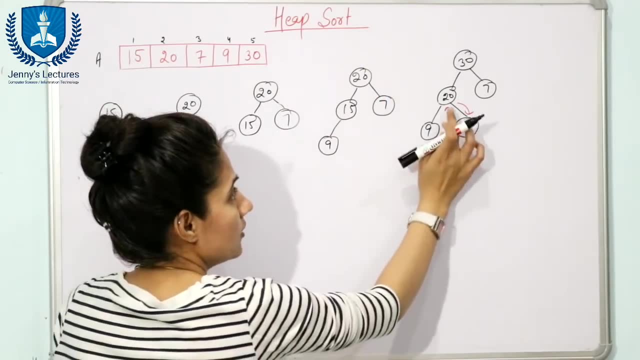 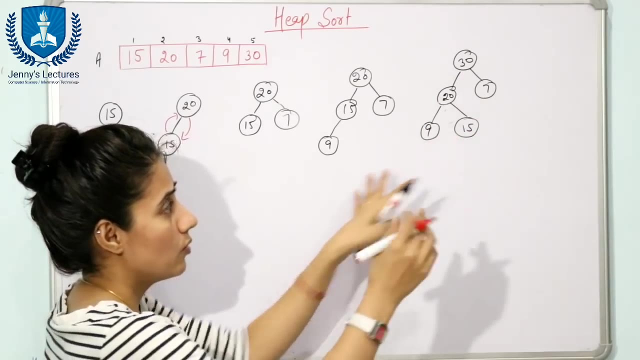 now 30 is the root element. now we are going to stop this comparison, because 30 is 30 is not having any parent node. now, fine, so this is now our maxi after inserting this data. now, this is our maxi. now, now, that array would be inserted to the right child of this 30, and now we are going to 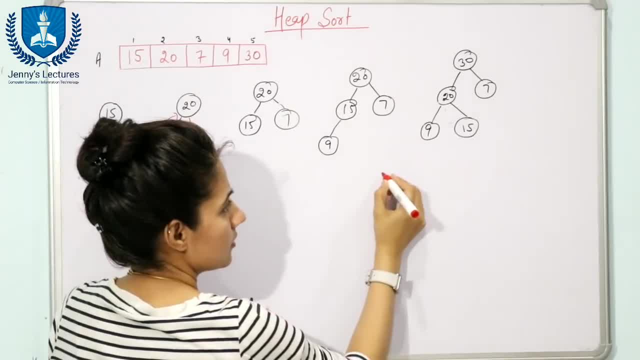 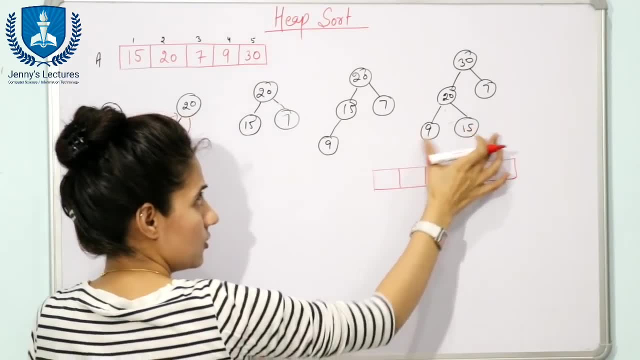 see the element of 30, again nowaguaan. you can see what is the movement. this is what is the movement of this array. gives you the trained being. all these are present elements of the tree. you have a certain element either, the repeated once in a row, clean line agency and the array. 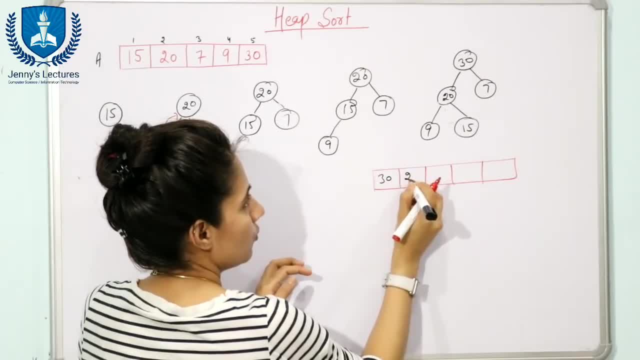 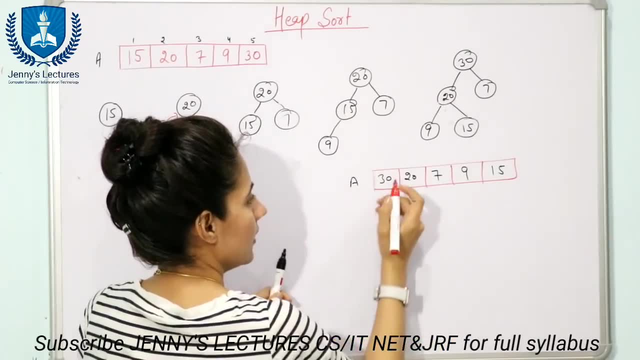 would, can you can? it would represent a tree. we have area in this between 11 and 11 to be play this. we have 30, we have 10, we have 15, we have 4, or we have 15 enemies- 9 out of us four, we have 20- makes up a keluar. come from this tree. we are opening clip that has 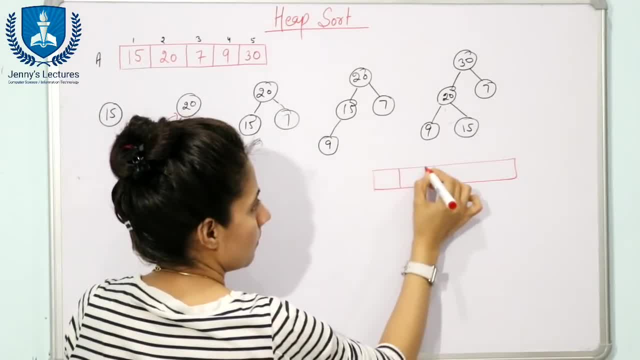 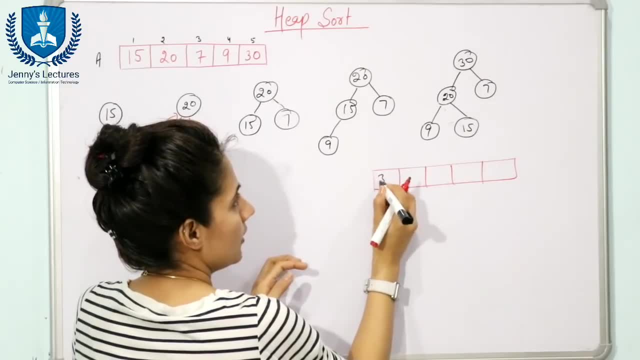 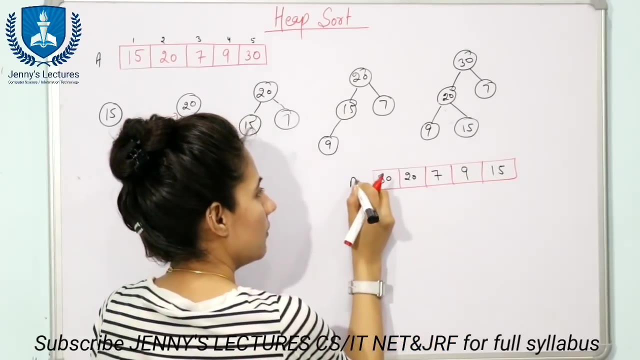 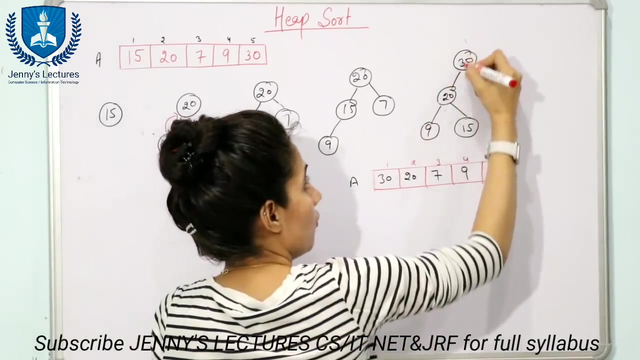 you can, you can. how do you can represent this, this tree, into this array form we have: first element is 30, then we have 20, then we have 7, level by level and from left to right. then we have 9, then we have 15. array name is a and index is 1, 2, 3, 4 and 5, right like indexes are 1, 2, 3, 4. 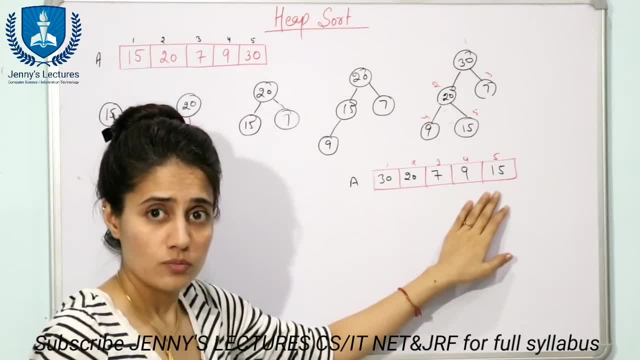 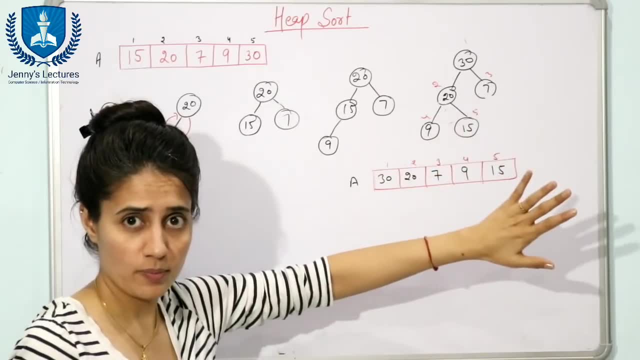 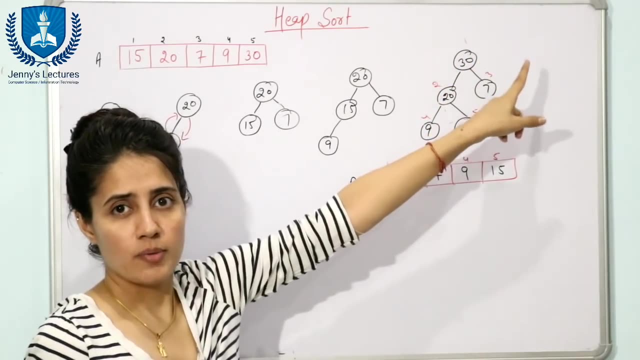 and 5 now the. this is the array now. now second step is: first step is over building a max heap. next step: you are you are supposed to delete data from max heap one by one. how data is to be deleted, that we have already discussed with example. always the data from root element would be deleted from a heap. 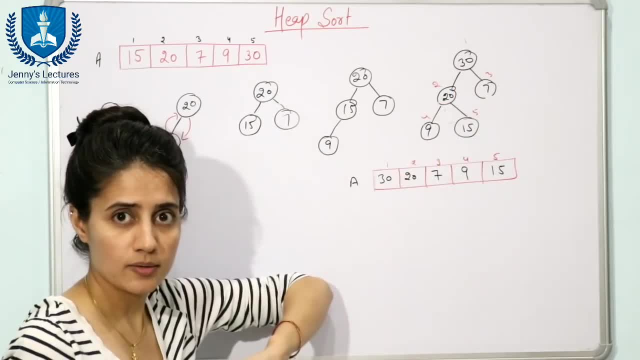 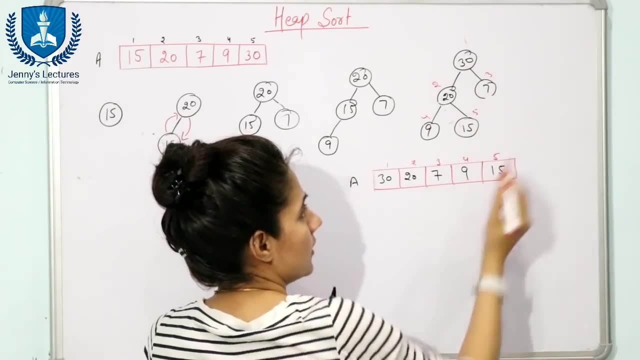 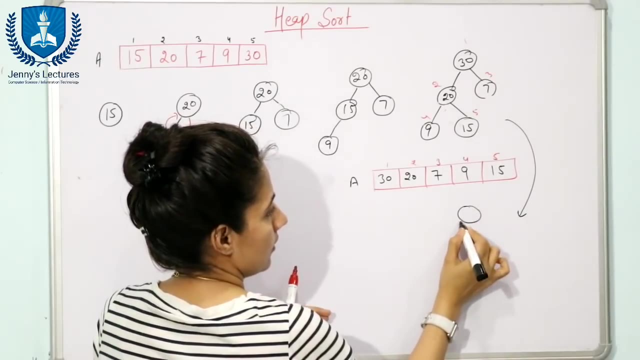 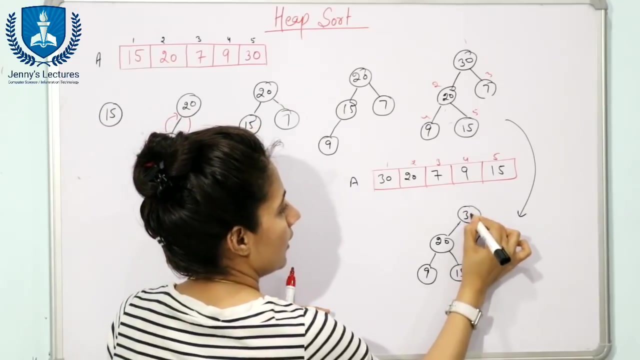 you cannot delete any data from the heap. always the root element would be deleted. in max heap, the root element would be the largest element. fine, now next step is deletion. so after deletion, the tree would be something like this: here we have 20, here we have 7, here we have 9, and here we have 15 and here we have 30. so we have: 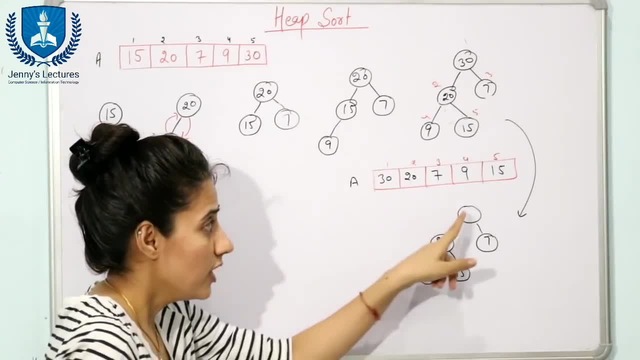 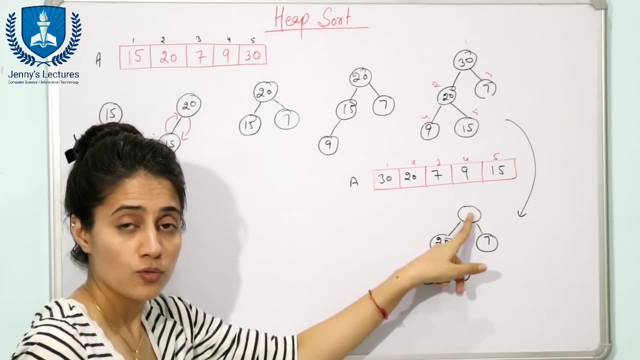 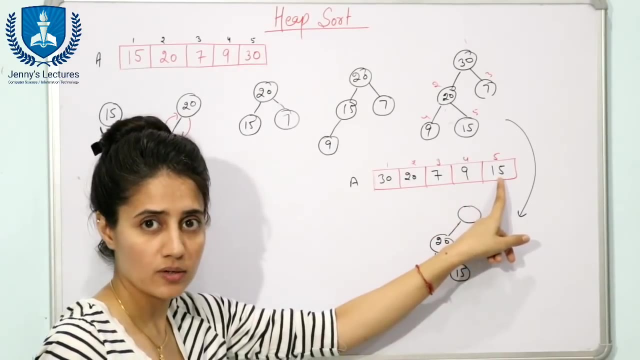 deleted this 30 right now. which element is there? which element is to be placed here instead of this 30? because we have deleted the root element now. always we used to put the last element. the last element in this tree is 15, or you can say: the last element in this array is 15.. 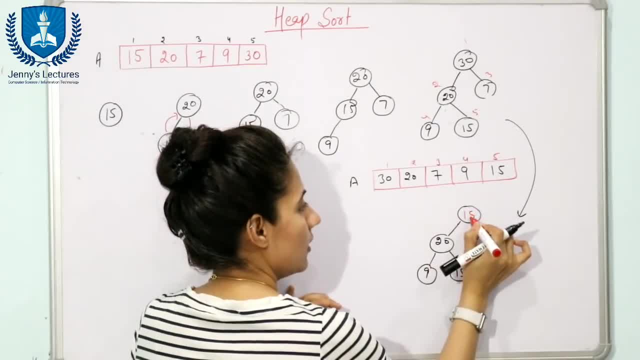 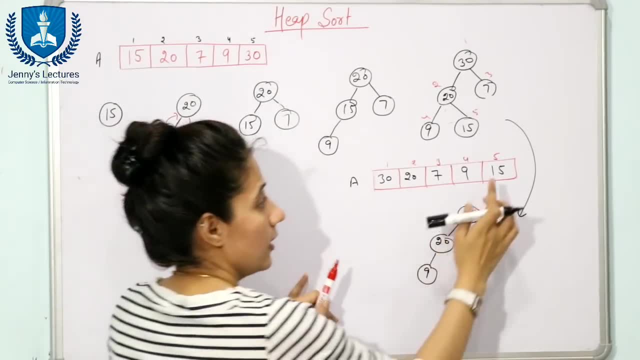 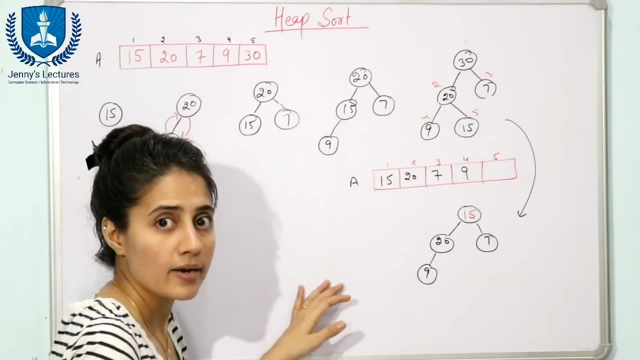 fine, so 15 would be shifted here. now, here we will write 15 and 15 would be deleted from here. okay, now this in this array- how array is to be updated- 15 is inserted here and and we have deleted 30 and you are going to sort this array. so now see. 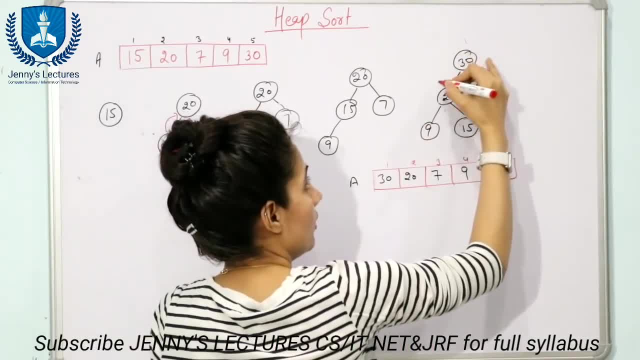 a variety. on the left, a number, ok, come from. on the right also, we are placing a select. those are the three tag tag 해 layer. Alright, okay, now clarion. you can see. the first element are 3, 2, 4 and there so 2 aH settab senki. 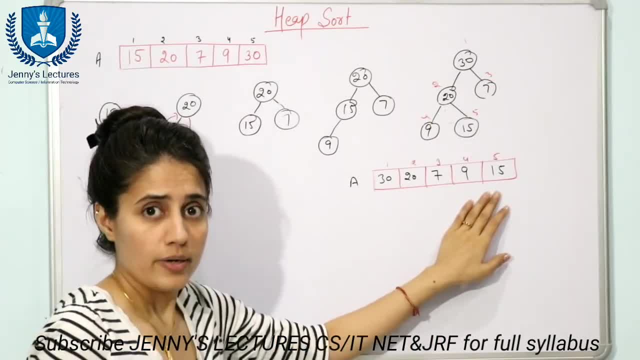 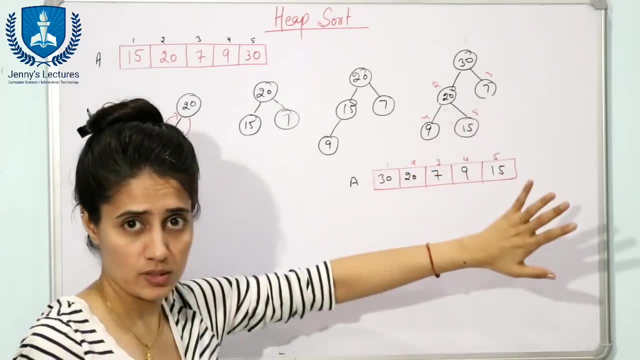 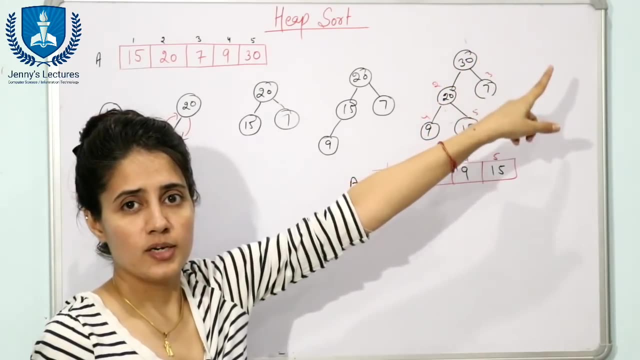 4 and 5. now this is the array now. now second step is: first step is over building a max heap. next step: you are you are supposed to delete data from max heap one by one. how data is to be deleted, that we have already discussed with example. always the data from root element would be deleted from a 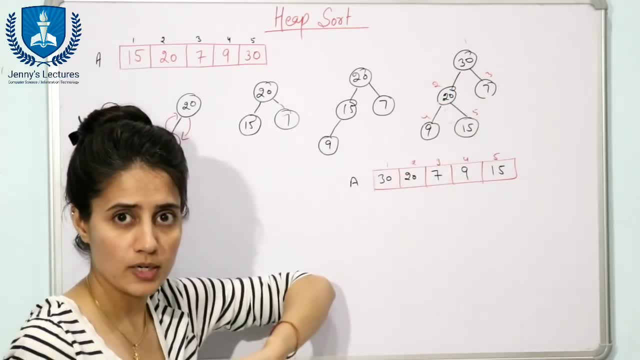 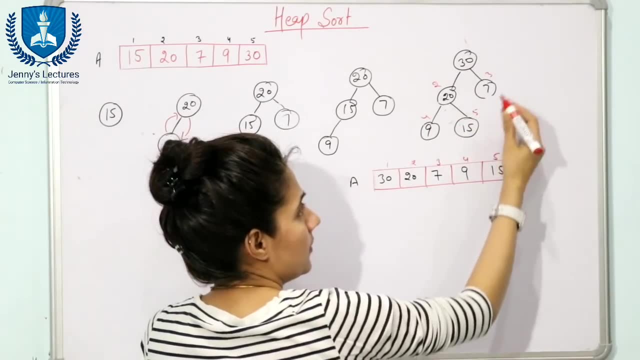 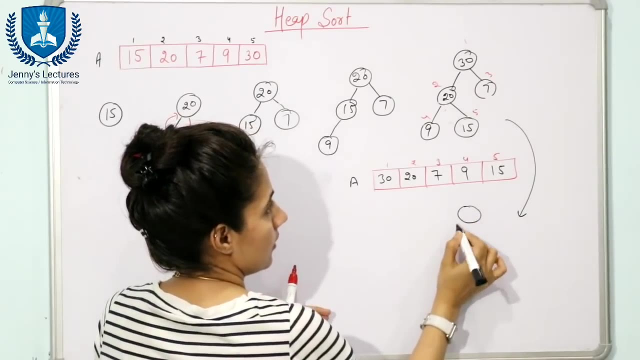 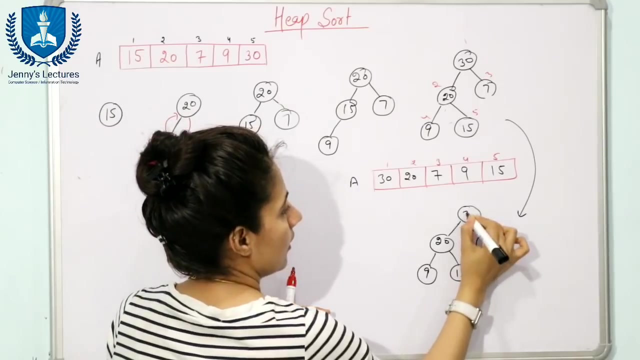 heap. you cannot delete any data from the heap. always the root element would be deleted. in max heap, the root element would be the largest element. fine, now next step is deletion. so after deletion, the tree would be something like this: here we have 20, here we have 7, here we have 9, and here we have 15 and here we have 30. so we 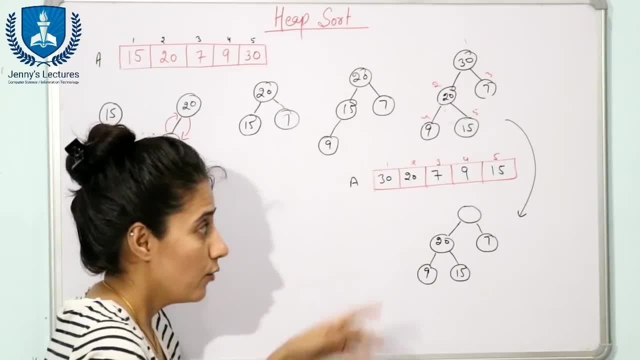 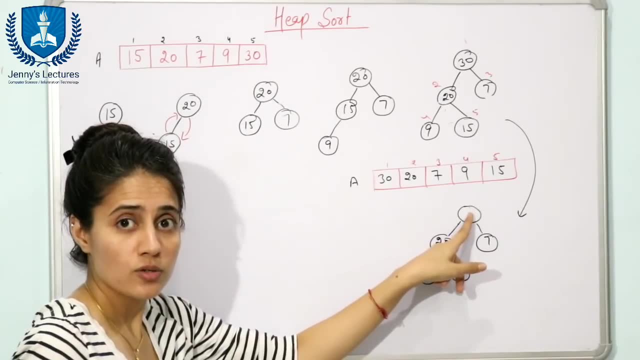 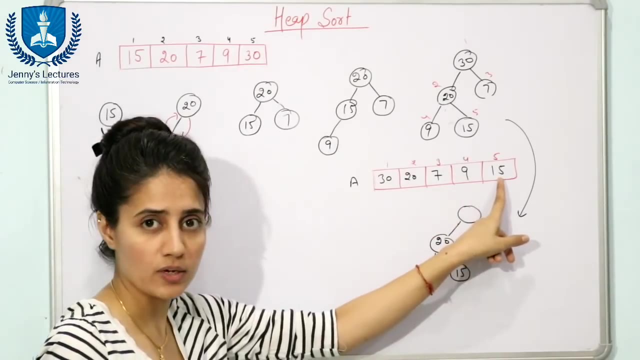 have deleted this 30 right now. which element is there? which element is to be placed here instead of this 30? have deleted the root element now. always we used to put the last element. the last element in this tree is 15, or you can say: the last element in this array is 15. fine, so 15 would. 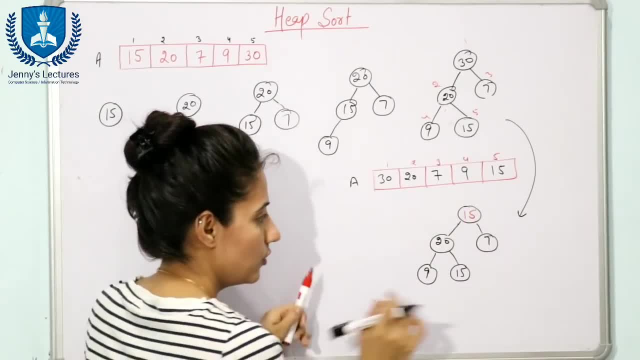 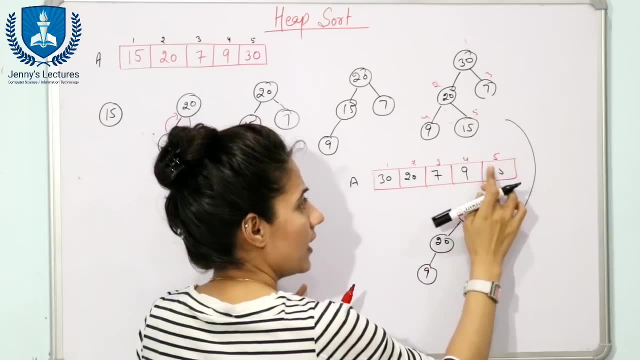 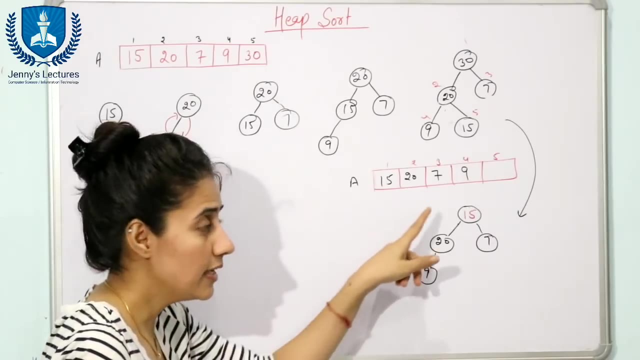 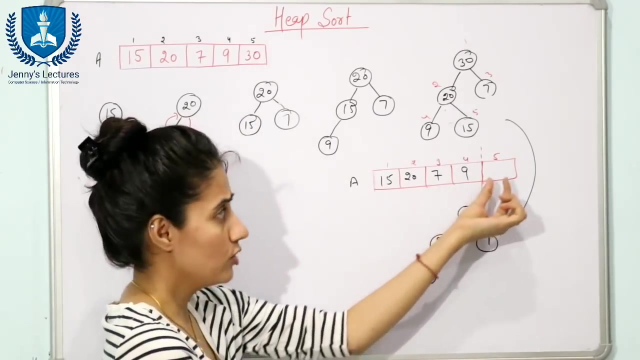 be shifted here. now, here we will write 15, and 15 would be deleted from here. ok, now this: in this array- how array is to be updated- 15 is inserted here, and and we have deleted 30 and we are going to sort this array. so now see: now heap is from here to here. now this: 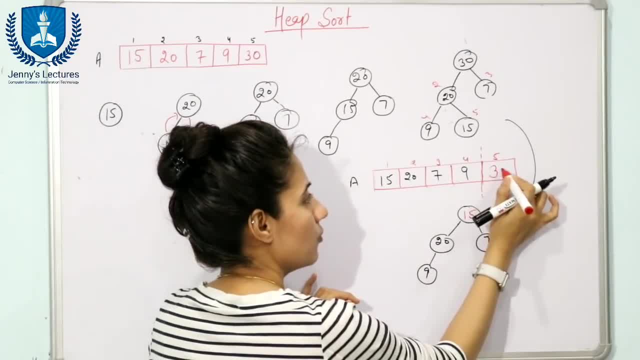 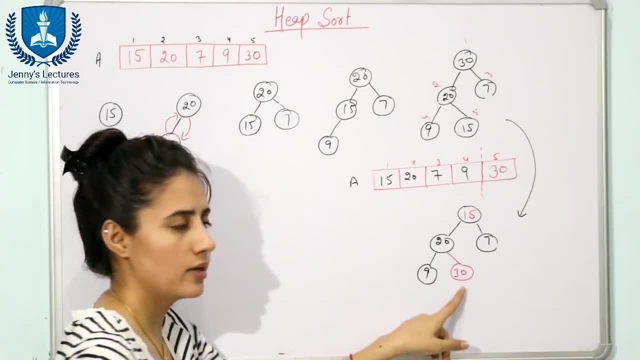 space is free, so the deleted element would be placed here. now. we will place 30 at this place in the tree also. you can, you can. you can draw something like this here. you can put 30, ok, but I am not going to put 30 here, I am just updating the array I am deleting. 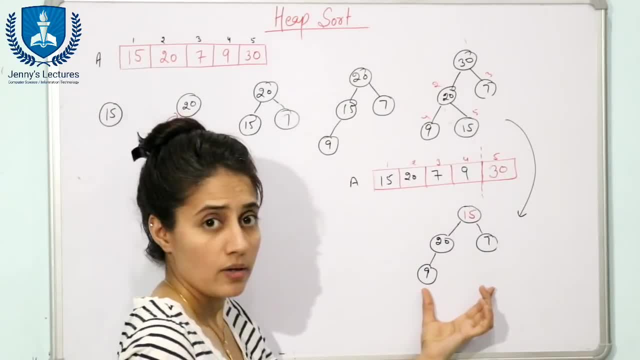 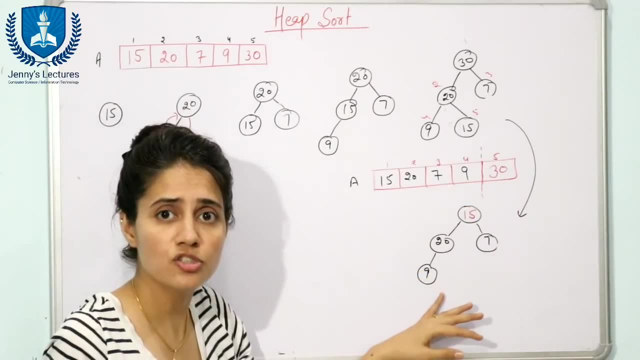 30 from here. now this is the tree now after the deletion. it's not like that deletion is done, Now delete. next element, that is 15.. Now, after each deletion, you have to check: is this tree still satisfying the property of max heap or not? 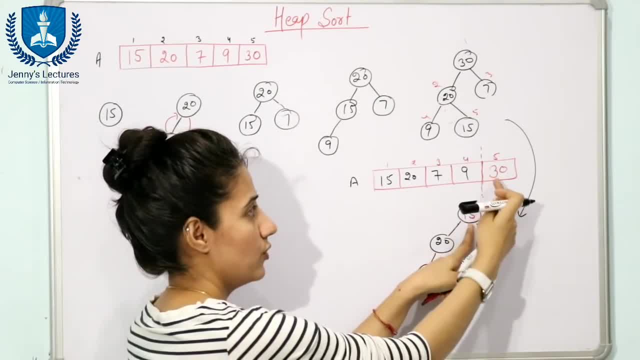 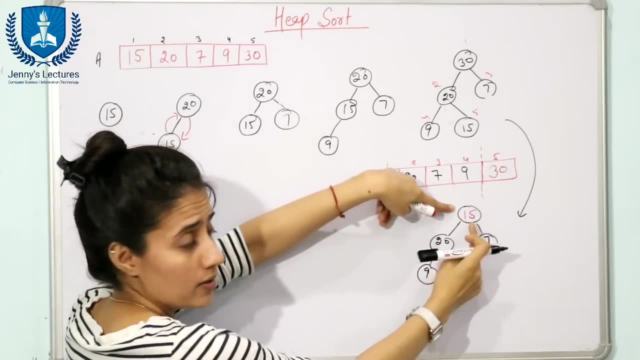 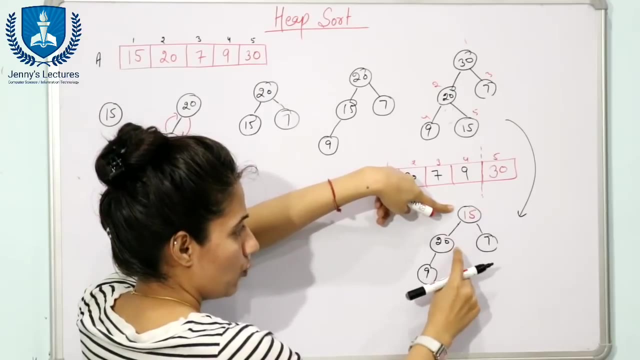 Check out. This is the element which we have shifted from last to here Now. you have to check from here. Now find out the child children of this element. We have two children. One is this one and one is this one. Now check out which one is larger. that is 20.. 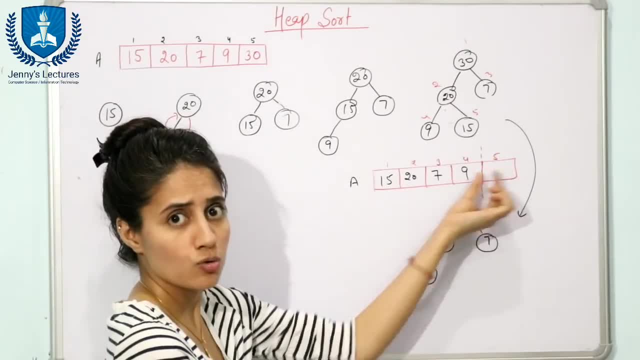 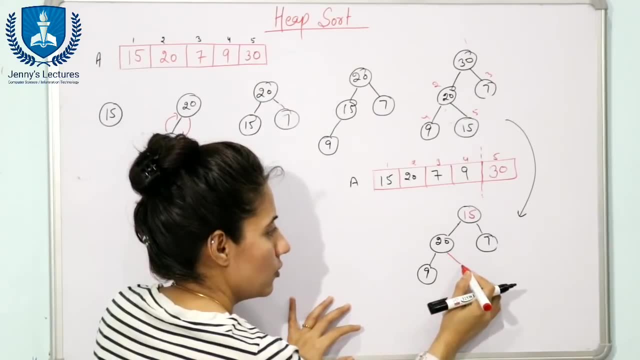 now heap is from here to here. now this space is free, so the deleted element would be placed here now. we will place it here here now. we will place 30 at this place in the tree also. you can, you can, you can draw something like this here. you can put 30, okay, but I am NOT going to put 30. 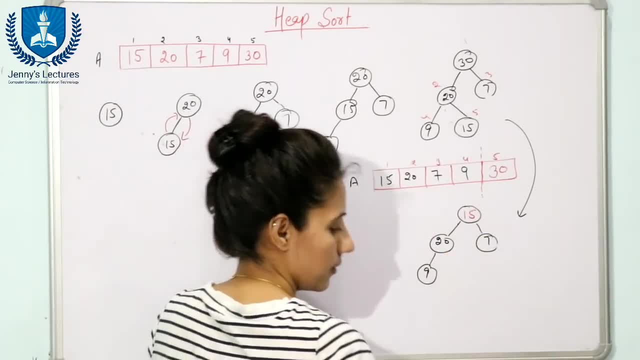 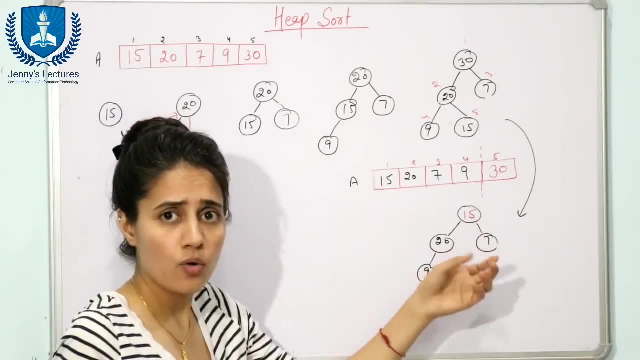 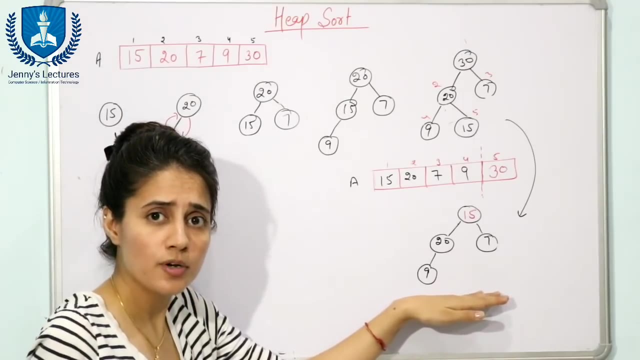 here. I am just updating the array. I am deleting 30 from here now. this is the tree now after the deletion. it's not like that deletion is done now delete. next element, that is 15. no, after each deletion you have to check: is this tree still satisfying the property of max heap or not? check out this is the. 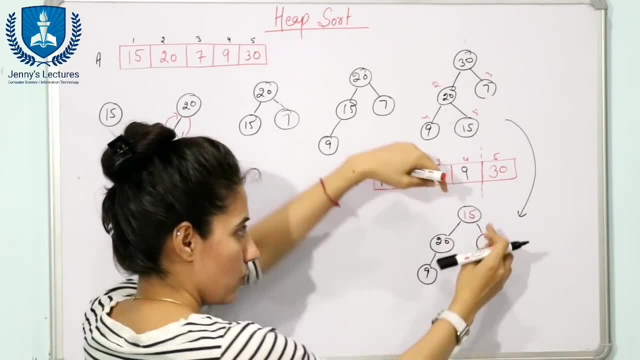 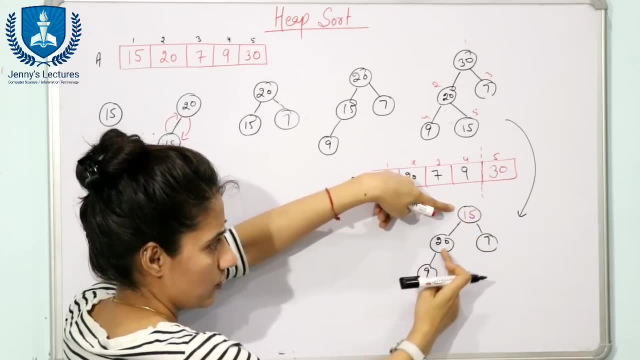 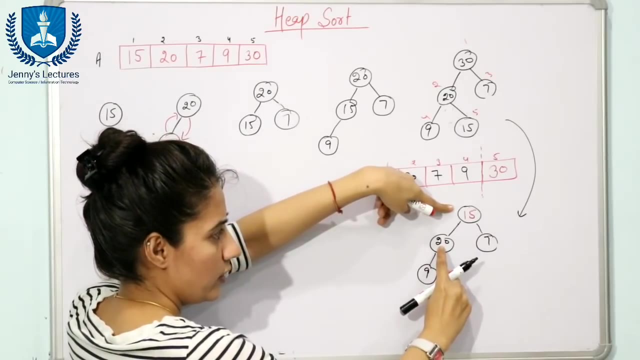 element which we have shifted from last to here now. you have to, you have to check from here now. find out the child, children of this element. we have two children. one is this one and one is this one. right now, check out which one is larger. that is 20 now. 20 would be compared with this 15. now. this 15, 15 is. 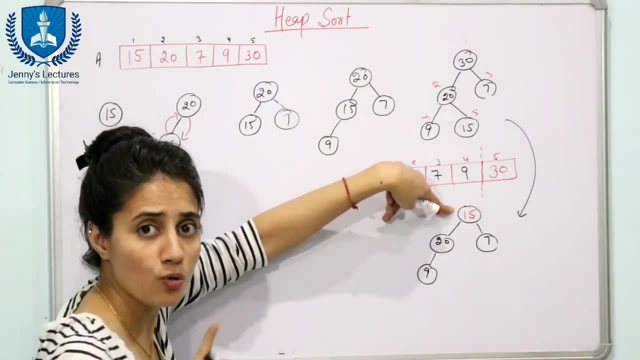 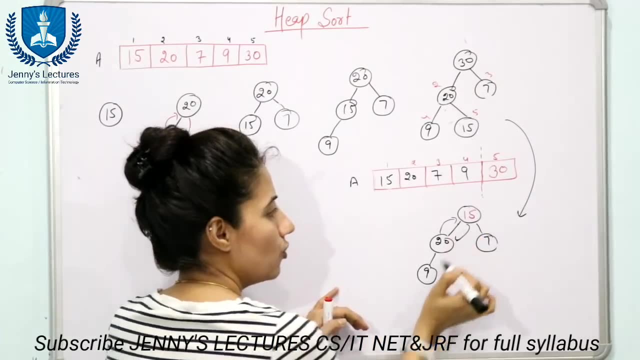 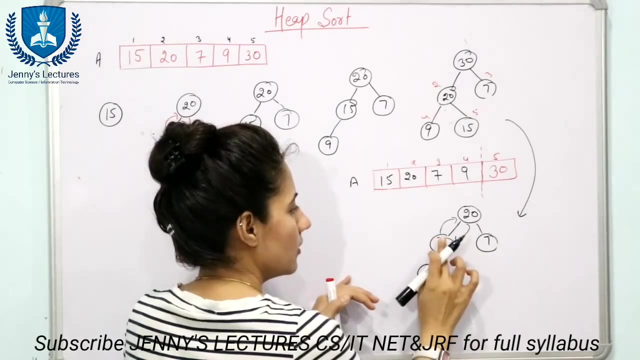 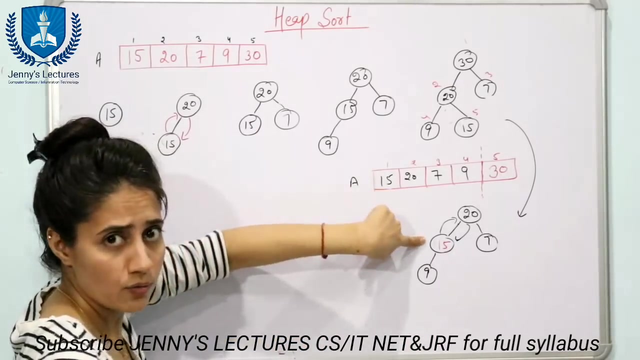 parent, and parent is less than its child, and that is not possible in max heap. now you have to do what swapping. now, 20 would go up and 15 would go down, right. so here we will write what 20, and here we will write 15. now, here we have 15. now, see, it's not done, we have done one. 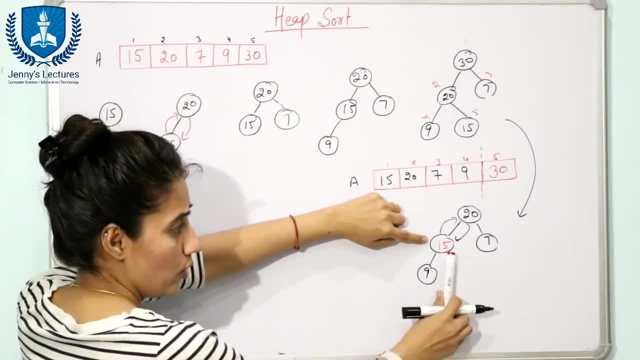 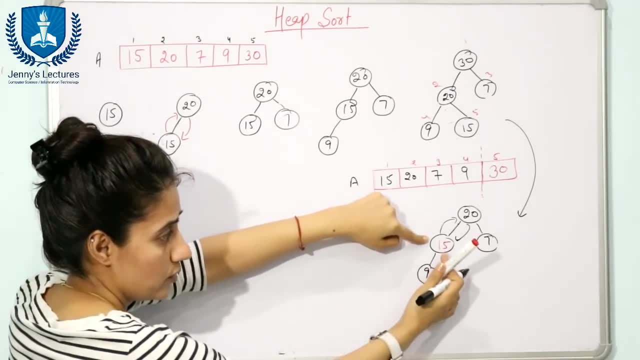 swapping and we are done with this. no, again, again. you have to, you have to tell, you have to find out this left and right and you have to find out this left and right child of this 15, and till till we reach to the last level, to the end of. 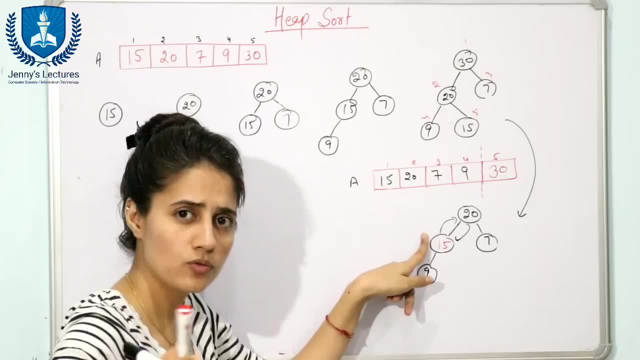 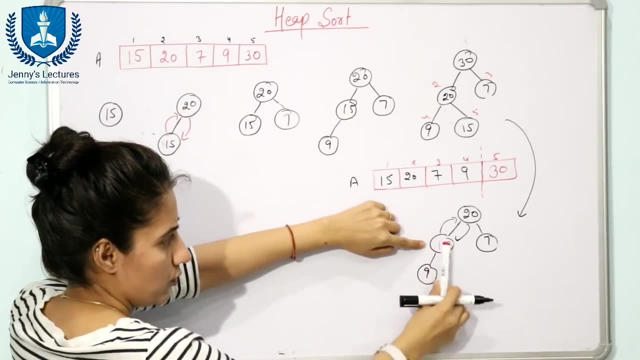 the array until until that. until then you will. you will find out the left and right child. fine, I am going to write down the code also now. 15 left child is 9. we don't have any right child, okay, compare with this one. 15 is parent 9, 8. 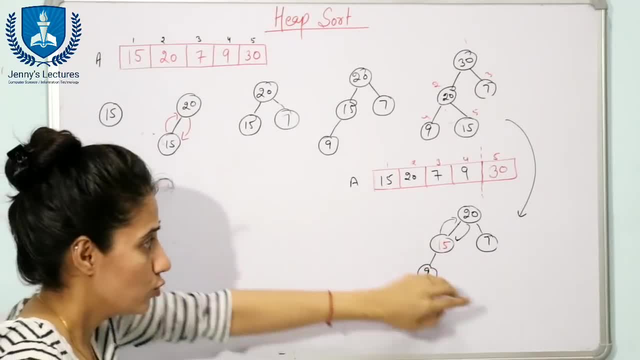 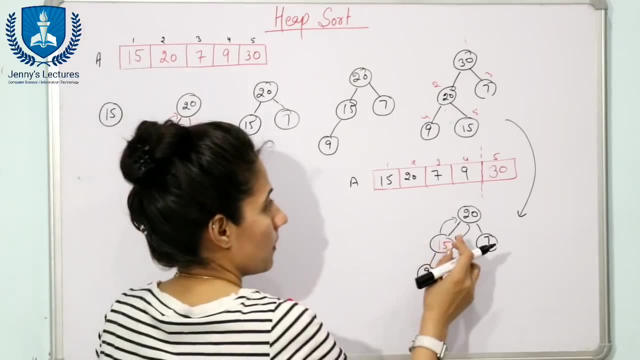 child and 15 is greater than 9, and that is fine. no swapping would be done. so this is now max heap, fine. now next next element would be 20. 20 would be deleted. now, see, we have. we have updated in this pre. when you are. 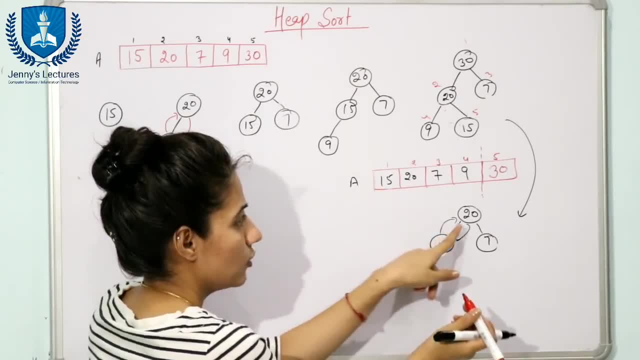 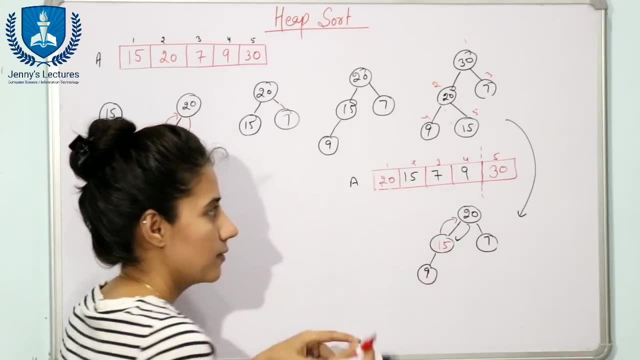 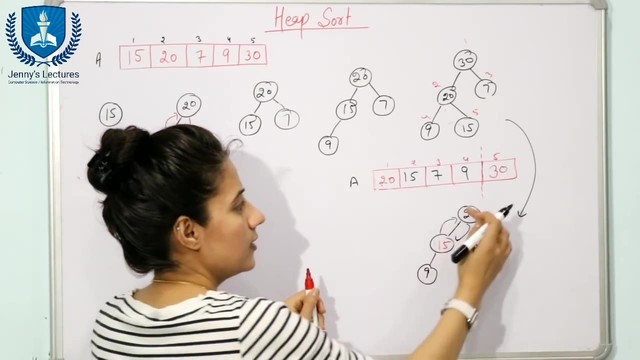 going to update in this array, then how? how this array would be updated. see, 20 would be, 20 would go there and 15 would go there right after this. this updation in this array. this would be the array now. now, next element to be deleted is: 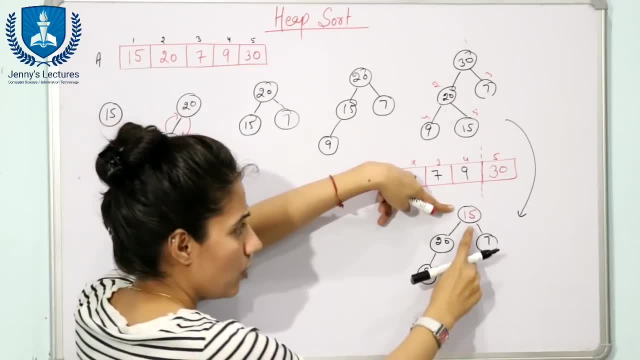 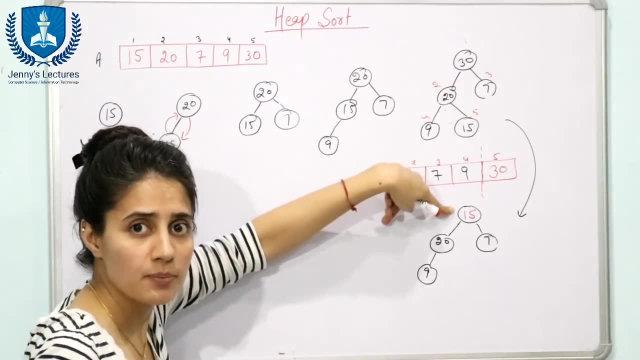 Now 20 would be compared with this 15.. Now this 15. 15 is parent, and parent is less than its child, And that is not possible in max heap. Now you have to do what Swapping? Now 20 would go up and 15 would go down. 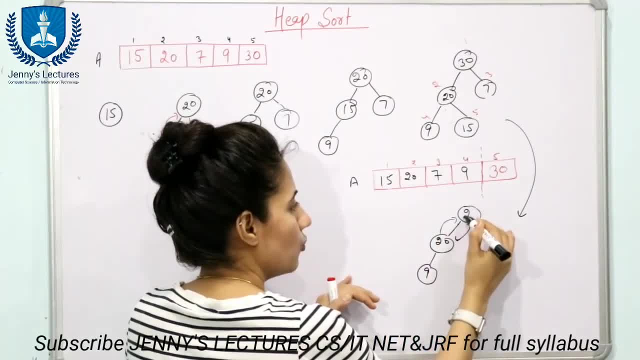 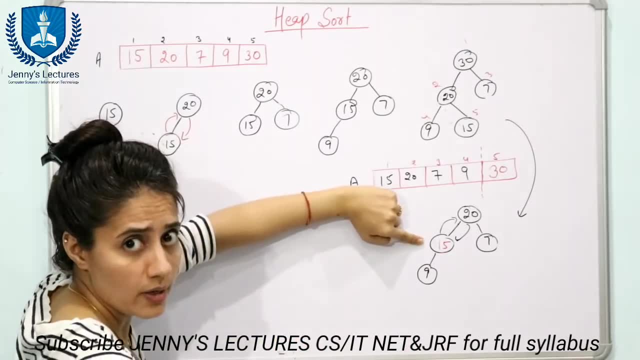 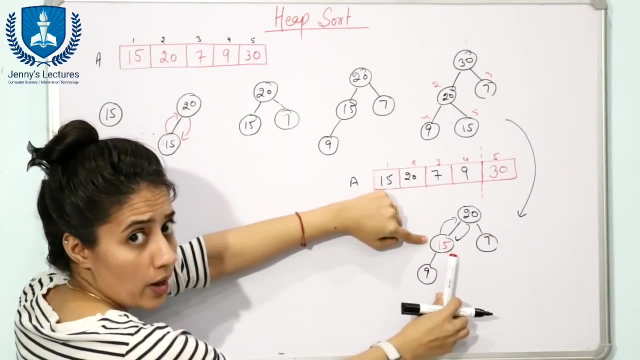 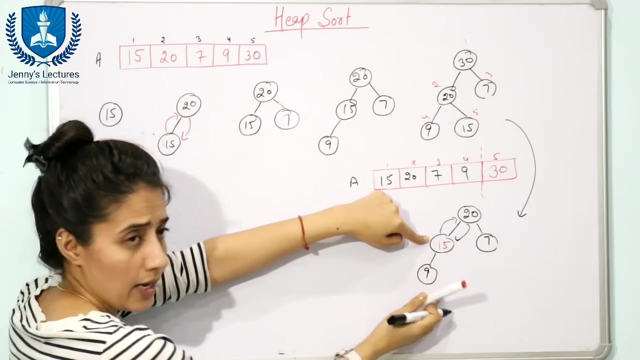 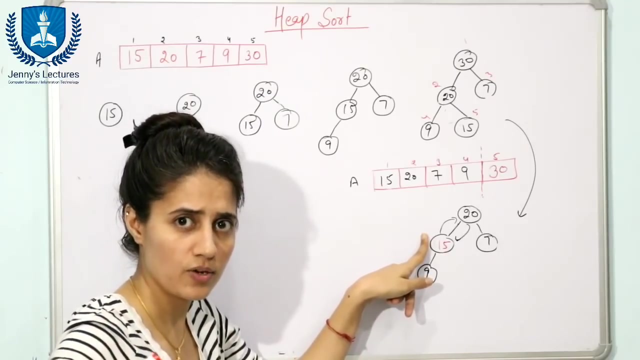 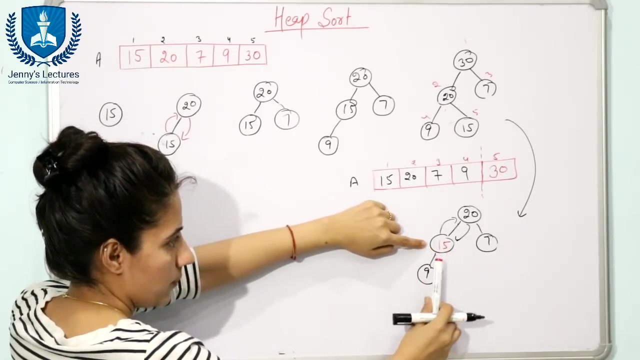 Right. So here we will write what? 20, and here we will write 15.. Now, here we have 15.. Now, see, it's not done. We have done one swapping and we are done with this. No again, again, you have to, you have to, you have to find out this left and right child of this 15. and till till we reach to the last level, to the end of the array, until until that, until then you, you will find out the left and right child. fine, I'm going to write down the code also. now, 15 left child is 9. we don't have any right child. okay, compare with this one: 15 is parent, 9, 8 child and 15 is greater than 9. and that is fine. no swapping would be done. 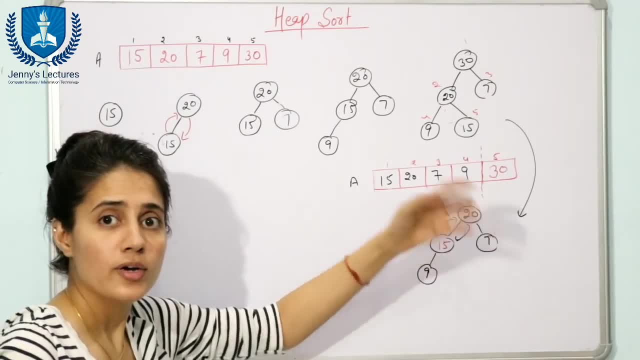 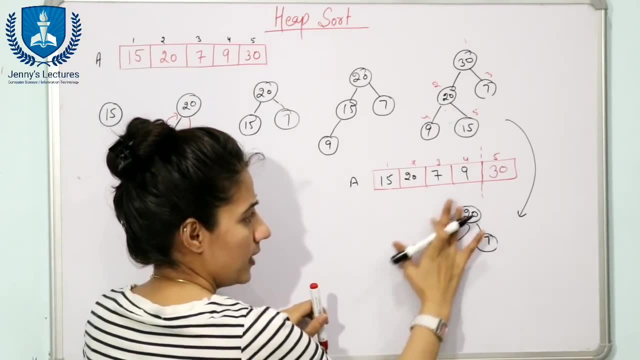 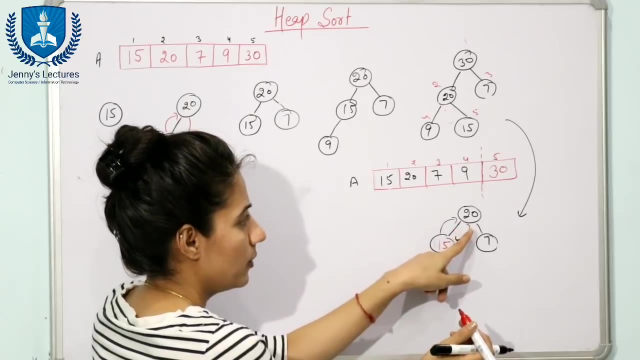 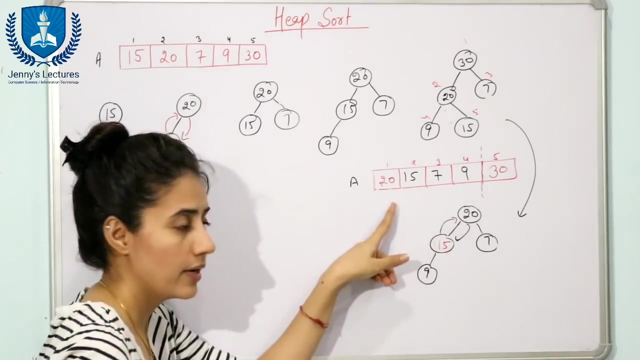 So this is now max heap. Fine, Now. next next element would be 20. 20 would be deleted. Now, see, we have. we have updated in this pre. when you are going to update in this array, then how, how this array would be updated. see, 20 would be, 20 would go there and 15 would go there. right after this, this updation in this array. this would be the array now. 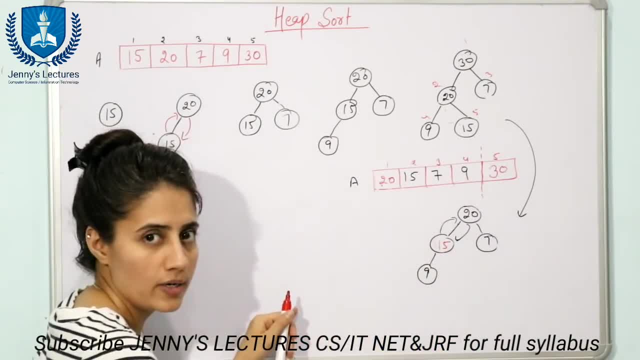 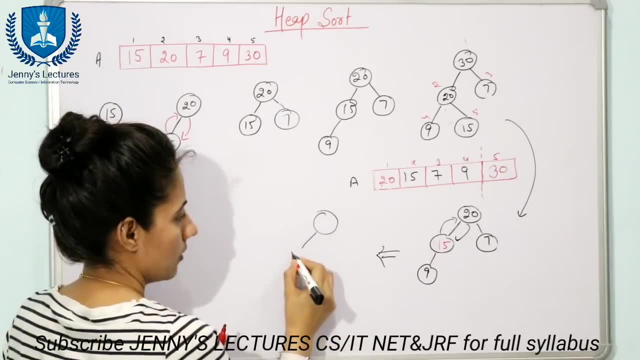 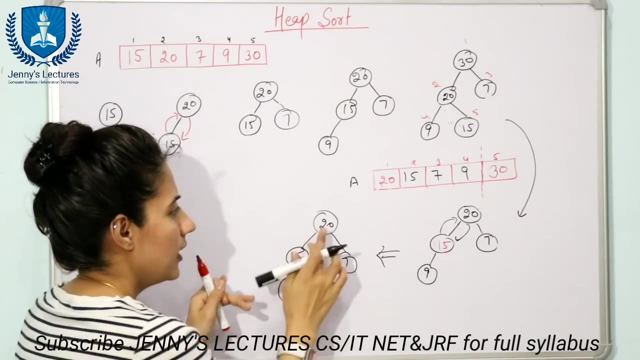 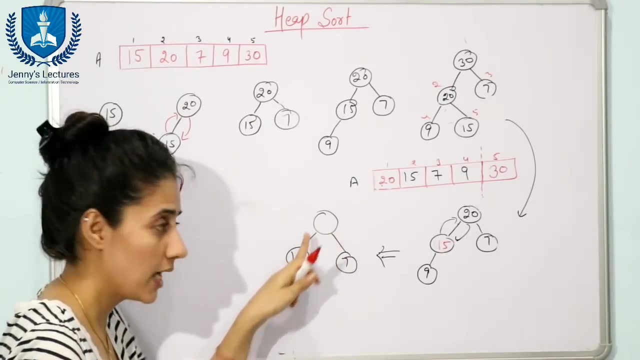 Now next element. Next element to be deleted is this 20. now, after deletion of this, 22 and 20 would be deleted here. now, next 20 would be deleted. now we have deleted this 20 and the place of this 20, we will shift which element. the last element, last element, is 9, so 9 would be shifted here. right, 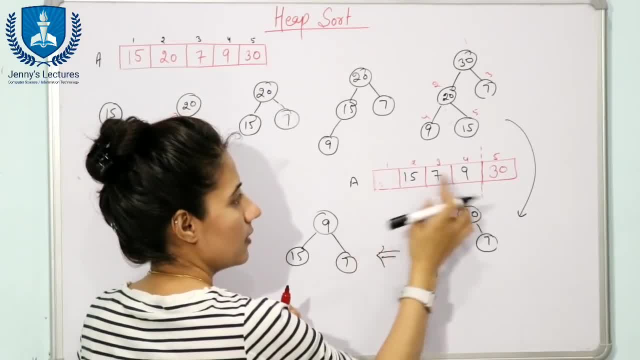 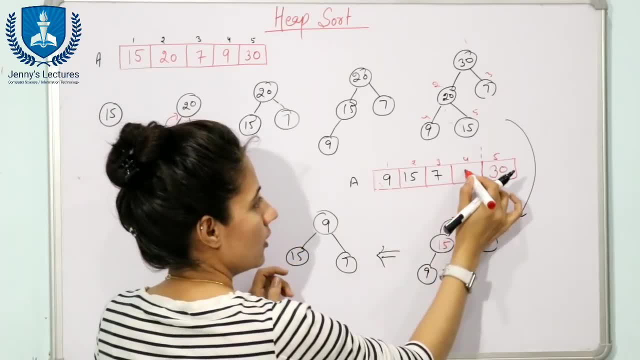 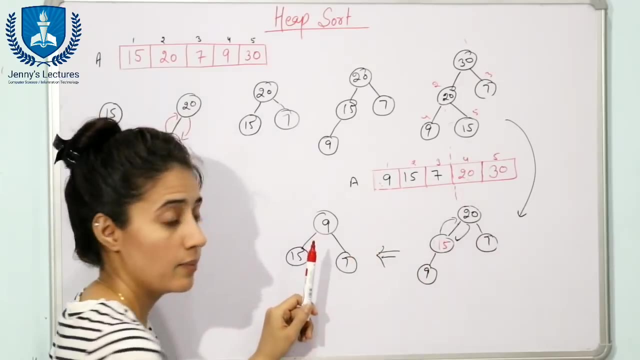 And if you are going to update In this area, then 20 would be deleted. this last element in this array is now heap is from 1 to 4. 9 would be shifted here and we will shift this 20 here. now this heap would be from 1 to 3. size had has been reduced again by 1. fine, 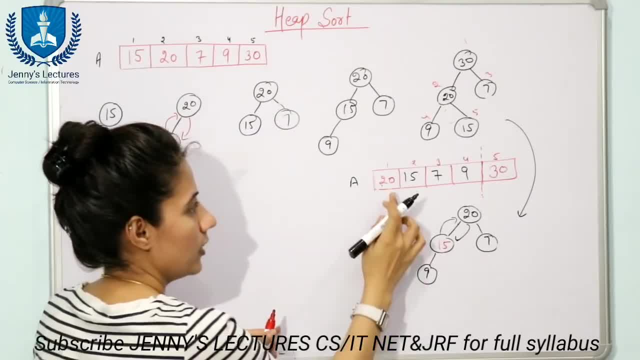 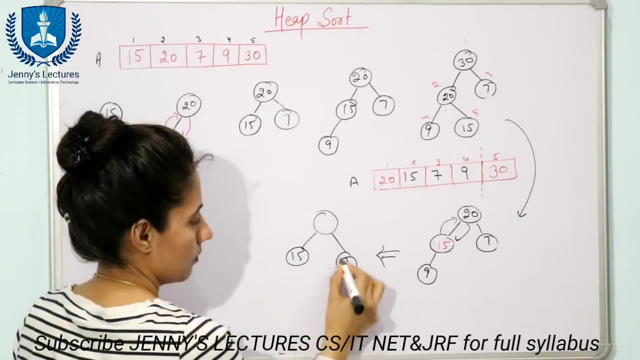 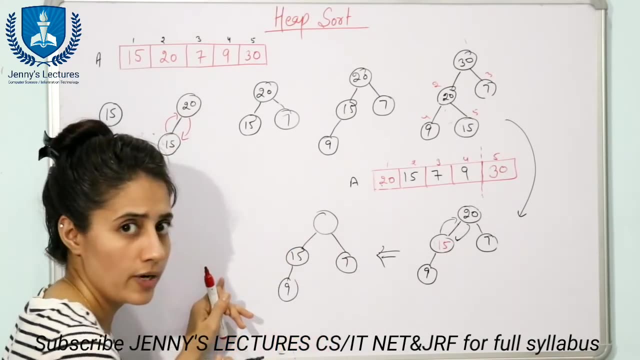 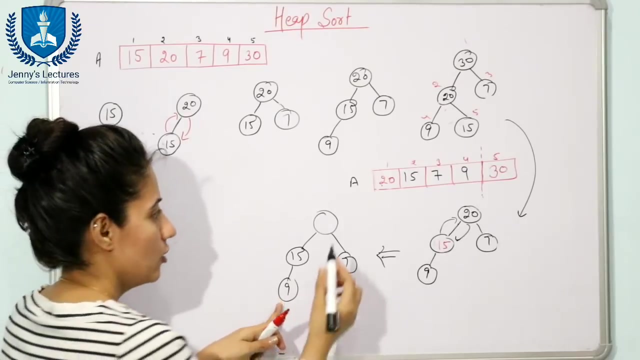 this 20 now, after deletion of this, 22 and 20 would be deleted here now. next 20 would be deleted. now we have deleted this 20 and the place of this 20, we will shift which element the last element. last element is 9, so 9 would be. 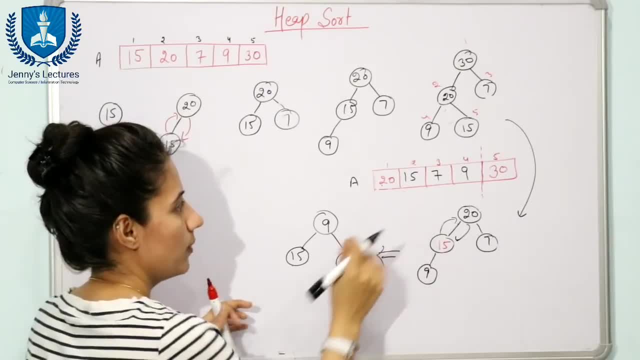 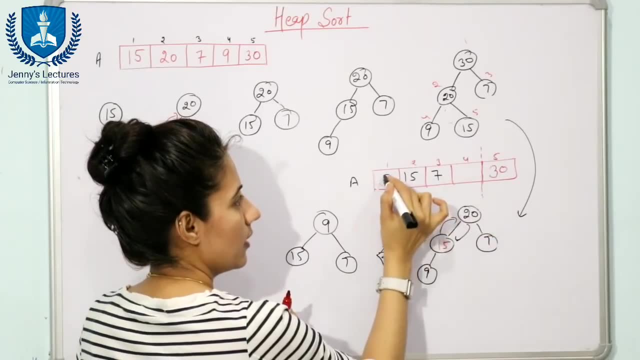 shifted here. right, and if you are going to update in this array, then 20 would be deleted. this last element in this array is now. heap is from 1 to 4. 9 would be shifted here and we will shift this 20 here. now this heap would be from 1 to 3. 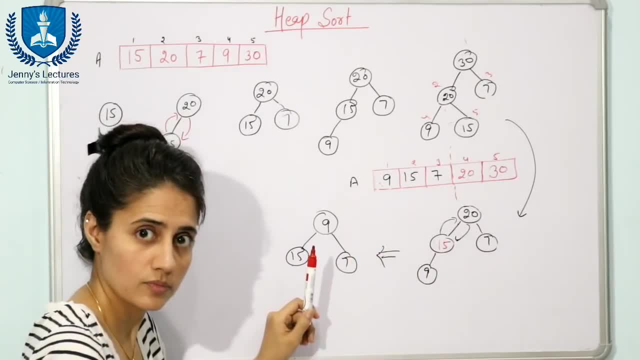 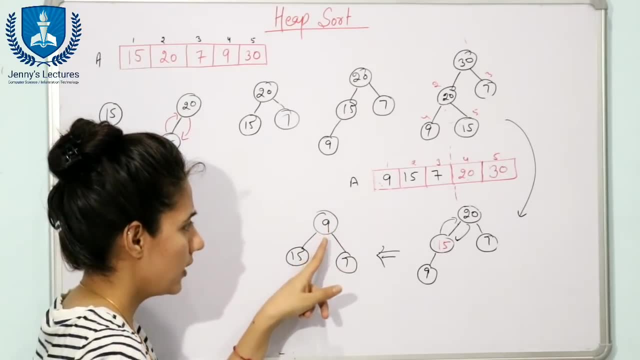 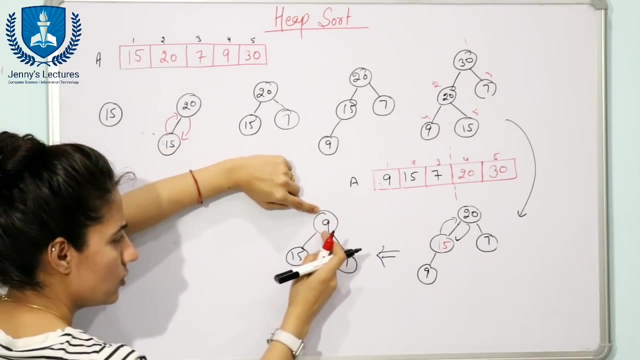 size had has been reduced again by 1. fine, now again check. because of this after, because of deletion of this 20, we have this tree. now now check this is maximum heap or not this? we have inserted this 9 at the starting. now find out, right. the? 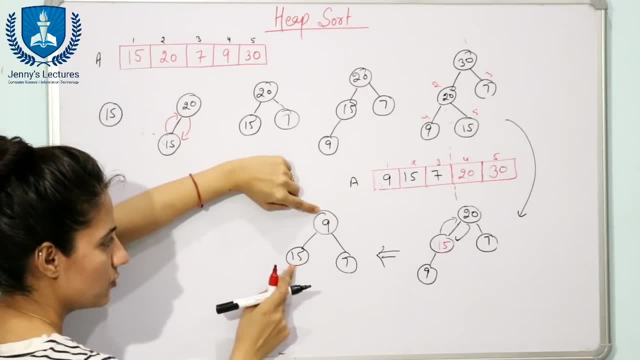 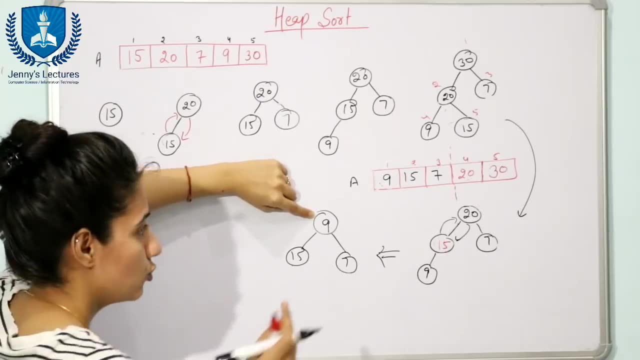 children. of this 9, 2 children are there: 15 and 7. which one is larger? 15, 15 weeks compared with this 9, and this 9 is less than 15, and that is not possible in mix heap. so now swapping would be done: 15 would go up, 9 would go down. so here: 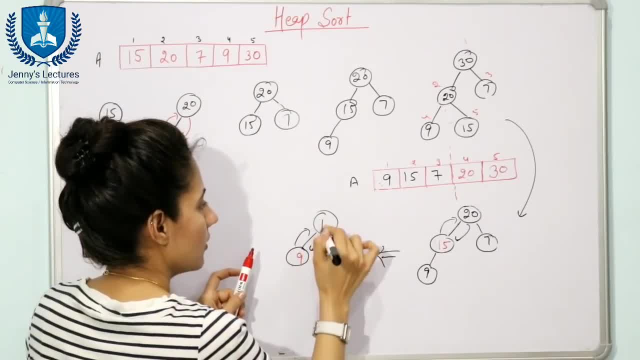 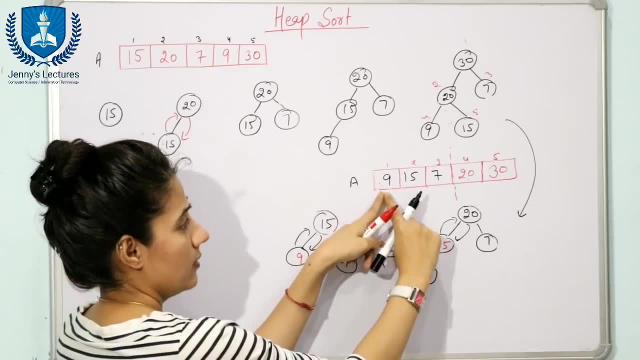 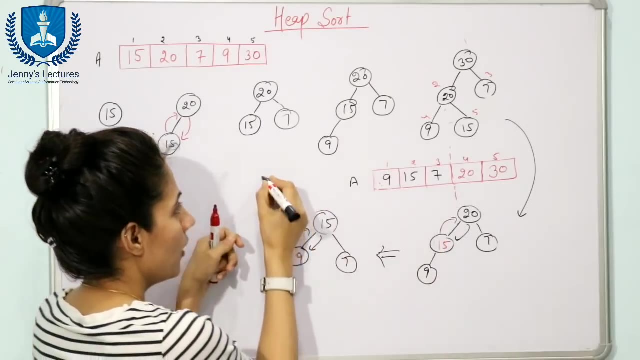 you will write 9 and here you will write 15. the array would also be updated right, right 9. i the see the how, how this right child and left child is to be calculated. we know the formula i value is 1, so the left child would be 2 into i, that is, at second index. right child would. 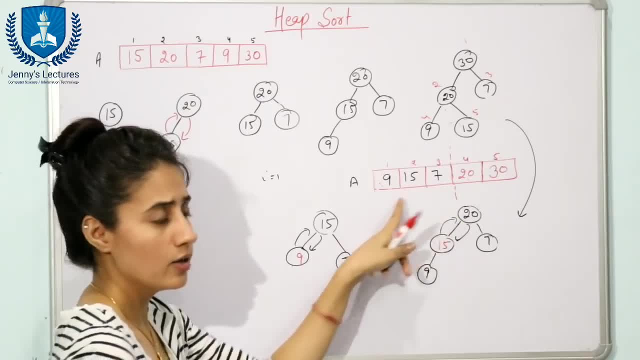 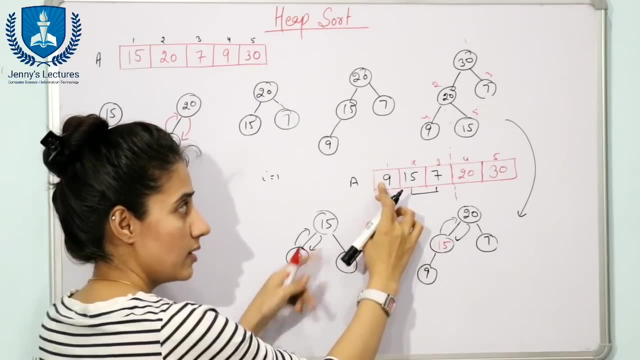 be 2 into i plus 1. that is at third index. 15 and 7 are two children of this 9. which one is greater? 15? 15 is compared with this 9 and 9 is parent, which is less than its child. that is not possible. 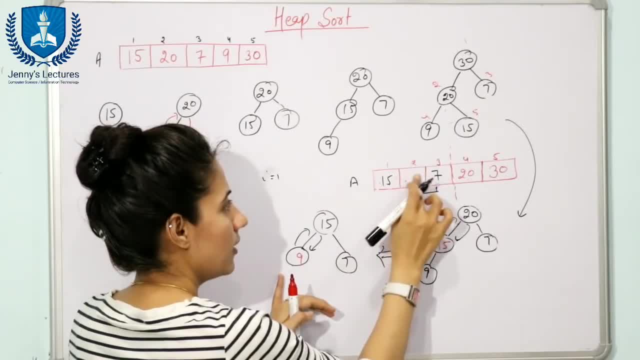 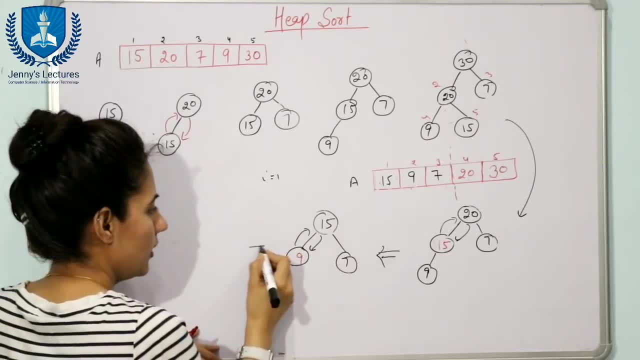 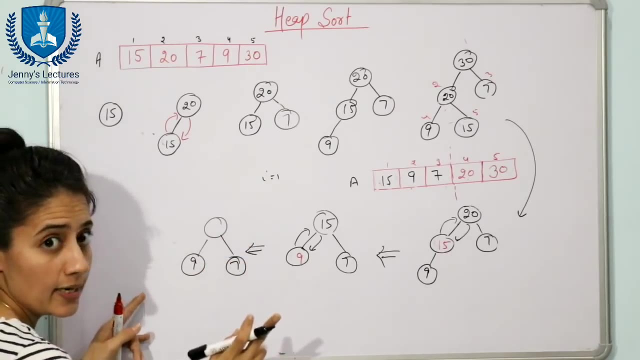 so we are going to shift. so 15 would go here and 9 would go here. now, this is the updated array. this is max heap now. fine, next element would be deleted. that is 15. right, so 15 would be deleted now instead of at the place of this 15. which element is to be there? the last element, last? 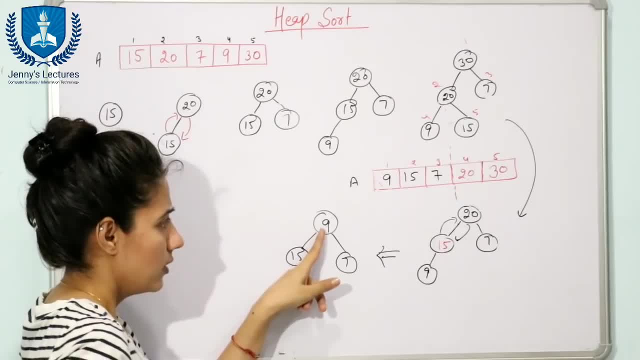 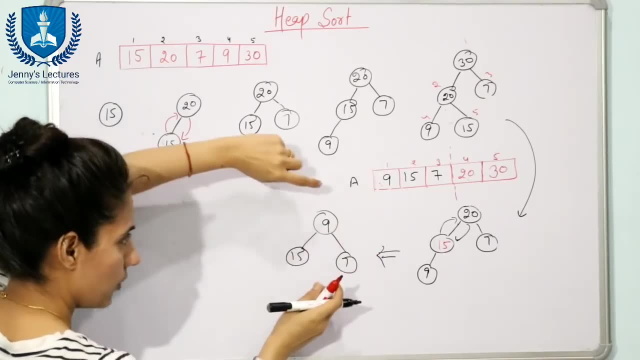 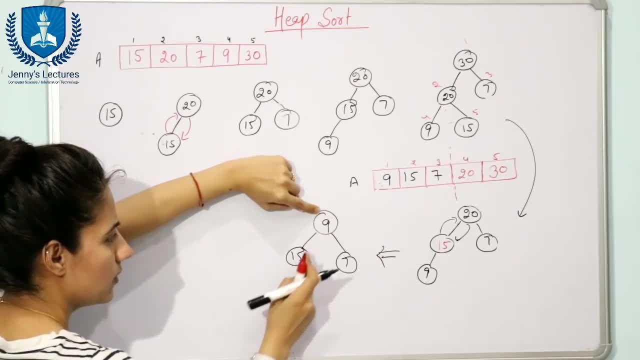 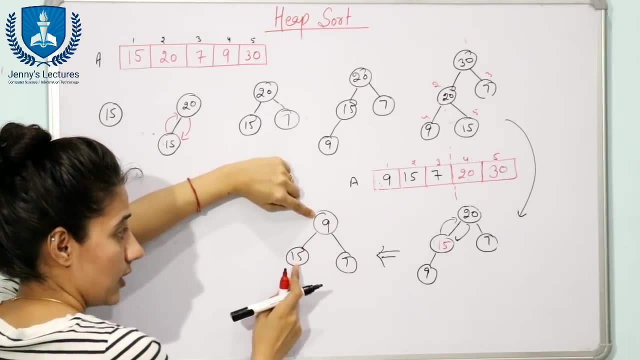 Now check, Now find out right, the children of this nine. two children are there, 15 and 7. which one is larger? 1515- he's compared with this 9 and this 9 is less than 15 and that is not possible in Max heap. 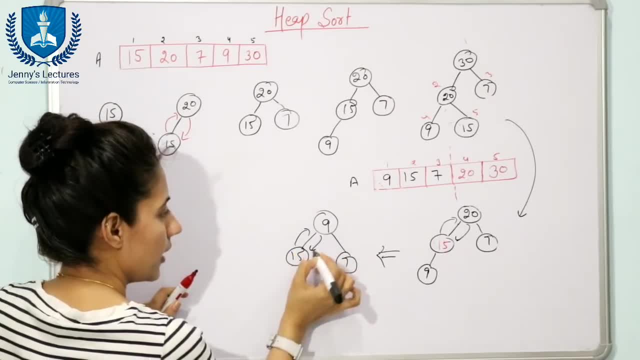 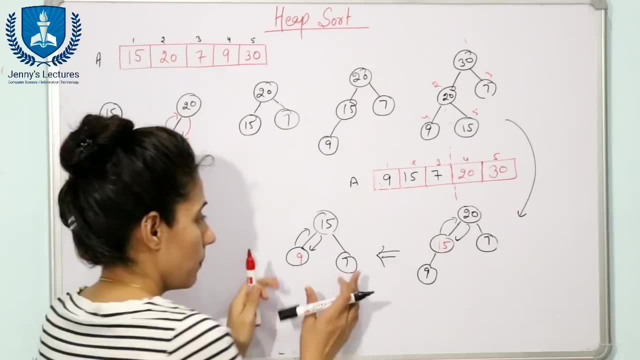 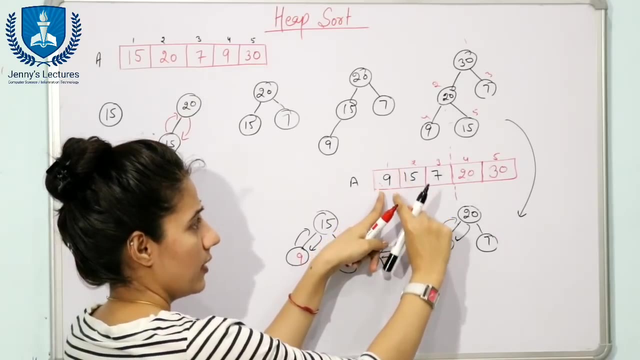 So now swapping would be done. 15 would go up, 9 would go down. So here you will write 9 and here you will write 15.. The array would also be updated right, 9.. See the how this right child and left child is to be calculated. we know the formula. i value is 1. 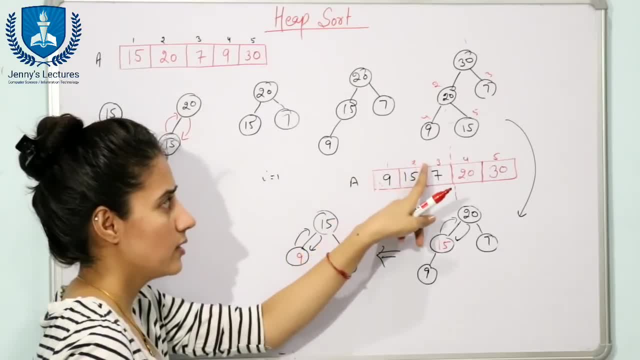 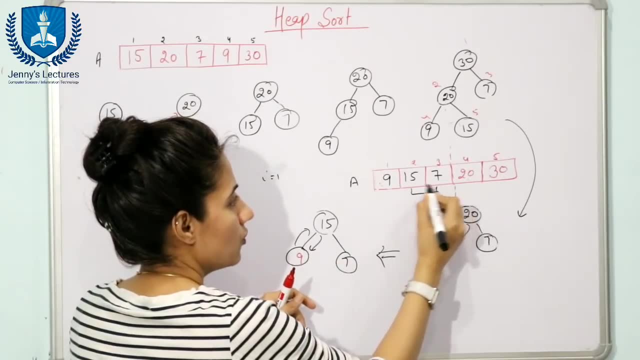 so the left child would be 2 into i, that is at second index. right child would be 2 into i plus 1 that is at third index. 15 and 7 are two children of this. 9, which one is greater? 15- 15 is compared. 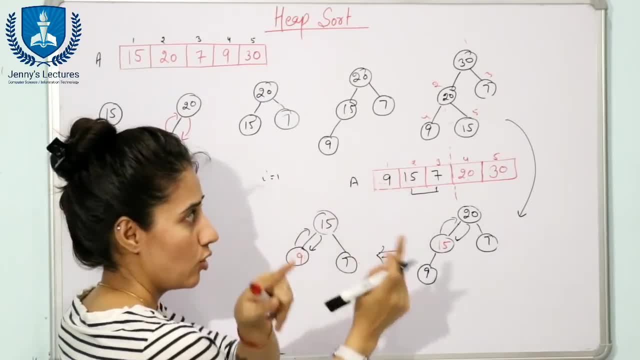 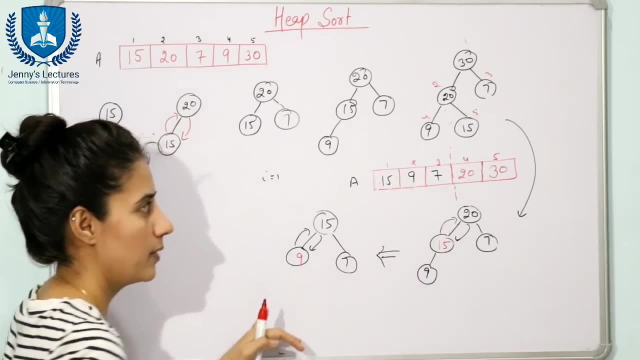 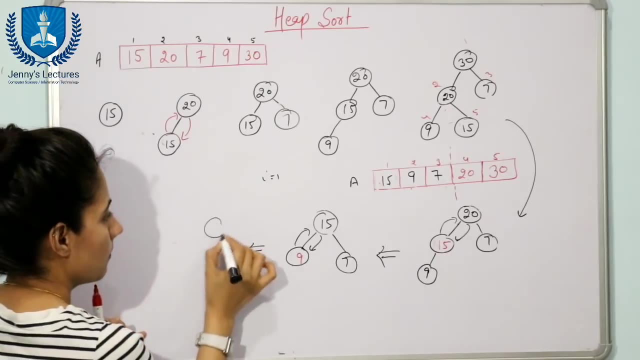 with this, 9 and 9 is parent, which is less than its child. that is not possible, so we are going to shift. so 15 would go here and 9 would go here now. this is the updated array. this is makes heap now fine. next element would be deleted, that is 15. right, so 15 would be deleted now instead of. 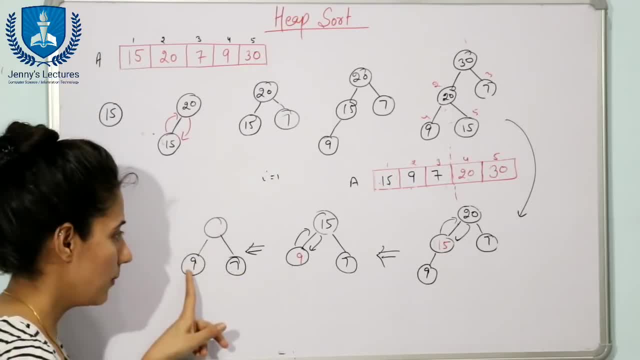 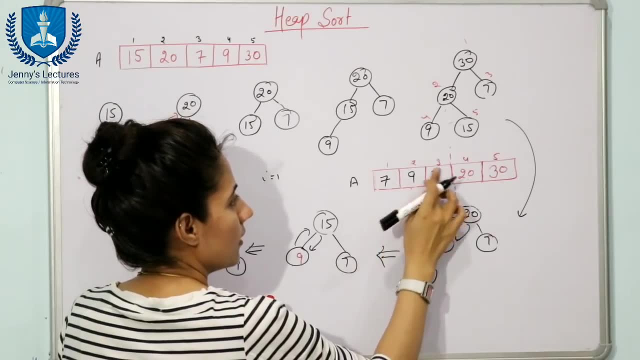 at the place of this 15. which element is to be there? the last element, last element in this tree, 7, or you can say the last element. this array is 7, so 7 would go here. the next element would be 15. right, so 15 would go here and 9 would go here, and so 15 would go here. 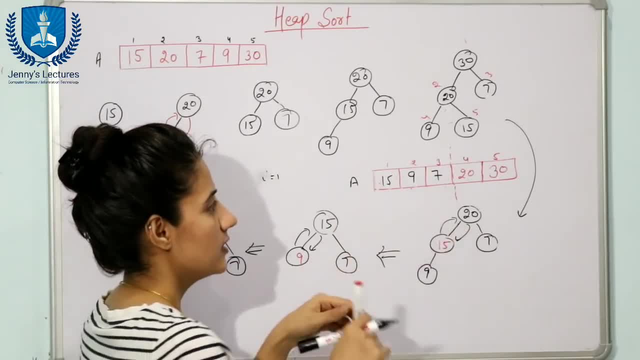 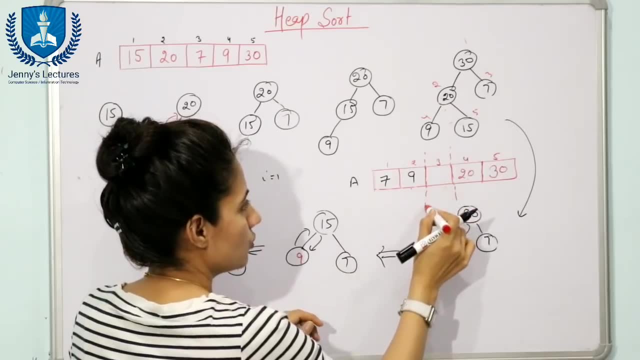 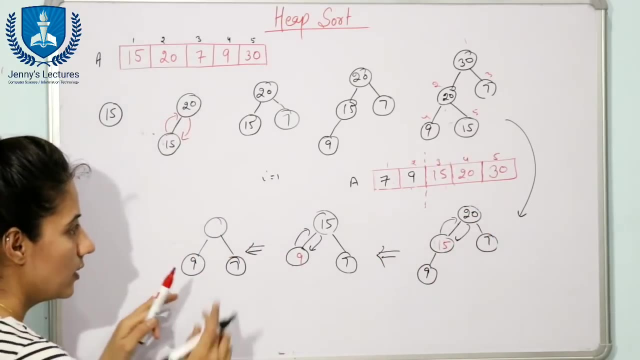 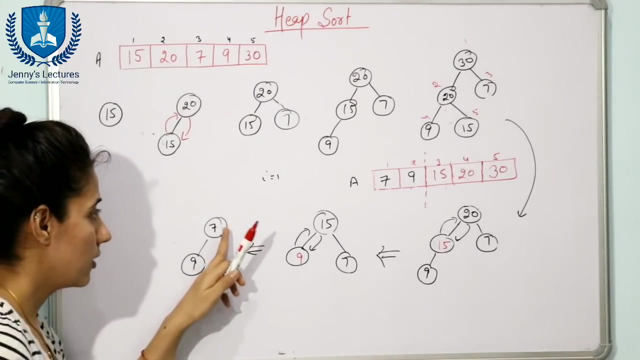 element in this tree is 7, or you can say the last element. this array is 7, so 7 would go here. and now the array size has been reduced and we shift 15 at this place. right, so now 7 would go here. now. we have only two element in this heap. now again check, find out the. 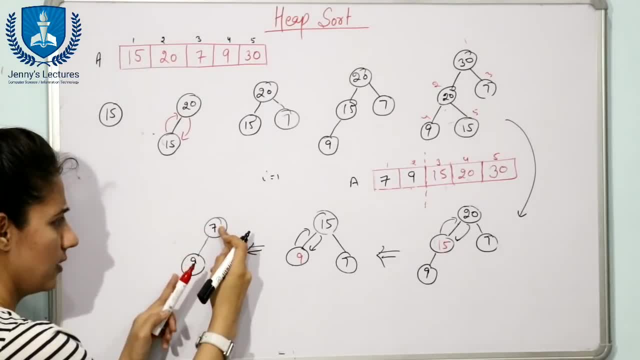 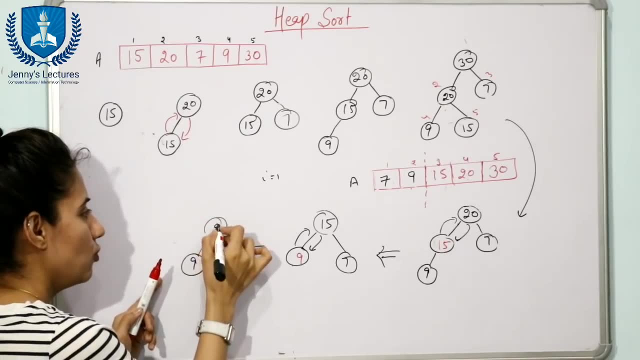 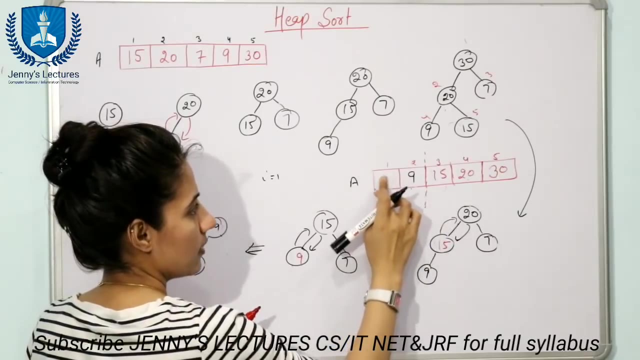 parent. the child of the 7 child is 9 and 9 is greater than 7. that is not possible, so we are going to do swapping. So would go up and 7 would go down, right here. also, after swapping, what is the array? 9 would go here. 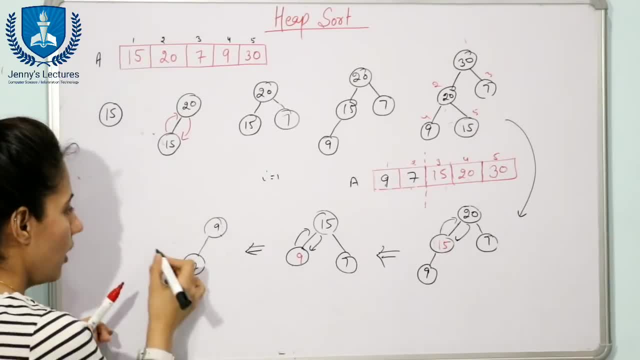 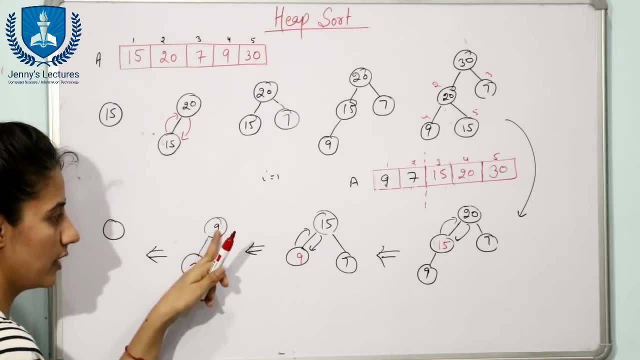 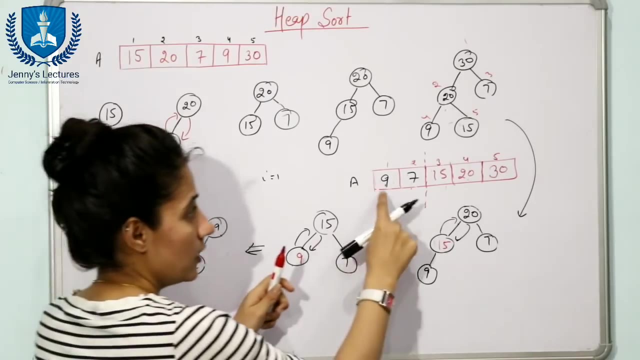 and 7 would go here. okay, now, next is 9 would be deleted. now, after deletion of this 9, which element is to be shifted? here? only one element is left, 7. so after deletion of this 9, we shift 7 at root node. same in array. how you will update. we will delete this 9 and the last element in this array. 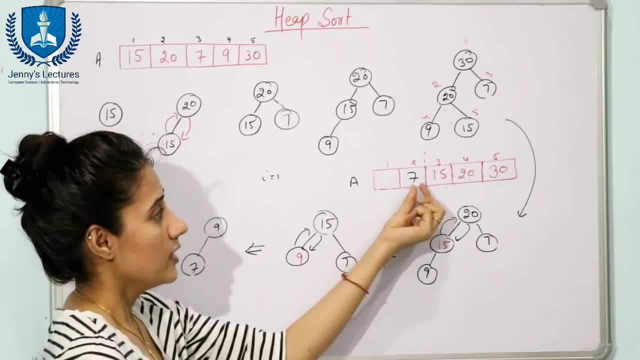 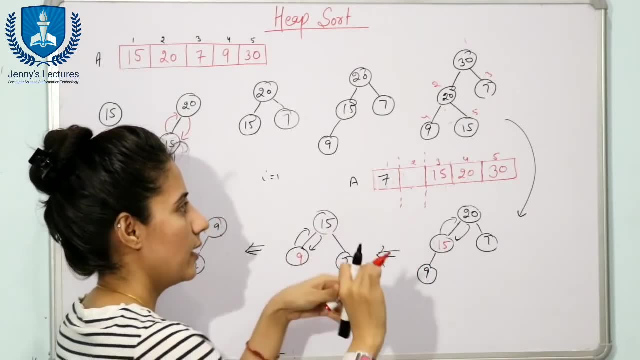 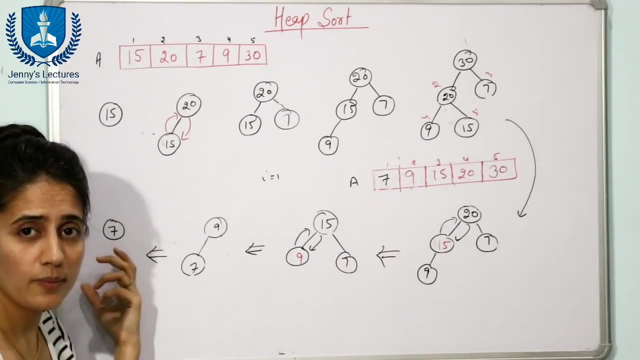 is because array size is now this only okay. last element is 7, so we shift 7 here. now the heap is from having only one element, so we will shift 9 at this place and now we have only one element and that one element is always we can say at max heap. so after deletion of this, 7 we are going to delete. 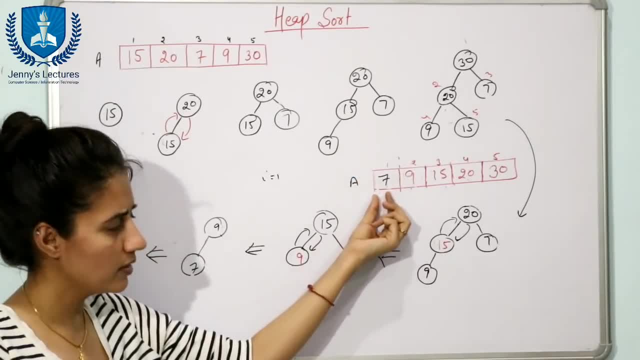 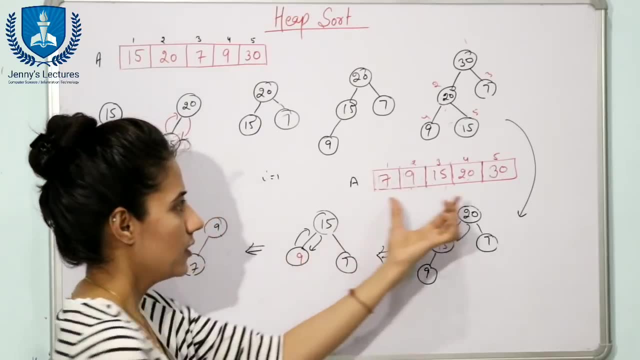 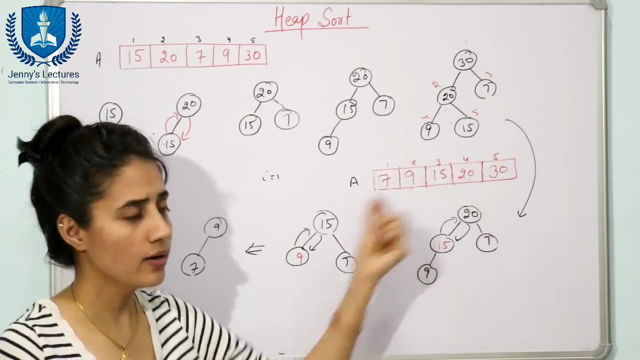 7 and obviously no one element is there. we are going to place 7 here only after deletion. fine, so this is now the array. this is now the array after deleting all the element one by one. so see, you can say that this is sorted now: 7, 9, 15, 20 and 30. so this is how you are going to do sorting: two steps first. 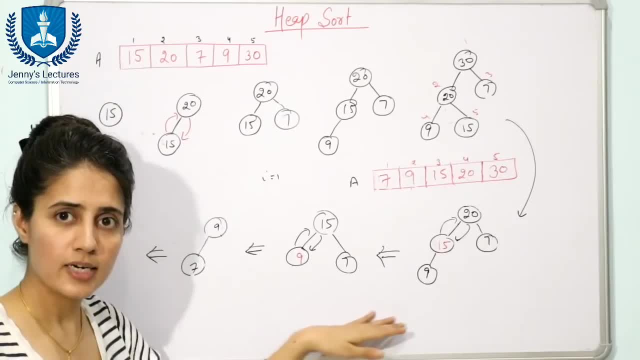 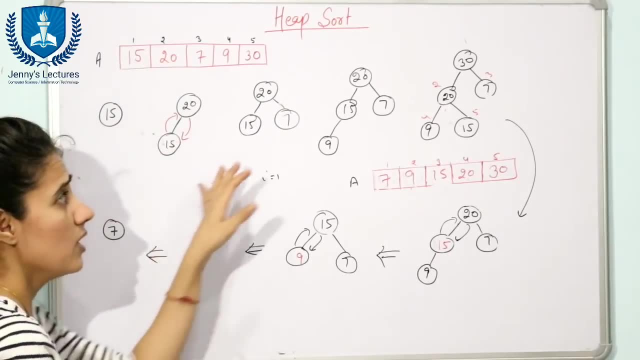 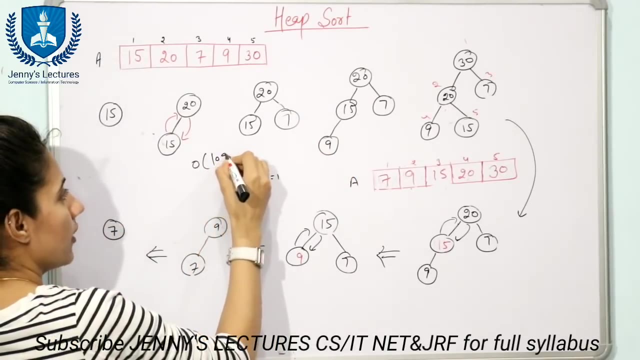 building of a max heap. next you are going to delete data one by one from the max heap and after deletion of all the elements you will get the array sorted now- see the time complexity i have already discussed to insert an element, the time taken would be order of log n. 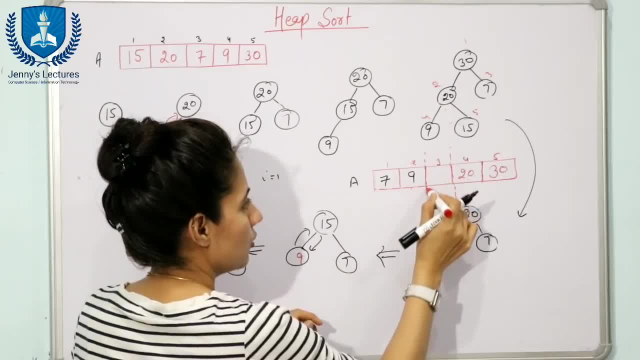 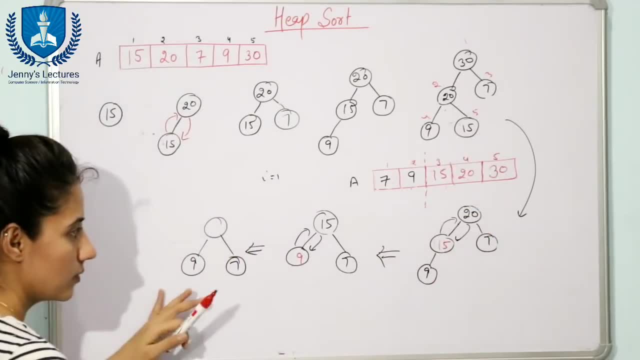 and now the array size has been reduced and we shift 15 at this piece. right, so now 7 would go here. now we have only two element in this heap. now again check, find out the parent. the child of the seven child is nine and nine is greater. 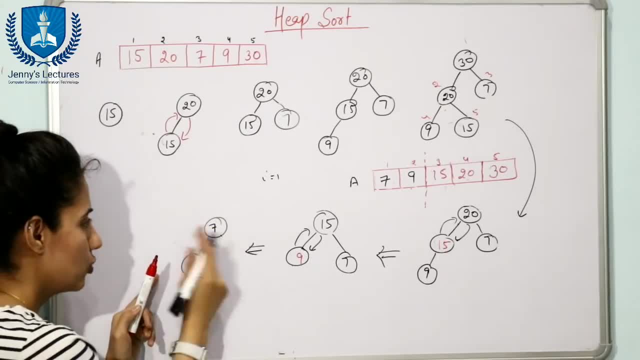 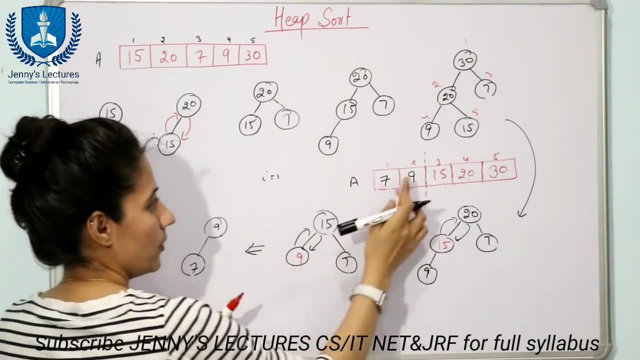 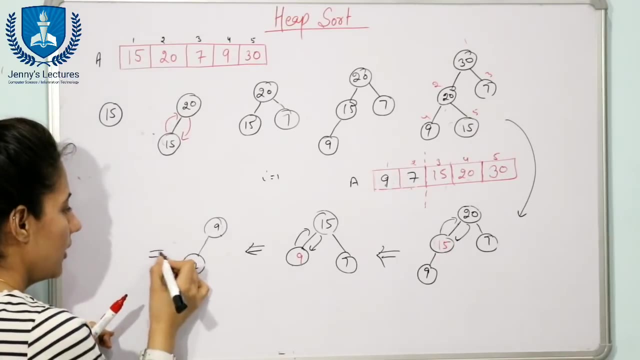 than seven. that is not possible, so we are going to do swapping. so nine would go up and seven would go down. right here also. after swapping, what is the array? nine would go here and seven would go here. okay, now. next is nine would be deleted. now, after deletion of this nine, which element is to be shifted? here only? 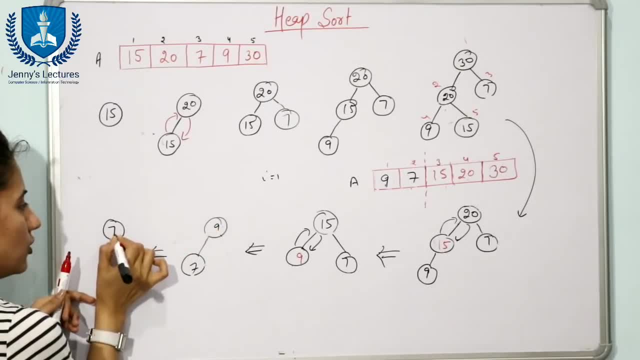 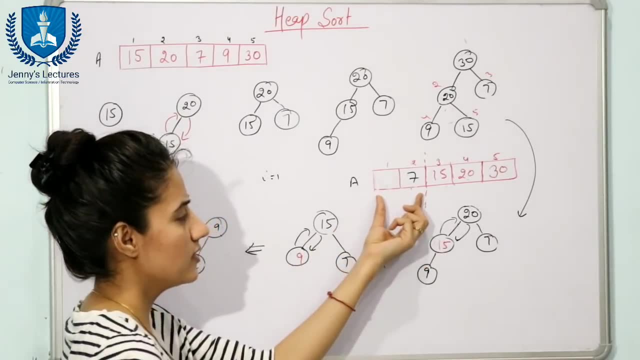 one element is left, seven. so after deletion of this nine, we shift seven at root mode, same in array. how you will update. we will delete this nine and the last element in this array is because the array size is now this only. okay, last element is 7, so we shift 7 here. 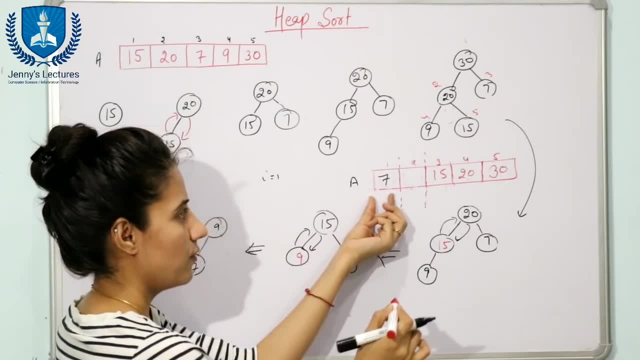 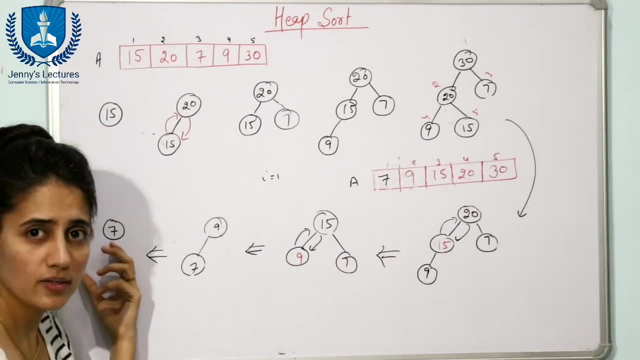 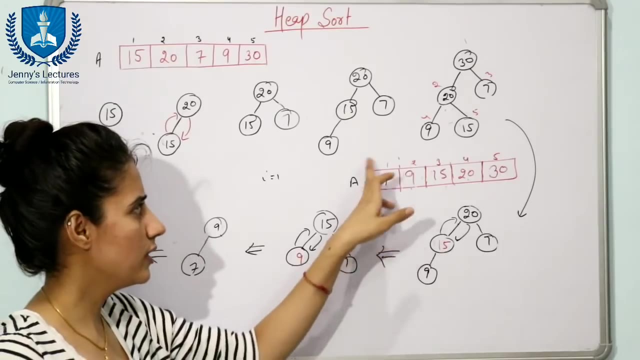 now the heap is from having only one element. so we will shift 9 at this place and now we have only one element and that one element is always, you can say, at max heap. so after deletion of this 7, we are going to delete 7 and obviously no one element is there. we are going to place 7. 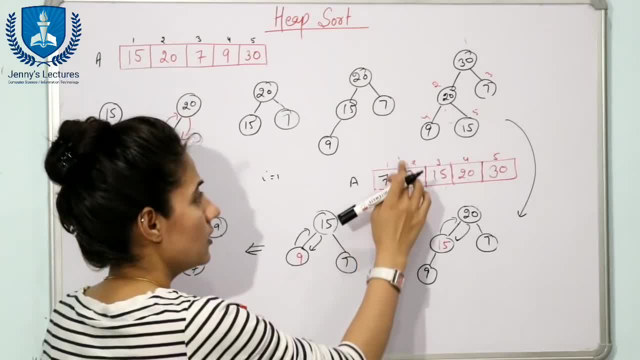 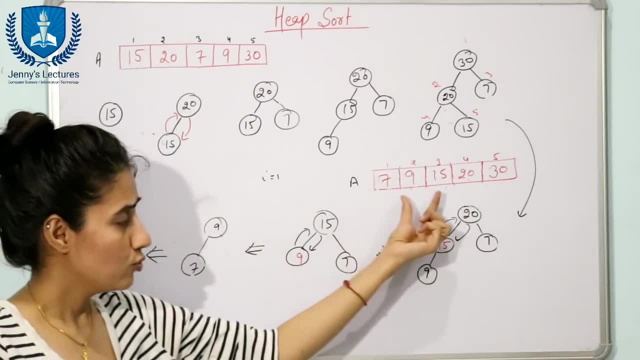 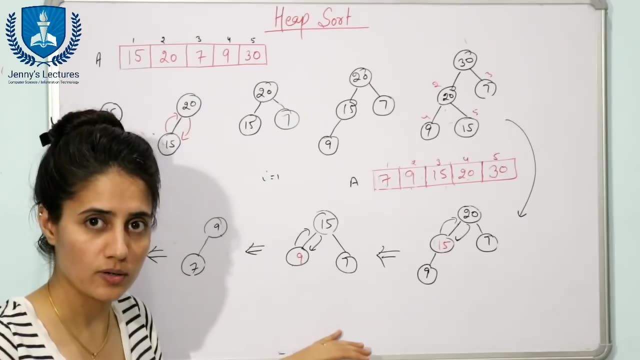 here only after deletion. fine, so this is now the array. this is now the array after deleting all the element one by one. so see, you can say that this is sorted now: 7, 9, 15, 20 and 30. so this is how you are going to do sorting two steps: first, building of a max heap. next, you are going to 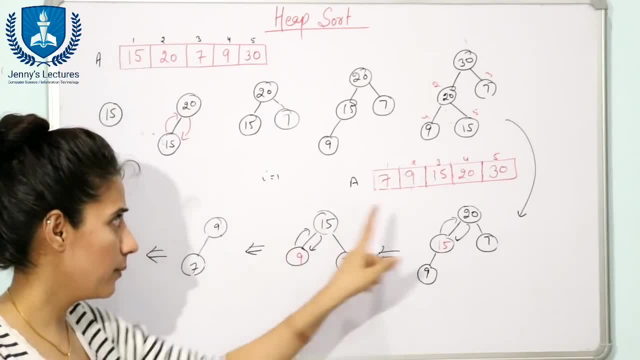 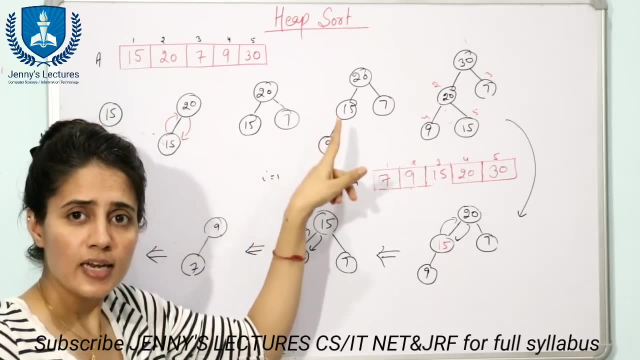 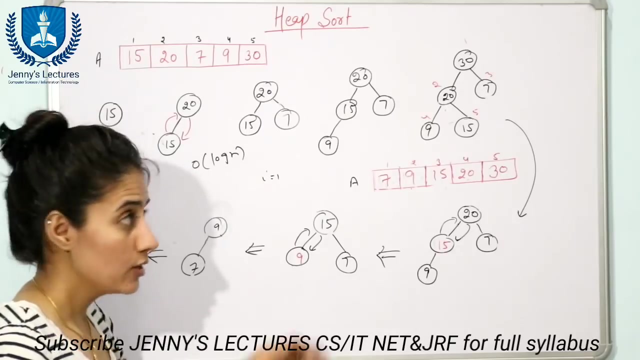 delete data one by one from the max heap and after deletion of all the elements, you will get the array sorted. now, see the time complexity i have already discussed. to insert an element, the time taken would be order of log n. fine, because to insert, we are going to insert an element at the last only, and maximum. we are going to that compare. 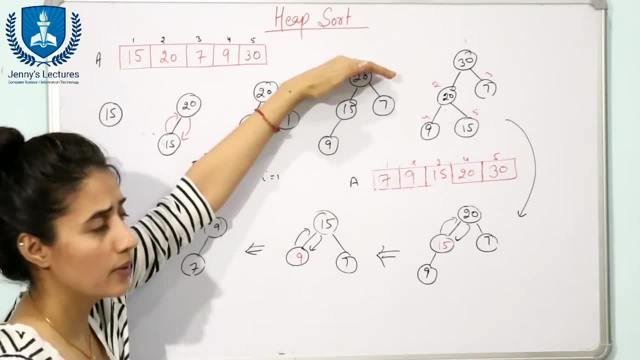 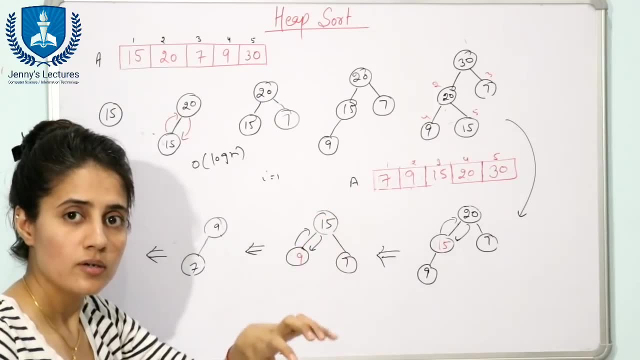 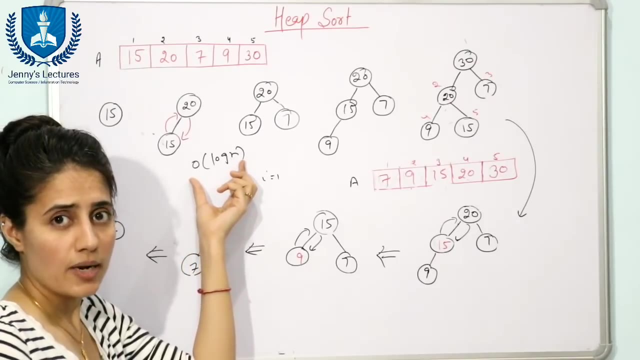 that element, with upper element, with its parent, then with its parent, according to the height we are going to compare. and height of a complete binary tree is log n. so to insert any data in the that complete binary, the worst case, in the worst case, the time taken is order of log n and we are, we are going to insert: 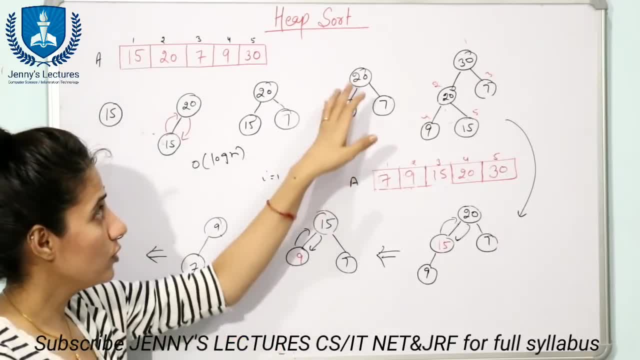 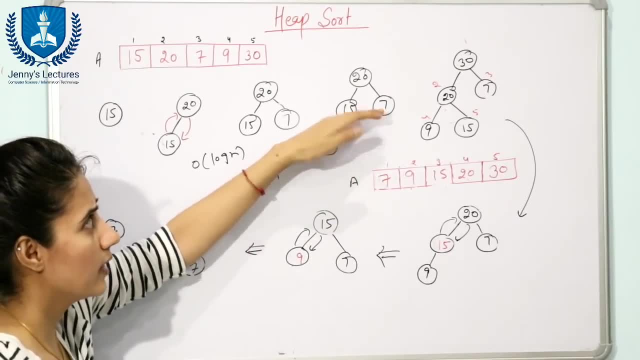 fine, because to insert, we are going to insert, an element at the last only and maximum. we are going to that. compare that element with upper element, with its parent, then with its parent according to the height we are going to compare, and height of a complete binary tree is: 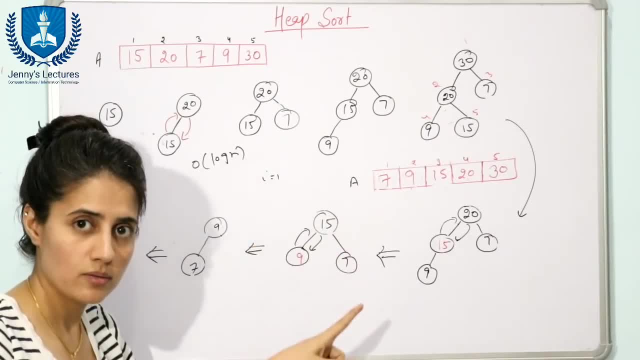 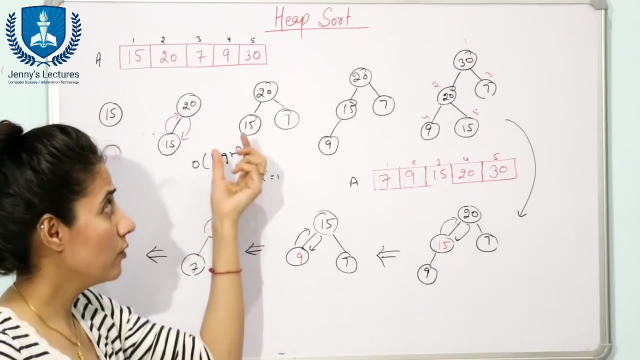 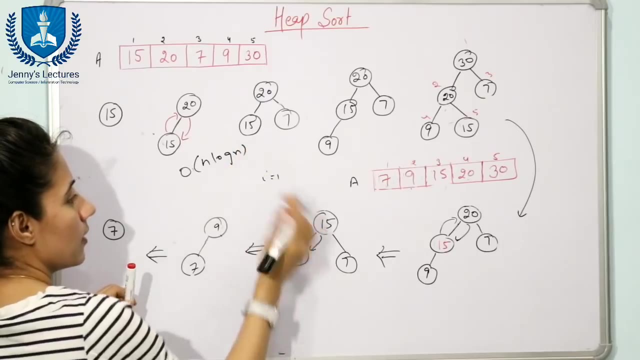 log n so to insert any data in the that complete binary tree. the worst case in the worst case, the time taken is order of log n and we are, we are going to insert n element. so for insertion the time complexity would be order of n log n and for deletion also, deletion also take. 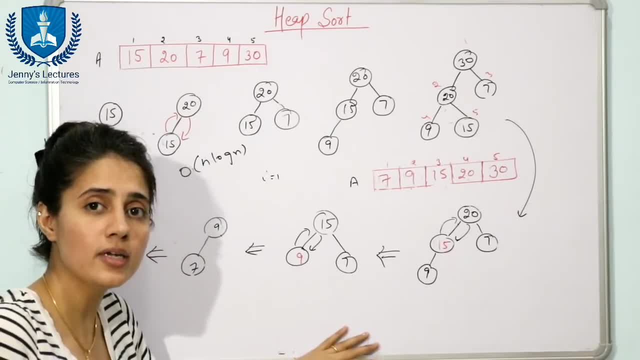 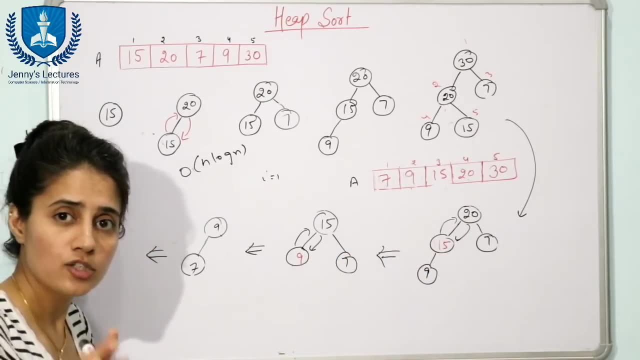 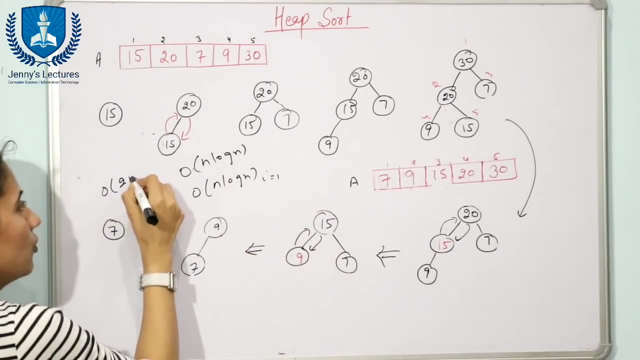 one element to be deleted and that element take how many time? order of log n. and you are going to delete n elements, all the elements are going to delete. so for deletion also it is going to take order of n log n. so total time complexity would be order of 2 n log n and by default 2. 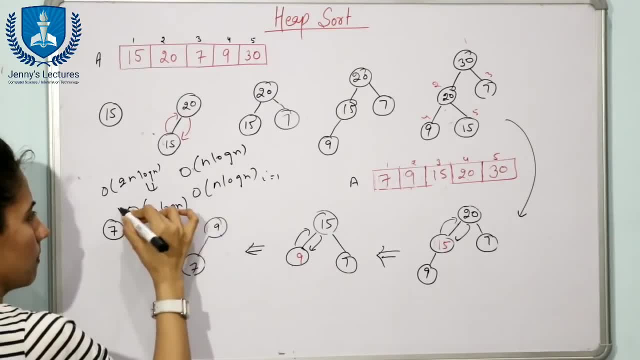 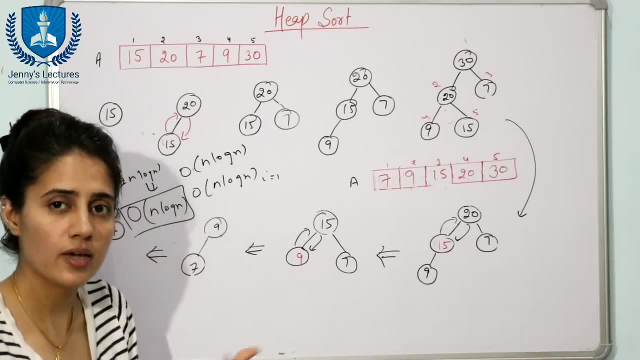 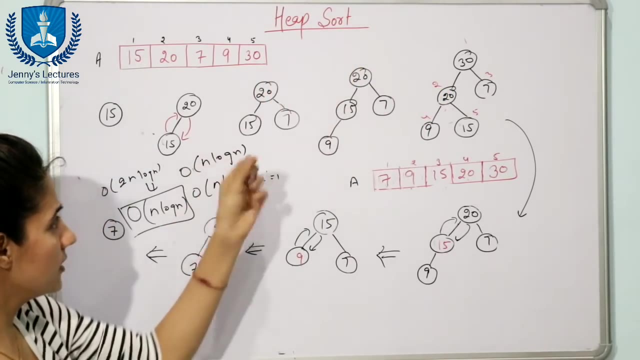 is constant, so you will write order of n log n. so time complexity of this heap sort is order of n log n, both in worst and best case and in average case also. fine, now see this building of this max heap here is taking order of n log n time. can we apply some another method in that case? the time? 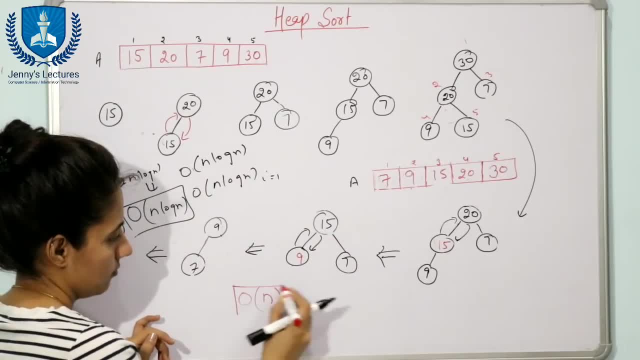 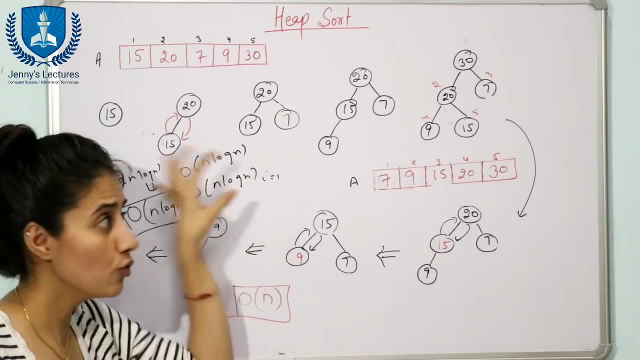 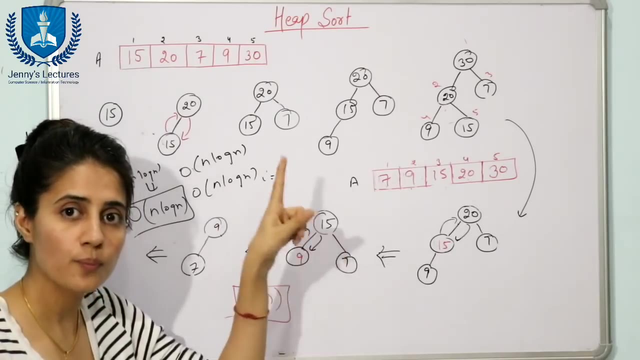 complexity is only order of n, because if you apply this method then time complexity would be order of n log n. it is just for building the max heap, creating the max heap. but now we are going to discuss another method in which that building of max heap will only take how much time. order of. 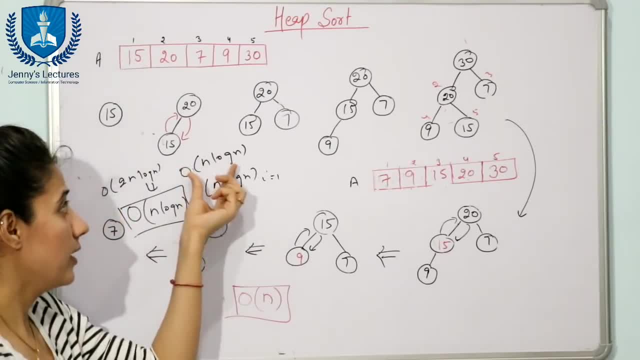 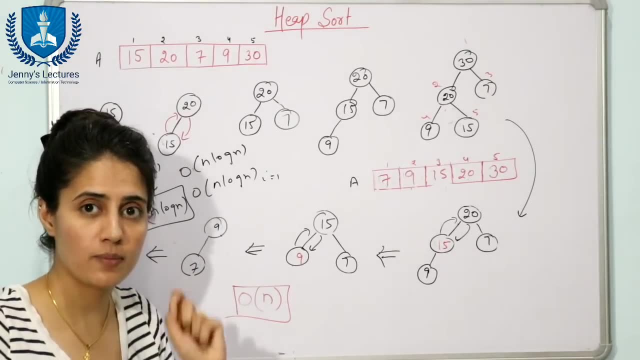 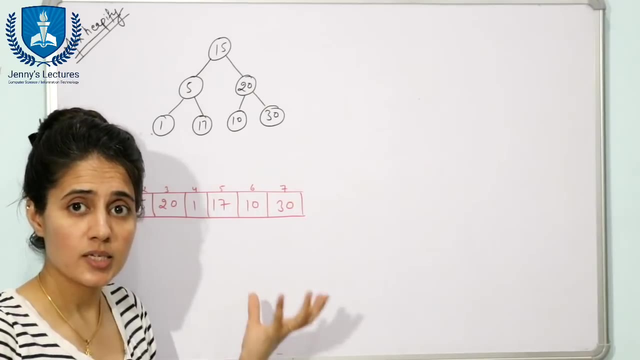 n only, and obviously order of n is better than n log n right, and that method is known as heapify method. now we are going to discuss what is heapify method and how this method, heapify method, can be used in heap sort. so now i will discuss heapify method, or i i can say mix heapify method, because 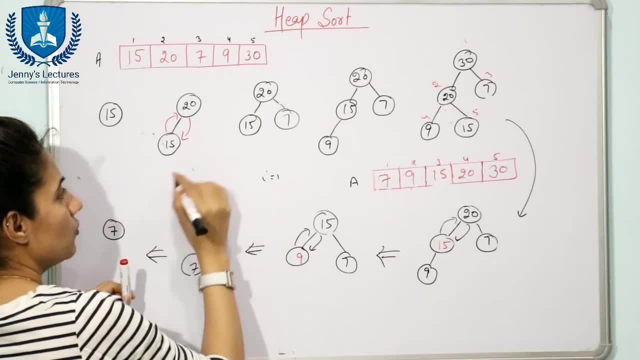 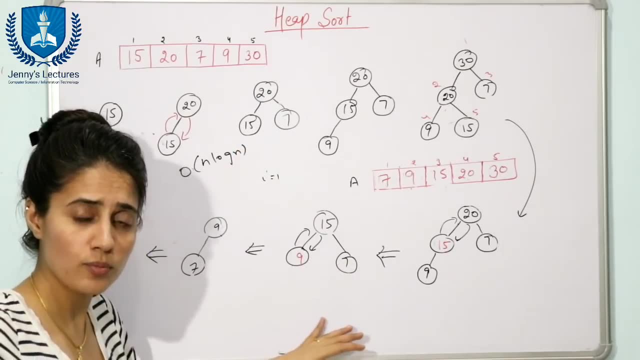 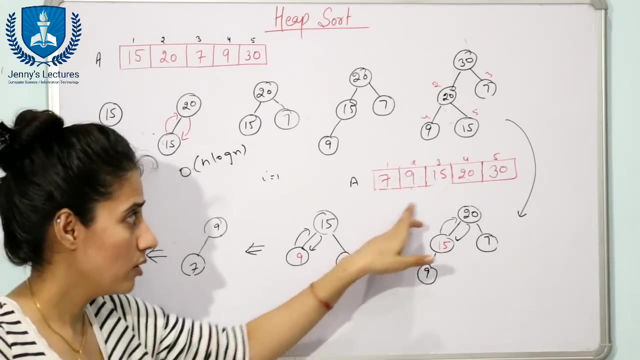 n element. so for insertion the time complexity would be: order of n, log n and for deletion also. deletion also take one element to be deleted and that element take how many time. order of log n. and you are going to delete n elements, all the elements are going to delete. so for deletion also. 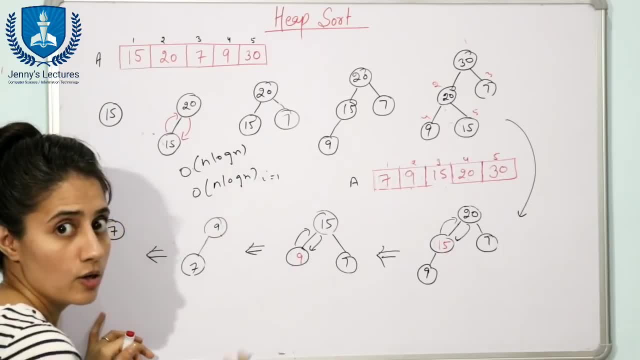 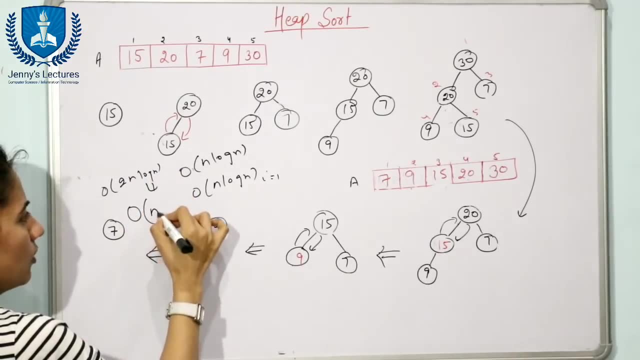 it is going to take order of n log n, so total time complexity would be order of 2n log n and by default 2 is constant. so you will write order of n log n, so time complexity of this heap sort is order of n log. 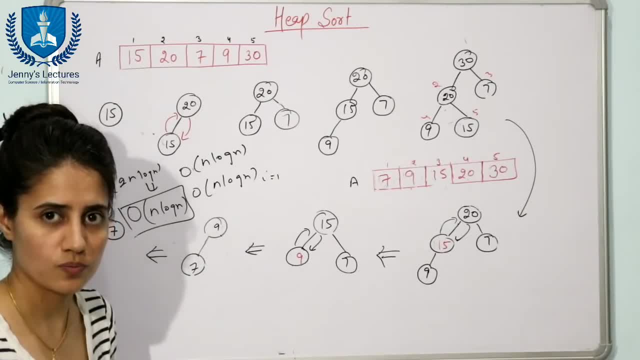 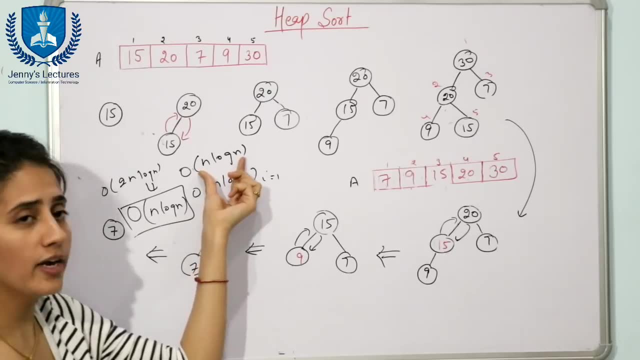 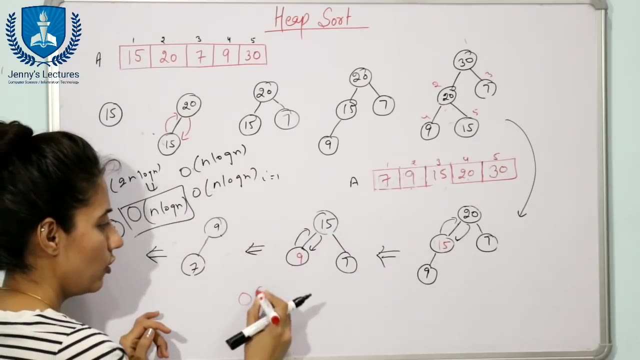 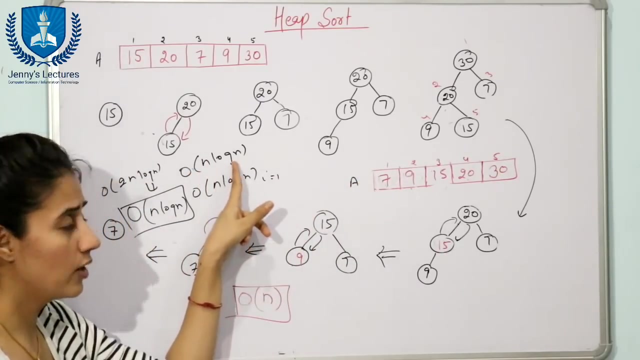 n, both in worst and best case and in average case also. fine, now see this: building of this max heap here is taking order of n log n time. can we apply some another method? in that case the time complexity is only order of n, because if you apply this method, then time complexity would be order of n log n. 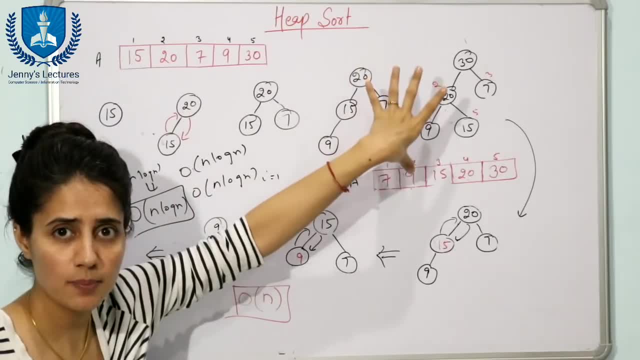 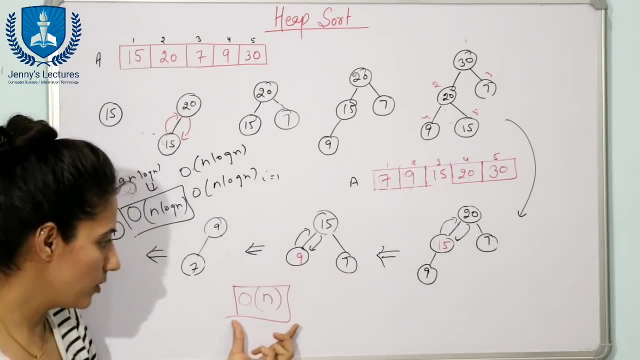 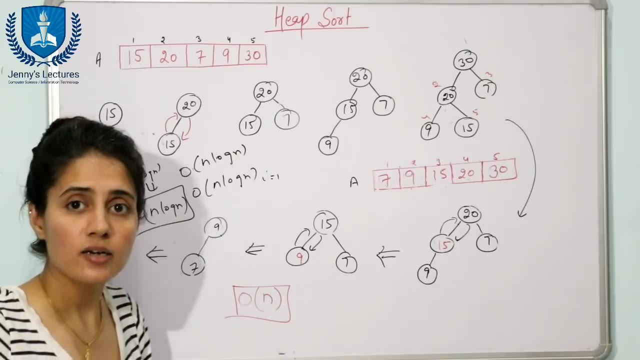 it is just for building the max heap, creating the max heap. but now we are going to discuss another method in which that building of max heap will only take how much time. order of n only, and obviously order of n is better than n. log n right and that. 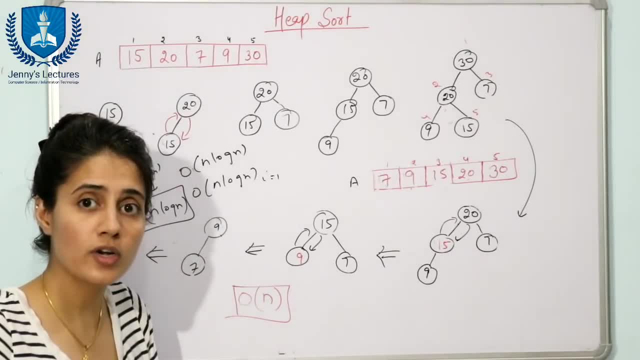 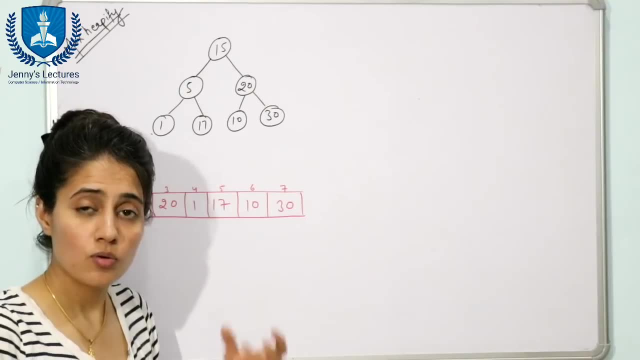 method is known as heapify method. now we are going to discuss what is heapify method and how this method, heapify method, can be used in heap sort. so now i will discuss heapify method, or i i can say max heapify method, because i am taking into consideration the max heap. how heapify method? 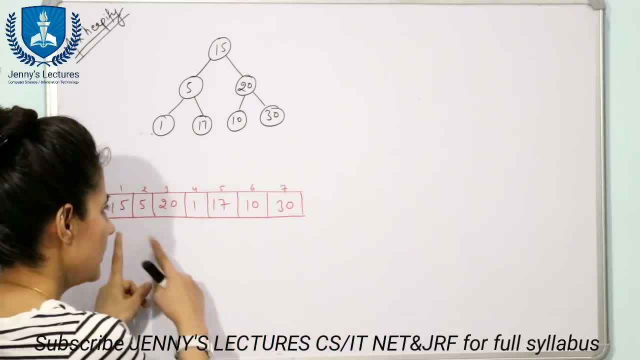 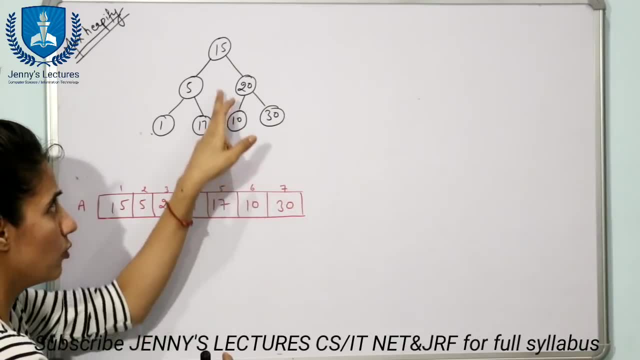 is used to build max heap. fine, let us take this array we have now. we have just represented this in the form of this complete binary tree. this is complete binary tree. according to this, this is the array, but this is not a max heap. you are supposed to take this array and you are supposed to take 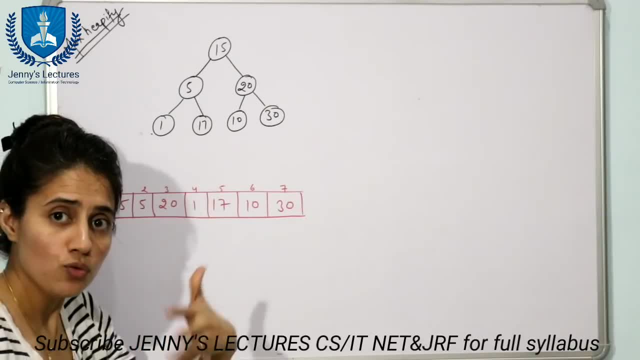 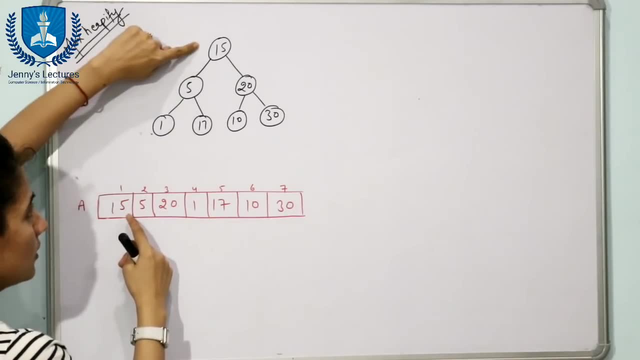 this array and you are supposed to make it max heap using heapify method. if you, if you use the method, the first method- we have discussed, that insertion method- then then what we will do: first 15 would be inserted, then 5 would be inserted and then, checking with this parent, then 20 would be. 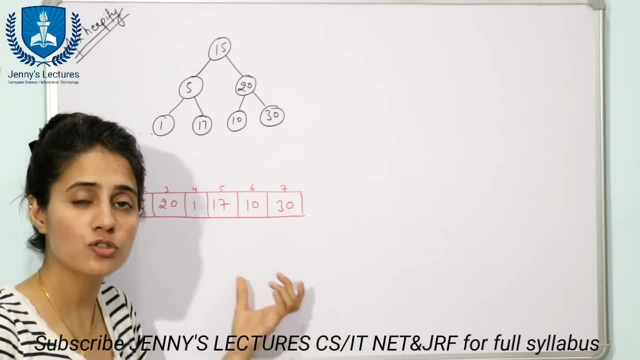 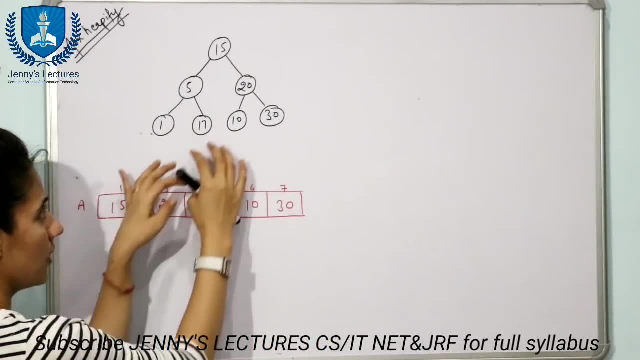 i am taking into consideration the mix heap, how heapify method is used to build max heap. fine, let us take this array we have now. we have just represented this in the form of this complete binary tree. this array will be useless. we have kept double space and this is only glowing over there. we just want to have extra space because, similarly, 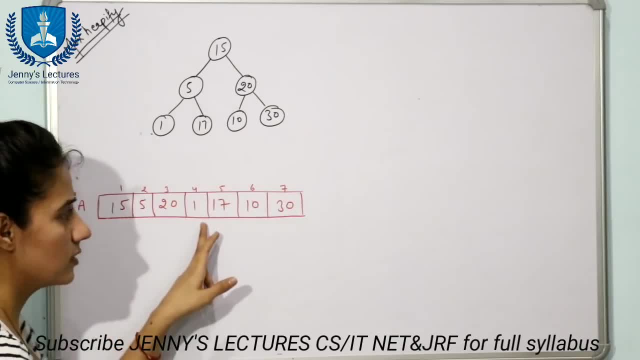 now we are going to create another heap with this method, so now we will start from back. complete binary tree. This is complete binary tree. According to this, this is the array, but this is not a mix heap. You are supposed to make it mix heap using heapify method. 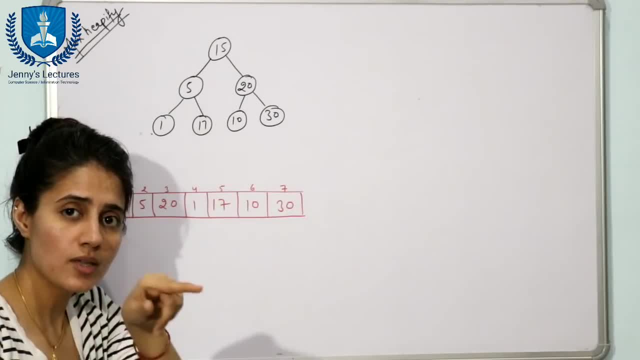 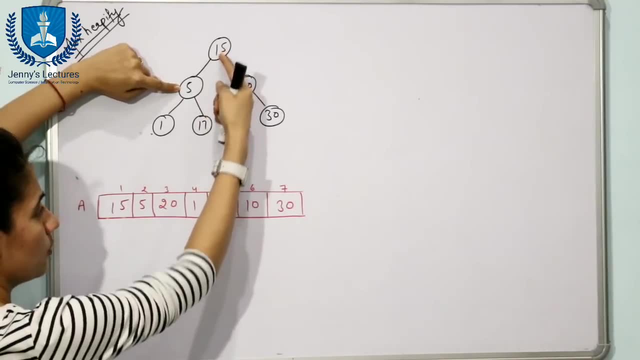 If you, if you use the method, the first method we have discussed, that insertion method, then then what we will do: first 15 would be inserted, Then five would be inserted, And then, checking with this parent, then 20 would be inserted, and checking with its parent, Then one would. 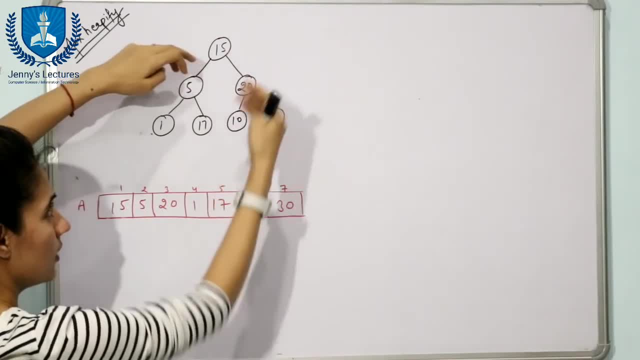 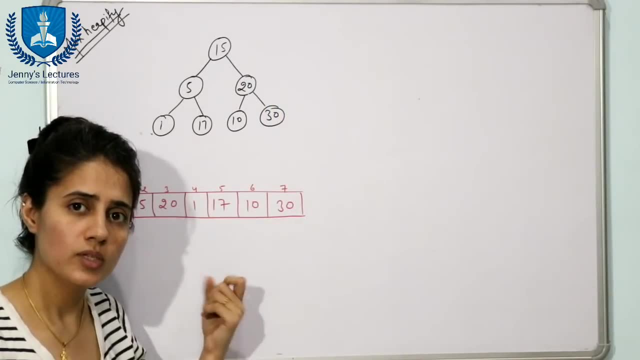 be inserted and checking with its parent and swapping, checking with parent and swapping in like this: then 17, then this 10 and then this 30. but here now we are not going to do this thing, we are going to use hippify method. now, what is that method? see first of all, see in the case of 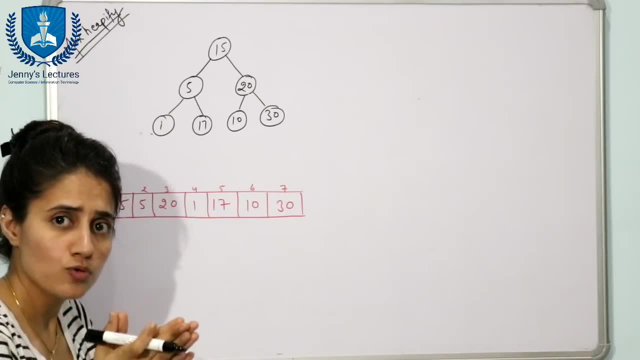 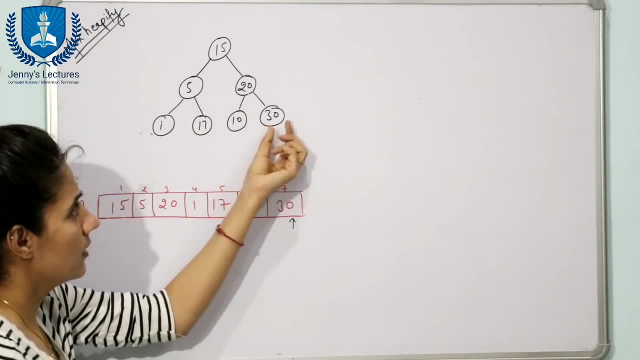 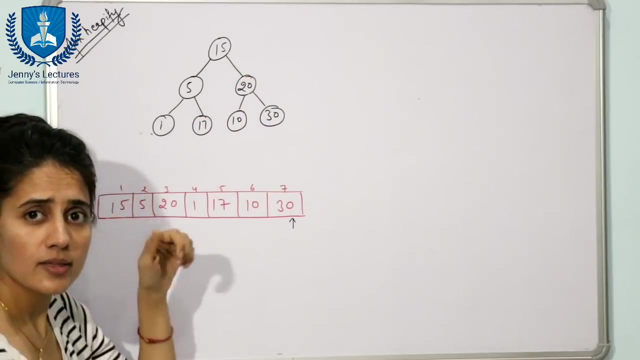 insertion. we have started from here. now let us suppose we have. we have changed our approach and we have started from here. first is 30 here. see this 30 only only check this 30. 30 is only one element. so if only one element is there, only one element is there, and that element is itself a. 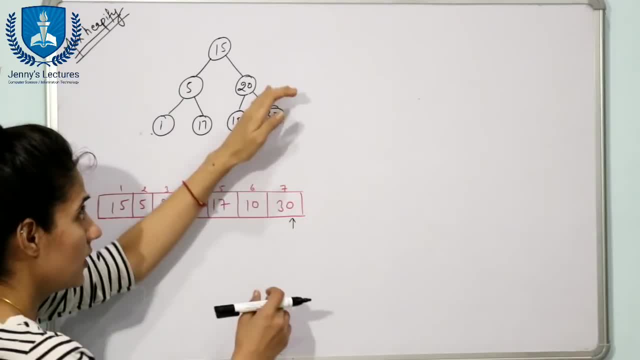 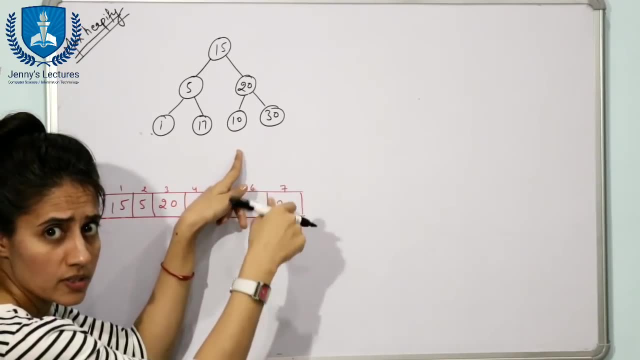 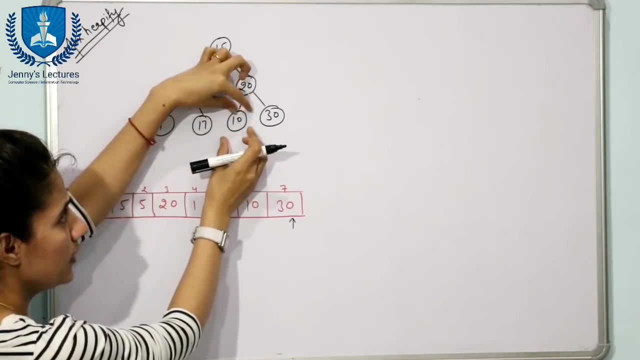 either max heap or min heap. here we are discussing max heap, so 30 is a max heap. now check for 10. 10 is 10 having any child node. we are going to check the descendants, we are not going to check the parent. here we are. we are changing our approach. fine, 10 check only 10. 10 is also. 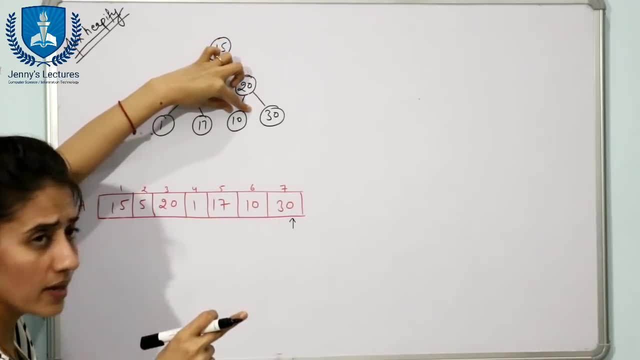 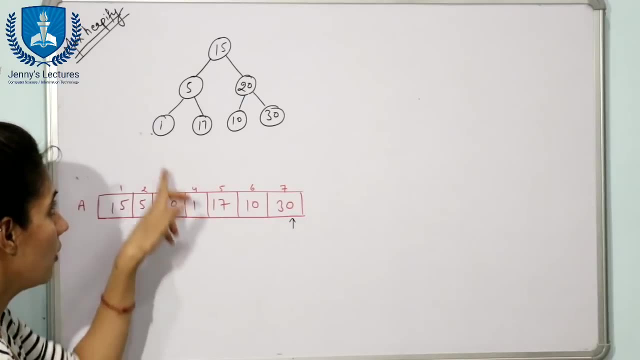 you can say: not having any child element, so this is itself itself a max heap. then 70, 17 is also one element. this is itself a max heap. then we have one. one is also one element: no child node is there, so it is itself a max heap. fine, now we will check for 20. now we have. 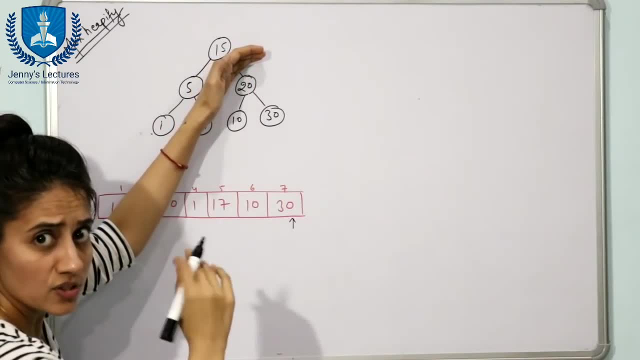 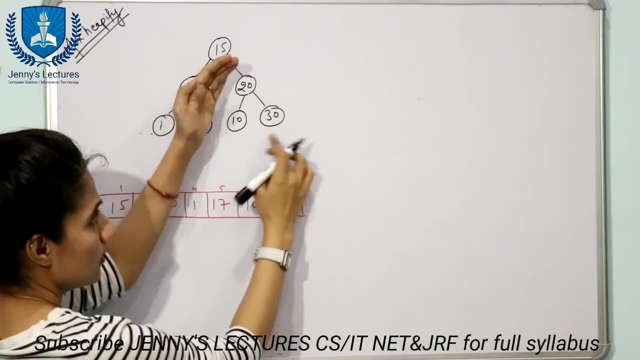 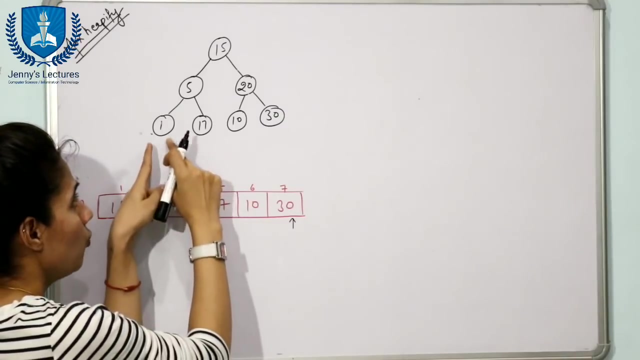 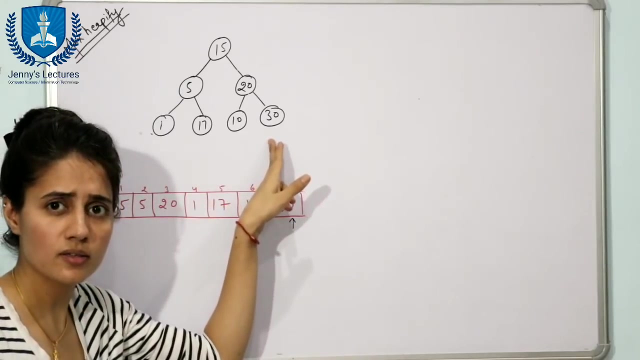 this one 20. 20 is having left child and right child also. now our main motto is to do: to make this tree, this tree, 20, 10 and 30 as max heap. fine, then we will consider 5 and then finally 15. ok, now check 1, 17, 10 and 30. these are leaf nodes. so we can say: if leaf nodes are, then if leaf nodes. 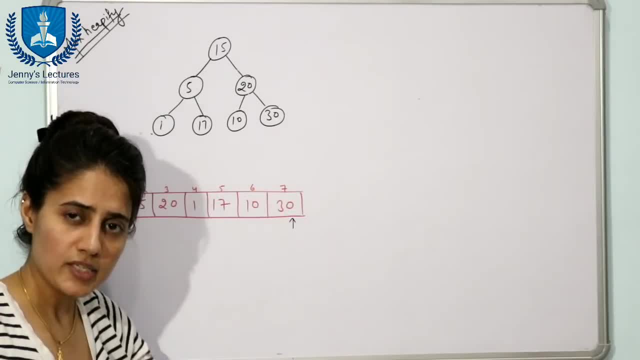 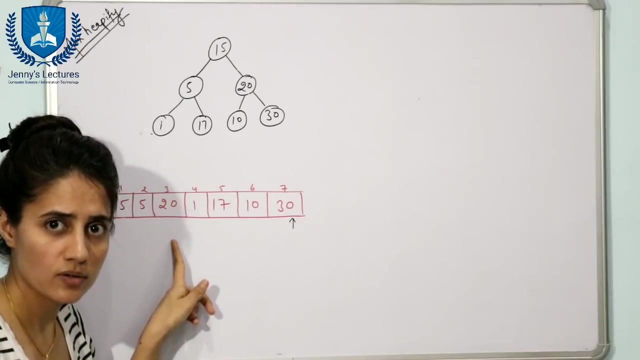 are there, then these nodes are itself max heap. no need to heapify those nodes. you can say something like this: right, so we need to apply heapify method, only your known leaf node right. and we are not going to start from here, we are going to start from right to left. so first of all, we are going. 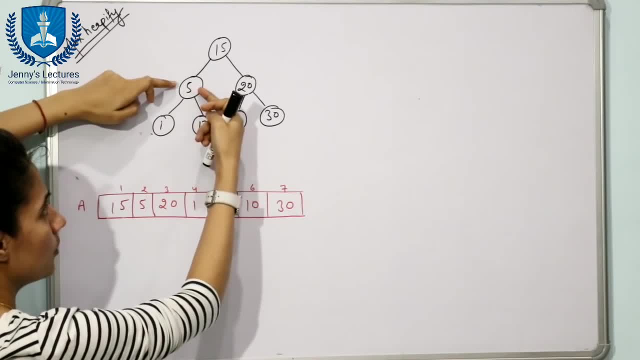 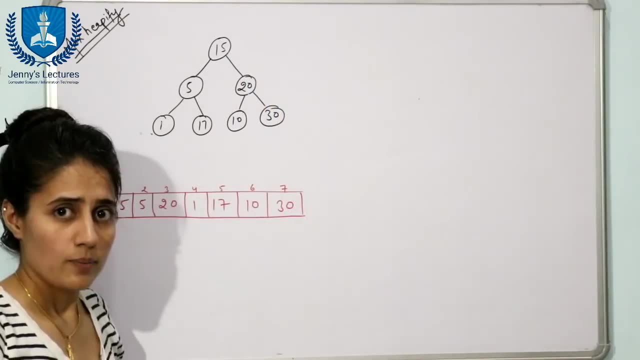 inserted, then checking with its parent, then 1 would be inserted, then checking with its parent and swapping, checking with parent and swapping, and like this: then 17, then this 10 and then this 30. but here now we are not going to do this thing, we are going to use heapify method. now, what is that? 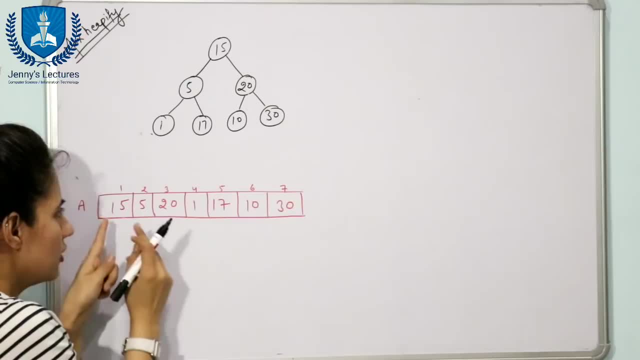 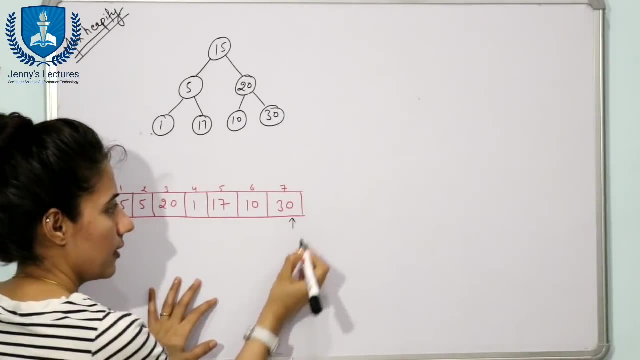 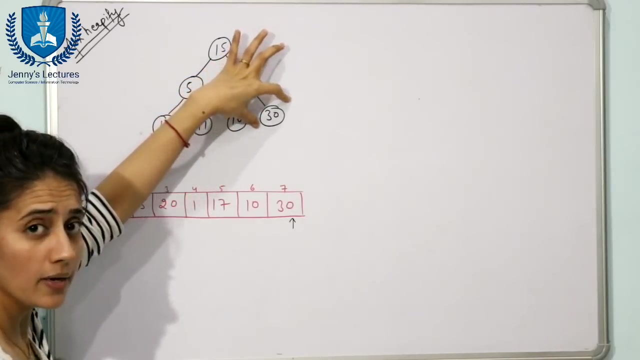 method: see first of all. see, in the case of insertion, we have started from here. now let us suppose we have. we have changed our approach and we have started from here. first is 30 here see this 30 only only check this 30. 30 is only one element. so if only one element is there, only one element is. 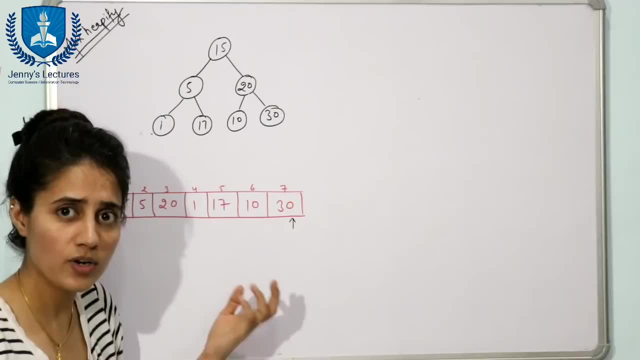 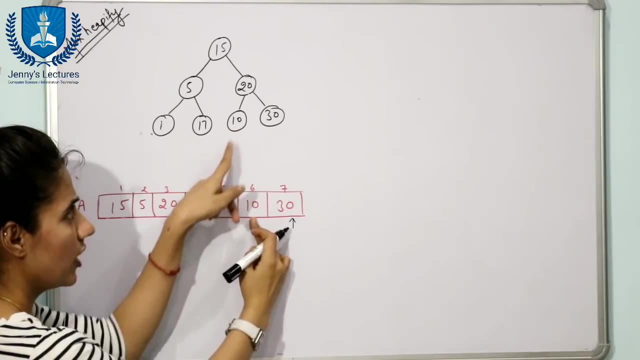 there and that element is itself either max heap or min heap. here we are discussing max heap, so 30 is a max heap. now check for 10. 10 is 10 having any child node. we are going to check the descendants, we are not going to check the. 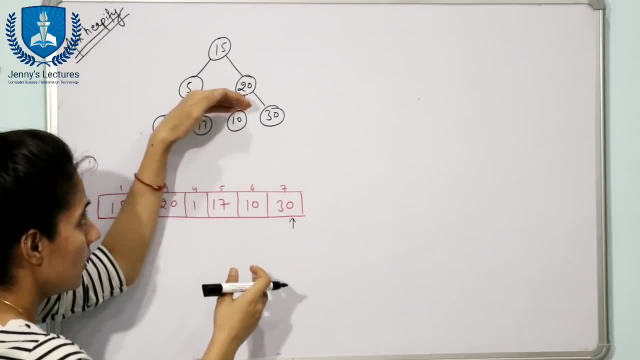 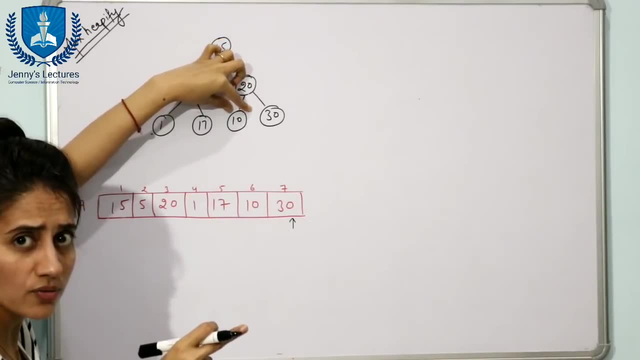 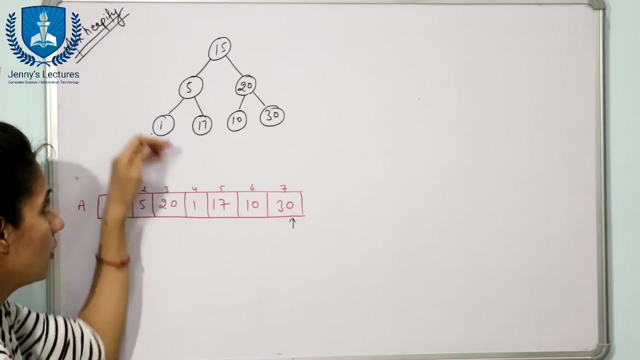 parent. here we are, we are changing our approach. fine, 10 check, only 10. 10 is also, you can say, not having any child element, so this is itself itself for maxi. then 17, 17 is also one element. this is itself a max heap. then we have one. one is also one element. no child node is there, so it is itself a 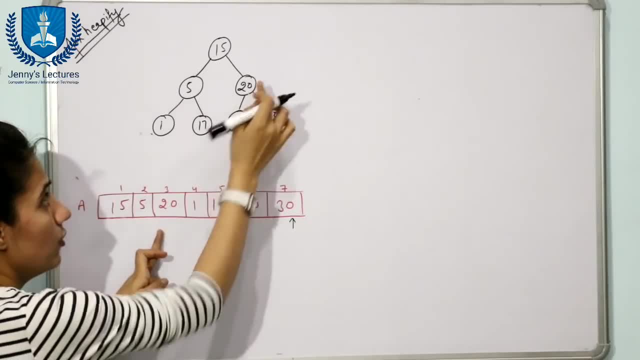 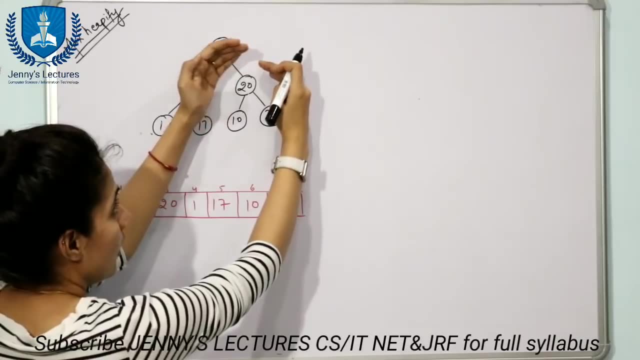 max heap. fine, now we will check for 20.. now we have this one: 20- 20 is having left child and right child also. now our main motto is to do: to make this tree, this tree, 20, 10 and 30 as max heap. 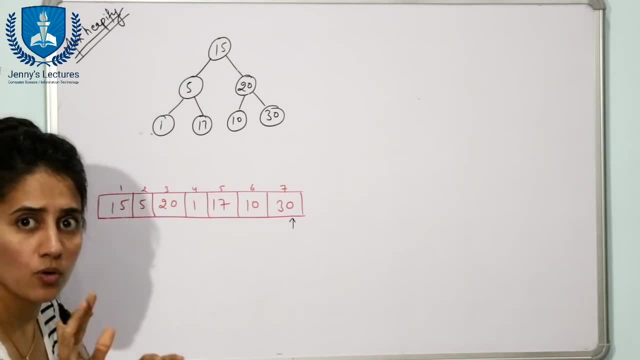 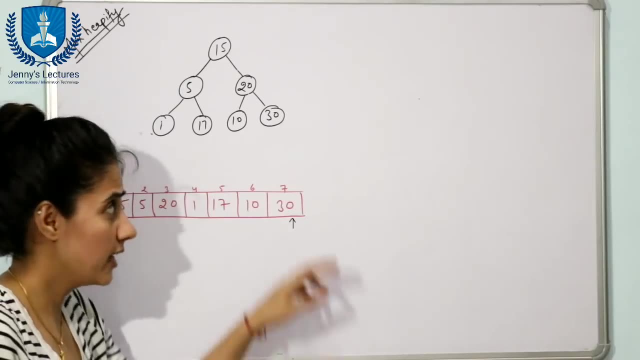 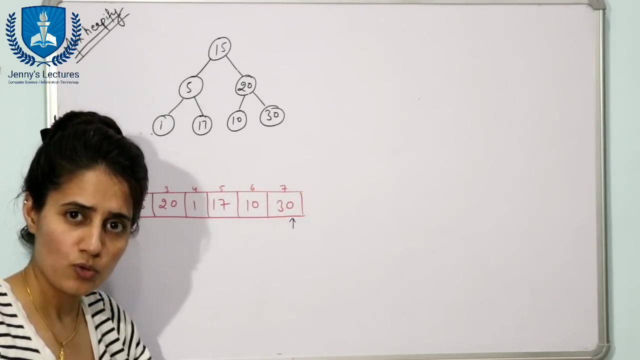 fine, then we will consider 5 and then finally 15.. okay, now check 1, 17, 10 and 30. these are leaf nodes. so we can say, if leaf nodes are, then if leaf nodes are there, then these nodes are going to, are going to grow, or even then it's jigged, or even then they will grow. 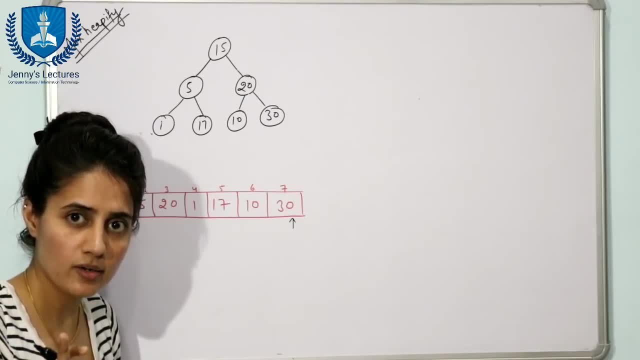 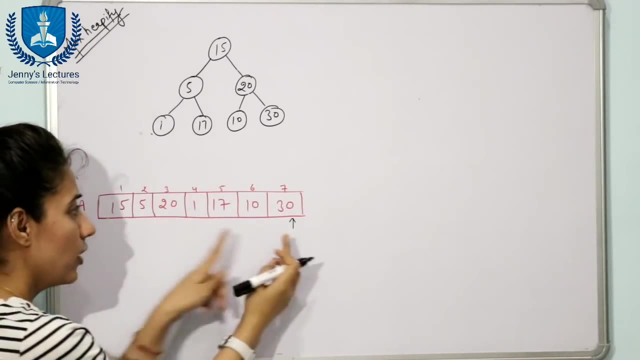 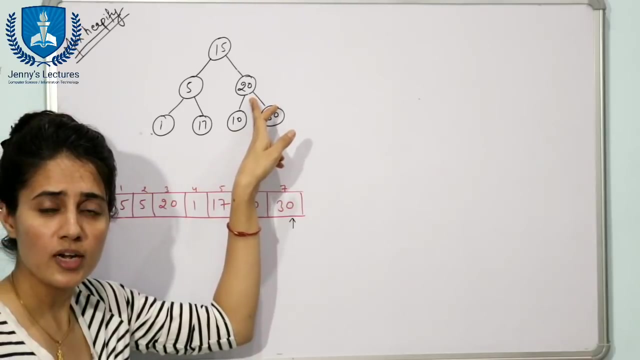 now, when we come to crunchers corners, if you zoom in, if you observe on my profile again, you will see that in the chart that we are going to watch, as we are going to allow here to exercise this graph, we are going to say that mindanja is moving to the left. now we have done. to apply our heapify method to the known leaf element which is at the largest index. see here. index are 1, 2, 3, 4, 5, 6 and 7. now at index 4, 5, 6 and 7, all the nodes are leaf node, so just leave. 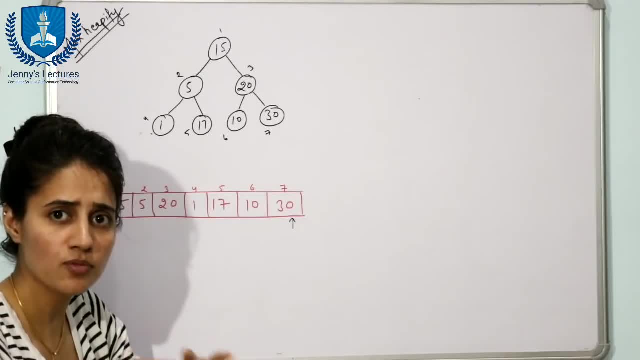 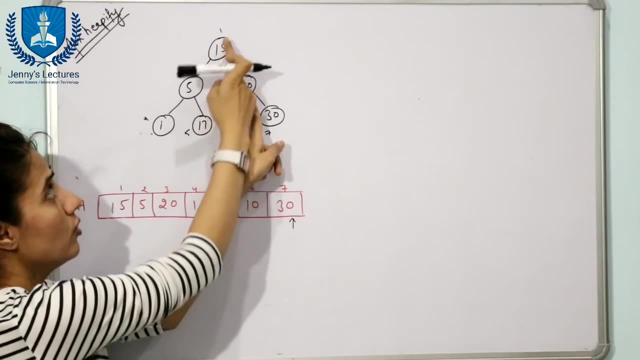 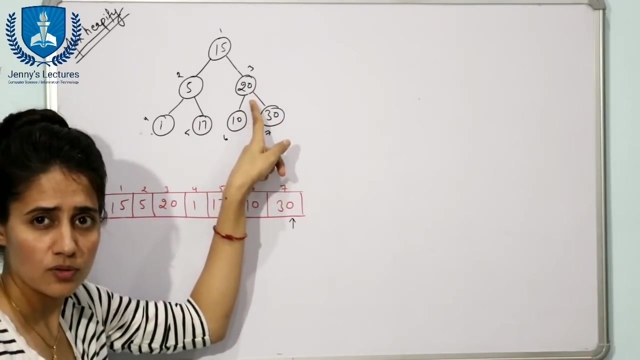 those nodes and we are going to start our loop or we are going to start our heapify method from 20 only and index of 20 is 3. the known leaf node are on the index 1, 2 and 3. so the largest index is 3, which is having the known leaf node. so we are going to start our 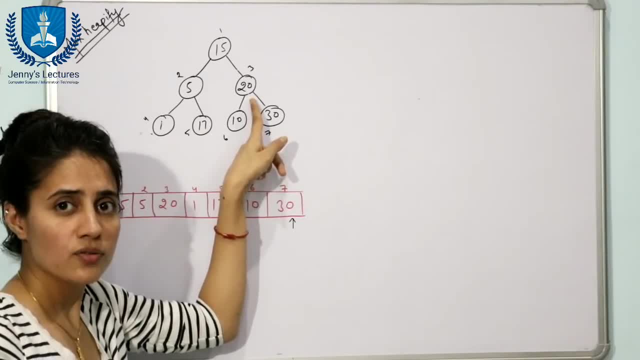 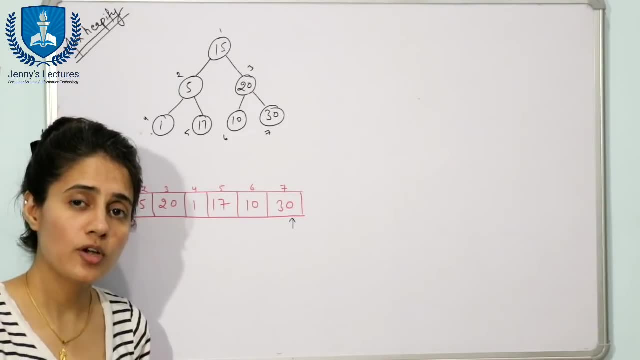 apply our heapify method from here the known leaf element which is at the largest index. fine, now how to find out which, at which index we are having leaf node and from which index known leaf node is going to start, from which the largest index known leaf node is going to start. so in a complete binary tree, the property of complete binary trees, the leaf node would be from n by 2 floor value plus 1 to n. here you can check here: n value is 7, 7 by 2, 7 by 2 is 3.5, floor value is 3, 3 plus 1 is 4. so from from 4 to 7, 4, 5, 6, 7. these are leaf. 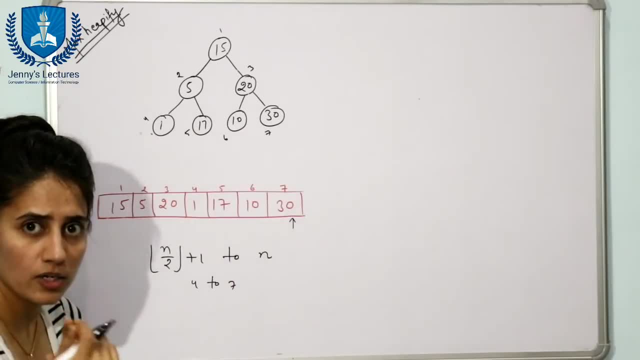 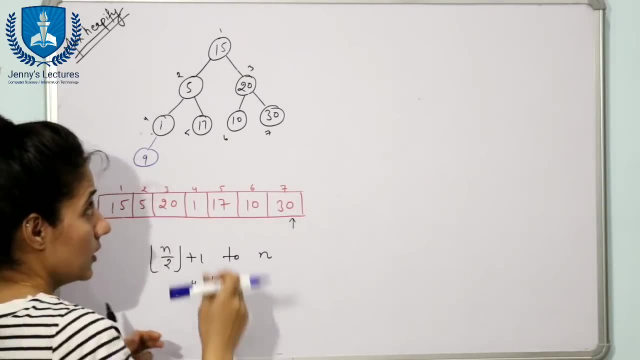 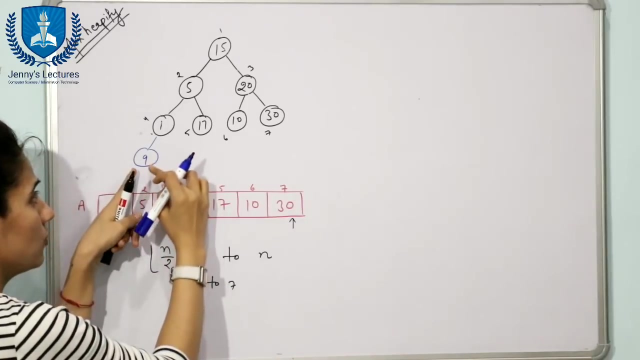 node as you can see in tree 4, 5, 6, 7, these are leaf node. suppose if i add one more element here, see, this tree is not still a maxi. we are going to heapify this to to make it a maxi. so suppose we have inserted 9 here. now leaf node are at the index 7 and here we have 8. suppose here we have. 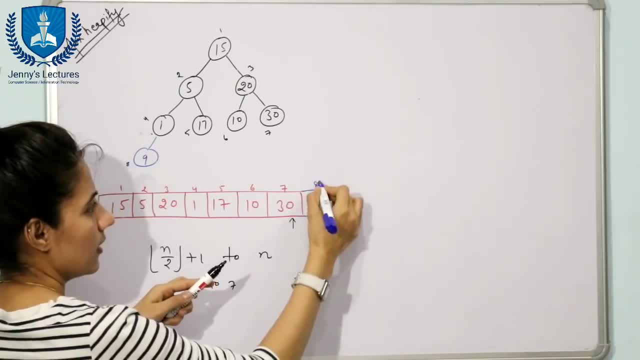 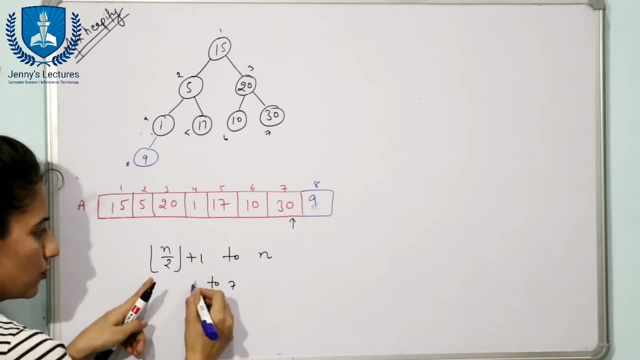 inserted this in the array. we will insert 8 here at the 8th index. now n value is 8. now 8 by 2, that is 4. 4 plus 1 is 5. from 5 to 8 we are having leaf node. so from 5 to 8 we are having leaf node. so 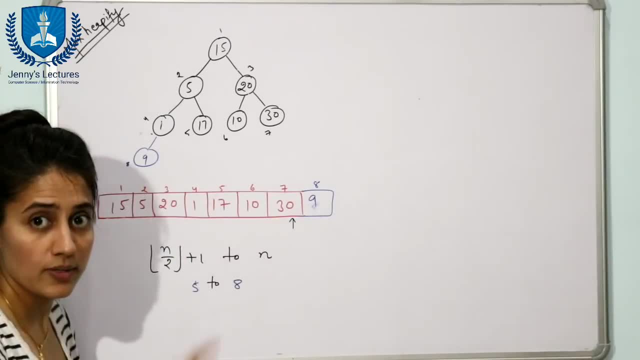 from 5 to 8: 5, 6, 7, 8 in the trick also you can see. so this is the formula. leaf node would be from here to here. now we are going to start our heapify method from the known leaf element, which is at the 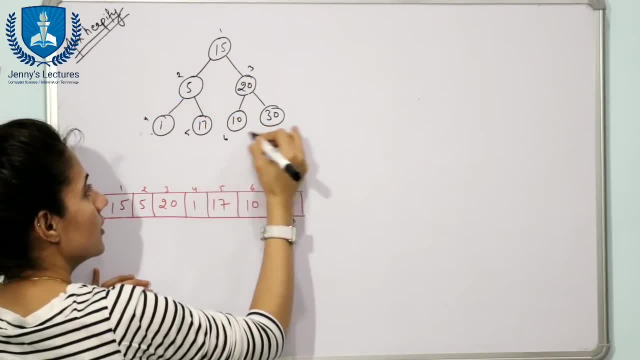 this definition. so let me get back in that section. I will at a next slide too. that way you can be able to find and 7. now at index, 4, 5, 6 and 7, all the nodes are leaf node. so just leave those nodes and we are. 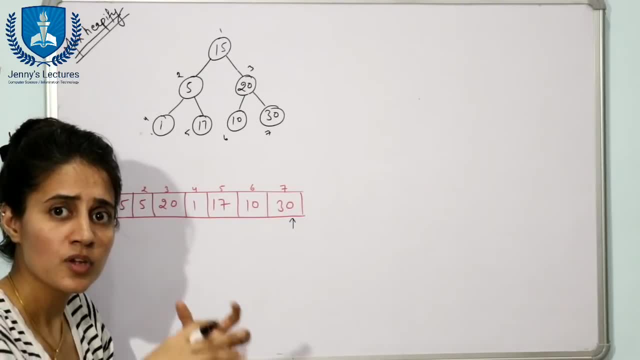 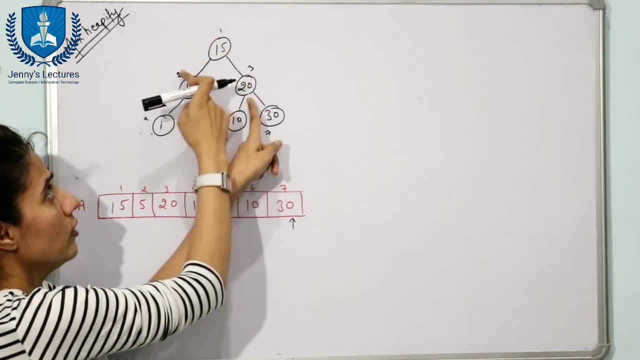 going to start a loop or we are going to start a hippify method from 20 only and index of 20 is 3. the non-leaf node are on the index 1, 2 and 3, so the largest index is 3, which is having the 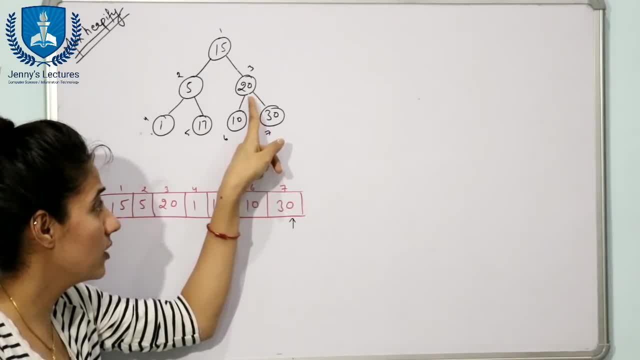 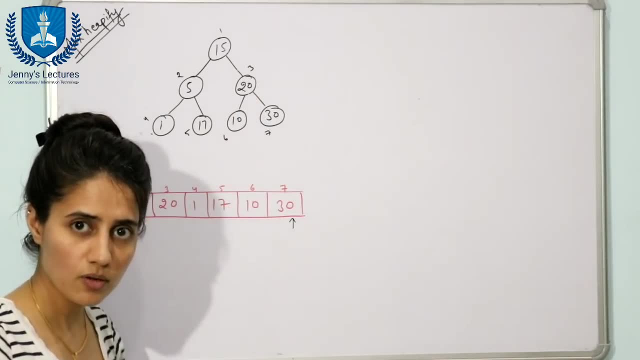 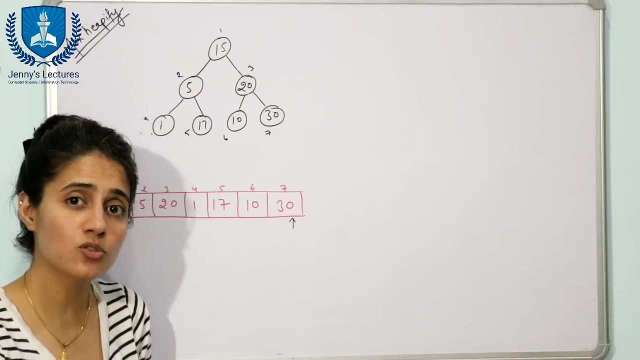 non-leaf node. so we are going to start our apply, our hippify method, from here the non-leaf element which is at the largest index. fine, now how to find out which, at which index we are having leaf node and from which index non-leaf node is going to start from which the largest index. 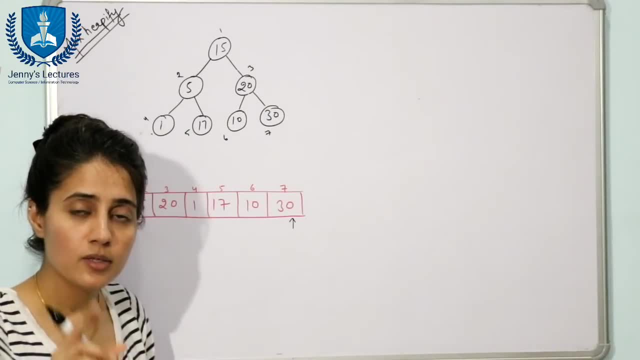 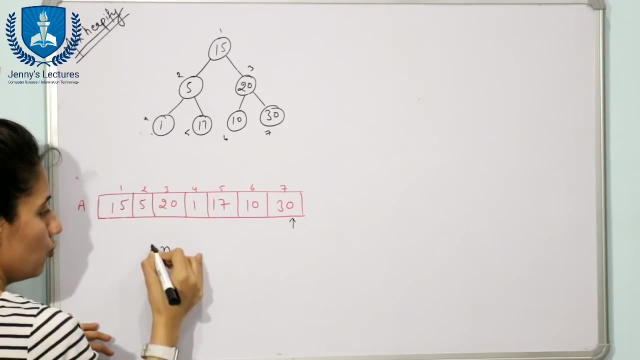 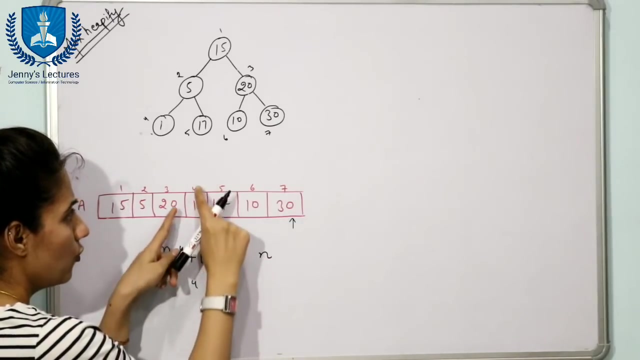 non-leaf node is going to start. so in a complete binary tree, the property of complete binary trees, the leaf node would be from n by 2 floor value plus 1 to n. here you can see that. check here. n value is 7, 7 by 2, 7 by 2 is 3.5, floor value is 3, 3 plus 1 is 4. so from from 4 to 7, 4, 5. 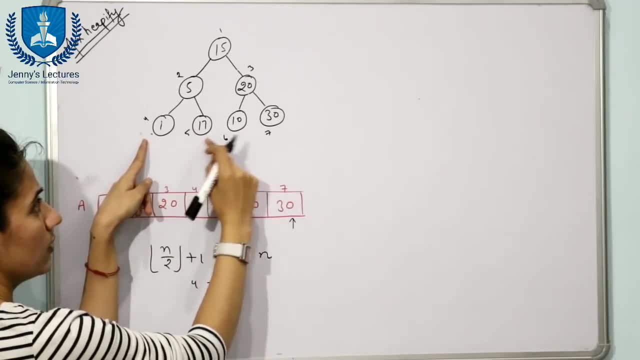 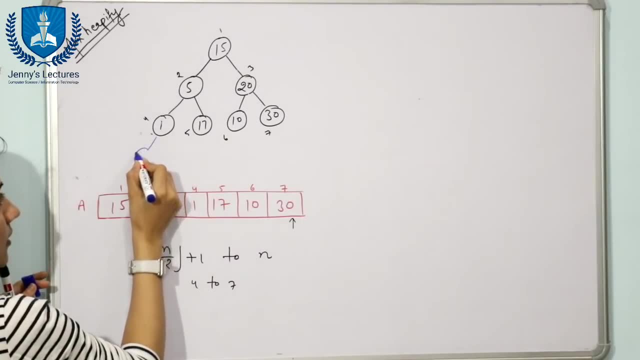 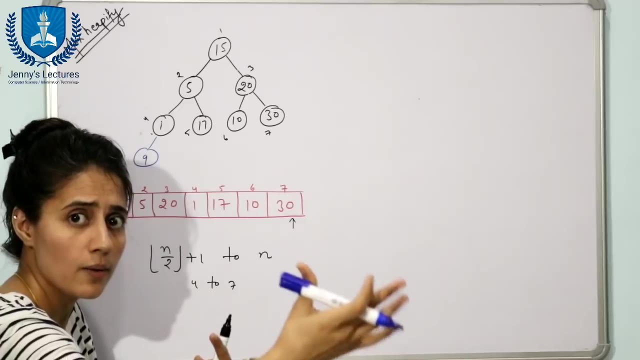 6, 7. these are leaf node, as you can see in tree 4, 5, 6, 7. these are leaf node. suppose if i add one more element here, see, this tree is not still a maxi. we are going to hippify this to to make it a maxi. 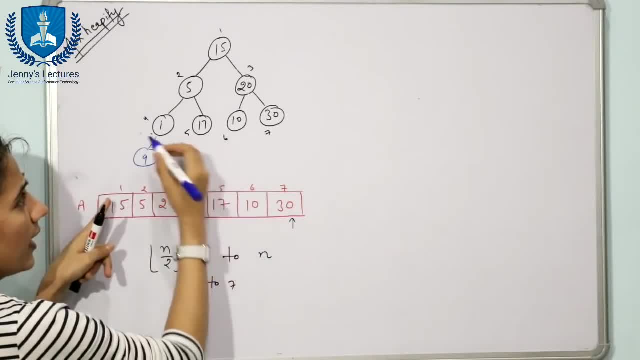 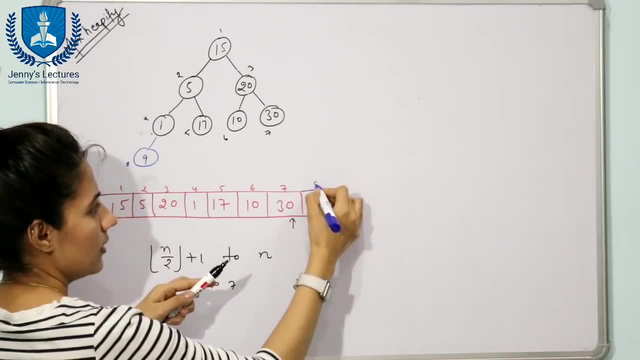 so suppose we have inserted 9 here. now leaf node are at the index 7, and here we have 8. suppose here we have inserted this in the array, we will insert 8 here at the 8th index. now n value is 8, now 8 by. 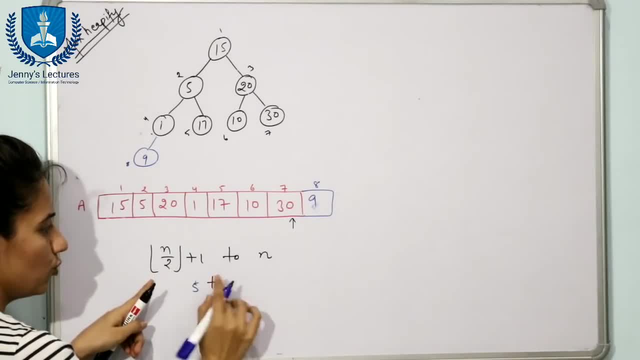 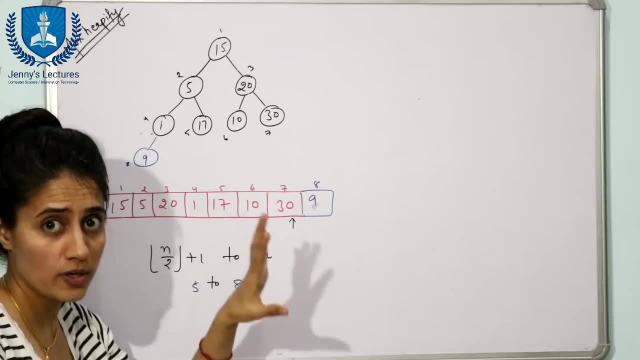 2, that is 4, 4 plus 1 is 5, from 5 to 8. we are having leaf node, so from 5 to 8: 5, 6, 7, 8 in the trick also you can see. so this is the formula. leaf node would be from here to: 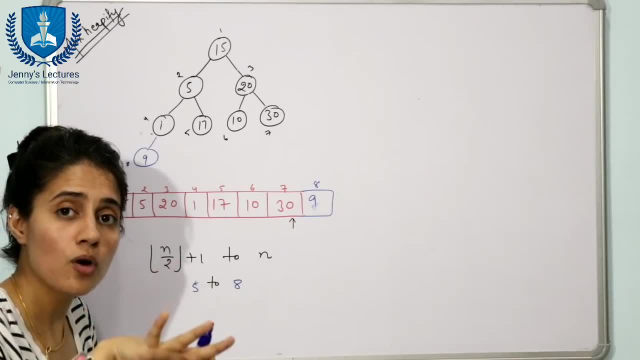 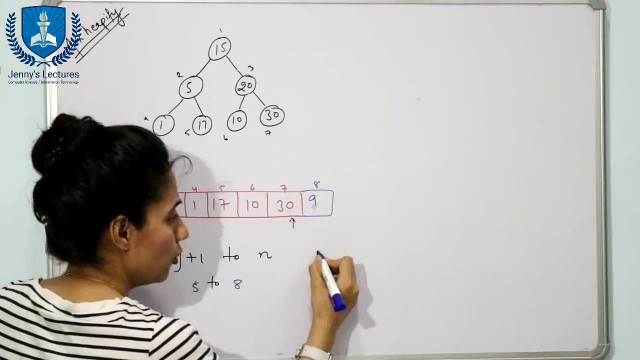 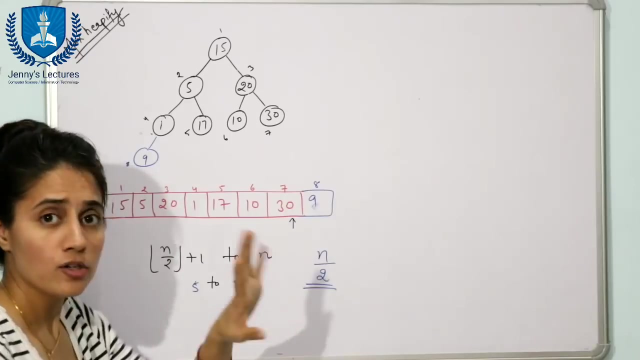 here. now we are going to start our hippify method from the non-leaf element, which is at the largest index. so from where we are going to start? we are going to start from n by 2. see here, n is 8. 8 by 2, that is 4. go to the fourth index. at fourth index we have 1 in the tree. also, you can say: 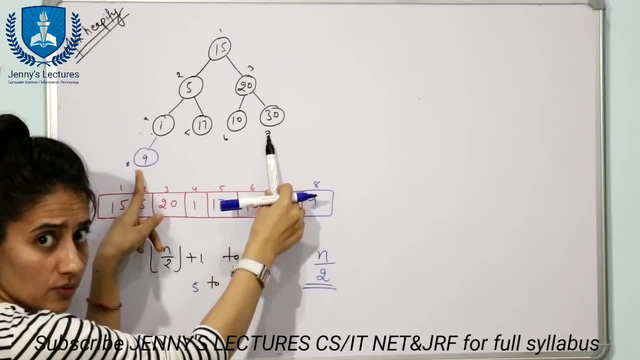 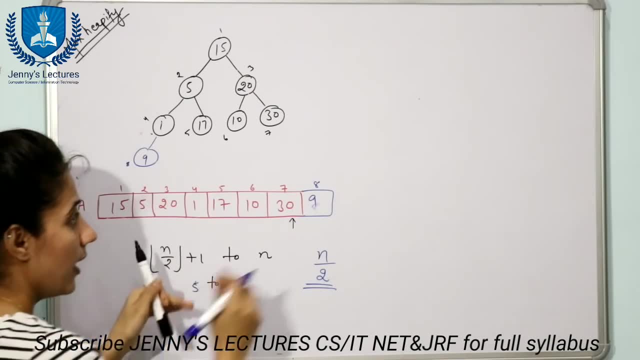 this, this, this, this are leaf node and non-leaf node is starting from index 4, so from here we are going to start our hippify method: from the non-leaf element, which is at the fourth index. this is the largest index, right, and if you delete this 9, this is what this was our. 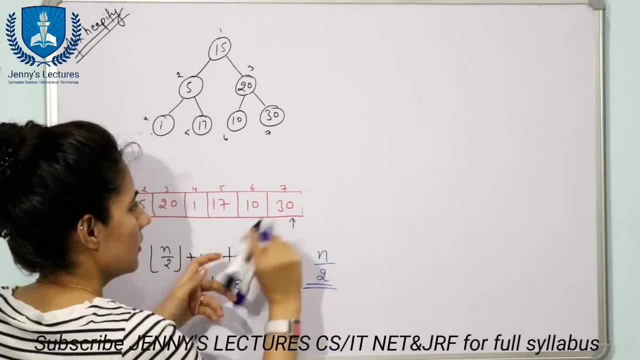 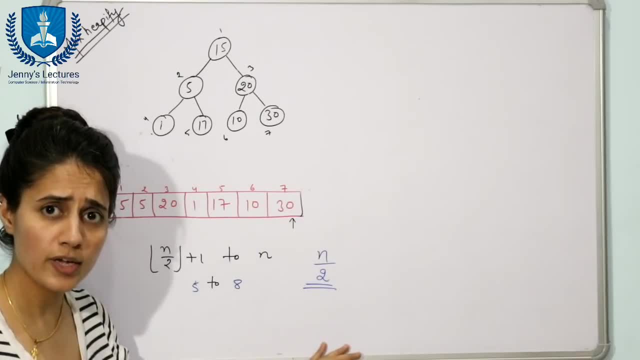 original tree. so i am going to delete this 9. now here n is what: 7, 7 by 2, integer value. we are going to take 3.5. we are going to take now 3. only go to the index. third, that is 20. here check, we are going. 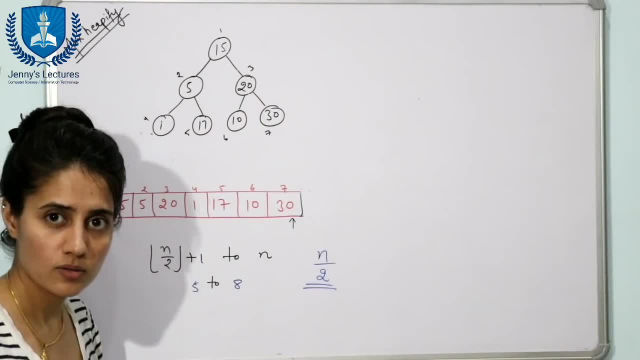 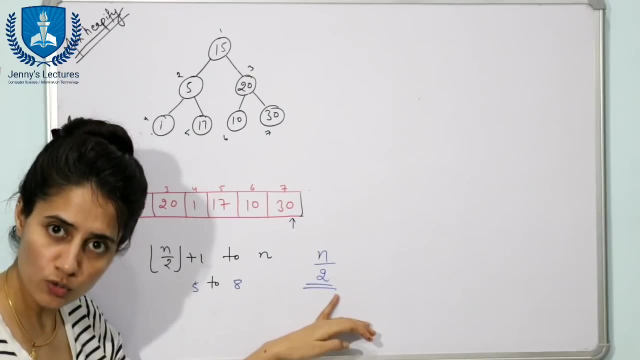 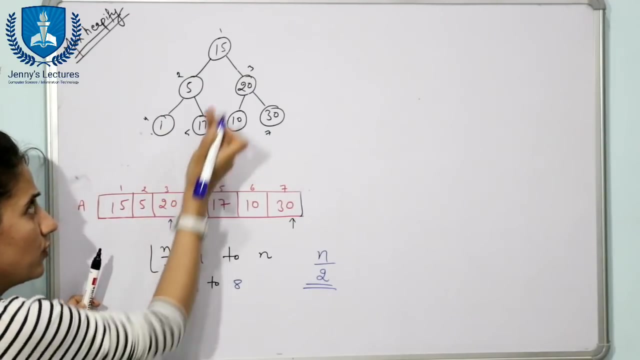 to start our hippify method from here only. so in this case, hippify method would be started from n by 2, one variable we are going to take, and from here only we are going to start that variable and that variable. variable would be decremented after 20. 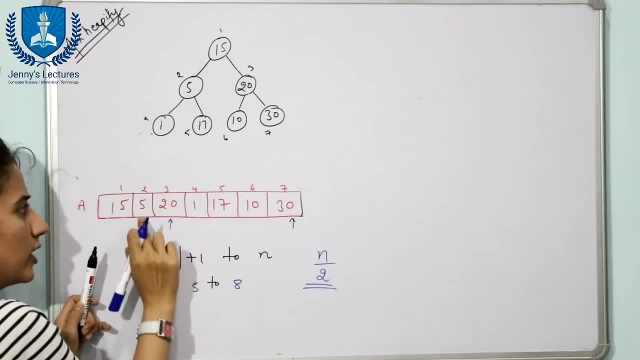 we are going to check 5. so 5 is at index 2. so we are going to decrement that variable again. we are going to decrement, and we have reached to the root node. till we reach to the root node. if you are going to take here index from 0, then then here you will write n by 2 minus 1. 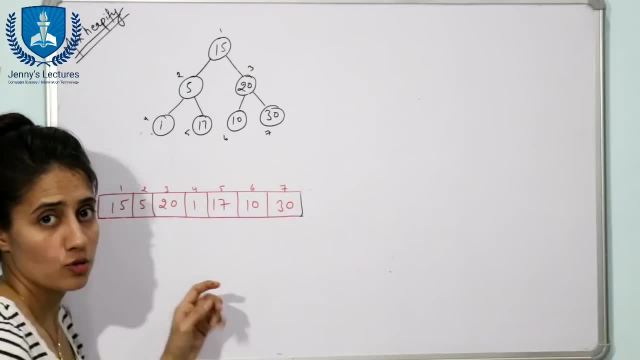 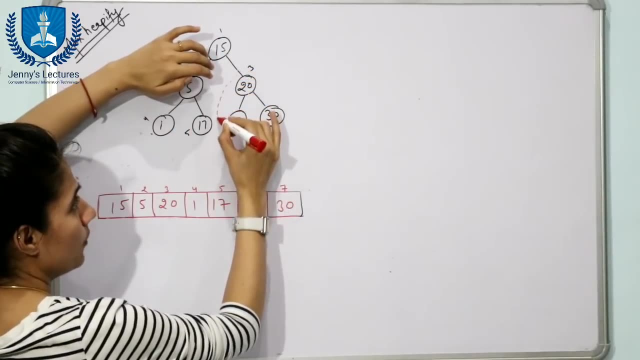 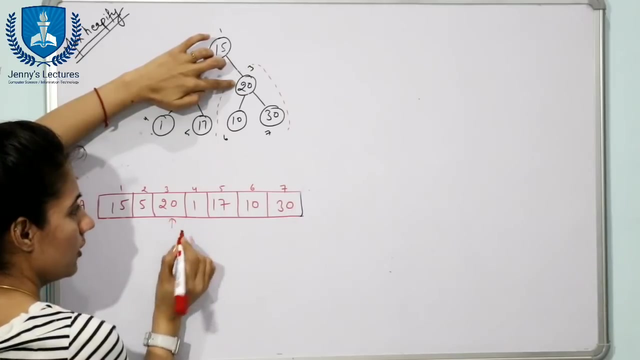 we are going to start our hippify method from n by 2 minus 1. so let us start to apply our hippify method. see, we are going to apply from here now. we are going to make this, this tree, as a max heap only because index is 3. we are going to start from here only because these are leaf node, no need to. 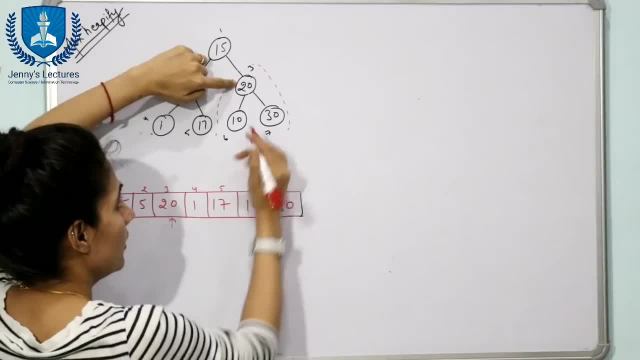 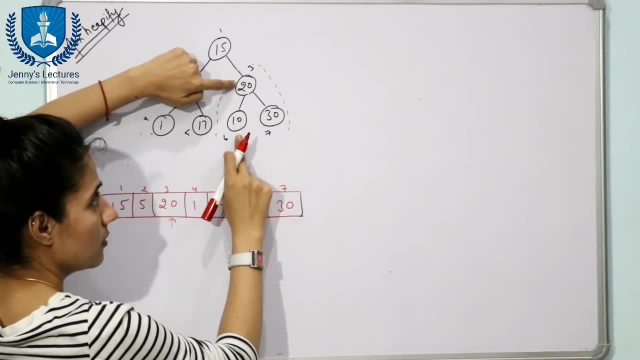 apply hippify method here, because these are itself a max heap. now find out child. of this 20, one is 10, one is 30. compare with this 10. this one is not larger than this parent, but 30 is greater than this parent. so we are going to swap. 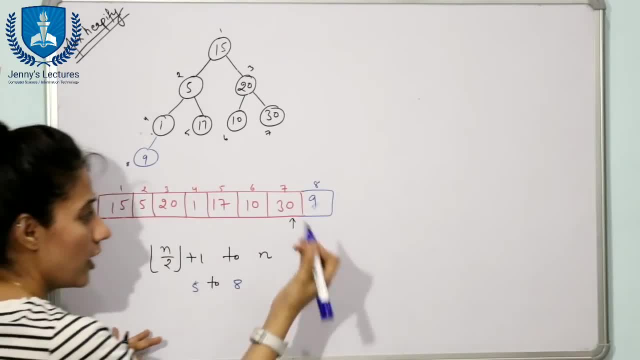 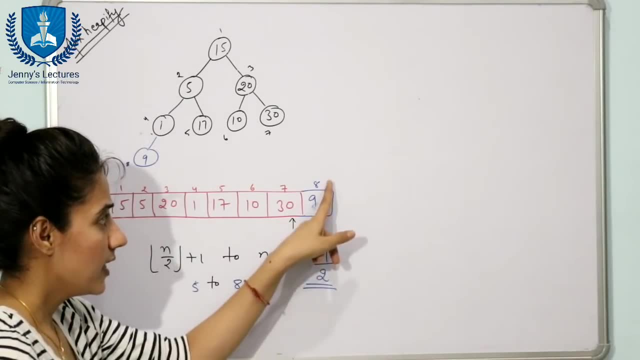 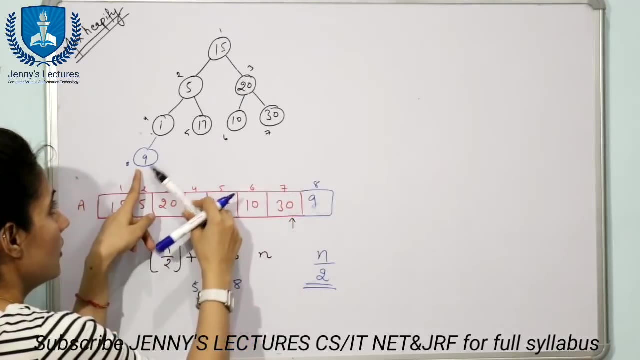 largest index. so from where we are going to start? we are going to start from n by 2. see here: n is 8, 8 by 2, that is 4. go to the fourth index. at fourth index we have 1 in the tree. also, you can say this: this, this, this are leaf node and non leaf node is starting from: 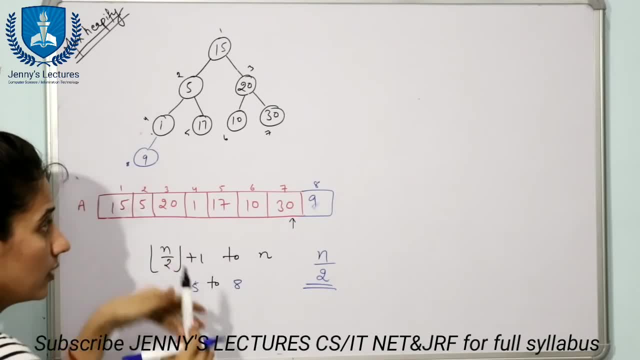 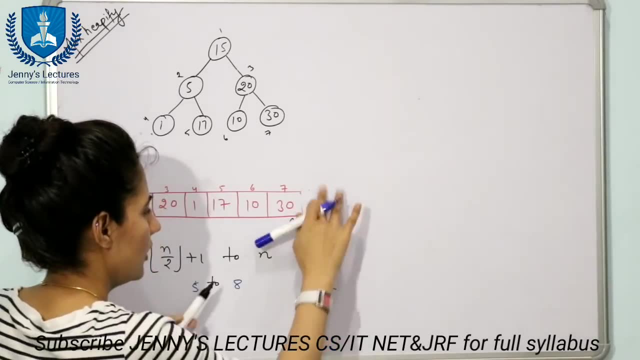 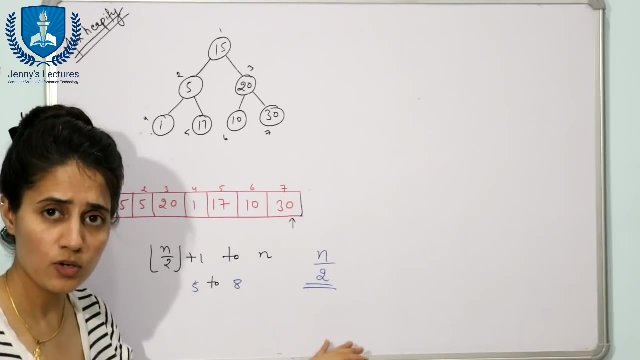 index 4. this is the largest index right, and if you delete this 9, this is what. this was our original tree, so i am going to delete this 9 now, here n is what 7, 7 by 2 integer value we are going to take. 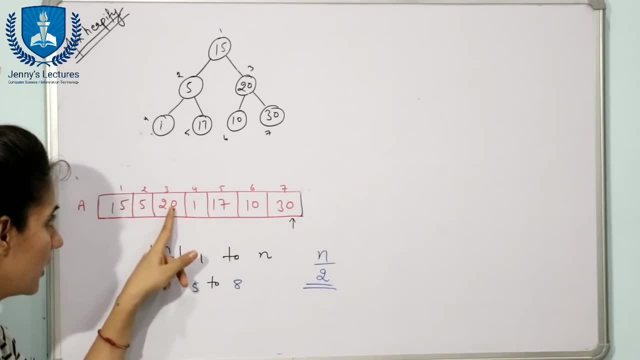 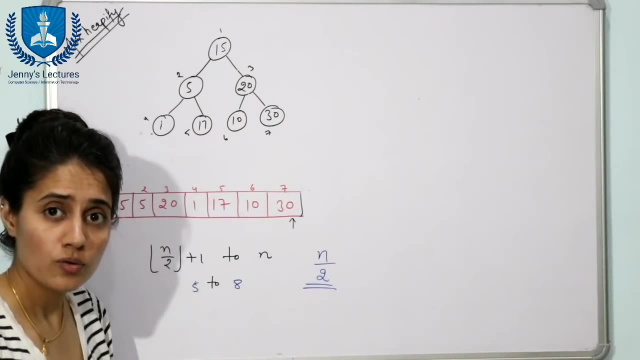 3.5. we are going to take now 3. only go to the index 3 and we are going to take 3.5, and we are going to take 3.5. that is 20 here. check: we are going to start our heapify method from here only so in this case. 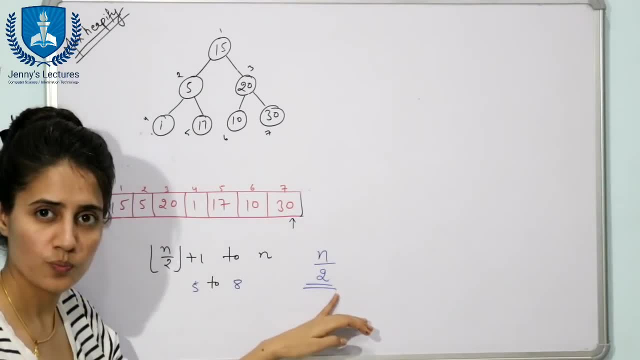 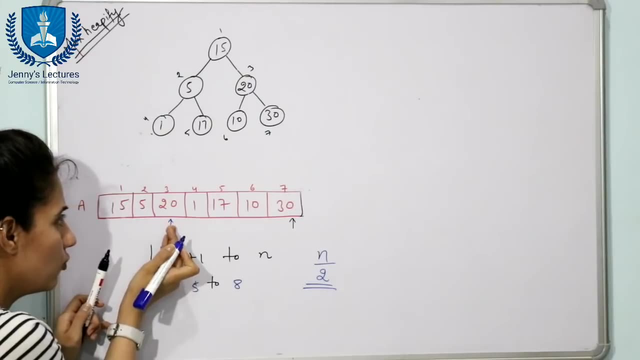 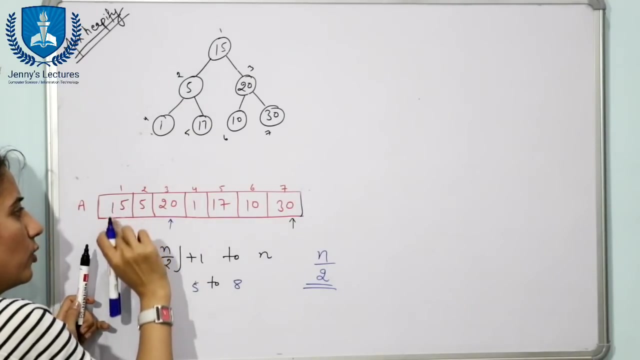 heapify method would be started from n by 2, one variable we are going to take and from here only we are going to start that variable and that variable would be decremented after 20. we are going to check 5, so 5 is at index 2, so we are going to decrement that variable again. we are 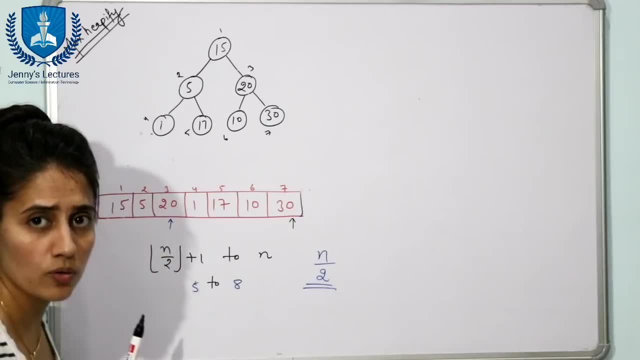 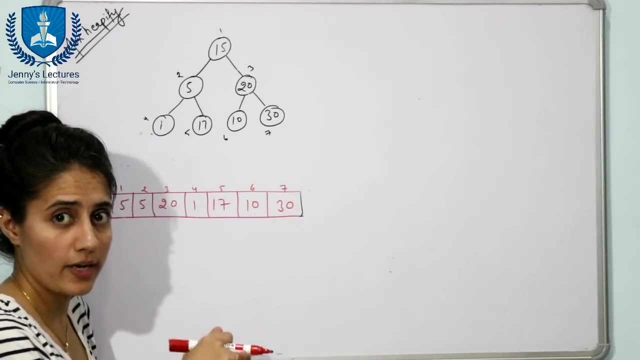 going to decrement and we have reached to the root node. till we reach to the root node, if you are going to take here index from 0, then then here you will write n by 2 minus 1. we are going to start our heapify method from n by 2 minus 1, so let us start to apply our heapify method. see: 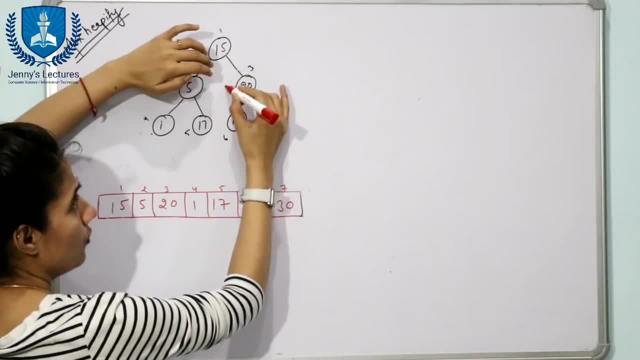 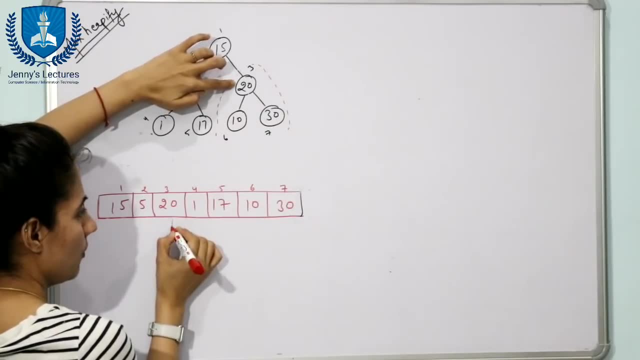 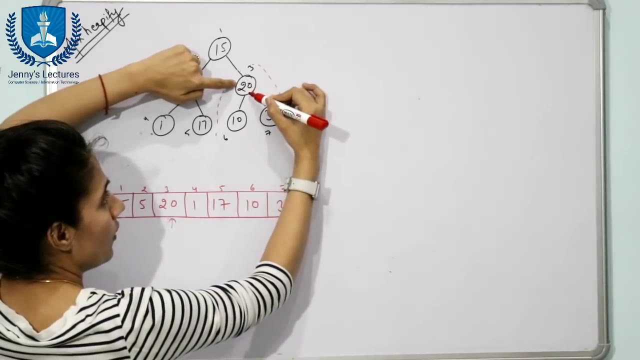 we are going to apply from here now. we are going to make this, this tree, as a max heap only because index is 3. we are going to start from here only because these are leaf node. no need to apply heapify method here because these are itself a max heap. now find out child of this: 20, one is 10, one is 30. compare with this 10, this one. 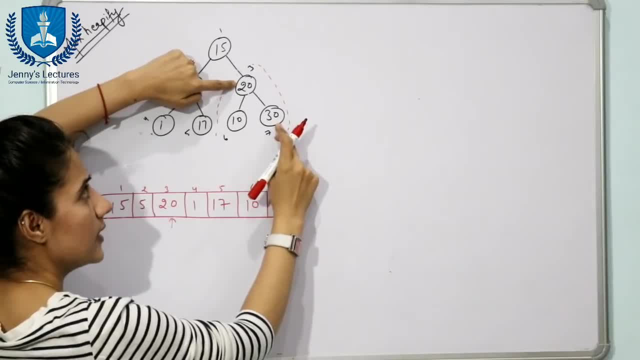 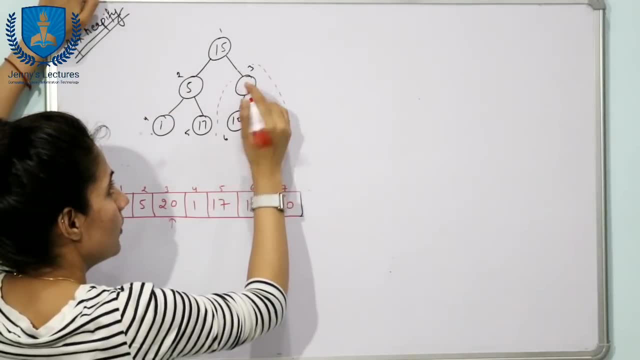 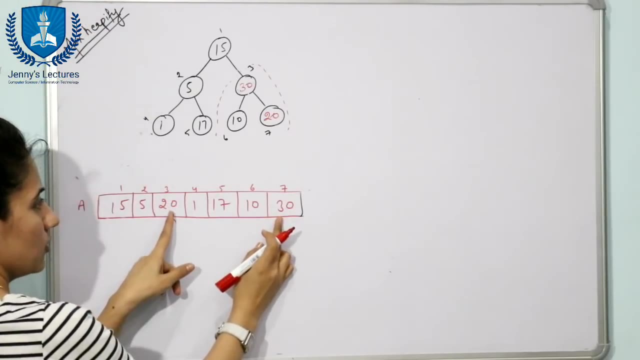 is not larger than this parent, but 30 is greater than this parent. so we are going to swap: 20 would go down, 30 would go up. so after swapping this tree would be 30 and 20. right here also, you are going to swap this 20 and 30. so here you will write what: 30. 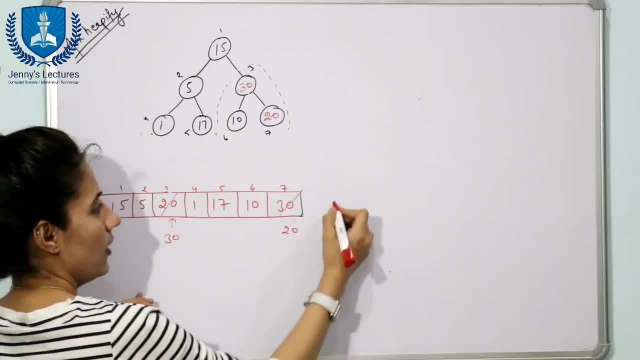 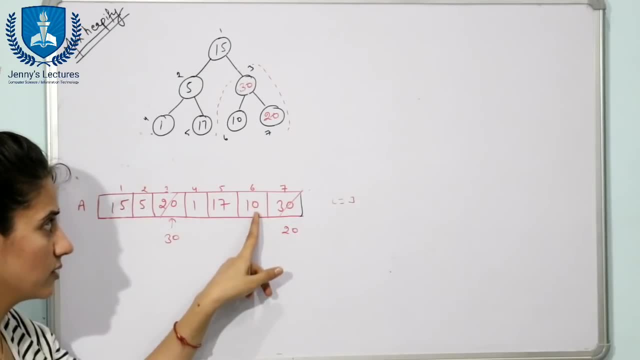 and here you will write 20. see here i value is 3, find out the left child and right. left is 3 into 2, that is at 6th index and right would be at 7th index. so here which one is greater: 30, 30 compare. 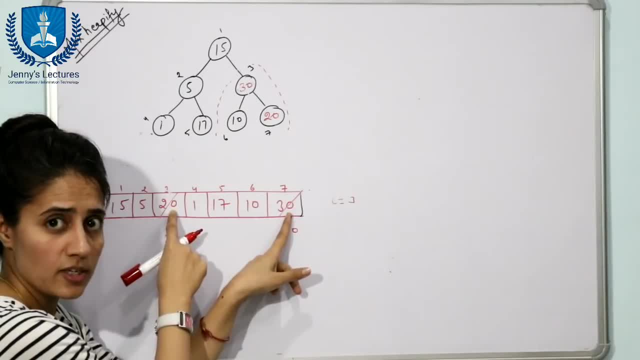 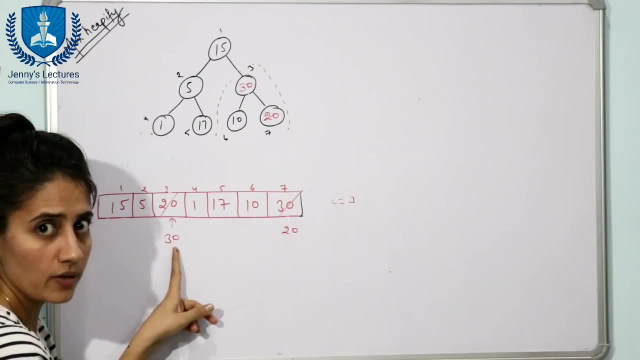 30 with 20. so obviously 20 is less than parent is less than so. that is not possible. so we are going to swap these two. now array would be something like this: here we will write 20, here we will write 30.. fine, now this, this. 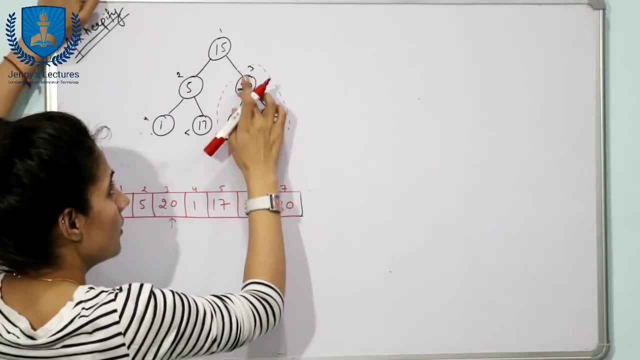 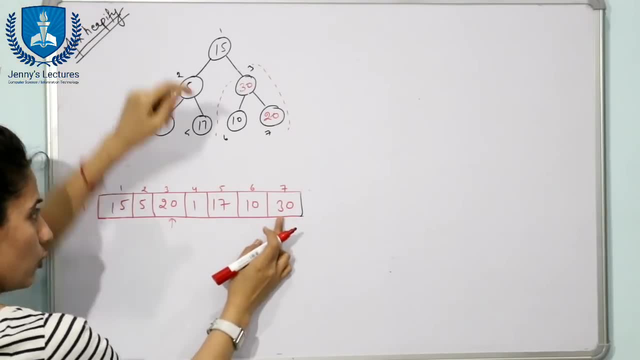 20 would go down, 30 would go up. so after swapping this tree would be 30 and 20. right here also, you are going to swap this: 20 and 30. so here you will write what- 30, and here you will write 20.. 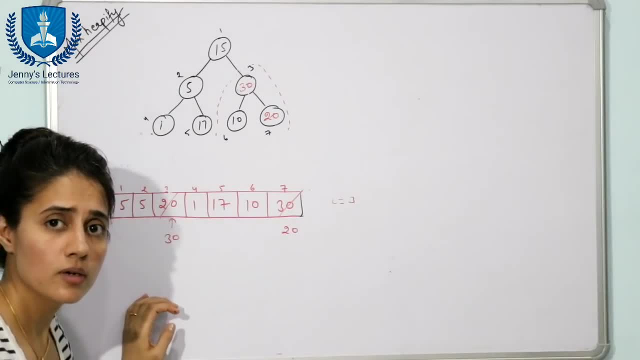 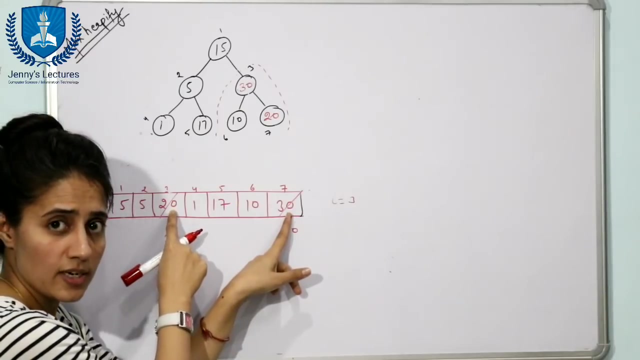 see here: i value is 3, find out the left child and right, left is 3 into that is at sixth index and right would be at seventh index. so here which one is greater: 30, 30, compare 30 with 20. so obviously 20 is less than parent is less than so that is not possible. so 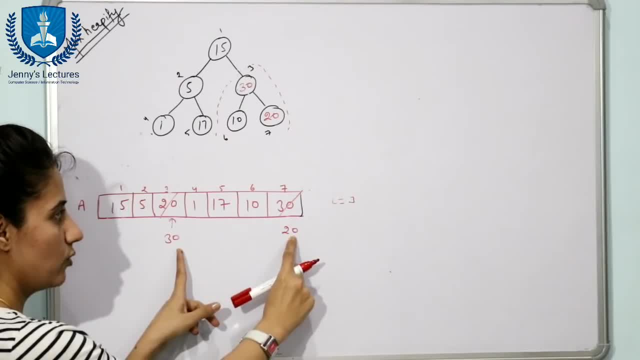 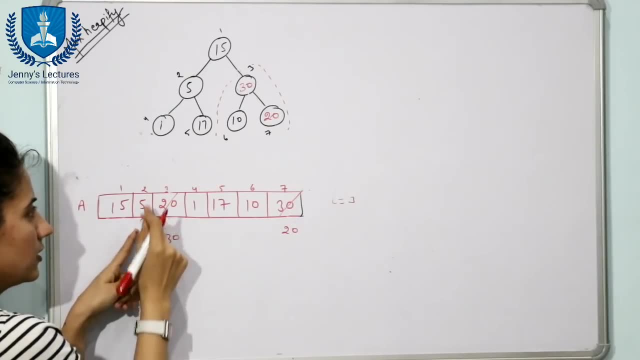 we are going to swap these two. now array would be something like this: here we will write 20, here we will write 30. fine, now this, this, this, this variable would be decremented. now i is at this place, at 2.. now we are going to check this one. you have to make this as a max here. 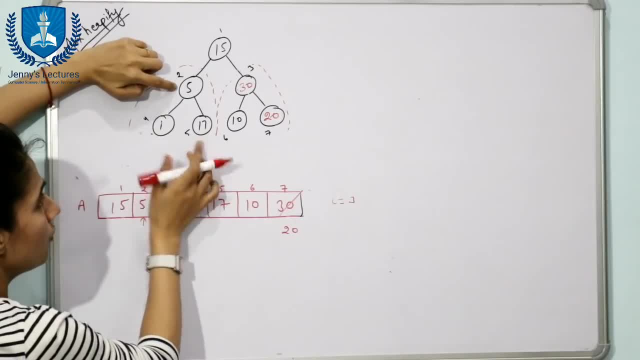 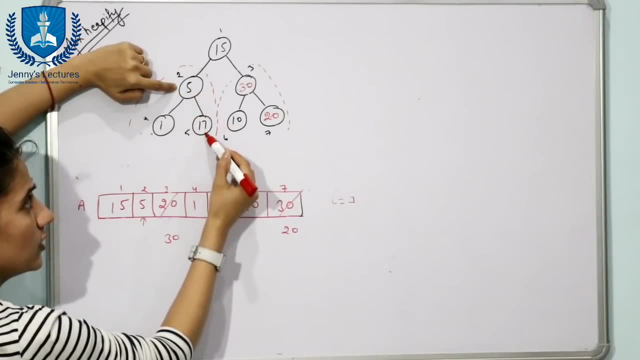 5. now check 5. find out left child and right child. 1 is left, 17 is right. 5 would be shifted with this 17 because 1 is less. than so no need to do shift. 17 is greater than this parent, so we are. 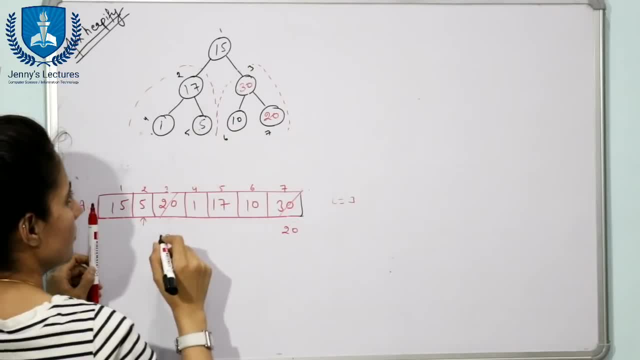 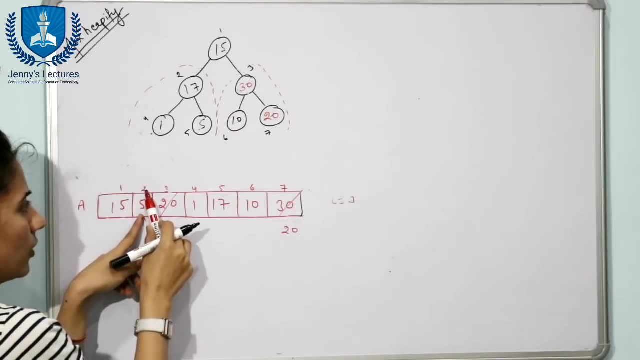 going to shift. here you will write 5.. here also you can say this: left side of this is 2 into, i is 1 and i is here 2.. left is 2 into 2 at 4 point. so this is possible. so we can say that the left child of this is 2 into, i is here 2, left is 2, two into 2 at 4 point. 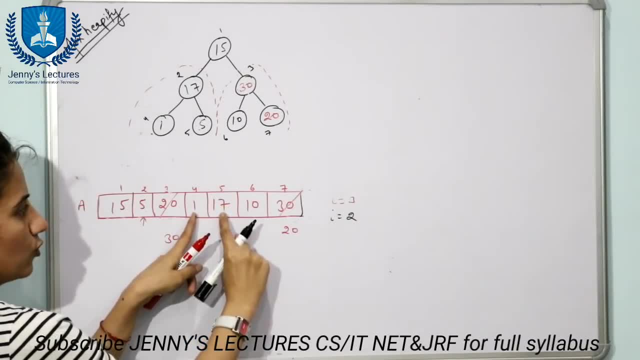 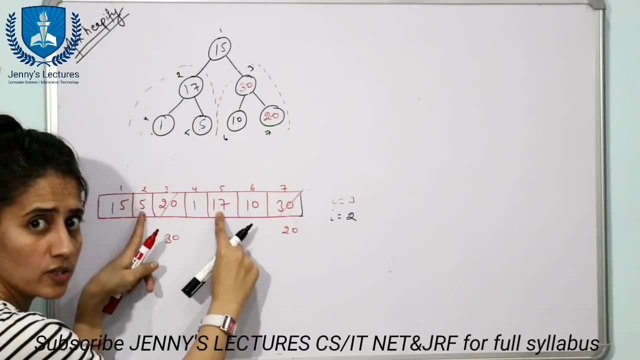 to the left is 2 into 2 at 4 point. here you can write down: right child is fourth index and right child would be at fifth index. which one is larger, 17, 17, compare with this. 5. so we are going to 5 is less than 17. which one is? that is parent and that is not allowed. 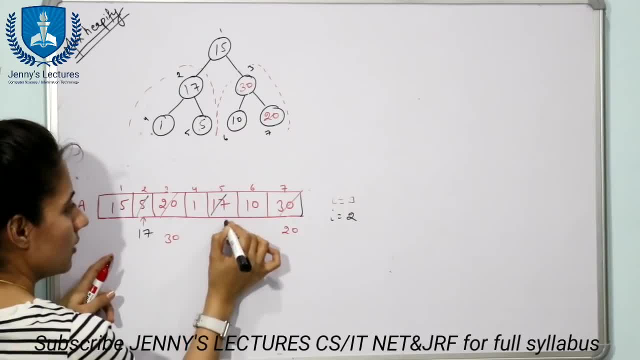 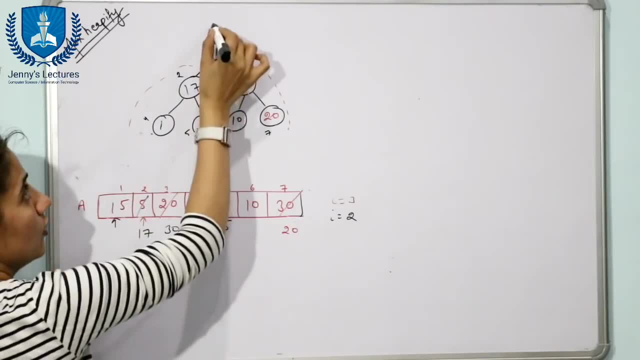 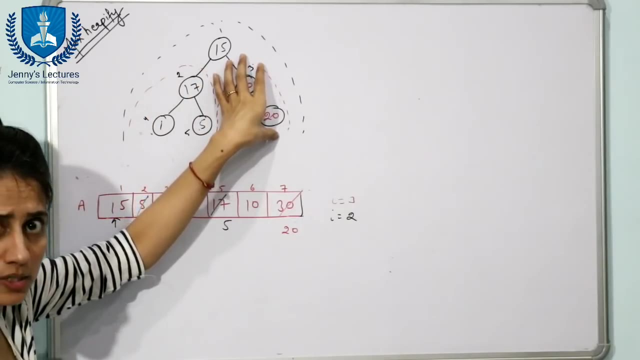 so you are going to do what? 17 would be here and 5 would be at this place in the array. fine, now this variable would be decremented. we have now at 15. now we are going to make this complete as a max heap: see 15. this left is a max heap. this right is also a max heap. right subtree. now we 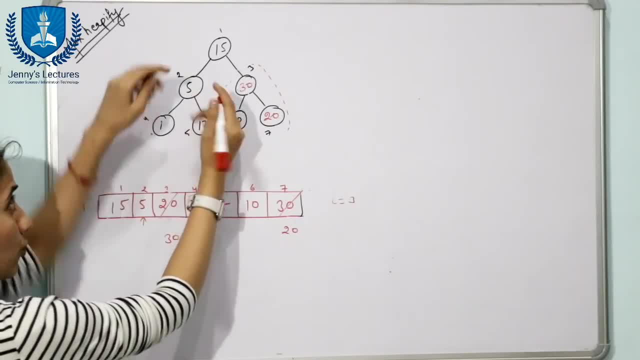 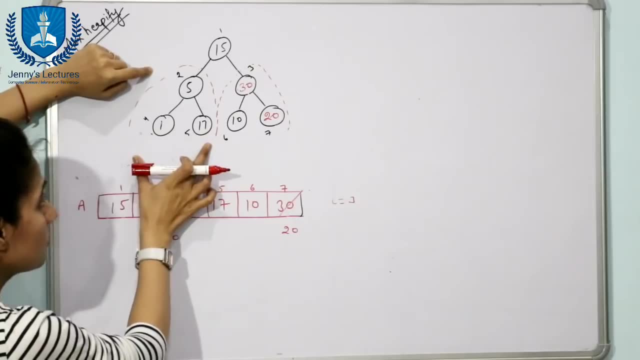 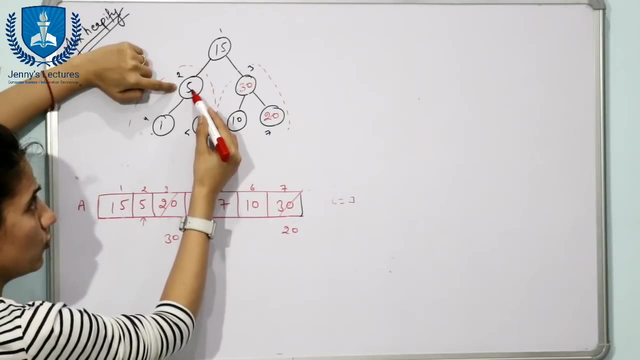 this variable would be decremented. now i is at this place at 2.. now we are going to check this one. you have to make this as a max heap. fine, now check 5. find out left child and right child. 1 is left, 17 is right. 5 would be shifted with this 17 because 1 is less than so no need to do shift 17. 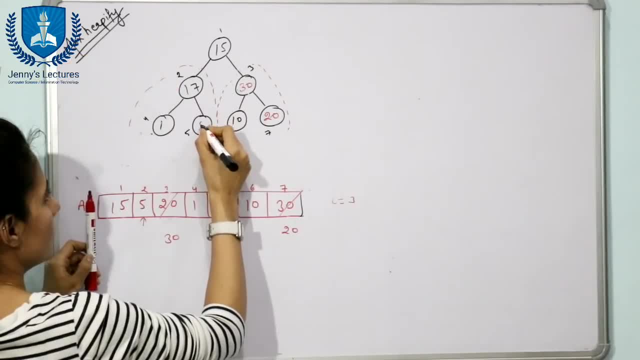 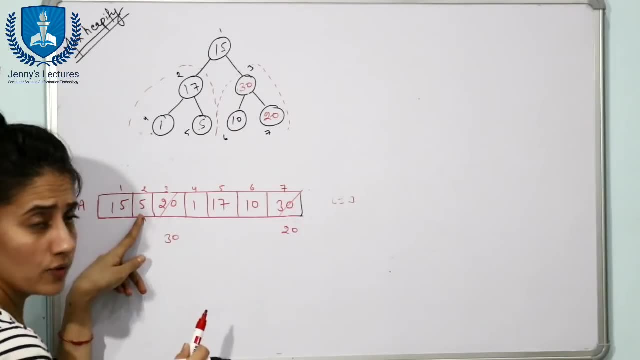 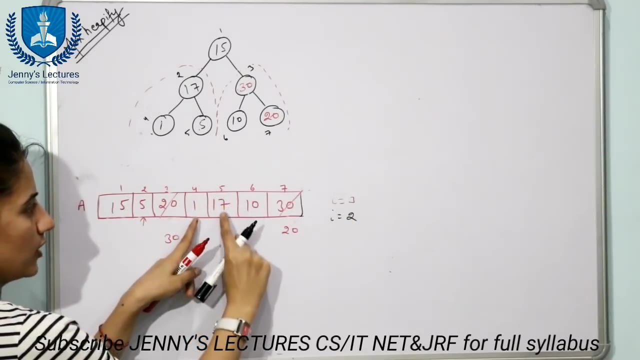 is greater than this parent, so we are going to shift. here you will write 5.. here also you can say this: left child of this is 2 into i is here, 2 left is 2 into 2 at 4th index and 4th child would be at 5th index, which. 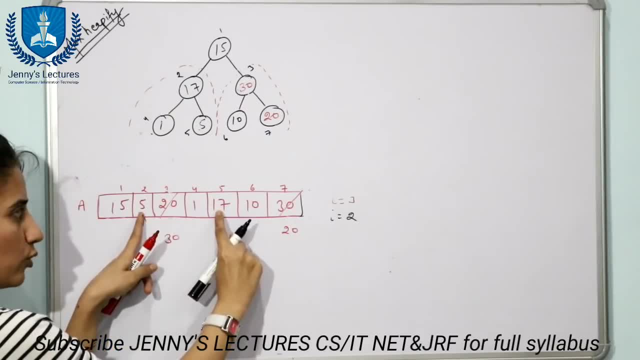 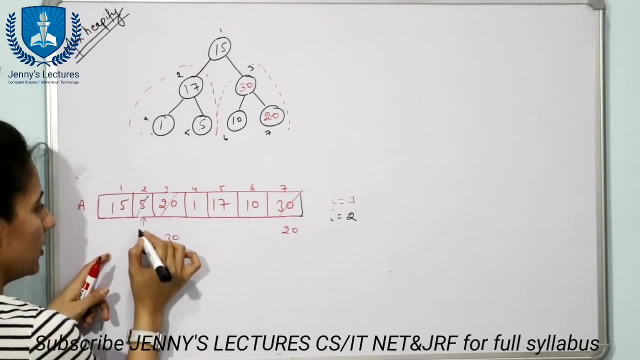 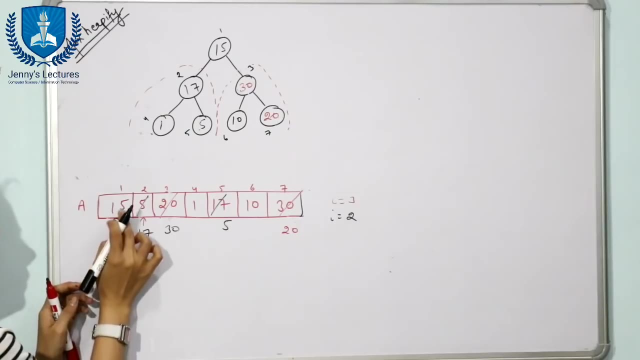 1 is larger, 17, 17 compared with this five. so we are going to: 5 is less than 17, which one is that is parent and that is not allowed. so you are going to do what? 17 would be here and 5 would be at this place in the array. fine, now this variable would be decremented. we have 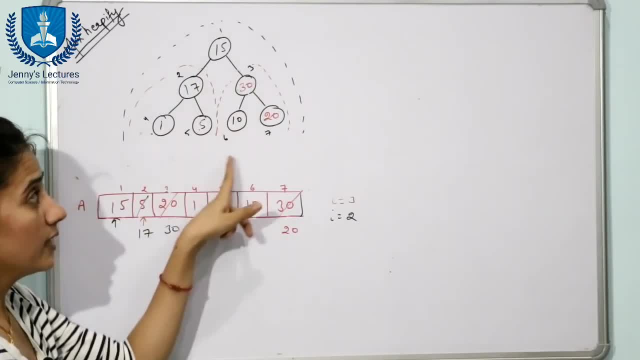 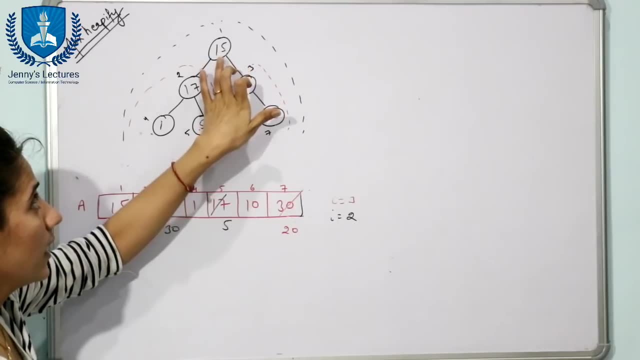 now at 50: 15.. Now we are going to make this complete as a max heap: See 15.. This left is a max heap. This right is also a max heap: Right subtree. Now we have added this 15.. Now you have to make this. 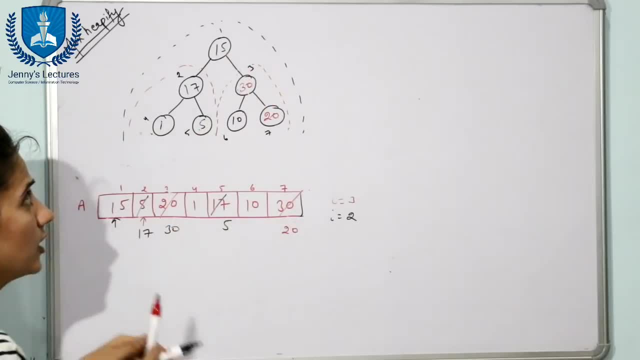 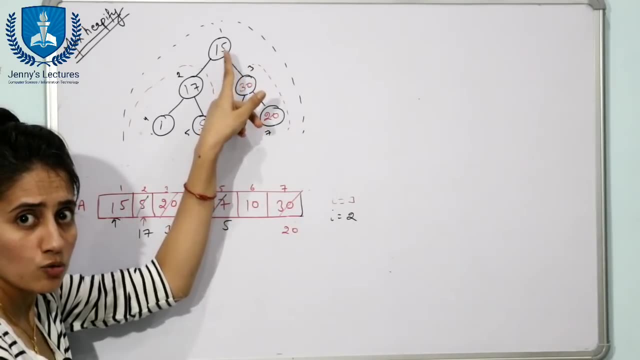 complete as a max heap. Now find out left and right side of 15.. 17 and 30. Which one is greater? 30. 30 is compared with 15.. 15 is less. So we are going to shift Here. you will write 15 and 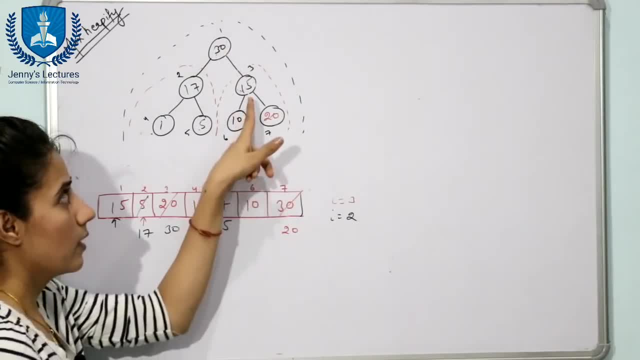 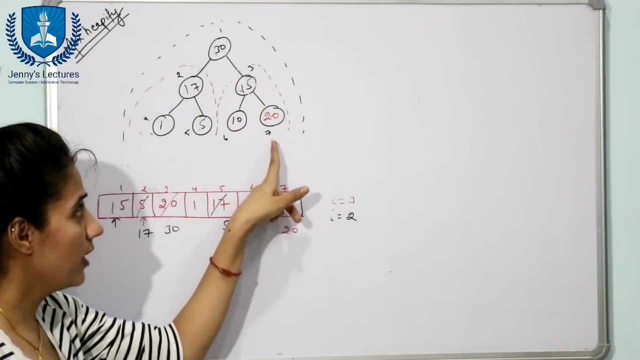 here you will write 30. But we are not done here. We are going to do the same process till we reach to the. this n value n is 7.. So now, child of this 15 is 10 and 20.. Which one is greater? 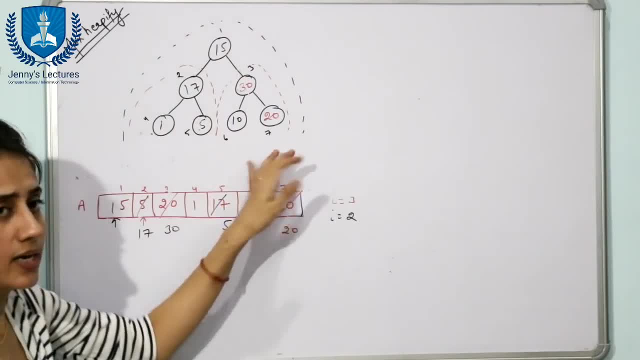 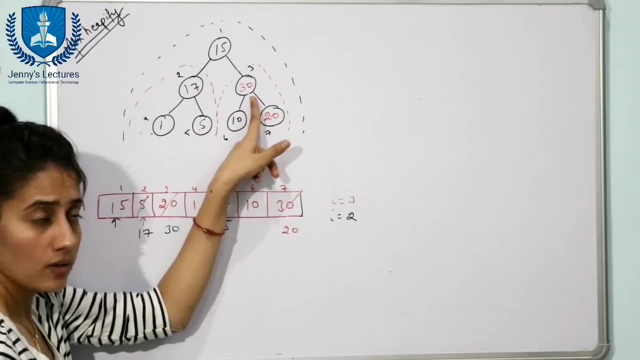 have added this 15. now you have to make this complete as a max heap. now find out left and right, child of 15, 17 and 30, which one is greater? 30, 30 is compared with 15, 15 is less. so we are. 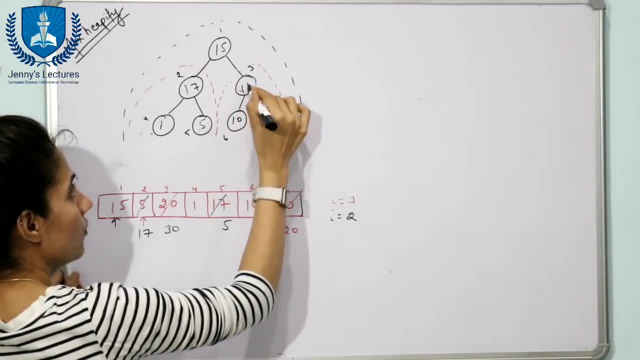 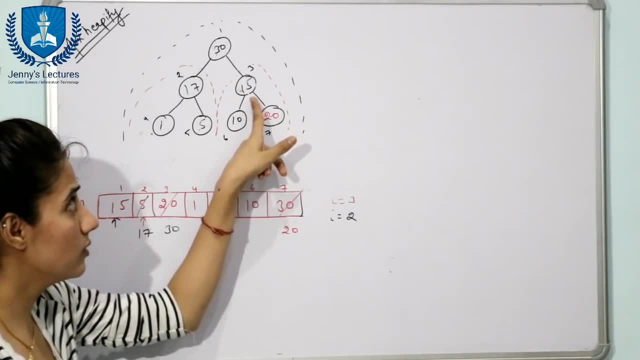 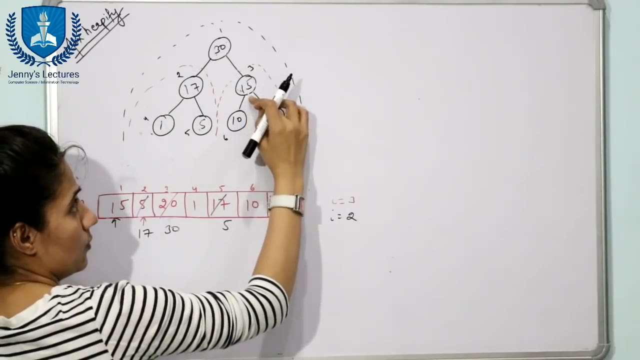 going to. we are going to shift: here you will write 15 and here you will write 30, but we are not done here. we are going to do the same process till we reach to the this n value n is 7, so now child of this 15 is 10, and 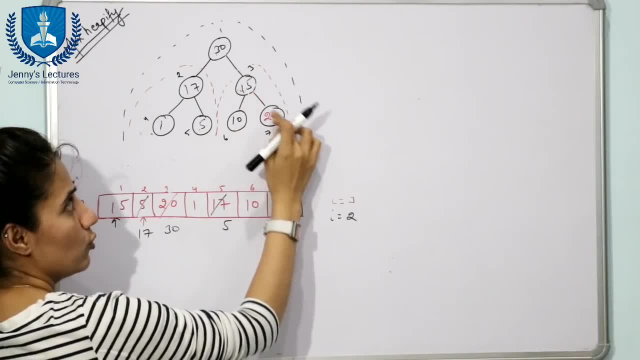 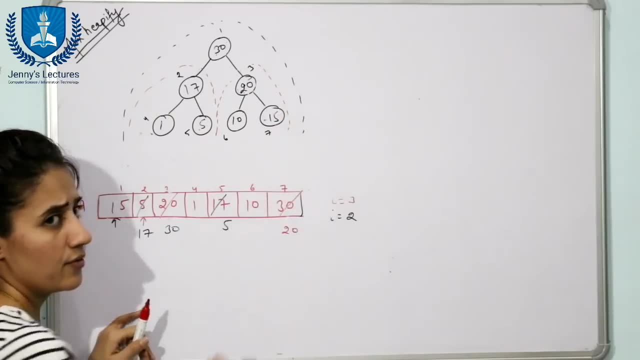 20. which one is greater? 20? 20 is compared with 15, so we are going to swap: here you will write 20 and here you will write 15. now there is no left and right child. we have reached up to this. 7: the 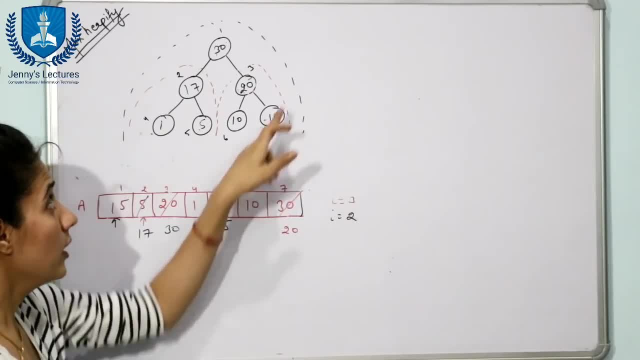 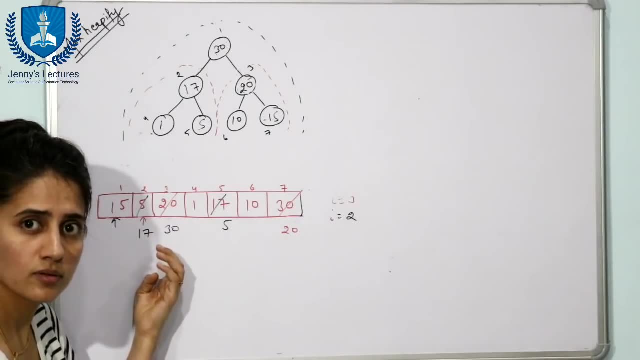 you know, at the end of this array, now we are going to stop. now, this is a max heap. this is how we are going to apply the heapify method from here only from right to left. okay, and this, this would take a time. complexity of order of n. 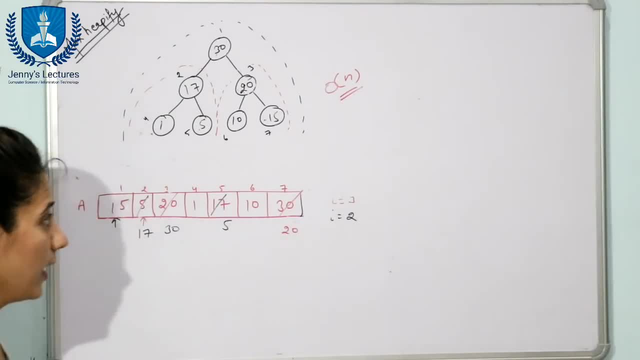 fine, and see here here in the array how you will update. i is 1, so left child would be at 2, right child would be at 3, so at 2 we have 17 and right we have 30, which one is greater, 30, 30 would be. 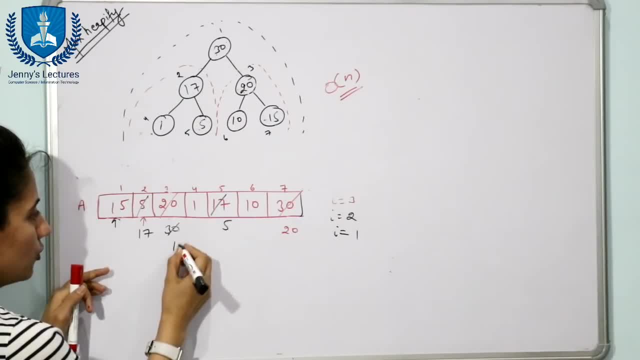 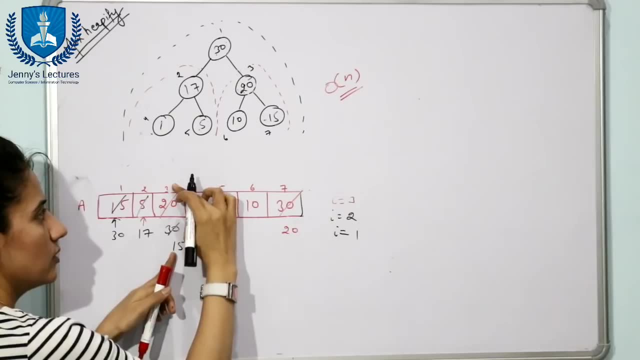 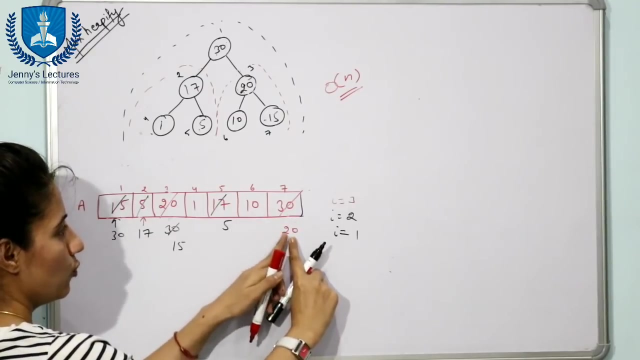 exchanged with this one. here you will write 15 and here you will write 30, then 15. 15 is at index 3, left child of this 3 is at 6th and right child would be at 7th index. at 6th we have 10. at 7th we have 20. which one is greater? 20, 20 is. 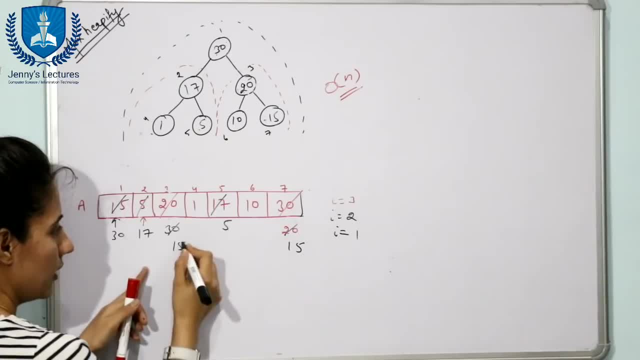 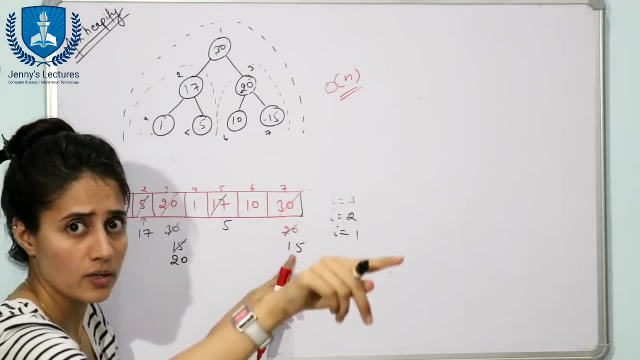 compared with again this 50. now we are going to shift: here we will write 15 and here you will write 20. right now, find out: left child of 15, 7 into 2, that is 14. but 14 index is greater than this. 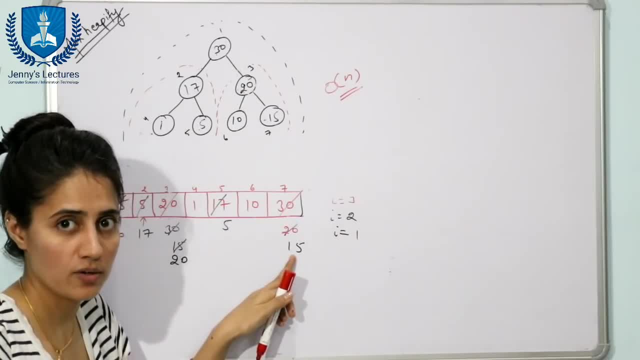 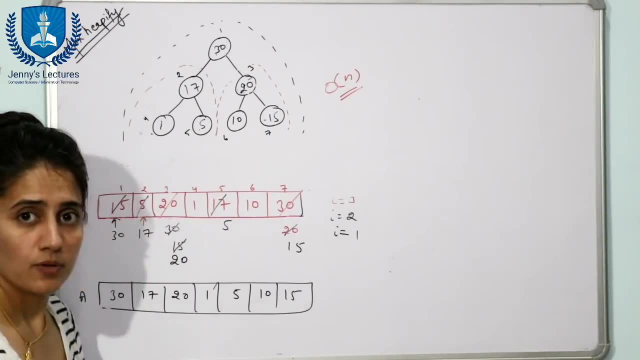 total of 30, and we are going to stop here. this is N, so we are going to stop here. we are not going to apply heapify here. fine, so after updation, the array would be something like this: now, this is max heap. first step is over. using heapify method, we have built max heap. now the next step. 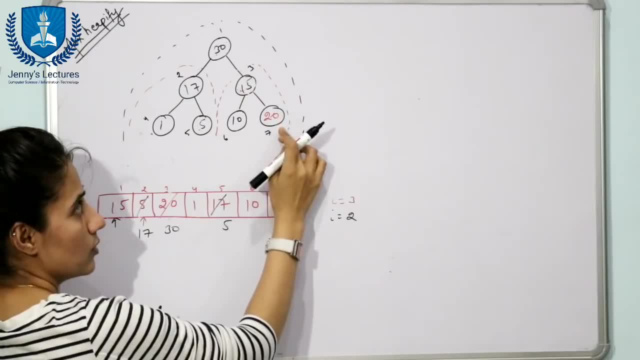 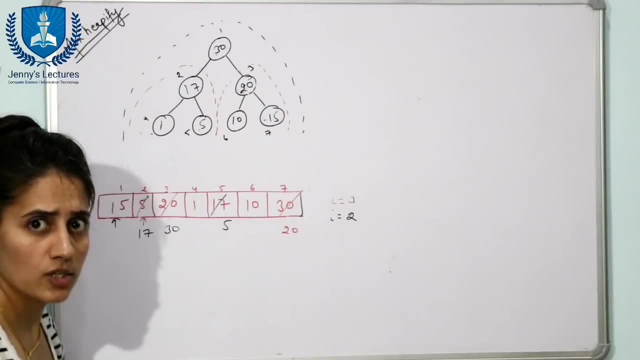 20? 20 is compared with 15.. So we are going to swap: Here you will write 20 and here you will write 15.. Now there is no left and right child. We have reached up to this. 7. The- you know. 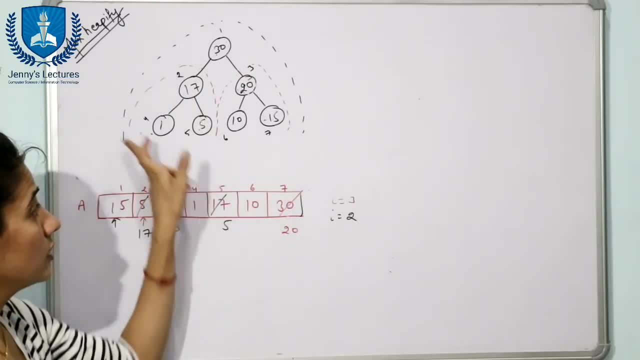 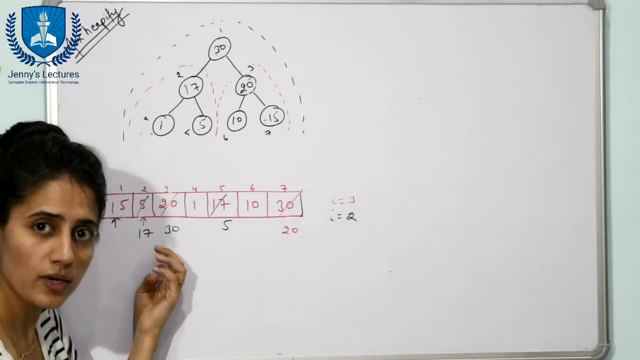 at the end of this array. Now we are going to stop. Now, this is a max heap. This is how we are going to apply the heapify method From here only From right to left. Okay, And this this: 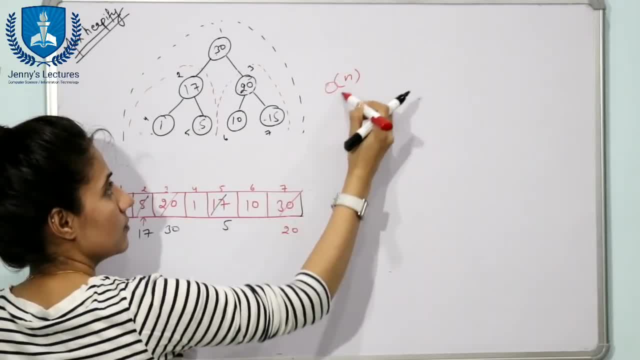 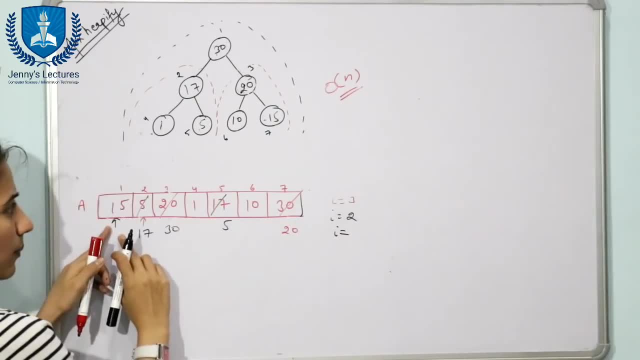 would take a time. complexity of order of n. Fine, And see here here in the array how you will update. i is 1.. So left child would be at 2.. Right child would be at 3.. So at 2, we have 17.. 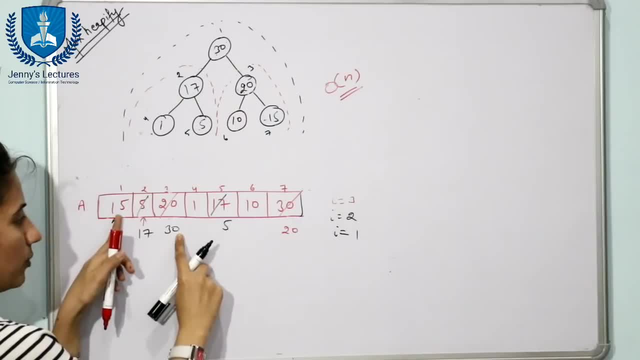 And right, we have 17.. So at 2,, we have 17.. And right, we have 17.. So at 2,, we have 17.. And right, we have 30. Which one is greater? 30. 30 would be exchanged with this one. Here you will. 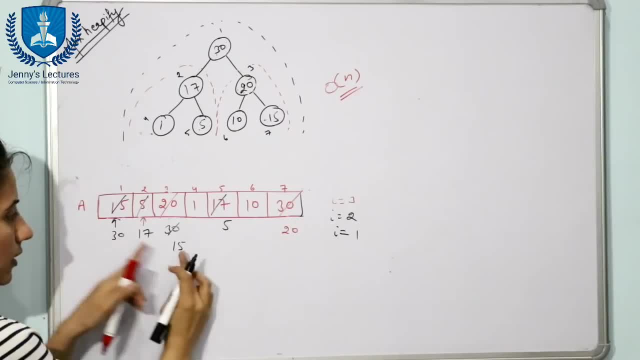 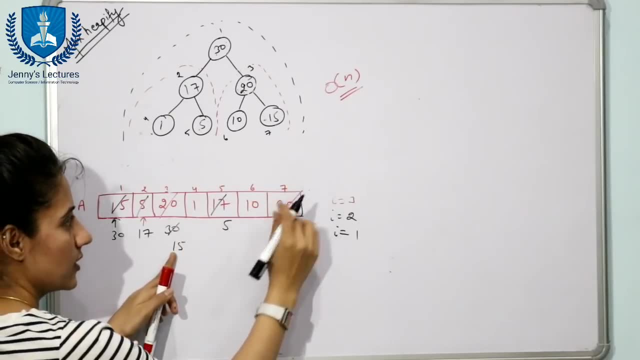 write 15.. And here you will write 30. Then 15.. 15 is at index 3.. Left child of this, 3, is at 6th And right child would be at 7th index. At 6th we have 10.. At 7th we have 20.. Which one is? 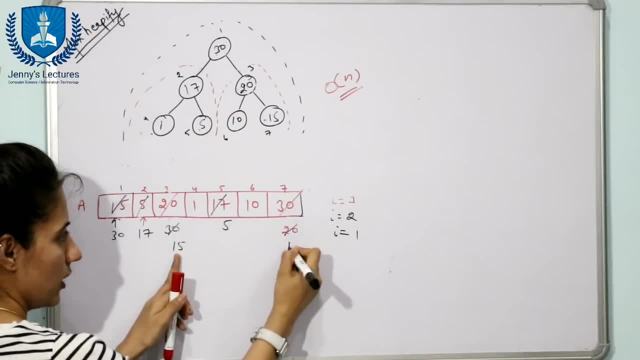 greater 20.. 20 is compared with again this 15.. Now we are going to shift. Here we will write 15.. And here you will write 20.. Right Now, find out: left child of 15.. 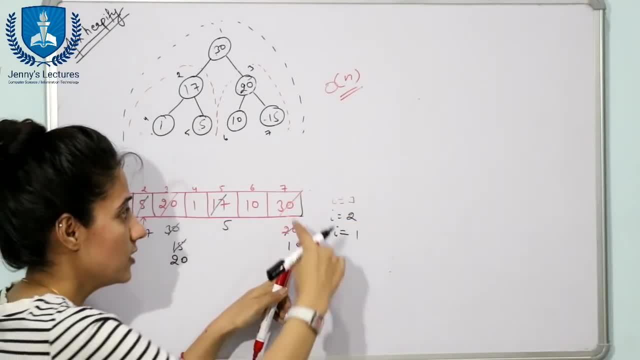 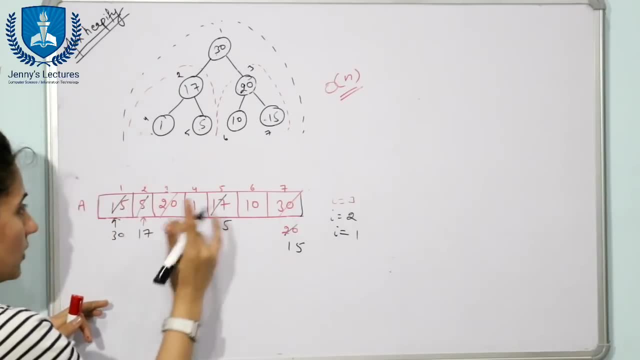 7 into 2, that is 14.. But 14 index is greater than this n, So we are going to stop here. We are not going to apply heapify here. Fine, So after updation the array would be something: 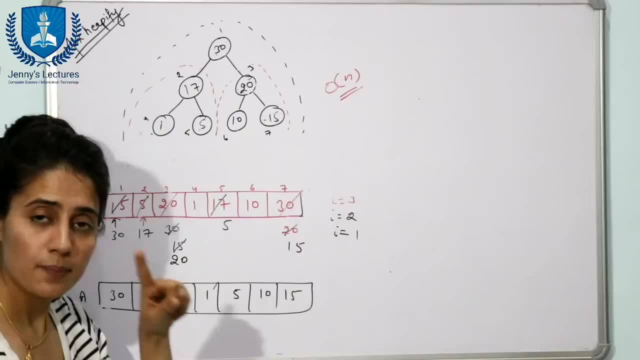 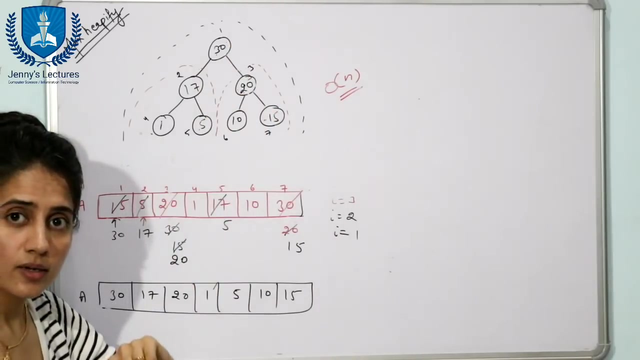 like this: Now, this is max heap. First step is over Using heapify method. we have built max heap. Now the next step in heap sort is: you are going to delete data. Always, the root element would be deleted. Fine, Here also, we are going to delete 30.. We are going to 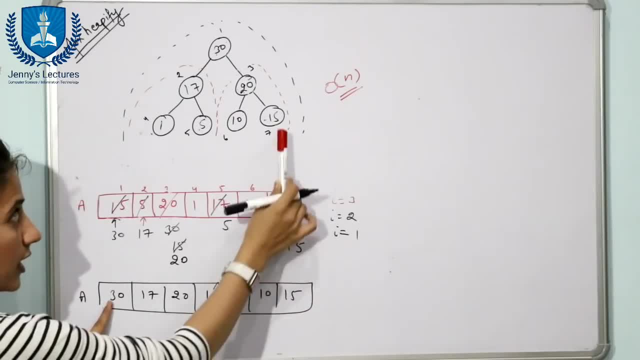 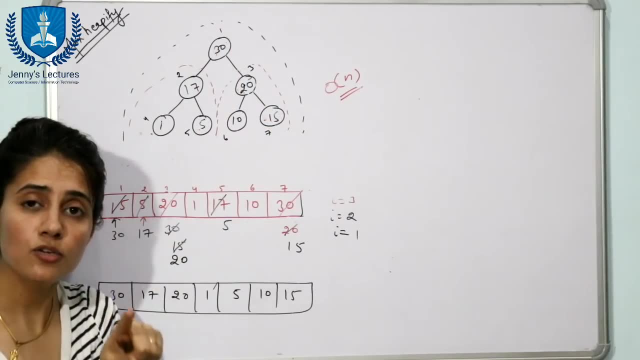 swap this 30 with this 15.. 15 would go here, Because last element in this array is 15.. So 15 would go here. 30 would go here Now, after 15 would go here again. you are going. 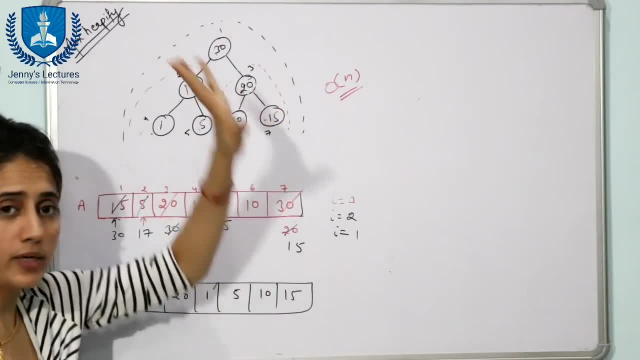 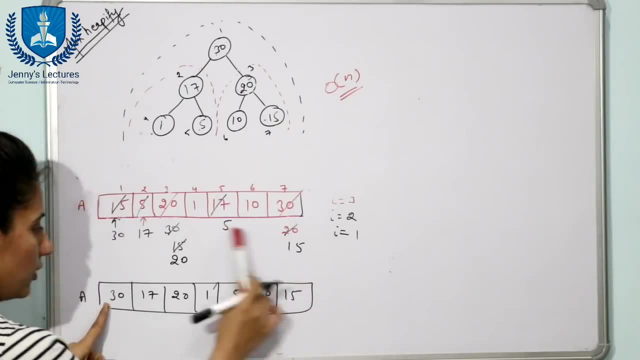 in heap sort is: you are going to delete data, always the root element would be deleted. fine, here also we are going to delete 30. we are going to swap this 30 with this 15. 15 would go here because last element in this array is 15. so 15 would go here, 30 would go here. 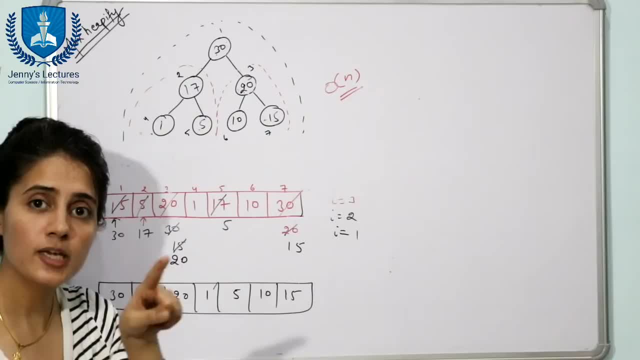 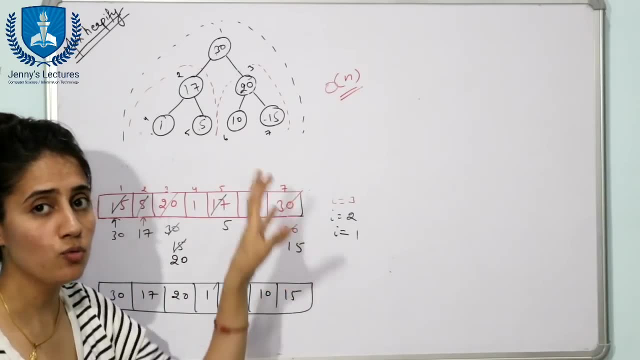 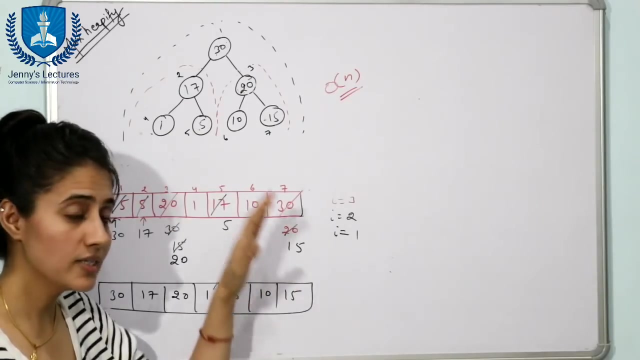 now after 15 would go. here again you are going to apply heapify method because after inserting 15 here, this is not a, this is no more a mix heap and you have to make it mix heap. now again, apply heapify method. now how we are going to write the code for this heapify method. 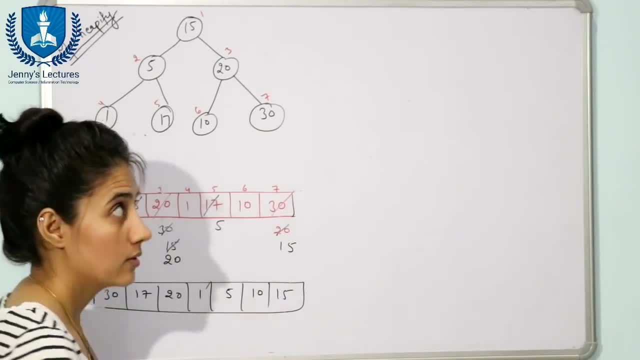 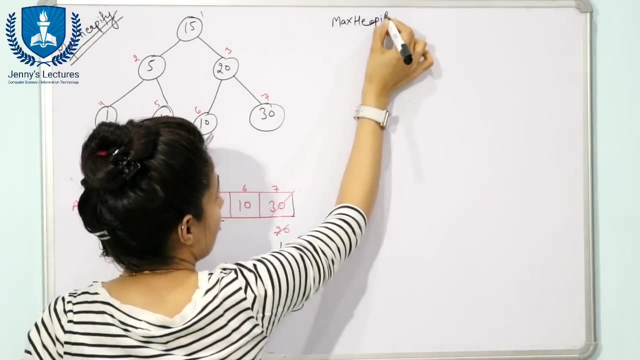 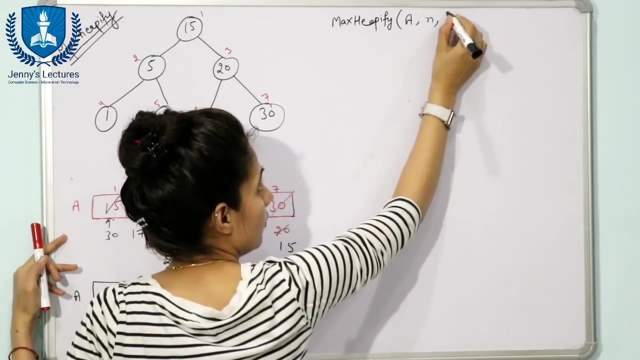 so now i am going to write a piece of code for this heapify method, or you can say, you can say mix heapify method. i am going to take mix heapify method. on the array name is a, n is total number of elements and one variable i am going to take i. 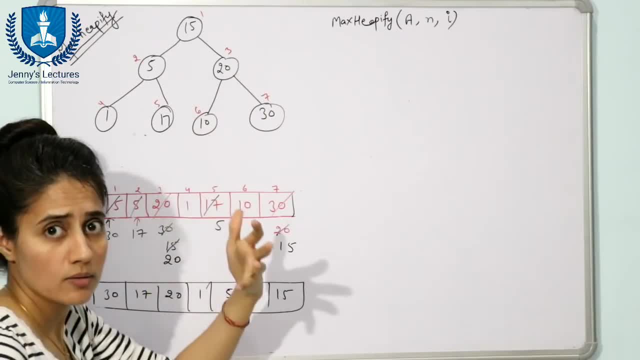 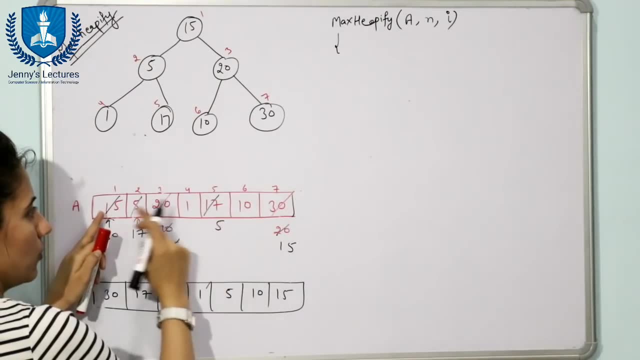 at which, at which index i am going to start? i am going to call the heapify method, fine, so now i am going to take the original tree, now, whatever we have considered at starting. so this is the original tree, fine, so now i am going to take the original tree, now, whatever we have considered at starting. 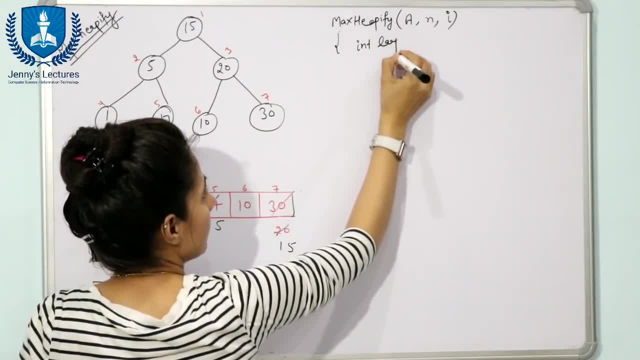 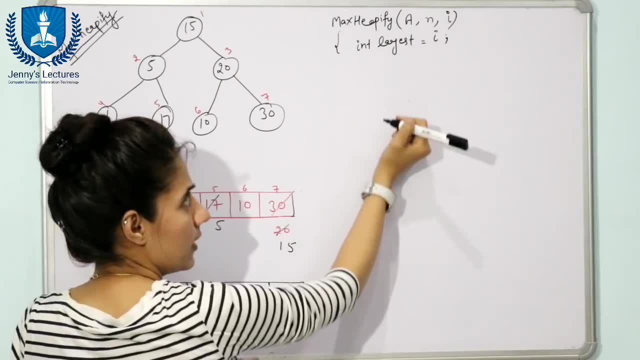 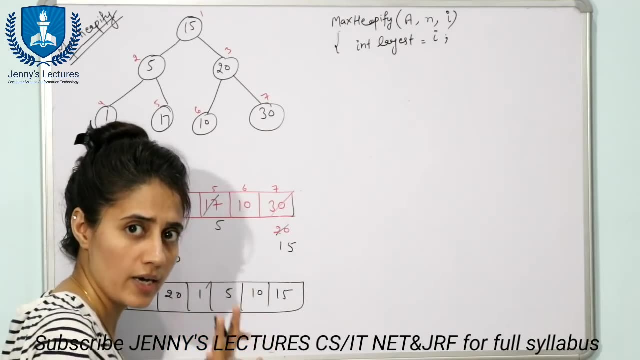 so this is the original tree, fine, so next we are going to take a variable: largest name is largest and i would be assigned to here, fine, and after that i am going to, uh, i am going to calculate the left and right child for that. i okay, suppose. here i value is: 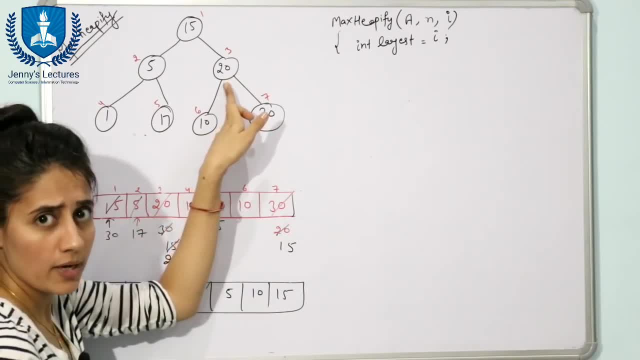 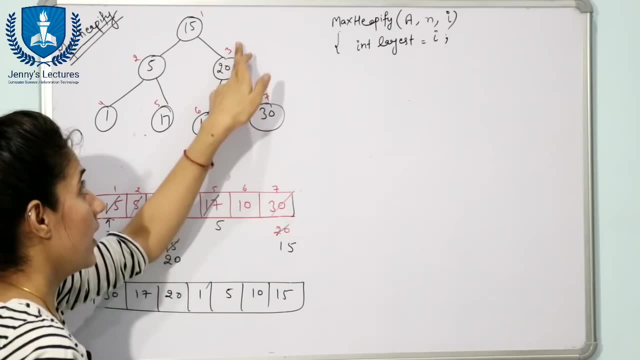 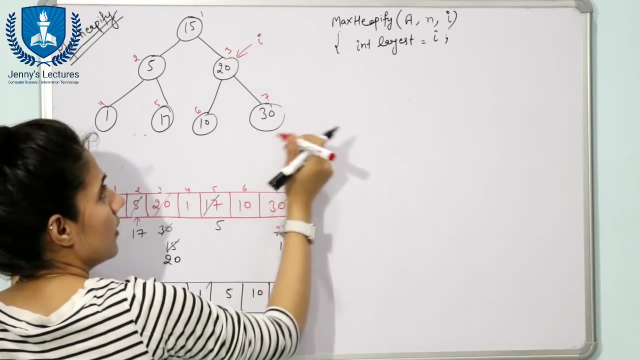 three i am going to see. obviously i am going to call heapify method from here, because these are leaf node. we are going to call the heapify method on non-leaf node and which is at largest split. that's what we are going to do here. s is equal to. let's say we are going to use a. 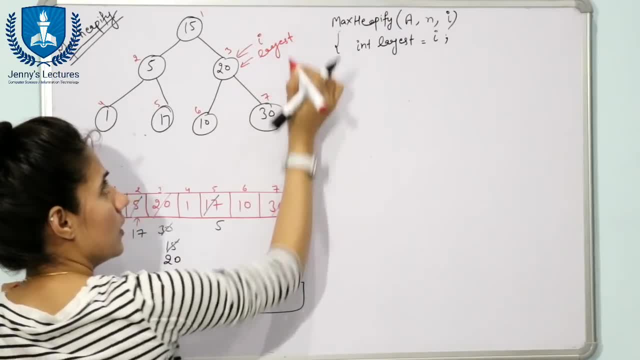 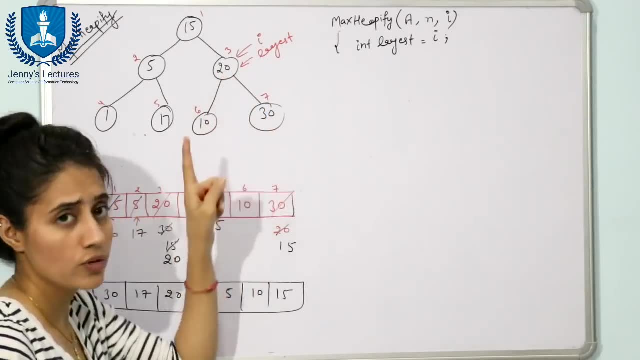 and i. so this is our i and this is the Principality souls. this is our copihat to the i and i is equal to 3. so here i is equal to 3. now it's starting at starting. see, here we have i and i is i value. 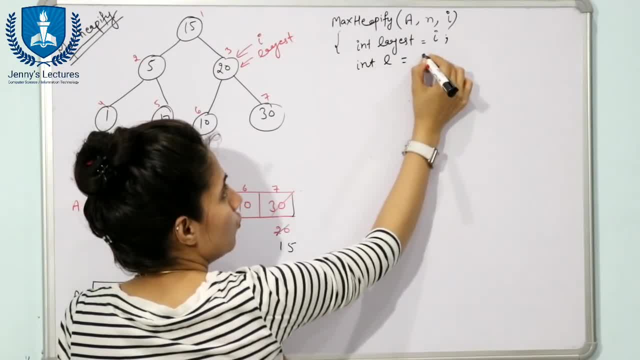 store to the largest. so here only we have largest. i'm going to consider this is the largest now. now next towards, we are going to calculate the left and right child of this twenty. okay, now how to calculate. suppose l is equal to 2, to i will give, we will know that, which is 50%. 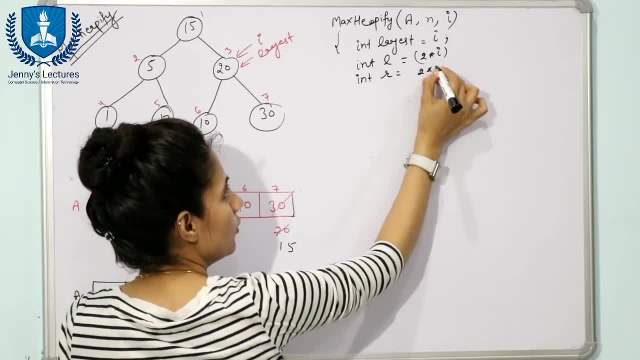 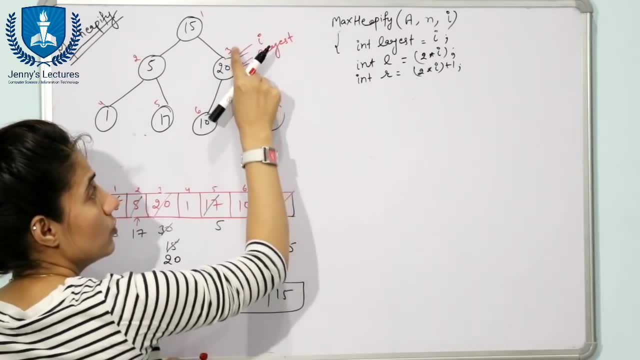 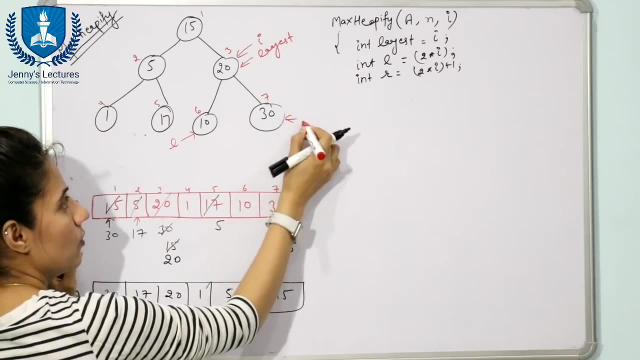 We know the formula. and r is equal to 2 into i plus 1.. 2 into i i value is 3.. So 2 into 3 is 6.. Here we have left and here we have r. now, Fine. 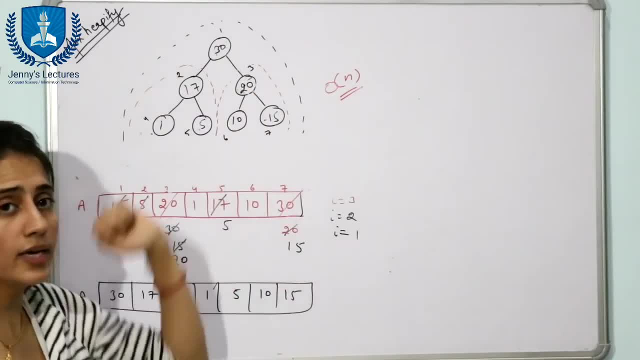 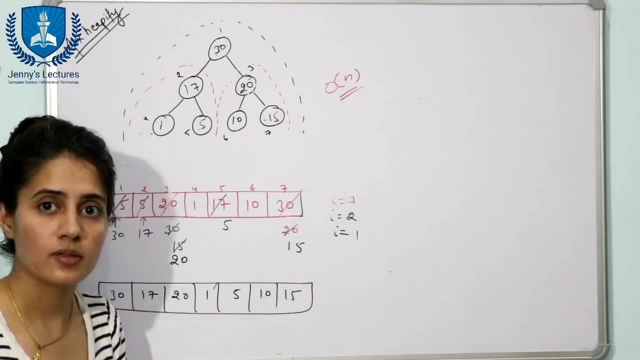 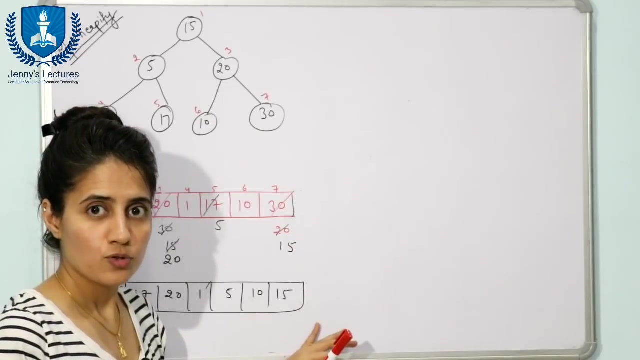 to apply heapify method, Because after inserting 15 here, this is no more a max heap And you have to make it max heap. Now again, apply heapify method. Now how we are going to write the code for this heapify method. So now I am going to write a piece of code for this. 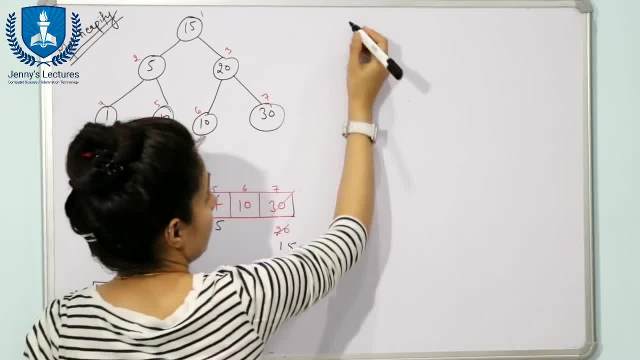 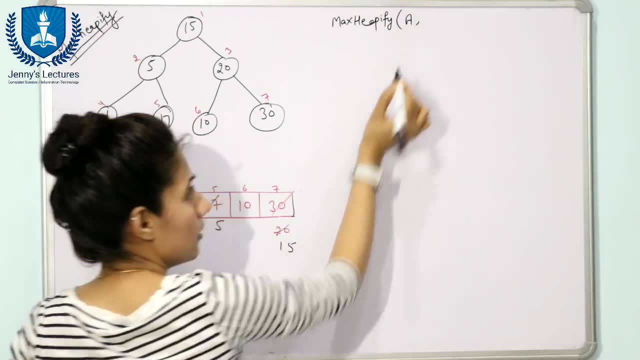 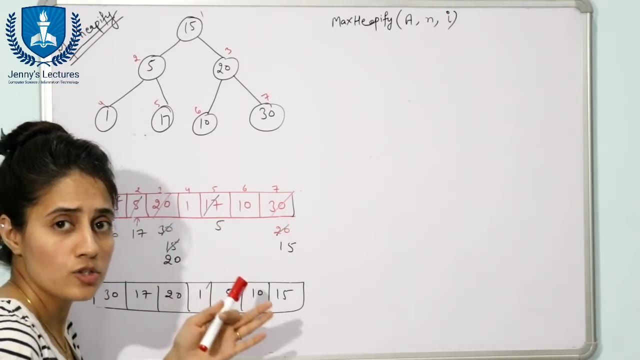 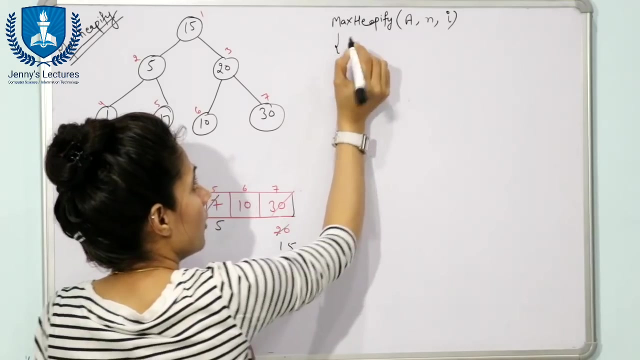 heapify method Or you can say max heapify method. I am going to take max heapify method on the array name is a and its total number of elements and one variable. I am going to take i. at which index I am going to start? I am going to call the heapify method, Fine. So now I am going 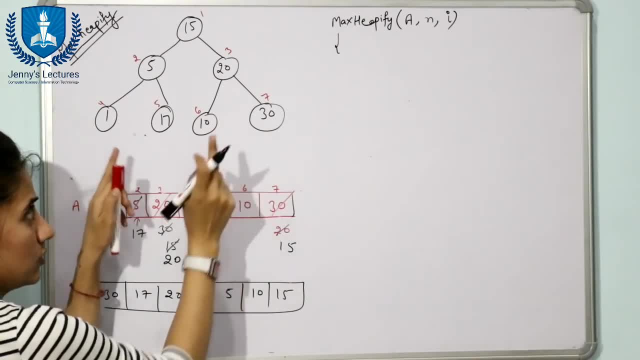 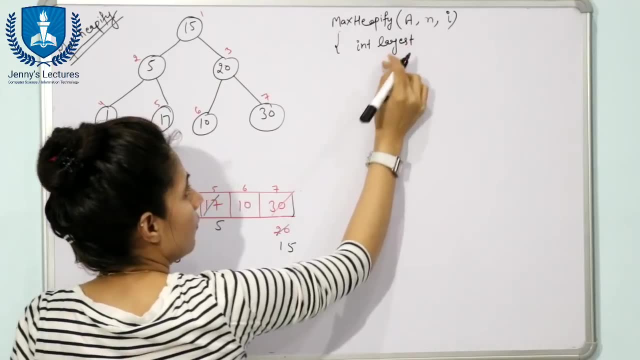 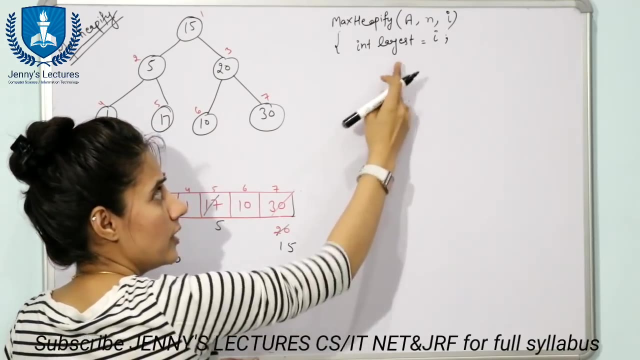 to take the original tree now, Whatever we have considered at starting. So this is the original tree, Fine. So next we are going to take a variable: largest name is largest and i would be assigned to here. Fine, And after that I am going to calculate the left and right child for. 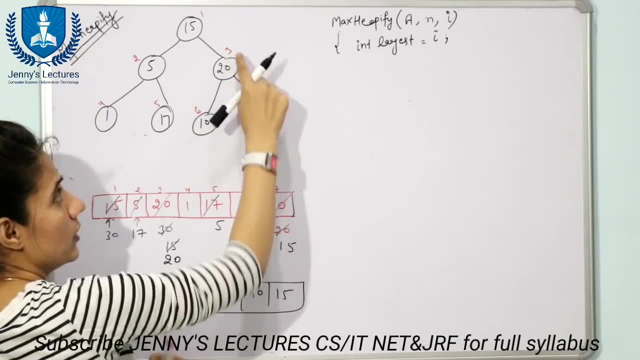 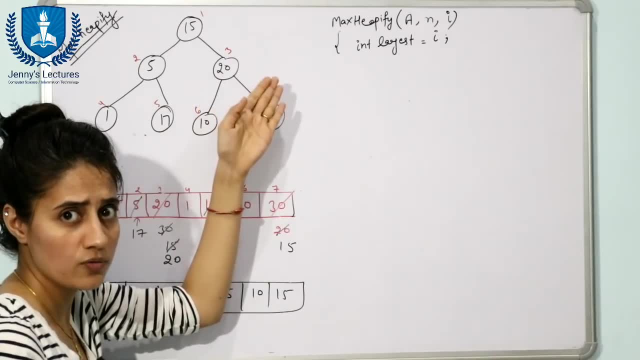 that i Okay Suppose here i value is 3.. I am going to see, Obviously I am going to call heapify method from here, Because these are leaf node. We are going to call the heapify method on non-leaf node and which is at largest. 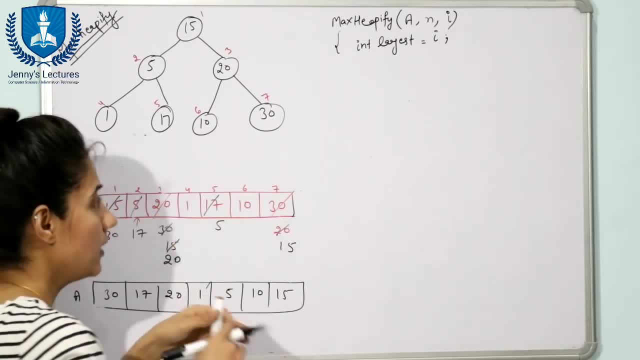 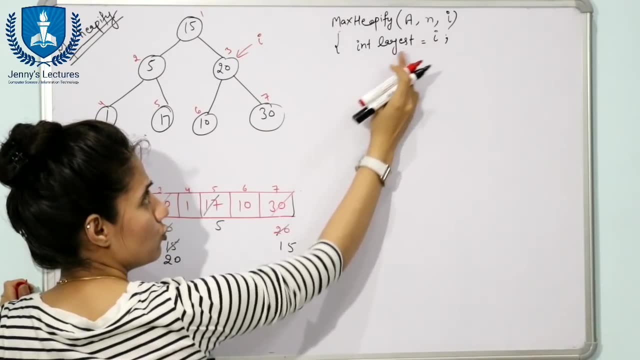 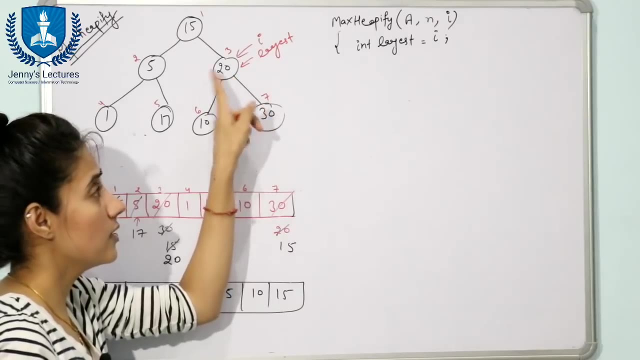 So here i is equal to 3.. Now, at starting, at starting, see here we have i and i is i. value is stored to the largest. So here only we have largest. I am going to consider this is the largest now. Now, next was we are going to calculate the left and right. 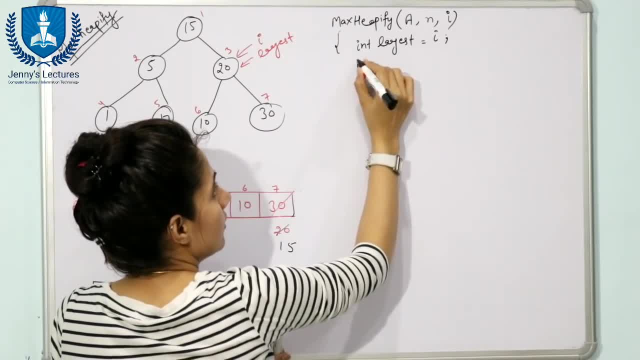 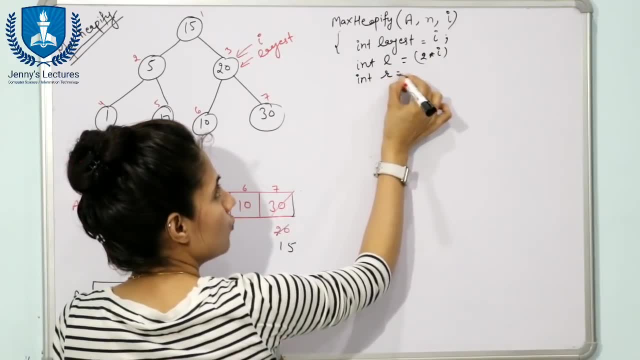 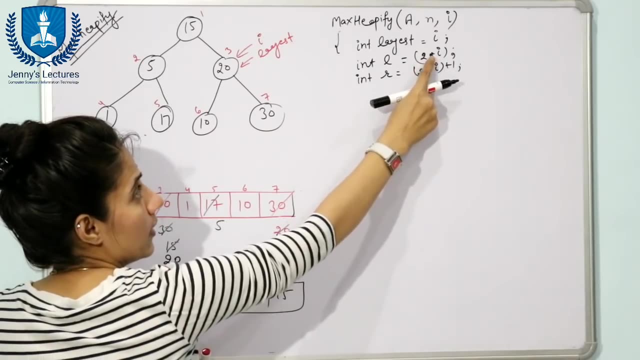 child of this 20.. Okay, Now how to calculate. Suppose l is equal to 2 into i is equal to i. We know the formula. and r is equal to 2 into i plus 1.. 2 into i, i value is 3.. So 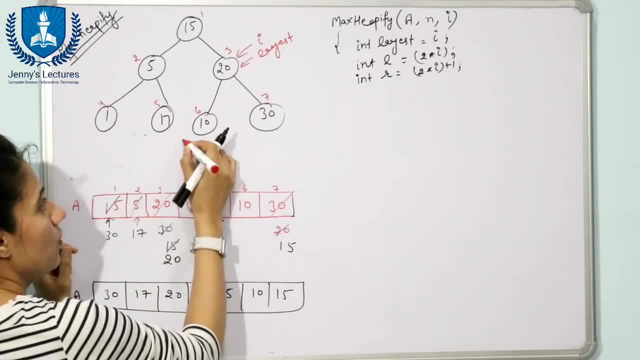 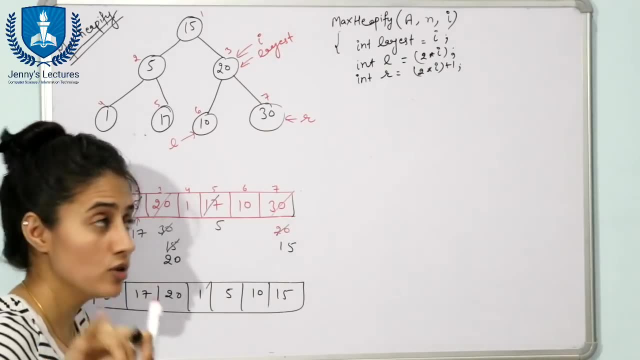 2 into 3 is 6.. Here we have, here we have left, and here we have r now, Fine. Now next step was: you are going to compare this with this left and right also. Now you are going to write a while loop. 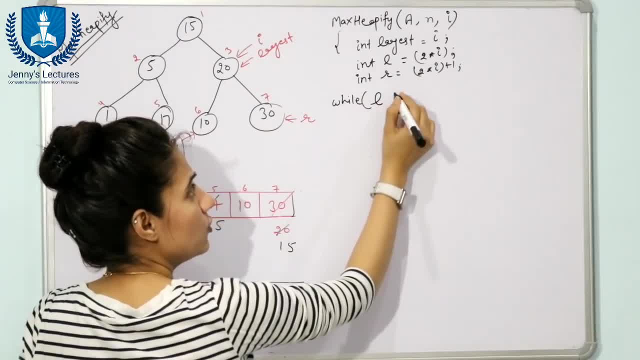 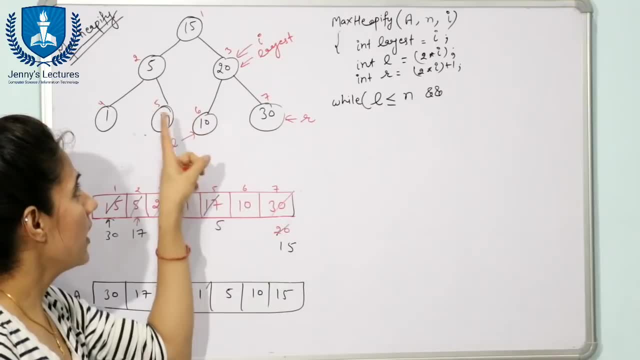 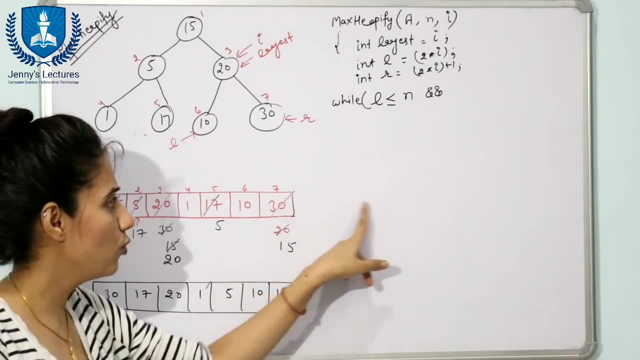 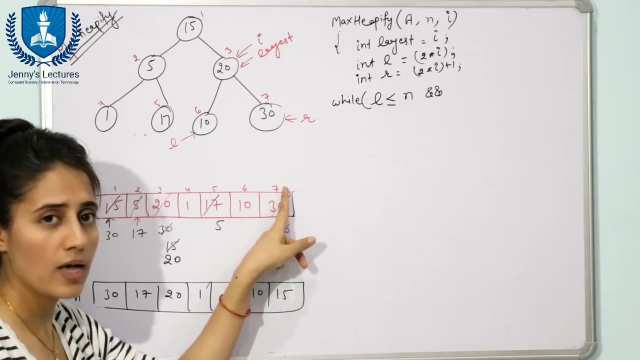 While, while first we will check, left should be less than or equal to n. Now suppose somewhere i is equal to 5. And so left child would be 2 into i. that is at 10th index, and here we do not have any 10th index. So this left and right, both child would be up to this last. 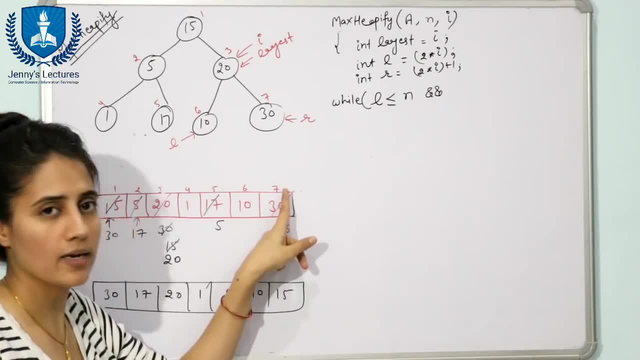 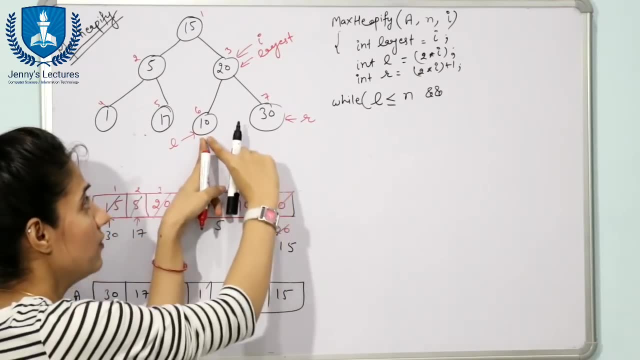 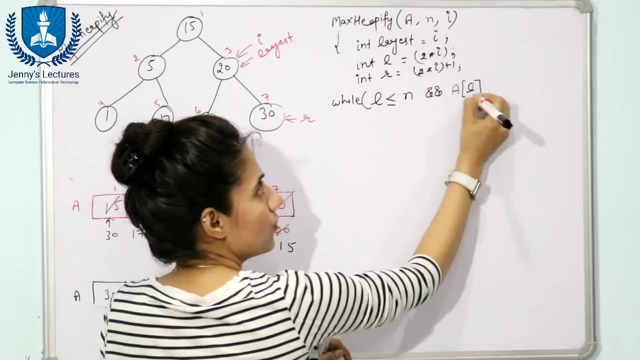 index, So it should be less than equal to this n n is here 7.. So one condition would be checked and, and we will check what is: is this left child greater than its parent? So here we will check: name of array: is a A of this left is greater than. 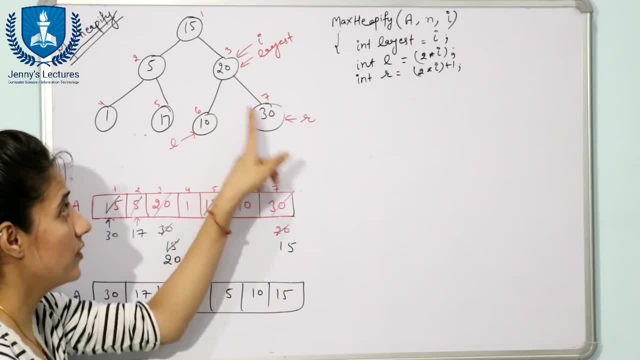 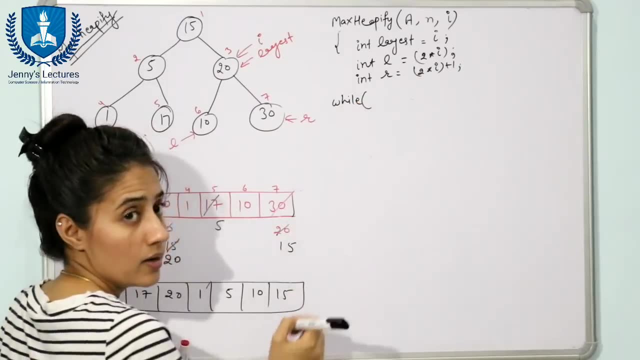 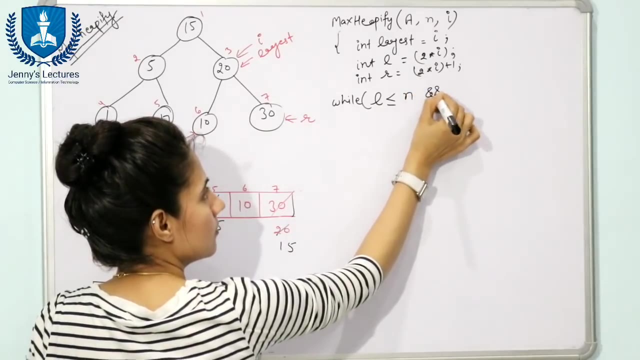 Now next step was: you are going to compare this with this left and right also. Now you are going to write a while loop, While first we will check. left should be less than or equal to n. Now suppose somewhere i is equal to 5.. 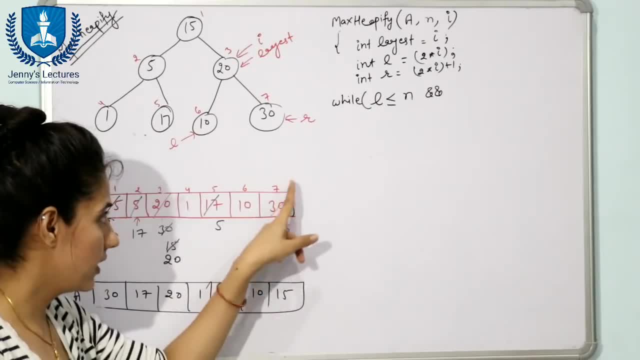 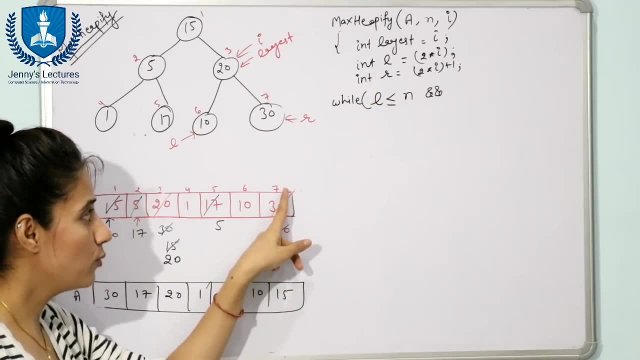 And so left child would be 2 into i. that is at 10th index And here we don't have any 10th index. So this left and right both child would be up to this last index. So it should be less than equal to this n. 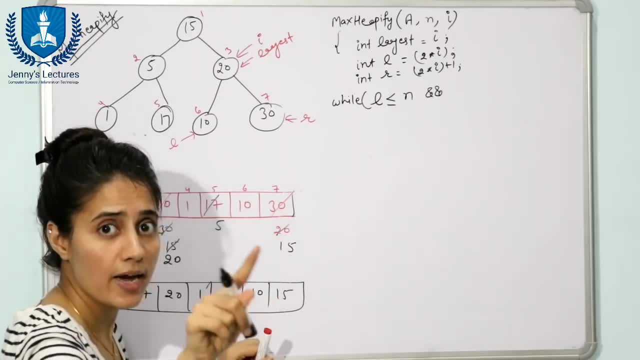 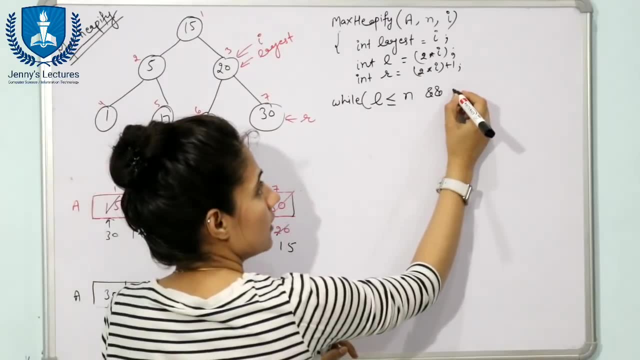 n is here 7.. So this is left and right. So this is left and right. So one condition would be checked And we will check what Is this left? child greater than its parent. So here we will check. Name of array is a. 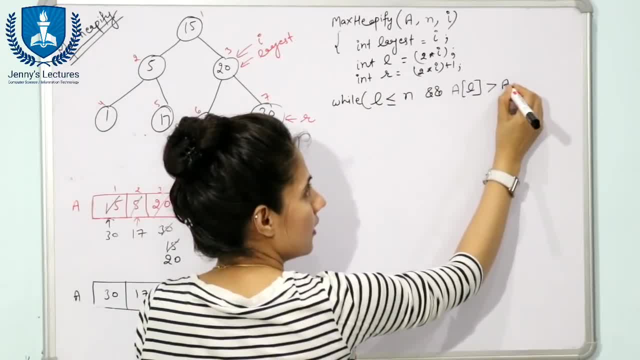 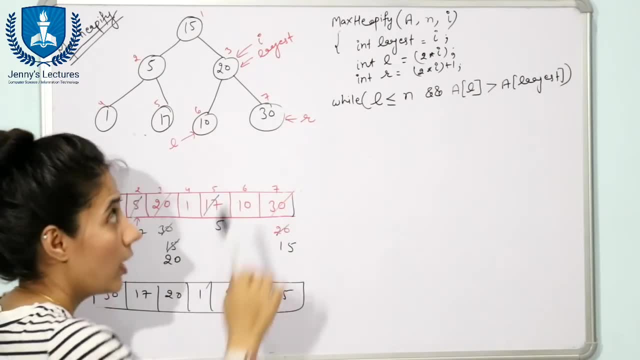 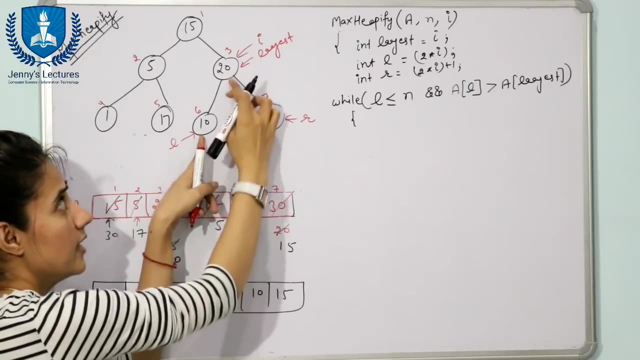 a of this left is greater than a of largest, Because largest is 20. now i and largest both are pointing 20.. Fine, If this is true, If this l is greater than this, This one, Because this is parent na. 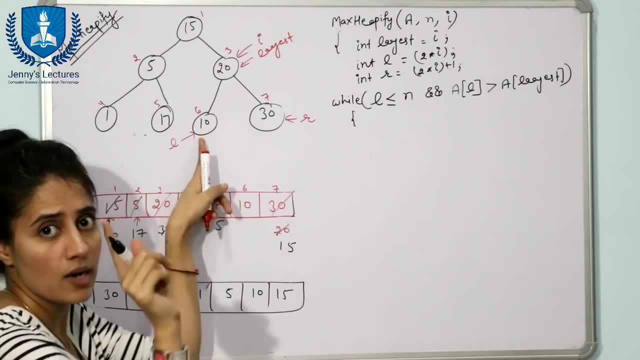 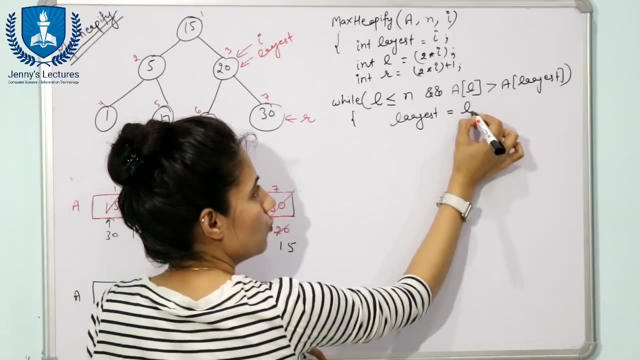 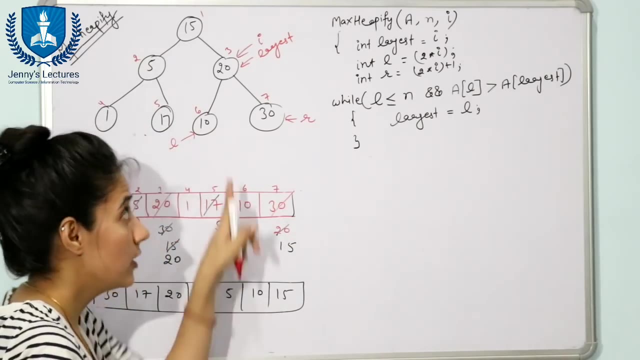 So now you will do what. You will consider this: This is the largest, So we do what? So we do what. Now, largest is equal to l. Fine, So this is done. Next you will check. This is only for left. 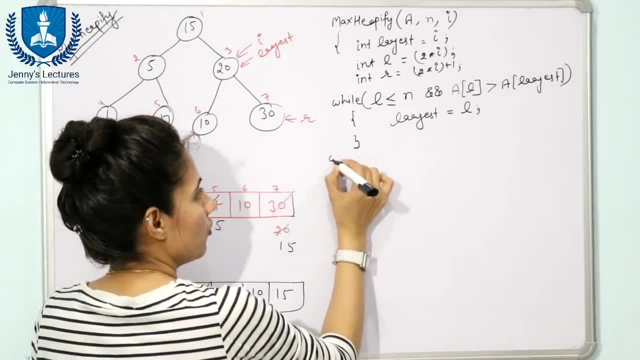 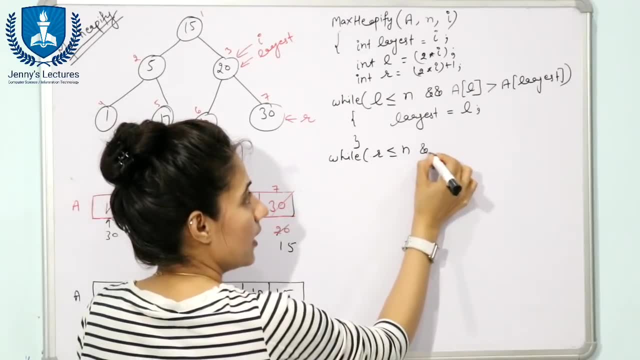 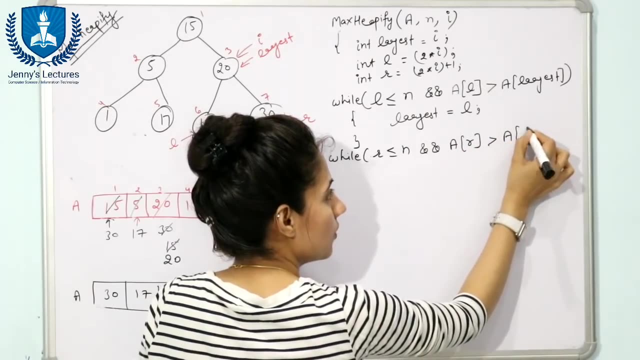 Next, also, we will check for right na. So again, same while loop would be applied, While Same condition. R should be less than And equal to this n size of this heap And we will check a of r. a of r is greater than a of largest. 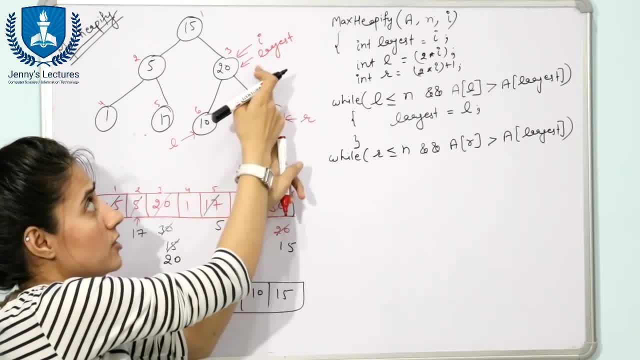 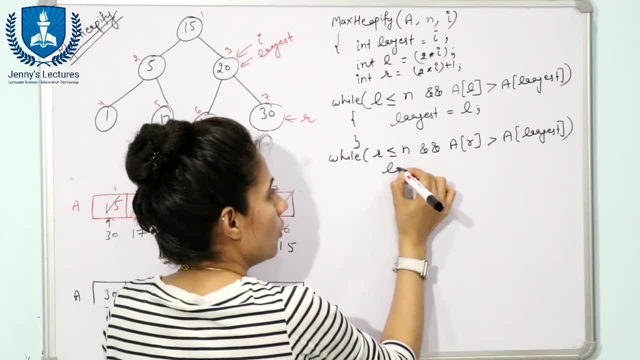 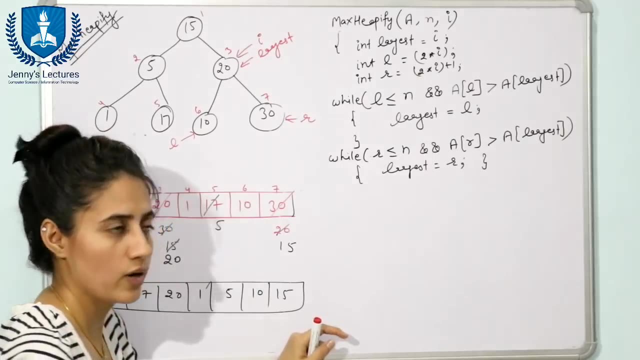 If a of r, this right child, is greater than this one, Because largest is at starting at this place. So we will consider what. This is the largest element, So we will do what Largest is equal to r. So this is the closing of this while loop. 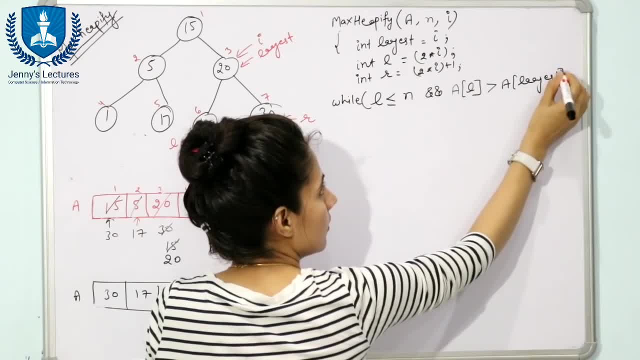 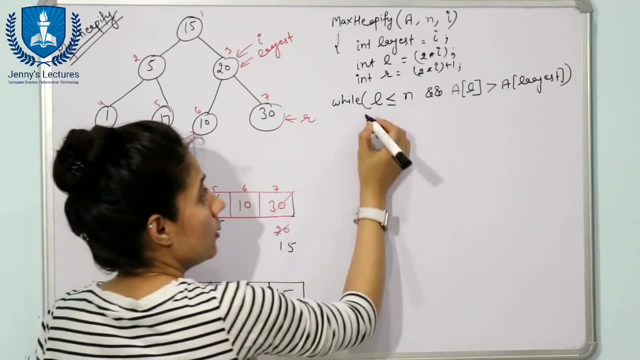 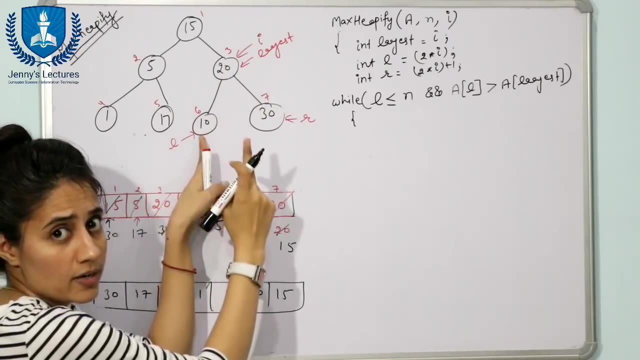 a of largest, because largest is 20. now, i and largest, both are pointing 20.. Fine, If this is true, If this l is greater than this, This one, because this is parent now. So now you will do what, You will consider this. 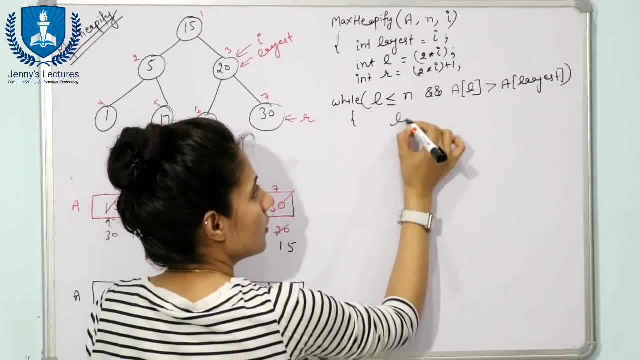 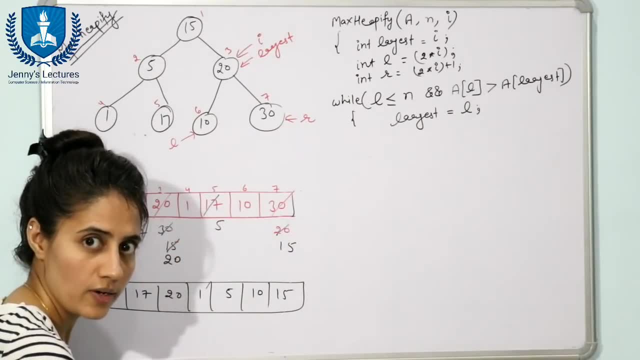 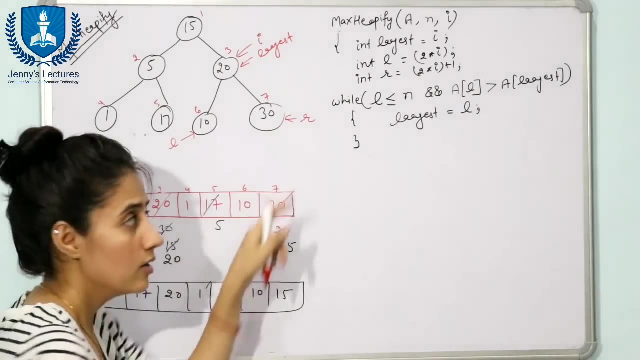 This is the largest, So we we do what, So we do what. Now, largest is equal to l. Fine, So this is done. Next, you will check. this is only for left. Next also, we will check for right now. So again, same while loop would be applied, while same condition- r should be. 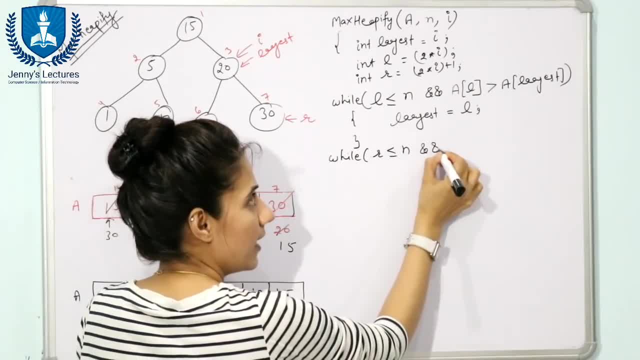 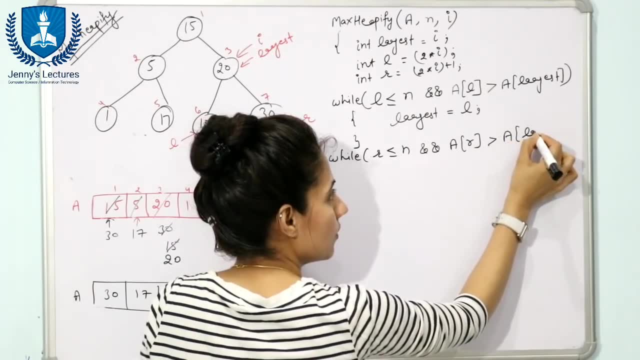 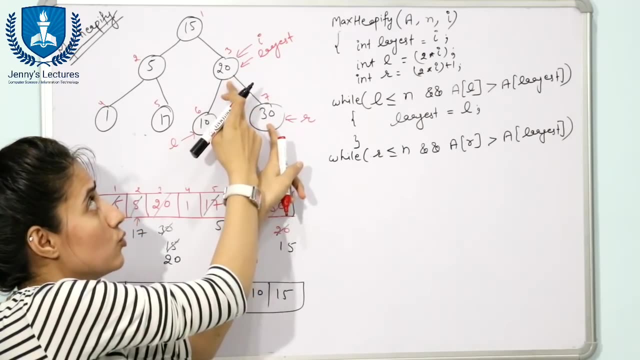 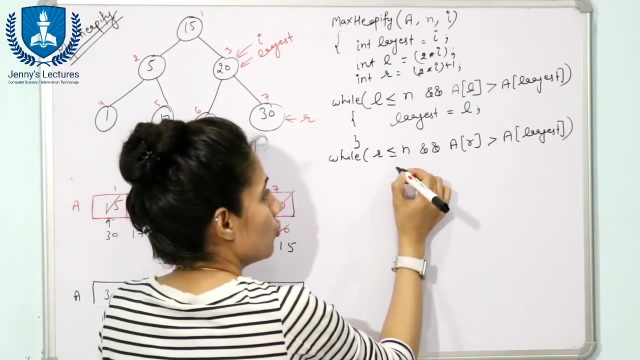 less than equal to this n size of this heap and we will check a of r. a of r is greater than a of largest If a of r, this right child, is greater than this one, because largest is at starting at this place. So we will consider what this is the largest element, So we will. 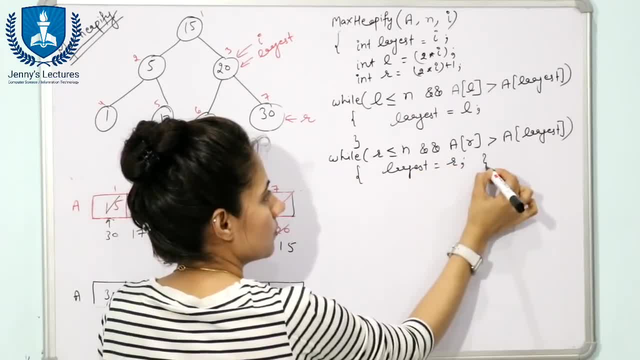 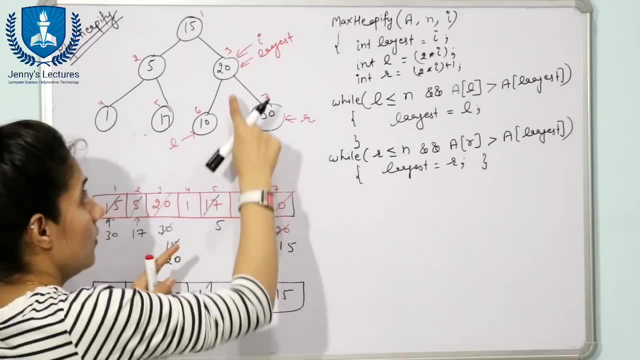 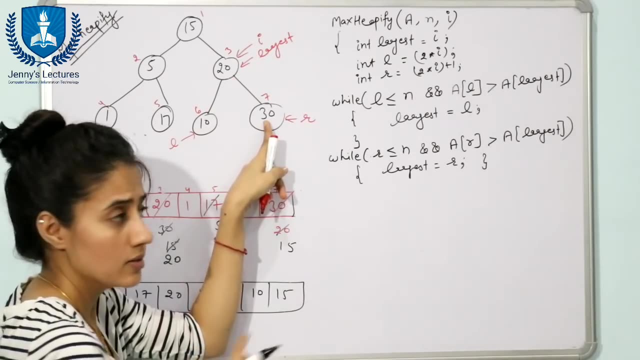 do what Largest is equal to r 18.85.. 38.25.. so this is the closing of this while loop. fine, and now, if suppose, like in this case, 10 is not largest, so this condition is not true, but 30 is greater than this 20. yes, both the 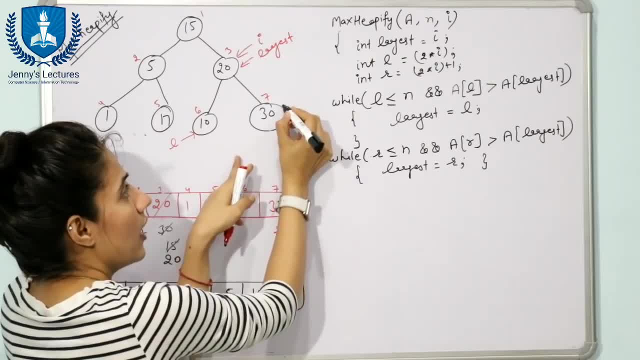 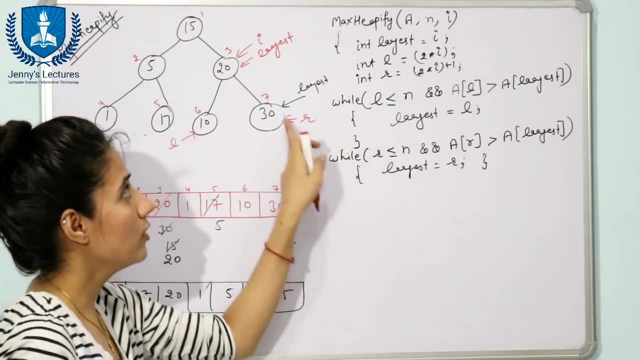 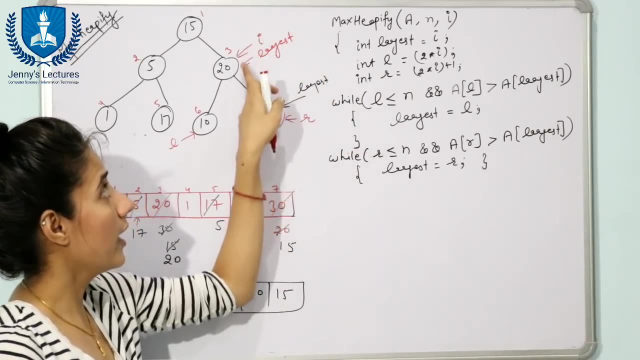 conditions are true. so now, in this case, the largest, this largest would be shifted to here, because our, our value is here. what 7? we have calculated here, 7. so now in largest, largest. first of all, I was there, I value was there, but now our value 7, 7 is in the variable, that is. 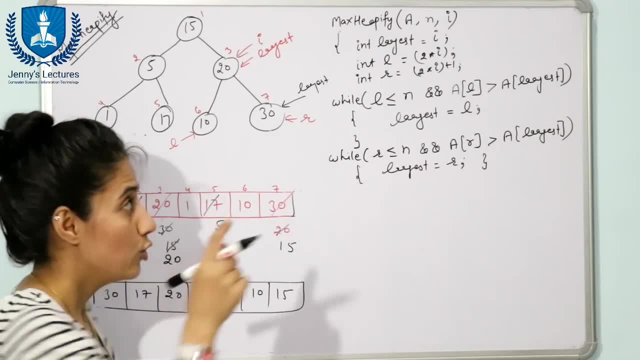 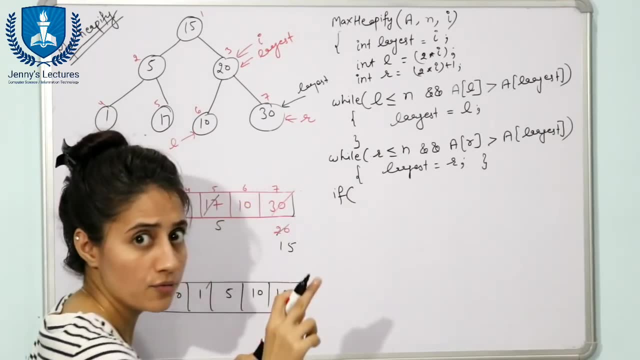 largest, so now here is the largest. so next step is what? we are going to swap: 30 bits with 20 right. so now we are going to check if, if first of all I, the largest element was same, so now we are going to check if, if first of all I, the largest element was same, so now 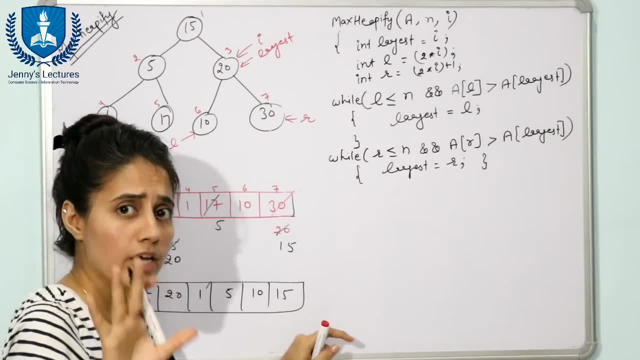 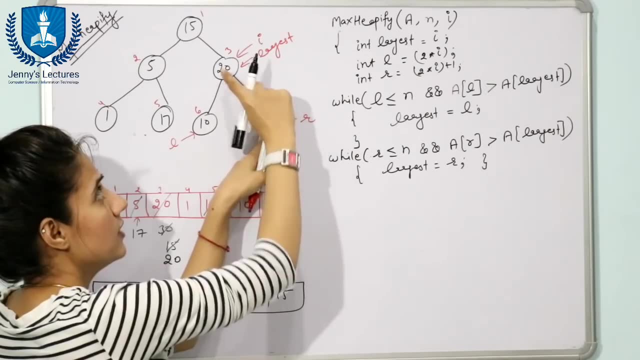 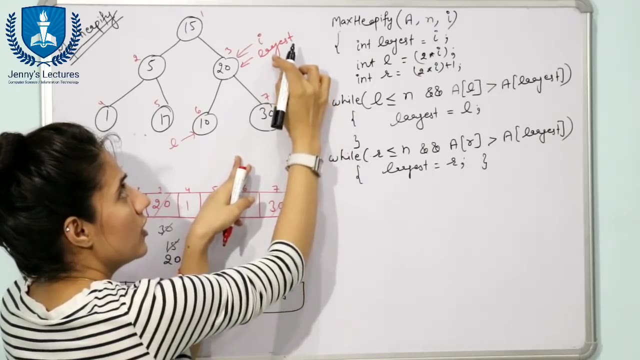 Fine, And now if suppose, like in this case, 10 is not largest, So this condition is not true, But 30 is greater than this 20.. Yes, both the conditions are true. So now, in this case, The largest, This largest, would be shifted to here. 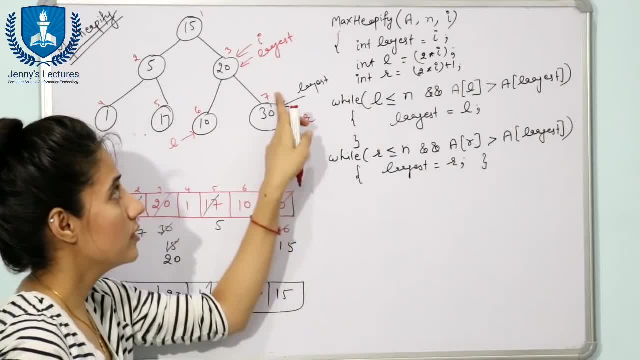 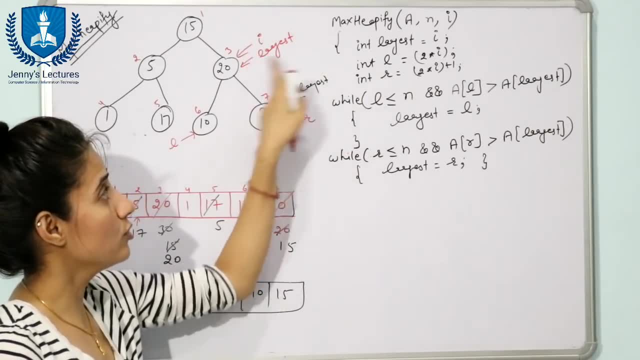 Because r, R value is here, what 7.. We have calculated here 7.. So now in largest, Largest. first of all, i was there, i value was there, But now r value 7. 7 is in the variable that is largest. 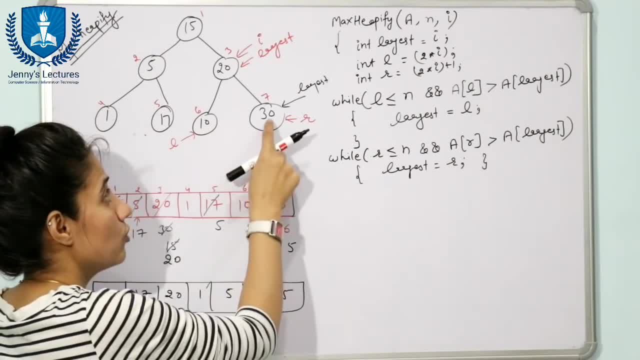 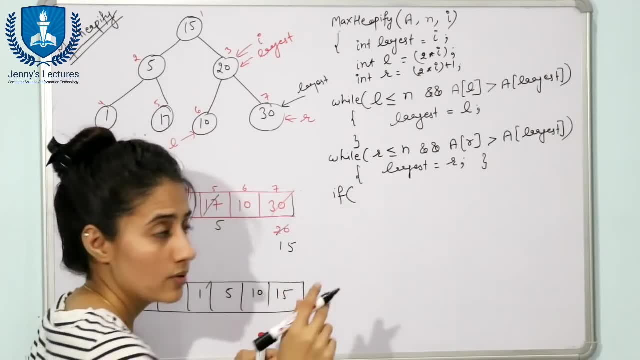 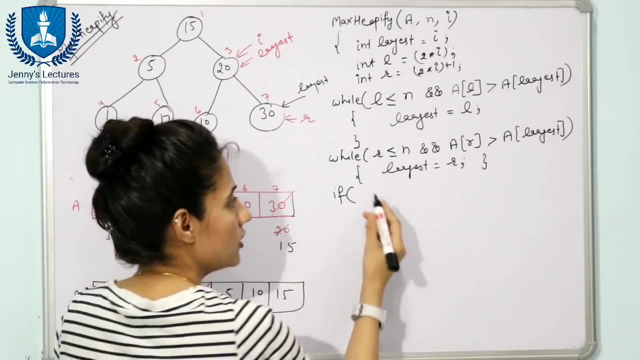 So now, here is the largest. So next step is what? We are going to swap 30 with 20.. Right, So now we are going to check If First of all i, The largest element was same as i, But now largest has been updated. 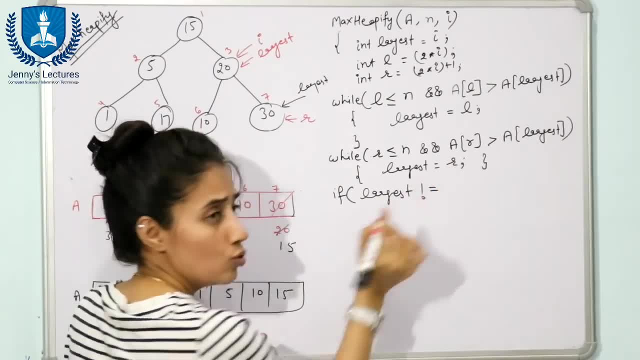 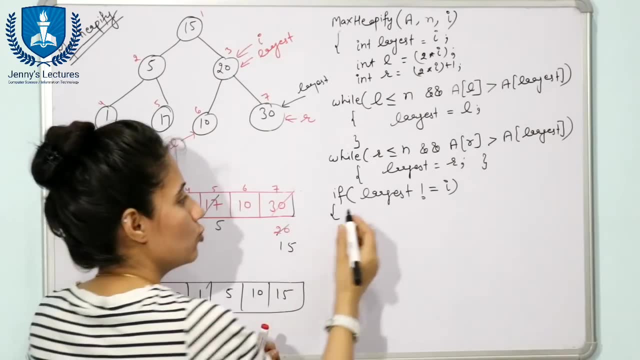 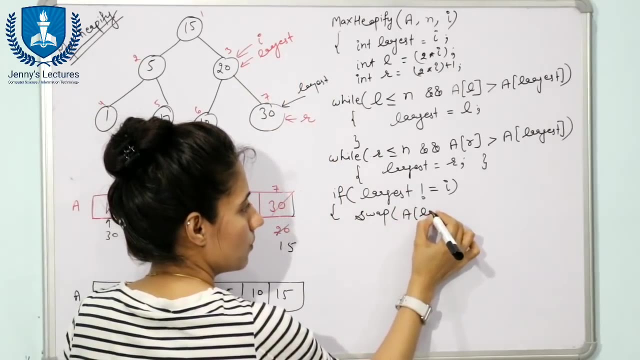 So now we will check. if Largest is not Equal to i, It means It has been updated. So now we are going to swap. So now we are going to swap What this with this? So you can say a of. 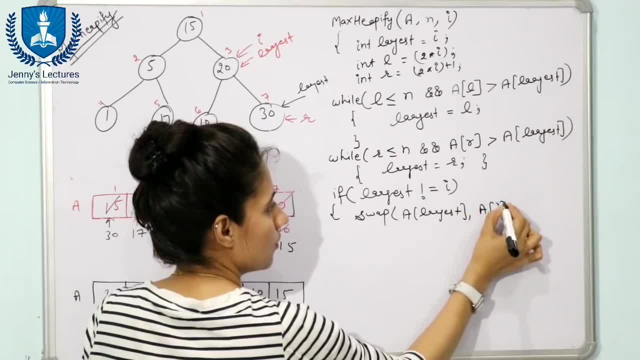 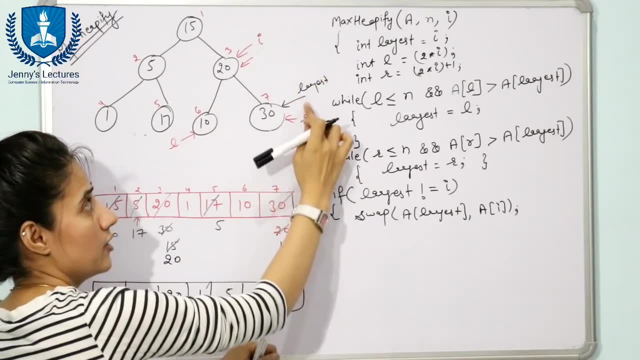 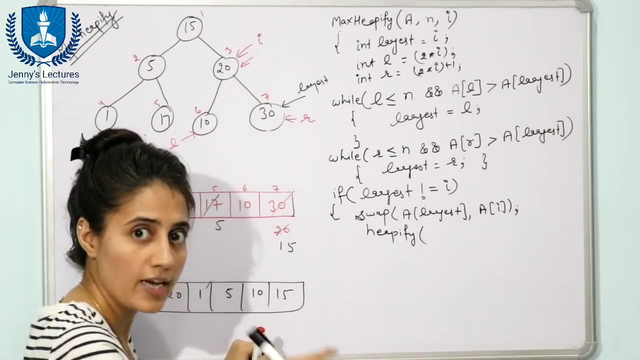 Largest And a of. i Right This with this one. This largest has been updated in this case, now And again. Here only, you are going to call Again hippify method, Hippify on array a, N, And here you are going to pass. 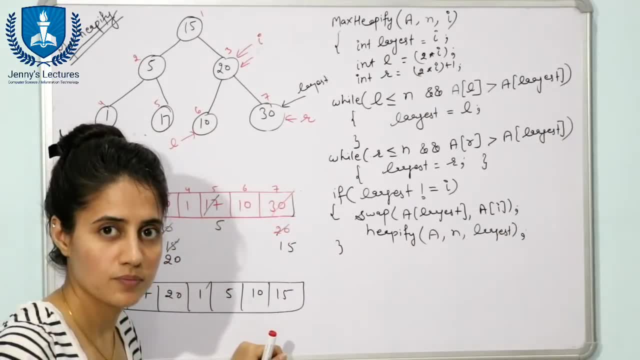 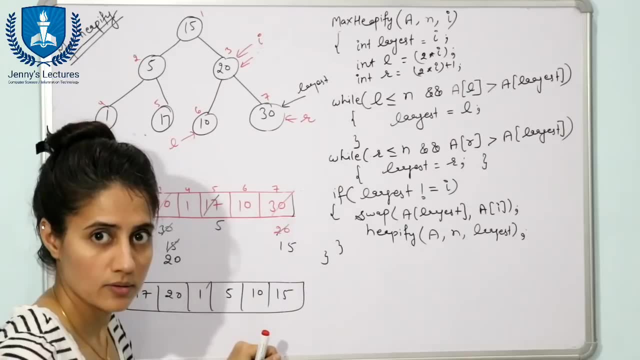 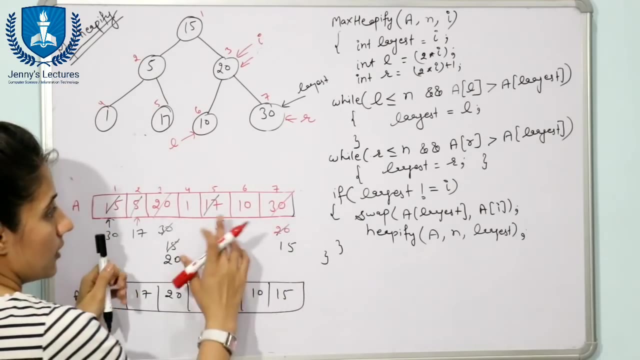 The value of this Largest variable. Fine, This is closed now, And here you can close this Hippify method. See now, here again we have called this hippify method, So this we will discuss with the help of one Example. 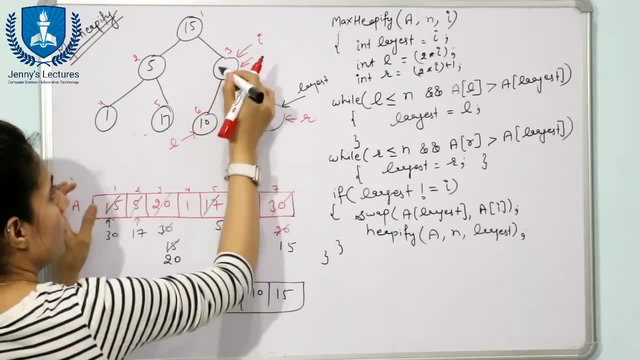 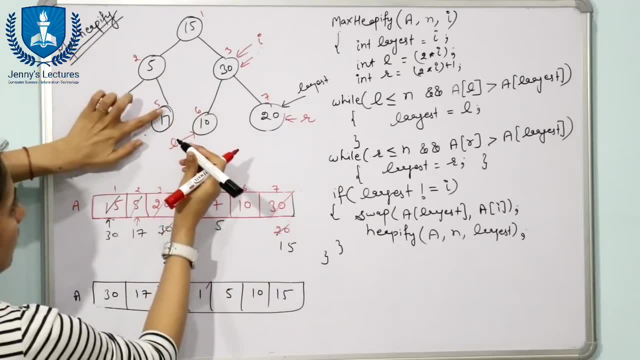 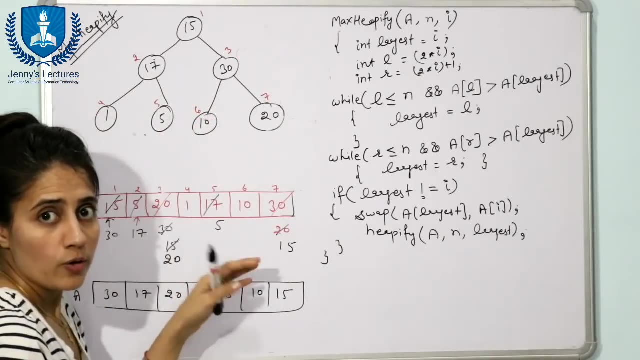 See, after this swapping this, Now, this array is what? 30 and here we have 20.. Fine, At this place, now it is called: Now 17 would go up And 5 would go Here. So now we are going to take a case. 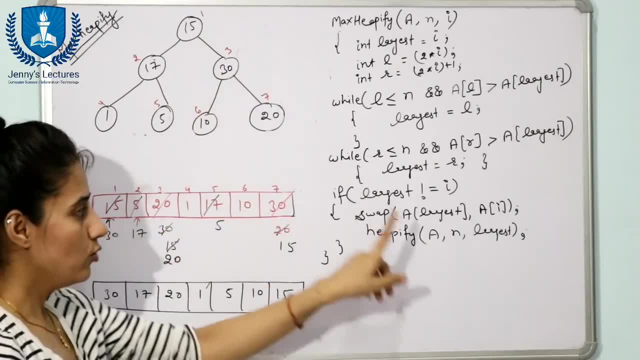 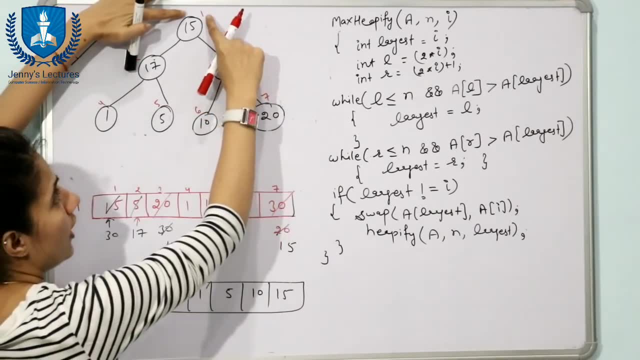 When hippify method is called here, only When i value is 1. Then you will come to know the value of this hippify Regressive call, of this hippify Fine. See here, suppose i value is 1.. N is we have 7.. 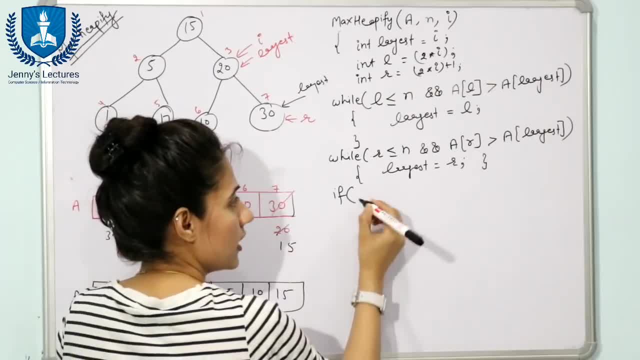 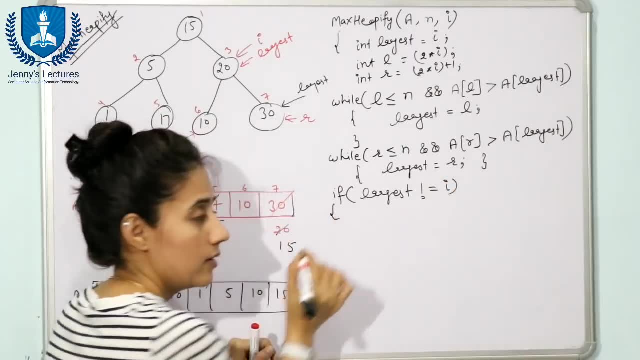 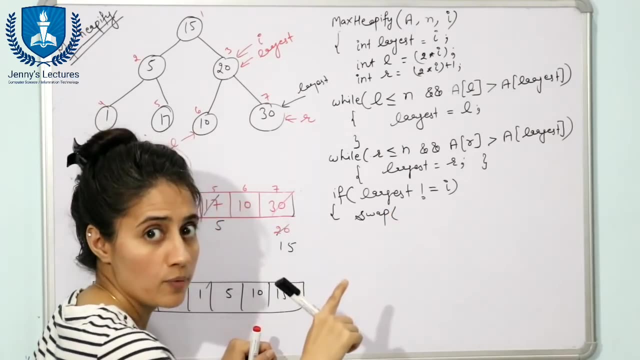 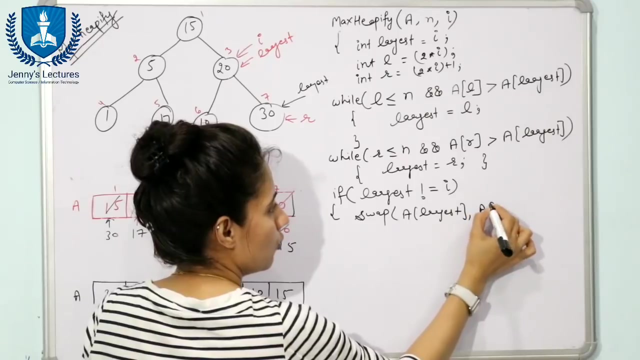 same as I, but now largest has been updated. so now you will check. if largest is not equal to I, it means it has been updated. okay, so now we are going to swap. so now we are going to swap what? this with this, so you can say a of largest and a of. I right this with this. 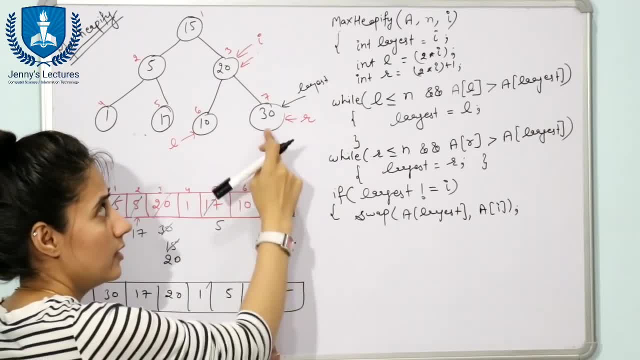 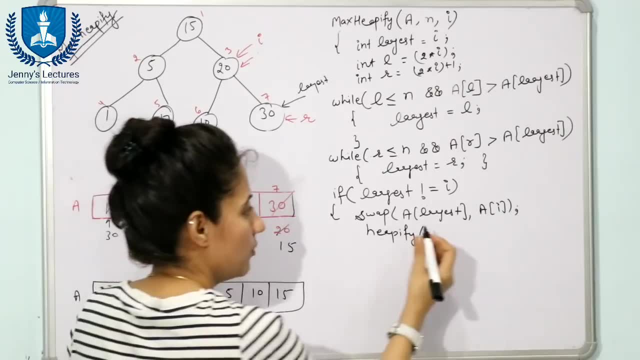 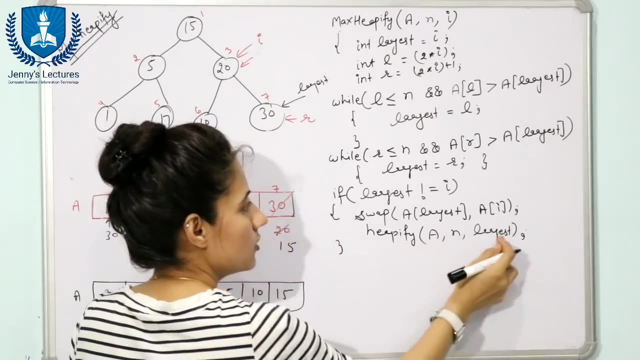 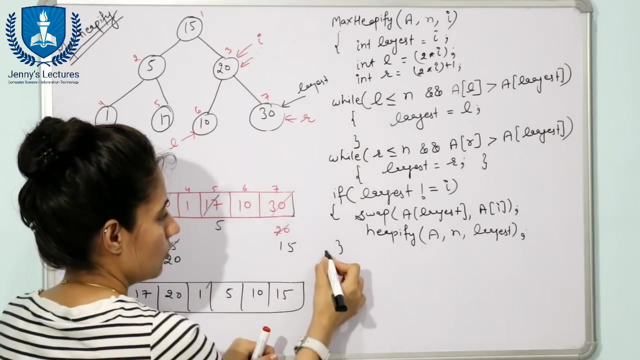 one, this largest, has been updated in this case now and again. here only you are going to call recursively. you are going to call again epify method, epify on array a, n, and here you are going to pass the value of this largest variable. fine, this is closed now and here you can close this. 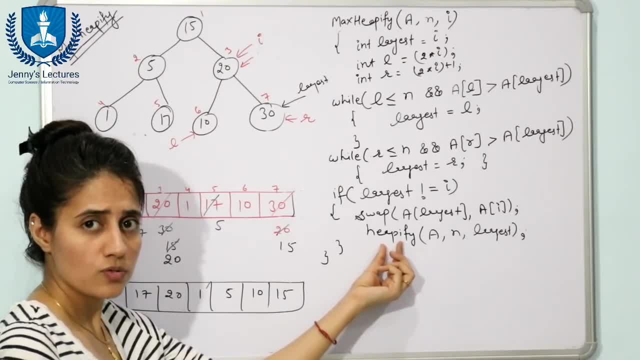 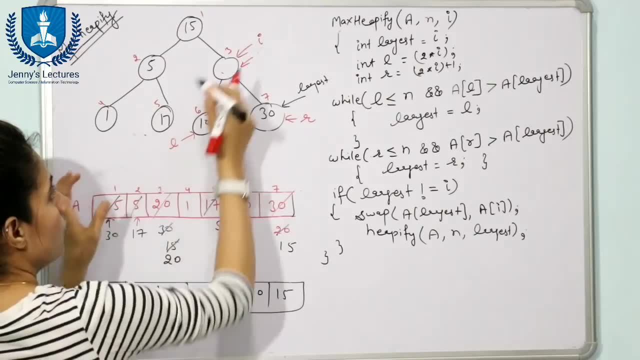 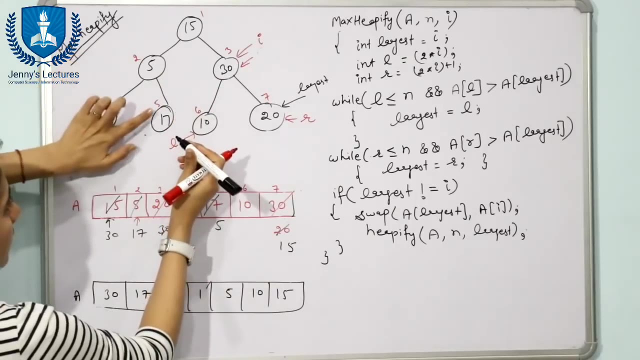 epify method. see now. here again, we have called this epify method, so this we will discuss with the help of one example. see after this. swapping this now. this array is what? here we have 30 and here we have 20.. fine, at this place, now it is called, now 17 would go. 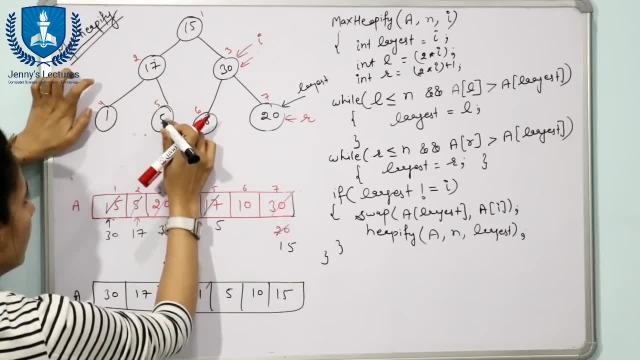 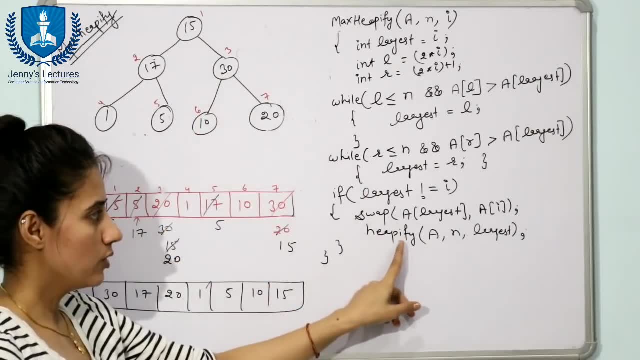 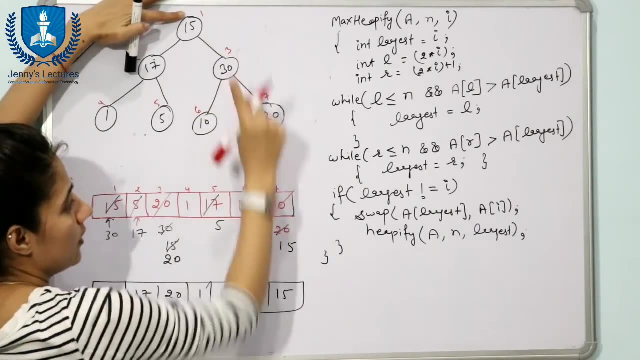 up and five would go here. so now we are going to take a case when epify method is called here, only when I value is one, then you will come to know the value of this epify recursive call of the epify. fine, see, here. suppose I value is one, n is we have seven arrays, this a. okay, now we have I value. 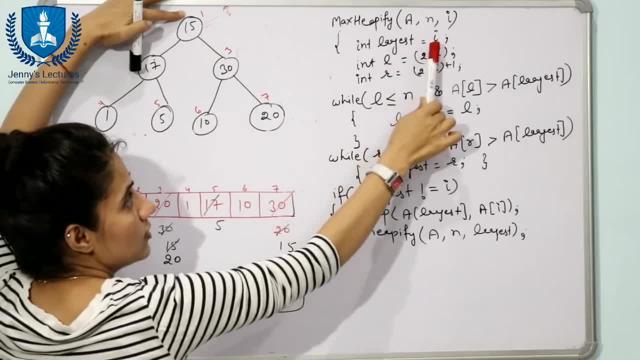 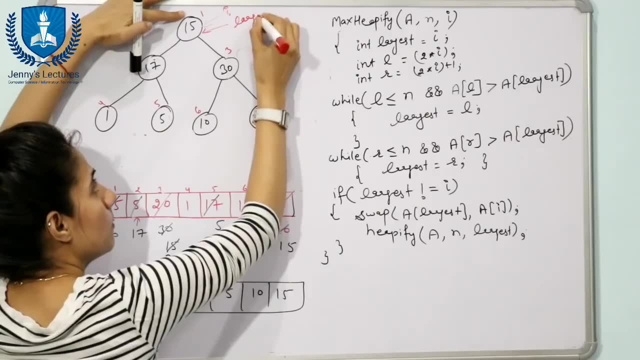 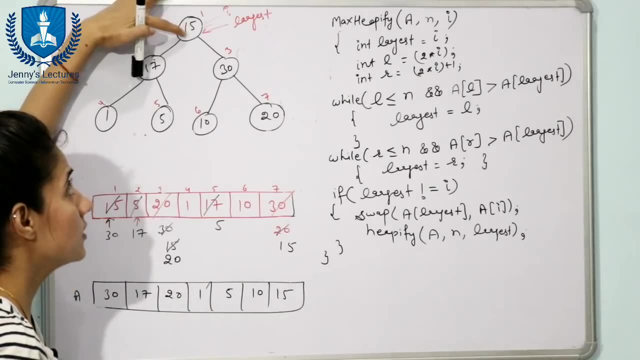 here, only here, we have I largest. I is equal to this. largest is equal to I means I value would be stored to largest only. so here also we have largest. okay, both I and largest is now same. at starting. we are considering this is the largest element. now next step is cons: find out. 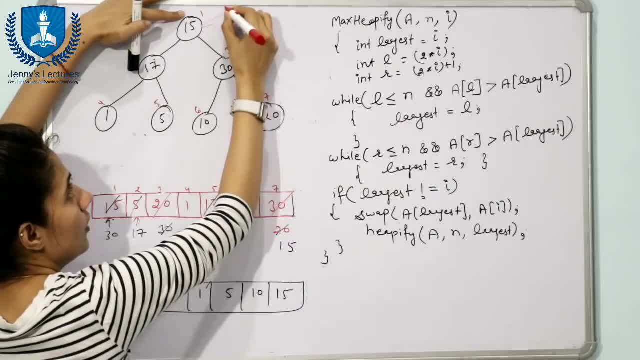 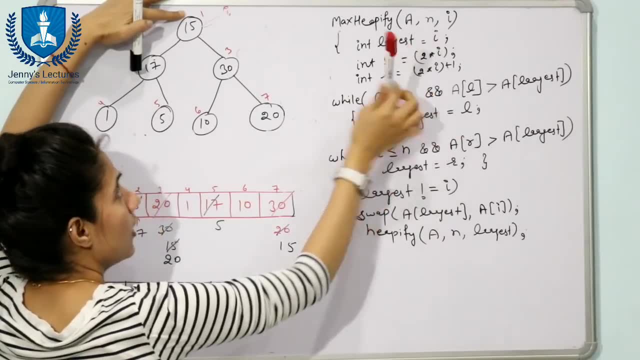 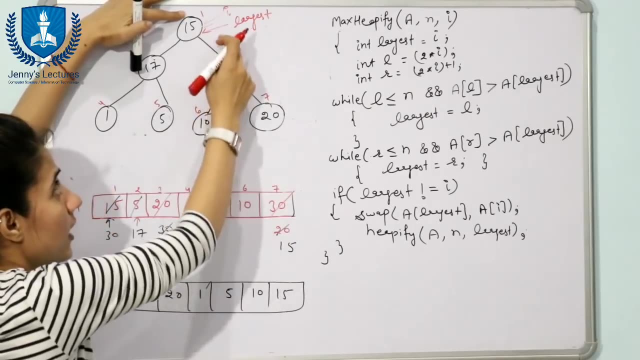 Array is this a. Now we have i value here, only Here we have i Largest. i is equal to This. largest is equal to i Means i value would be stored to largest only. So here also we have Largest, Okay. 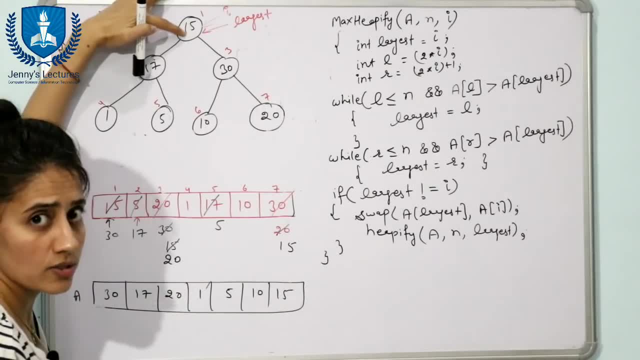 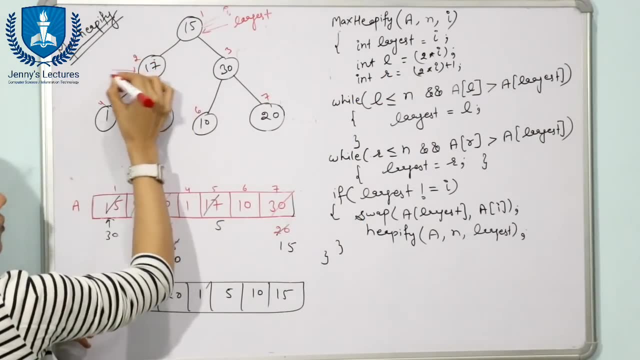 Both i and largest is now same At starting we are considering this is the largest element. Now. next step is Find out left and right child. Left child is 2 into i, That is, 2 into 1.. Here we have left. 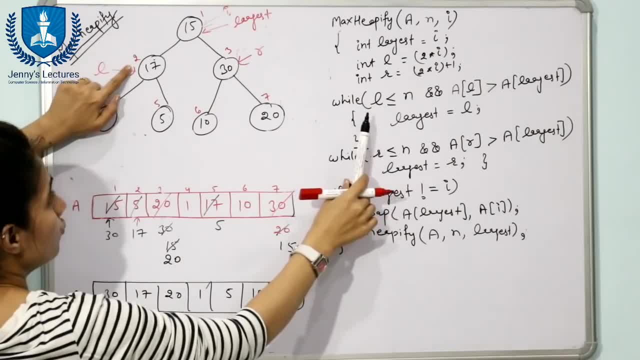 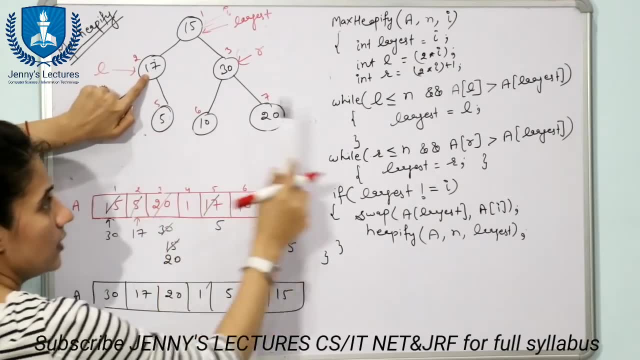 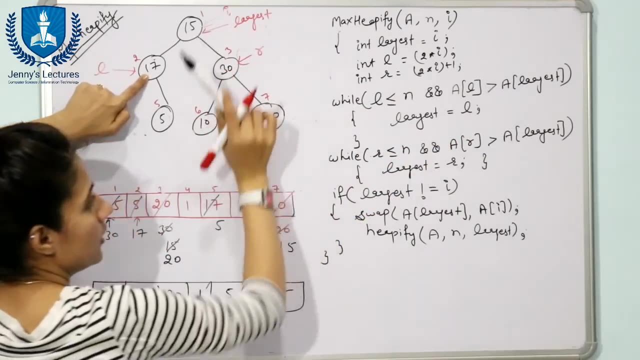 Next step is Check these conditions. Left is 2.. 2 is less than equal to n. n is 7.. Yes, a of left, a of 2, is 17.. And a of largest Largest is equal to this 1.. 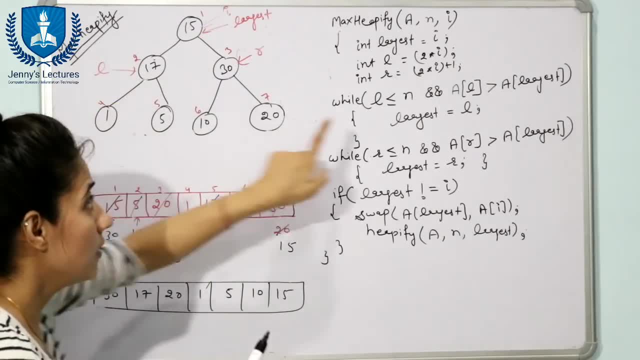 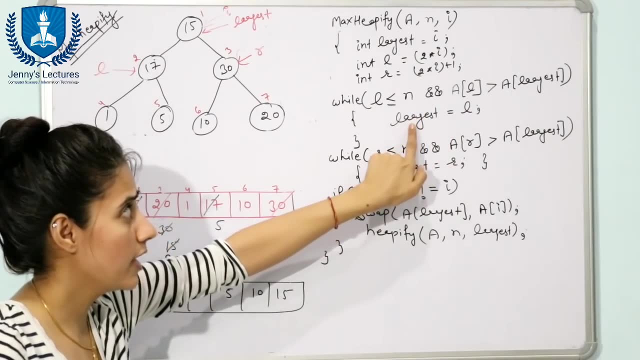 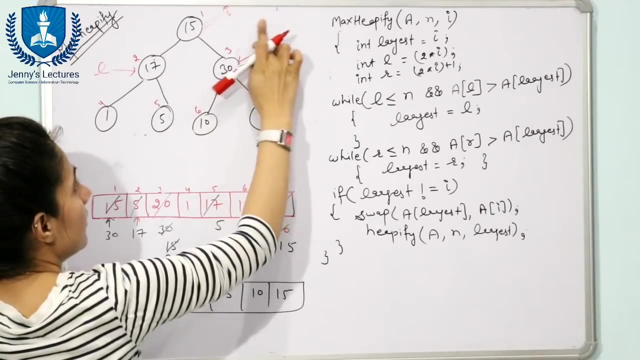 And this one is 15.. So 17 is greater than 15.. Yes, In that case, what will happen? L value will be passed. L value would be assigned to this Largest variable, So now The largest has been updated. 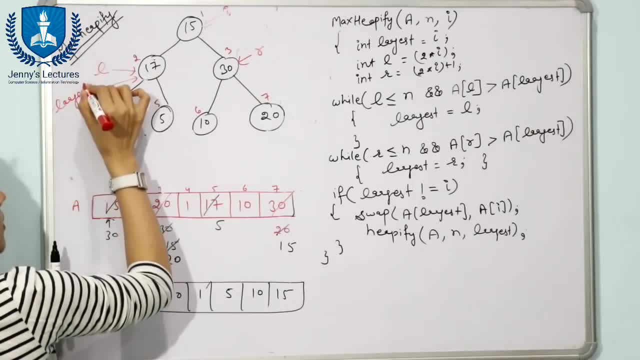 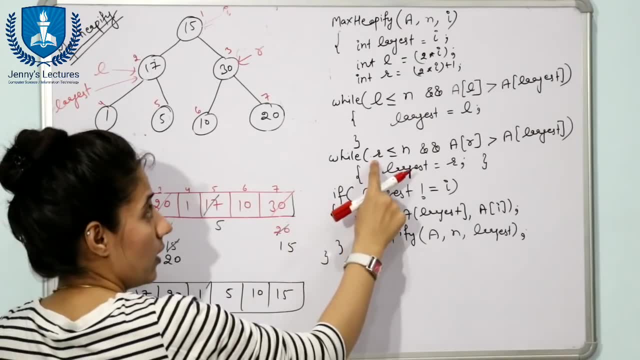 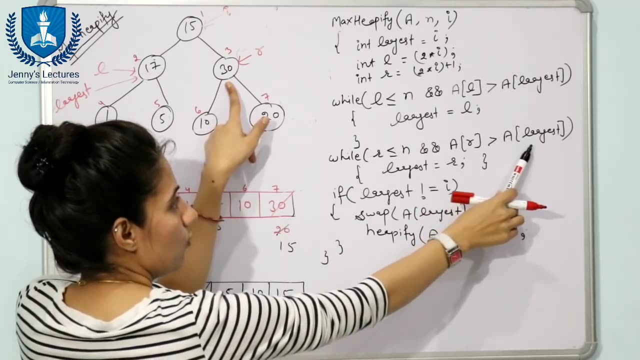 And now, here we have, Largest Right. Now we are going to check with right Right also Right child also R. R value is 3.. 3 is less than n. Yes, A of r, 1. Not i. 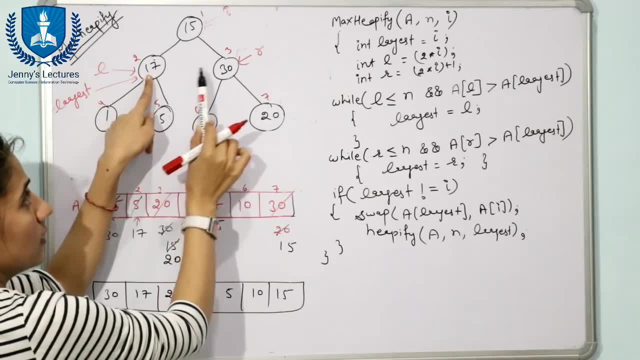 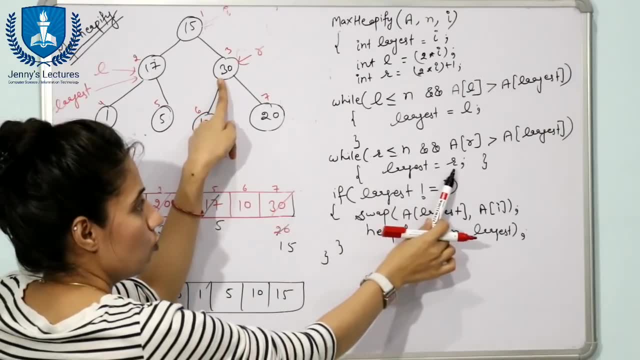 Now largest has been updated, So largest is now 17.. But 30 is greater than 17.. So this condition is also true. Now what is done? Largest is equal to r. R value is assigned to largest. So now again, largest would be updated. 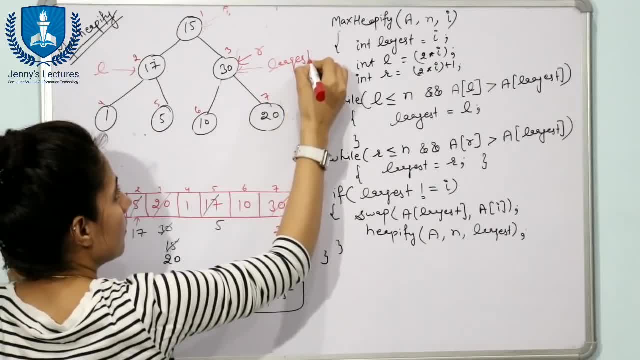 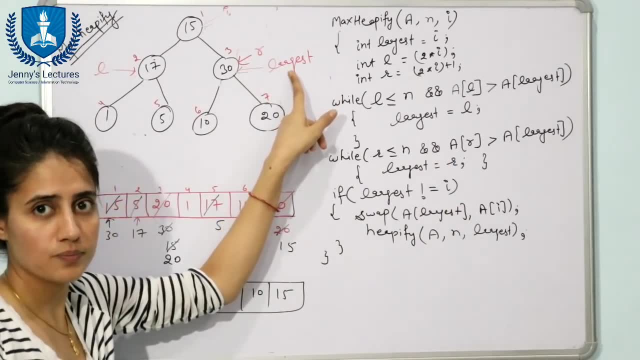 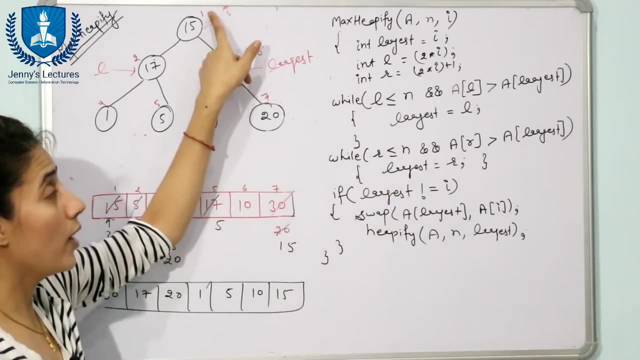 And here we have now. This is now the largest element, Same as r. R value is 3.. Largest is also now 3.. Now next step is you have to check If largest is not equal to i. i value is still 1.. 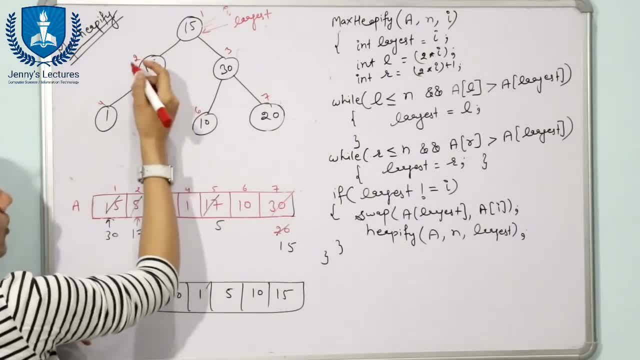 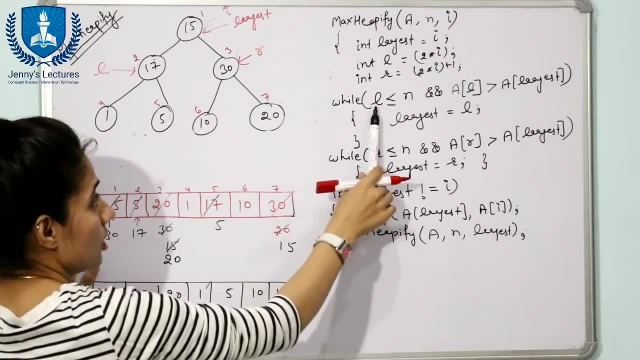 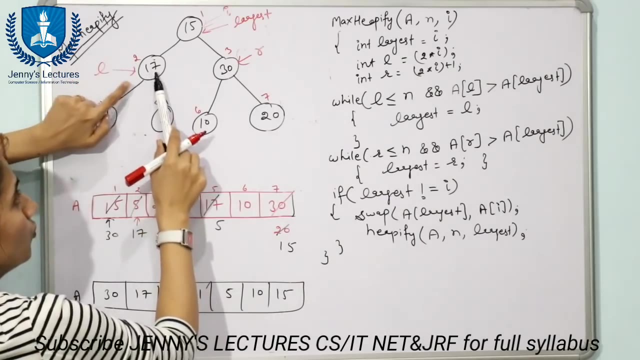 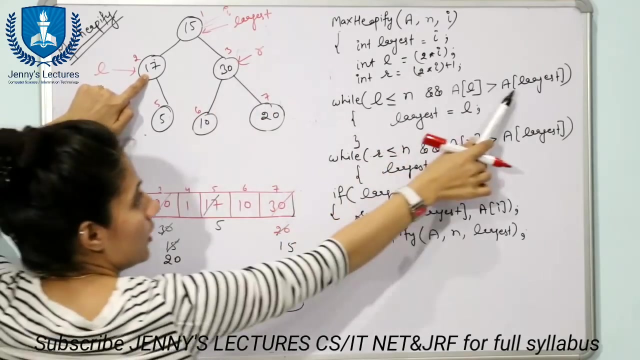 left and right child. left child is two into I, that is, two into one. here we have left and here we have right. next step is check these conditions. left is two, two is less than equal to n and is seven. yes, a of left, a of two is 17 and a of largest. largest is equal to this one and this, this one is 15.. so 17 is. 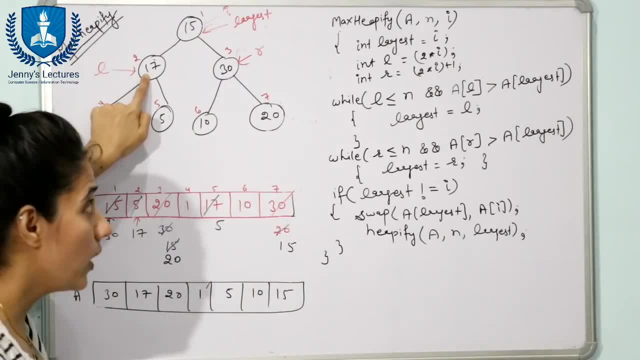 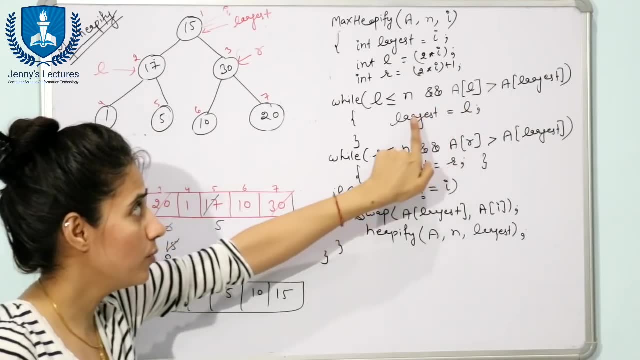 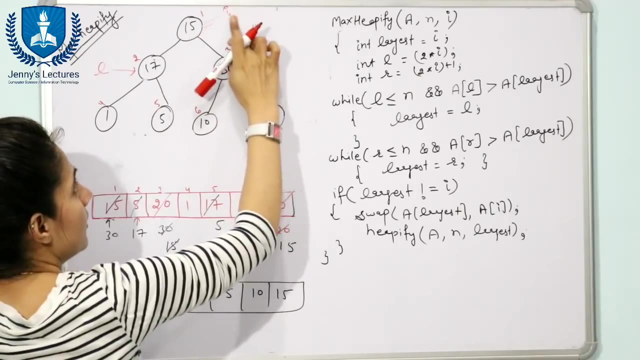 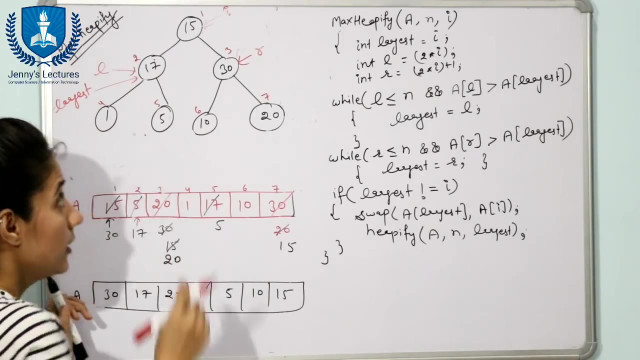 greater than 15. yes, in that case, what will happen? this largest is equal to l, so l value would be passed, l value will be would be assigned to this largest variable. so now the largest has been updated and now here we have largest. right now we are going to check with right, right also, right child also R, R value. 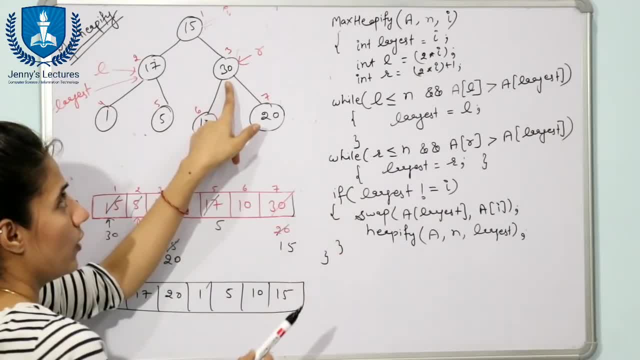 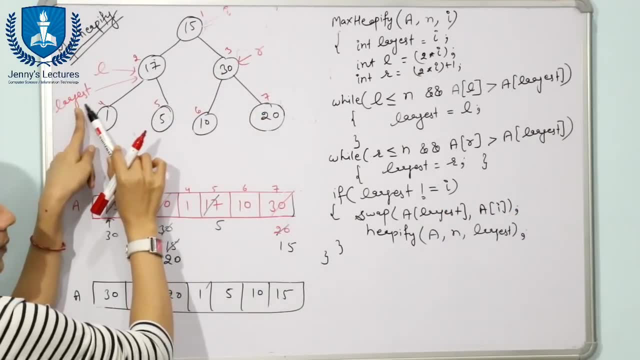 is three. three is less than n. yes, a of R. a of three means value. value is what? 30, 30 is greater than a of largest. now, largest is what? this one, not I. now, largest has been updated, so largest is now 17.. but 30 is greater than 17.. so 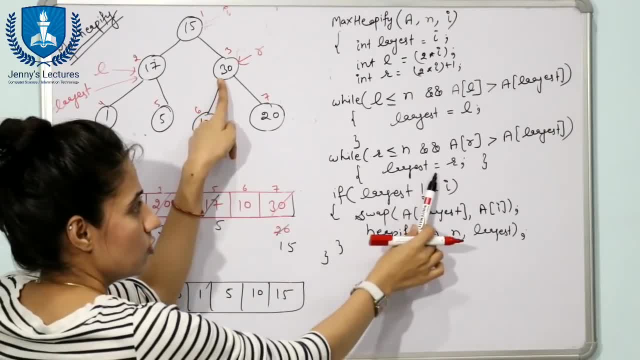 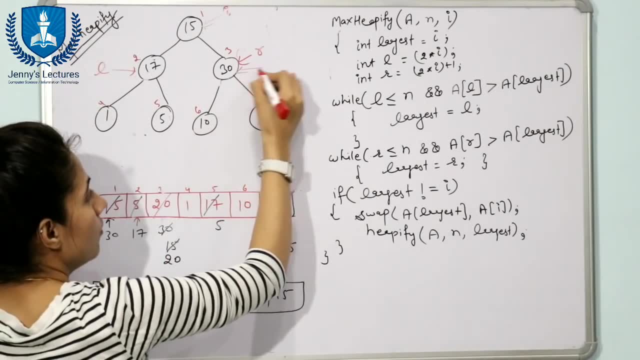 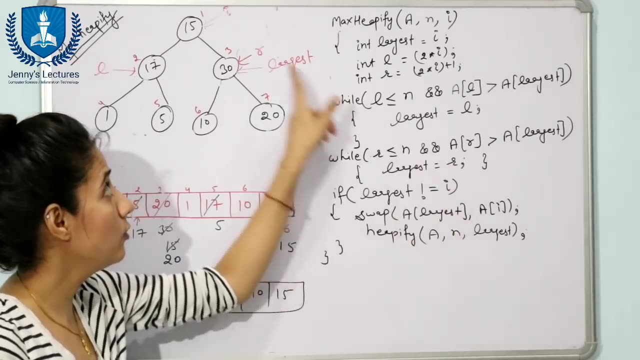 this condition is also true. now, what? what is done? largest is equal to R. now R value is assigned to largest. so now again, largest would be updated. and here we have now. this is now the largest element, same as R. R value is three. largest is also now three. fine, now next step is you have to check if 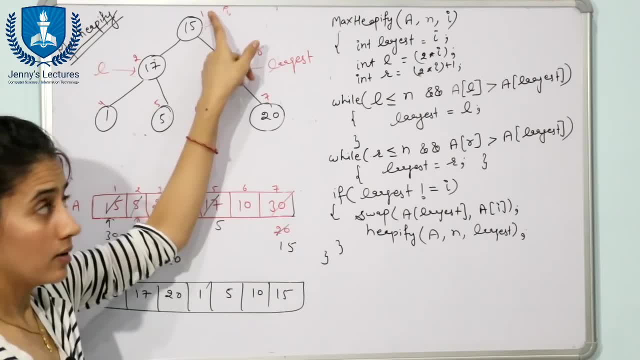 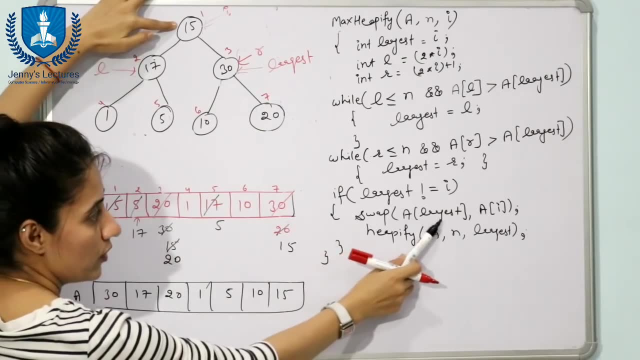 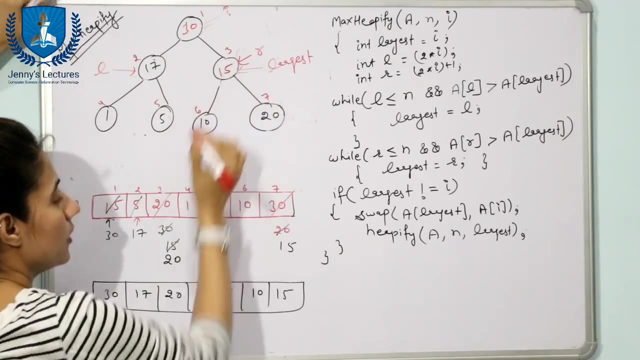 largest is not equal to I. I value is still one, largest value is three. so this condition is also true. then you will do what? swapping of this 15 and 30, swapping of a of largest with a of I. so now we will do what: 30 would go up and 15 would go. now, right, but we are not done yet. 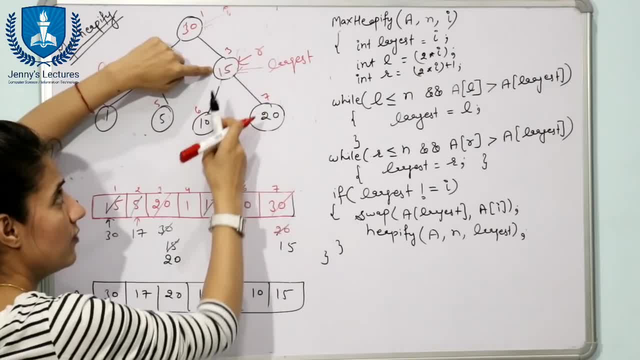 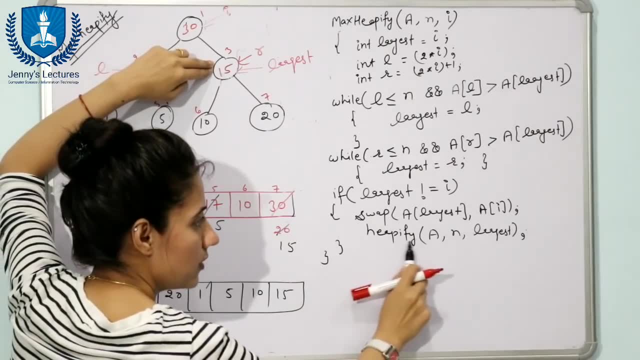 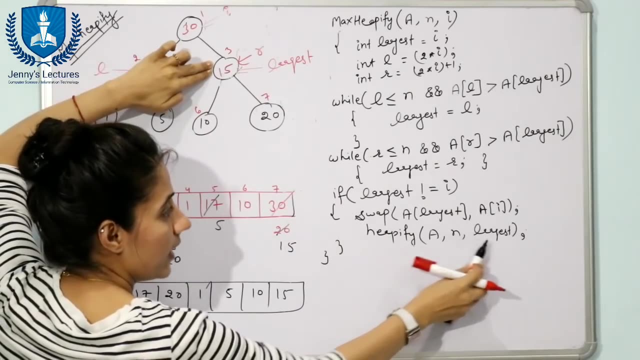 we are going to, we are going to calculate again left and right child of this one till we reach to the end. fine, that is why we, we are recursively calling this ep5 method here now. we are going to call ep5 at this point, at this point, array n and largest, largest value is what? three now. so, 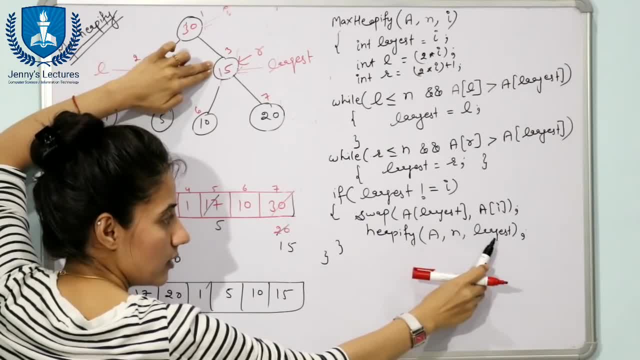 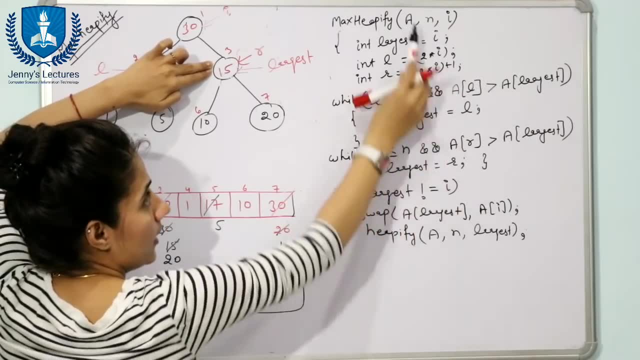 largest is three now. so that is why we are going to pass largest here here we are. that is why we are going to pass here largest value. so now, here we are going to pass a n and largest. so largest value is now three. so three would be. 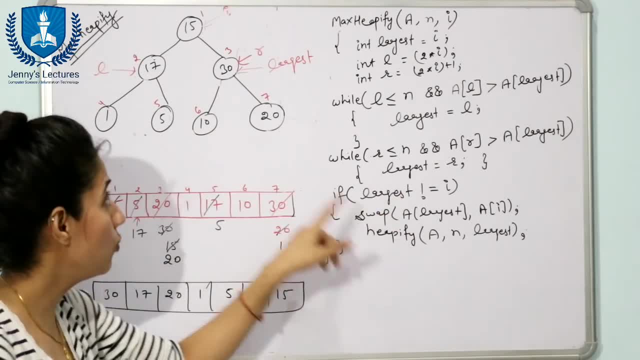 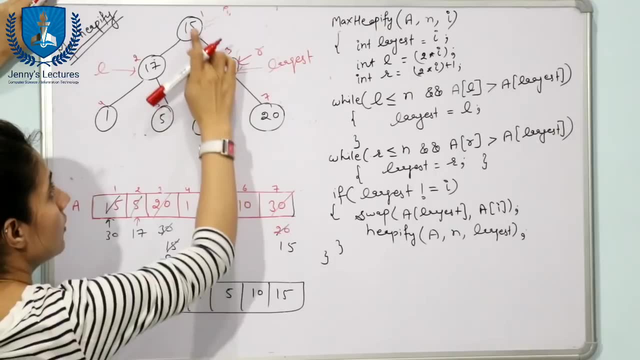 Largest value is 3.. So this condition is also true. Then you will do what? Swapping of this 15 and 30. Swapping of a of largest with a of i. So now we will do what 30 would go up. 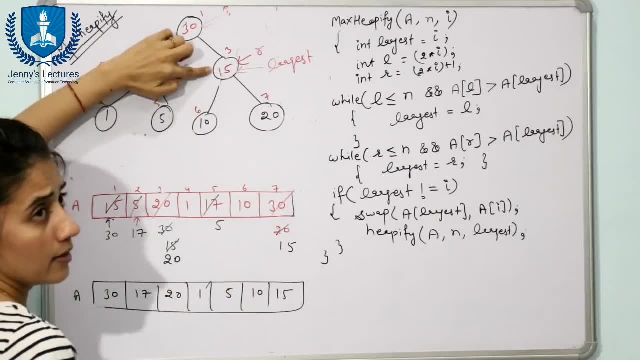 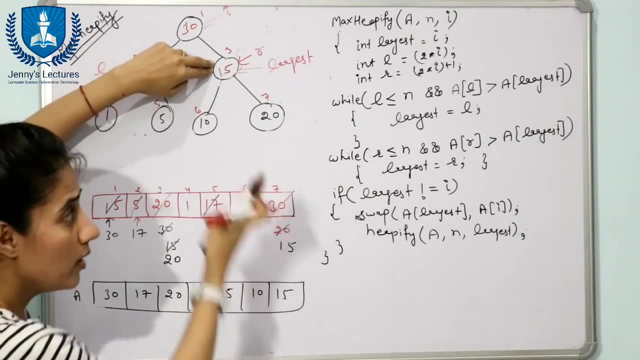 And 15 would go down Right. But we are not done yet. We are going to calculate again Left and right child of this one, We reach to the end, Fine. That is why we are recursively calling this epify method here. 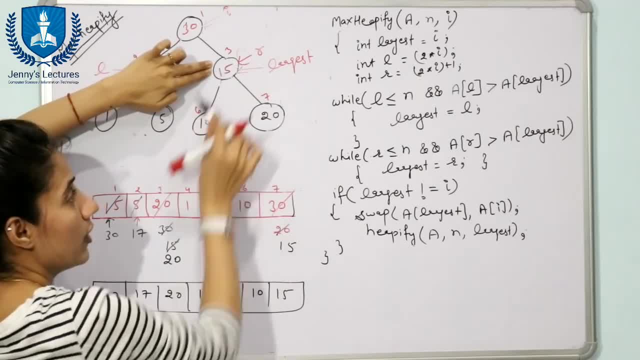 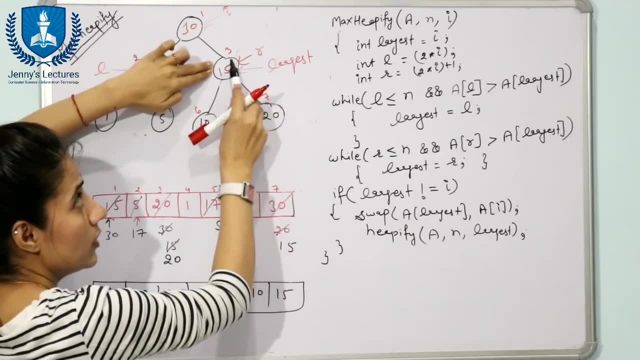 Now we are going to call epify at this point, At this point, Array n and largest, Largest value is what? 3 now. So largest is 3 now. So that is why we are going to pass largest here. That is why we are going to pass here largest value. 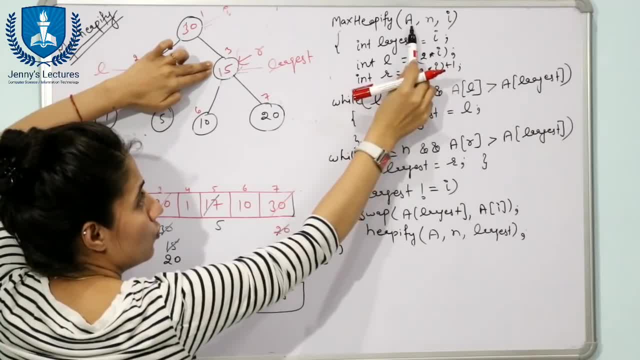 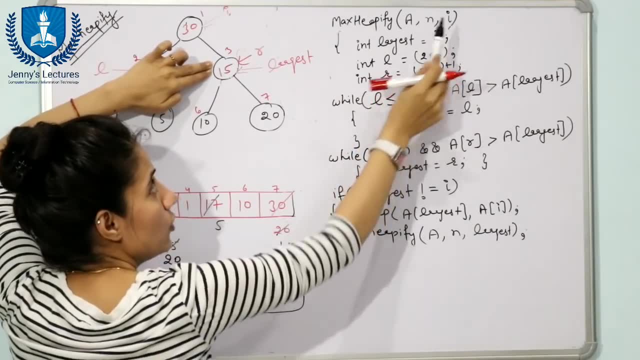 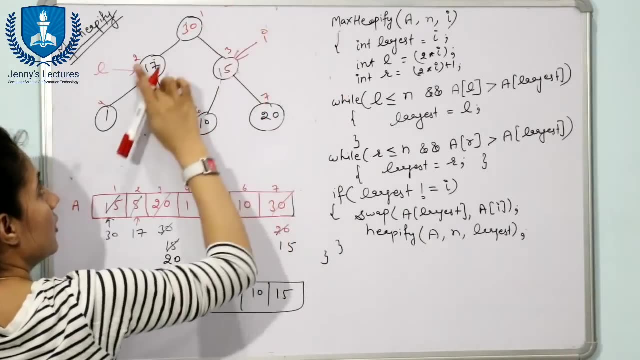 So now, Here we are going to pass a and largest, So largest value is now 3.. So 3 would be passed. So now i value is 3.. So now, Again, here we have i. i has been updated. 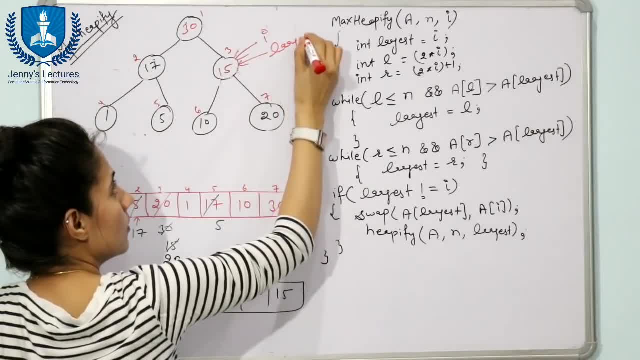 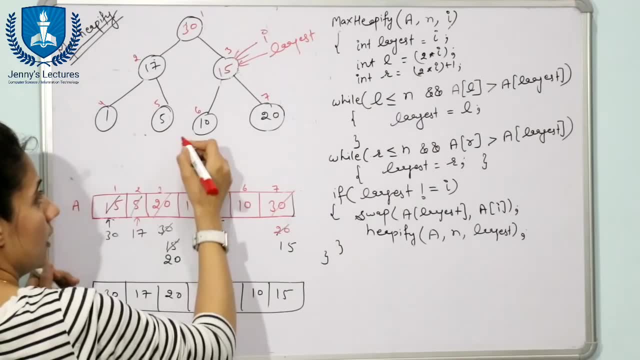 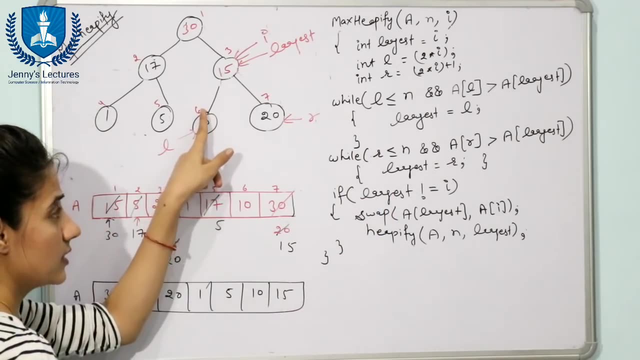 And here also we have Largest Fine. Calculate l value 2 into i, 3 into 2, that is 6.. Here we have l. And here we have now r. Again, check same condition, Left 6.. And a of l. 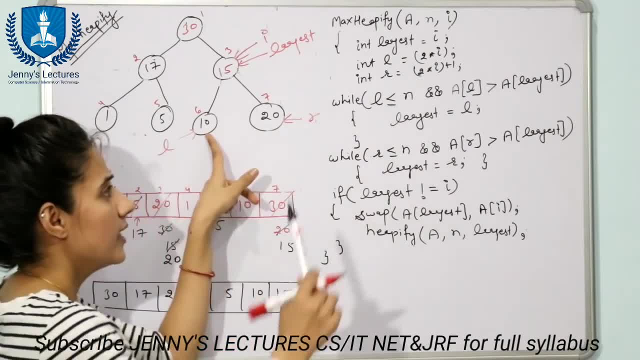 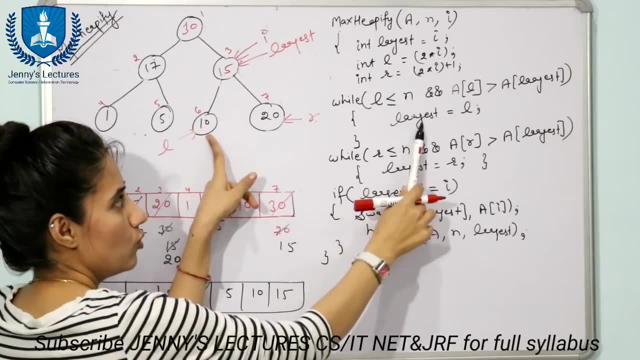 a of l value is 10.. Is 10 greater than a of largest? Now largest value is here, now this one: 10 greater than 15? no, So control will not go to this loop Again, this y loop. Check for right child. 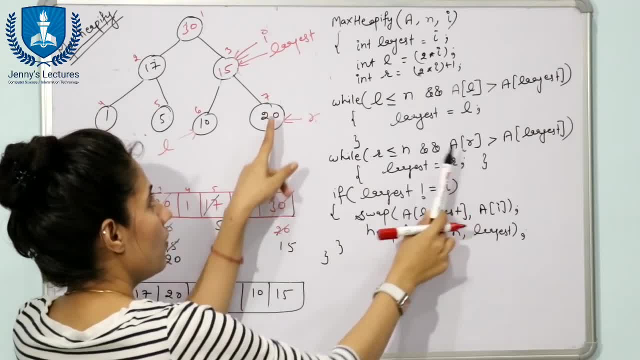 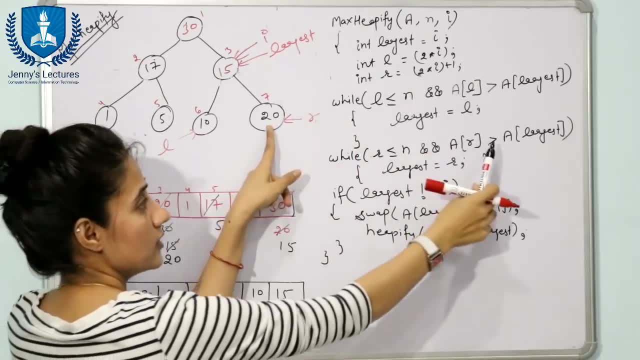 7 is less than equal to 7.. Yes, this condition is true. And a of r, a of r is 20.. 20 is greater than a of largest Largest value is 15.. So is 20 greater than this 15.. Yes, This condition is also true. 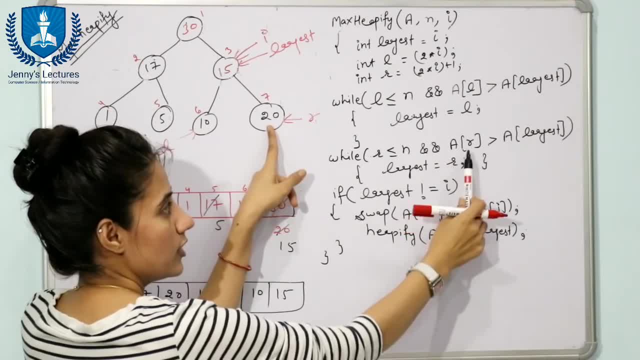 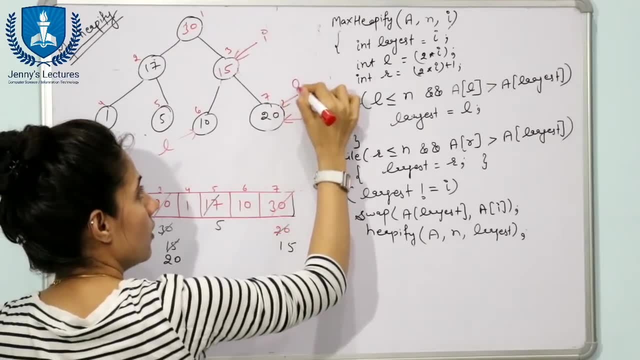 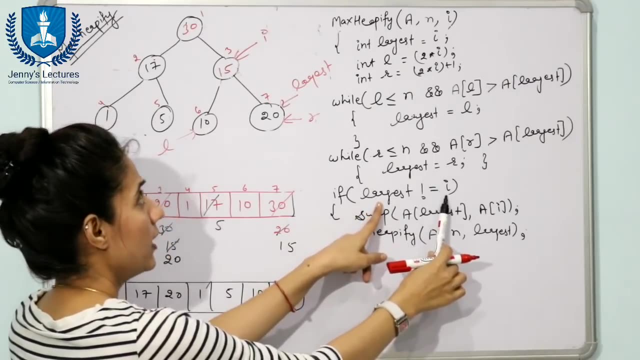 Control will go to this loop. Now largest is equal to r r value is here what 7.. So now 7 would be passed to largest. Now largest has been updated And here we have now Largest. Ok, Now check if largest not equal to i. 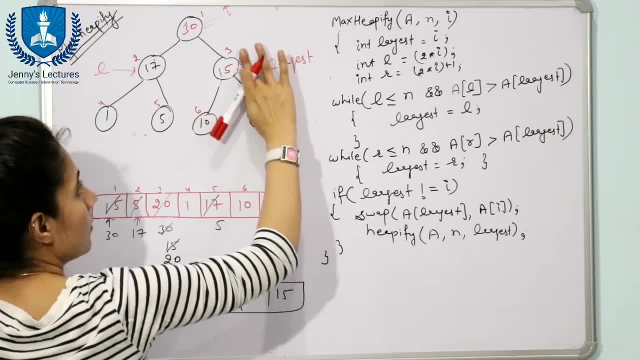 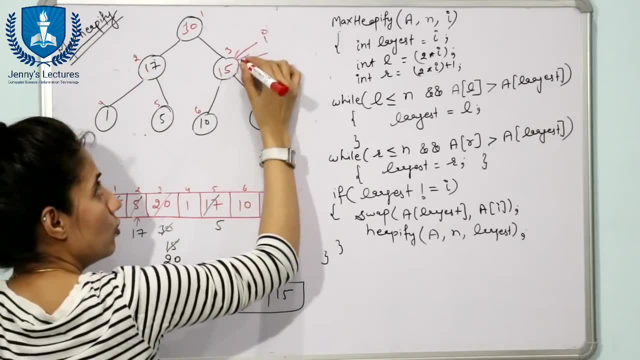 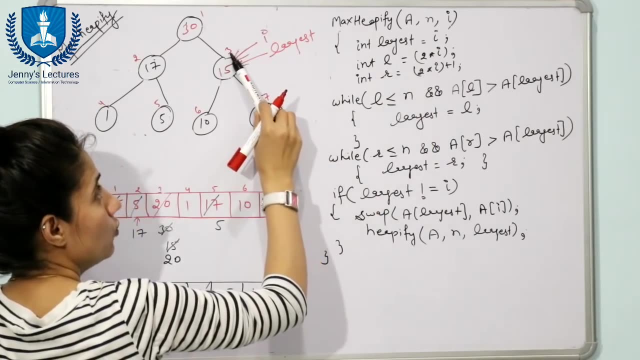 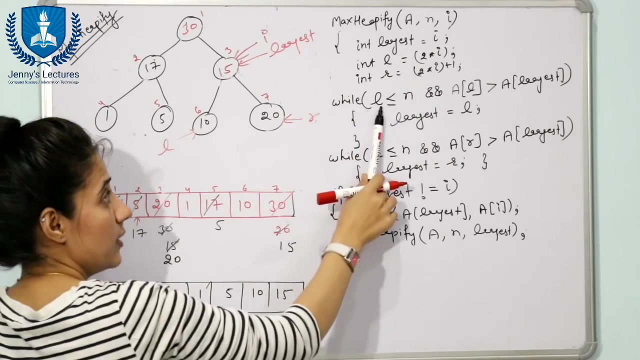 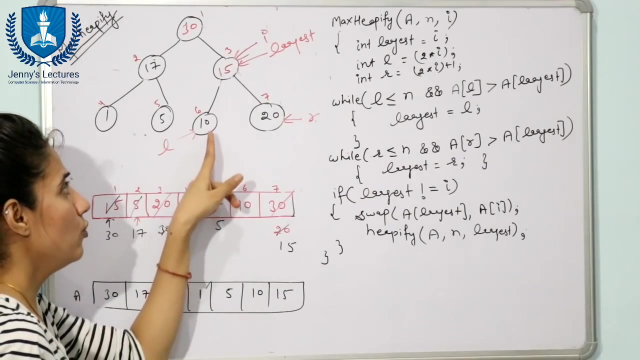 passed. so now I value is three. so now again, here we have I. I has been updated and here also we have largest fine calculate L value: two into I, two into I, three into two, that is six. here we have L and here we have now R. again check same condition: left six. six is less than seven. yes, and a of L. a of L value is: 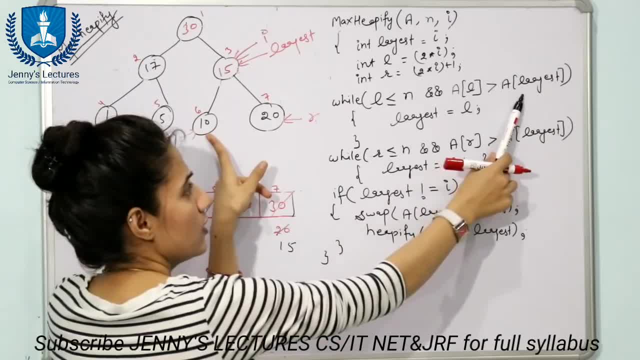 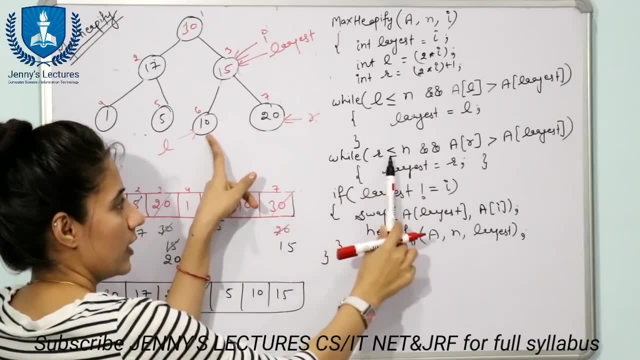 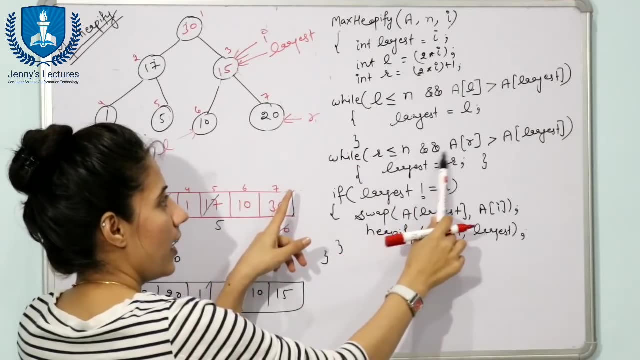 10. is 10 greater than a of largest? now, largest value is here now this one: 10 greater than 15. no, so control will not go to this loop again, this Y loop. check for right child R is less than seven is less than equal to seven. yes, this condition is true. and a of R, a of R is 20. 20 is greater than a of. 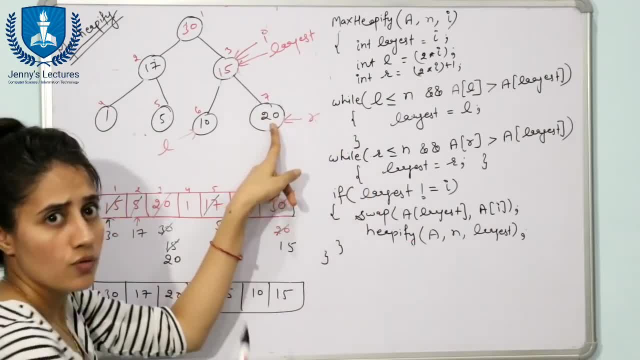 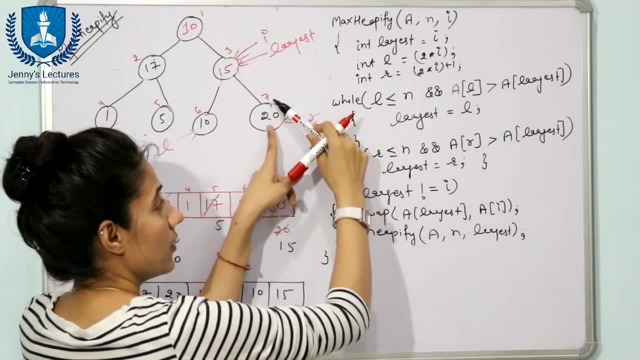 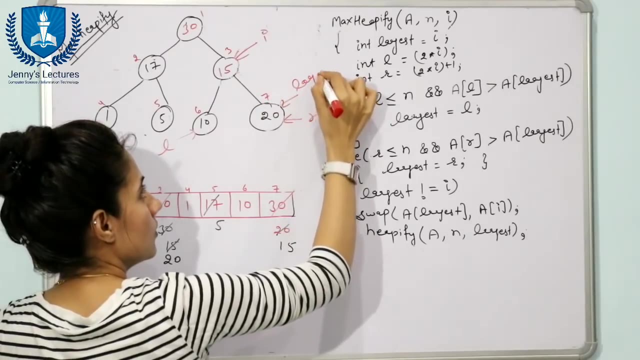 largest. largest value is 15.. so is 20 greater than this 15? yes, this condition is also true. now control will go to this loop. now, largest is equal to R. R value is here. what seven? so now seven would be passed to largest. now largest has been updated and here we have now largest. okay, now check if 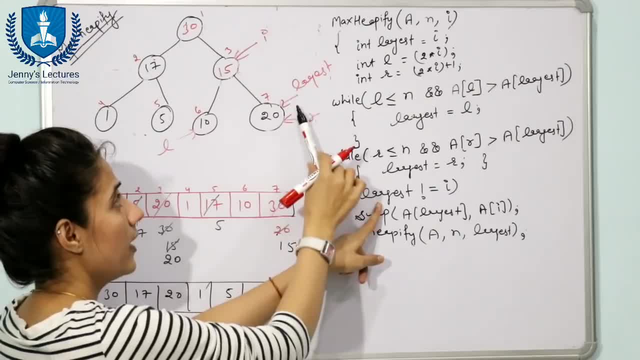 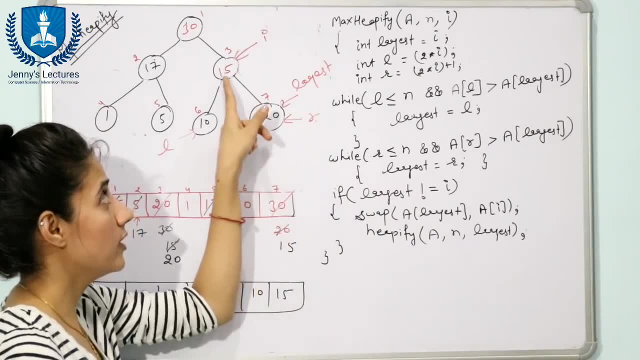 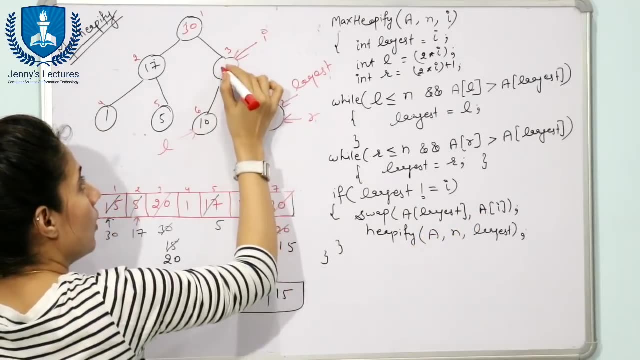 largest not equal to I. I is equal to three still, and largest is seven. so this condition is also true. largest has been updated. fine, because this right child is having value greater than parent. so next step is what we have to do: swapping, swapping of a of largest with a of I. now we will do what: 20 would go up and 15 would go down. 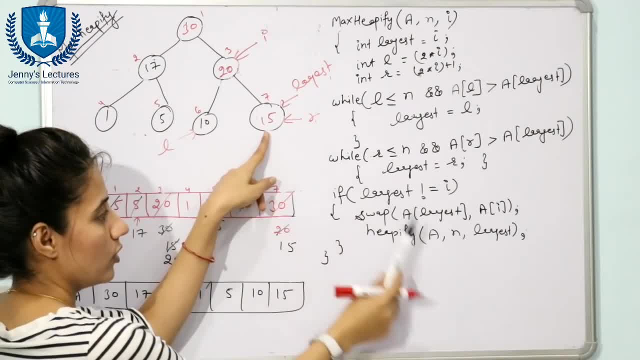 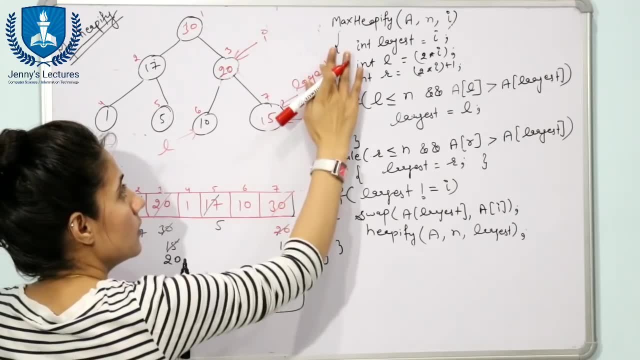 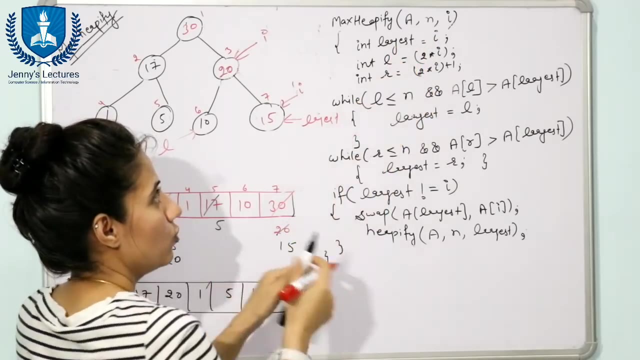 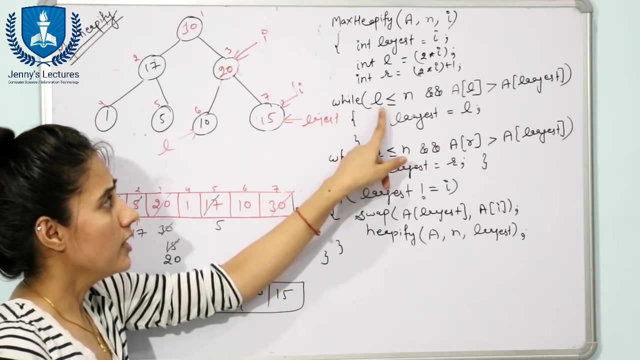 swapping again. hippify method would be called here. only a n and largest, largest value is seven. so now seven would be passed. now I value is I value as this and largest is also at this place, because I is equal to largest. now calculate L value: 7x I, 7x 2, that is 14 and this is 15. now check is 14. now in this case L value is 14 and right value is. 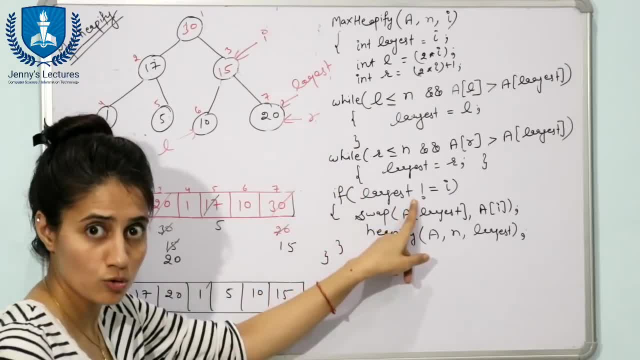 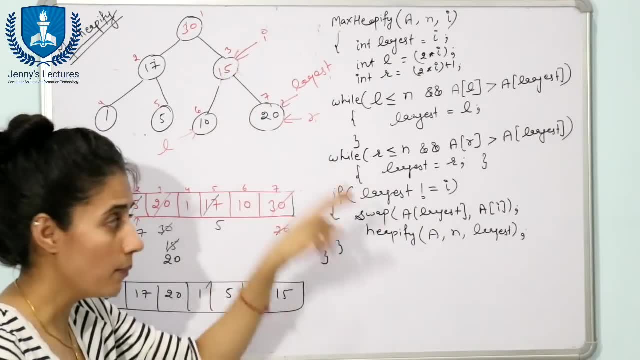 i is equal to 3 still, And largest is 7.. So this condition is also true. Largest has been updated. Fine, We have to do swapping, Swapping of a of largest with a of i. Now we will do what. 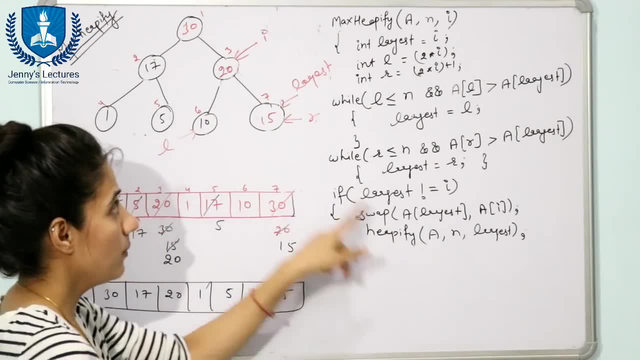 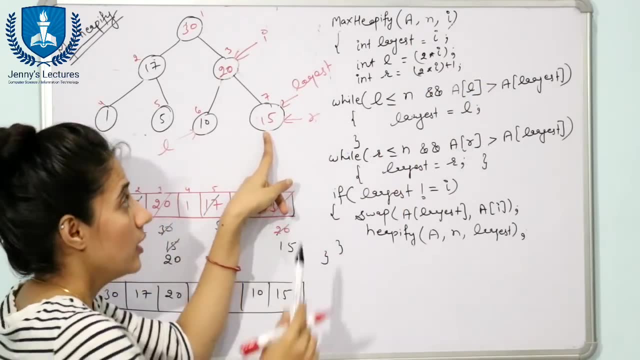 20 would go up and 15 would go down. Swapping Again, hippie phi method would be called here only a n, and largest, Largest value is 7.. So now 7 would be passed. Now i value is: 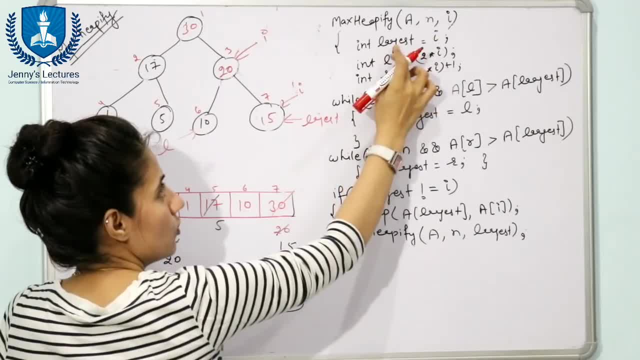 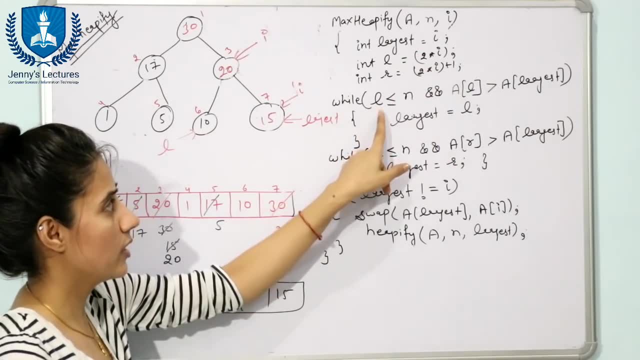 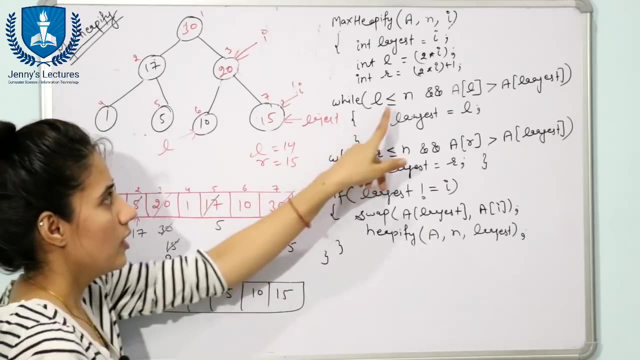 i value is this And largest is also at this place, Because i is equal to largest. Now calculate l value: That is 14.. And this is 15.. Now check Is 14.. Now, in this case, l value is 14 and right value is 15.. 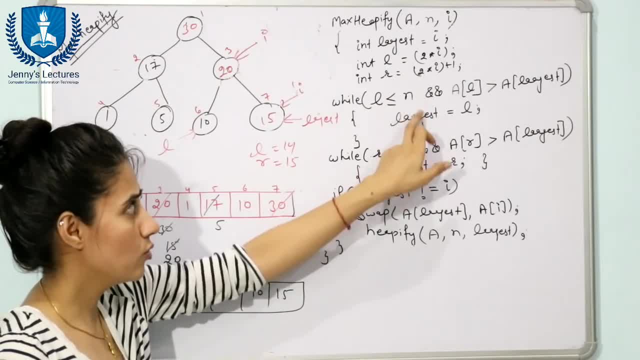 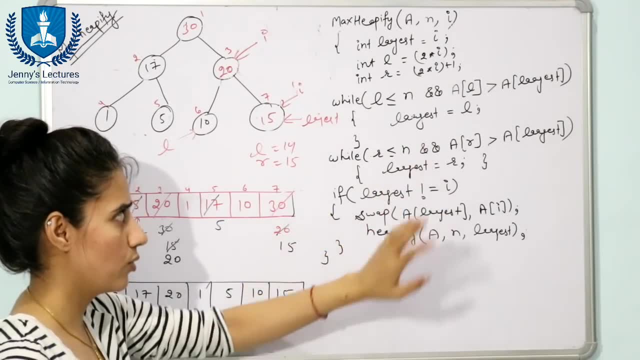 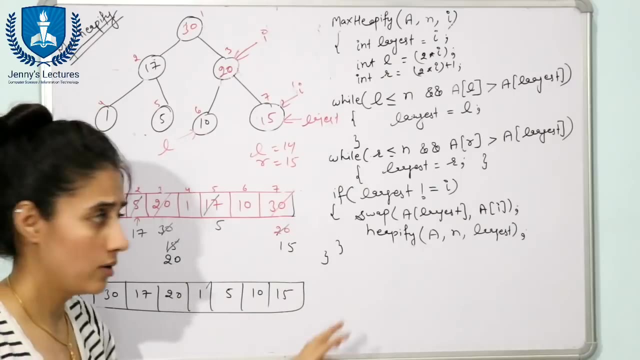 Now check: Is 14 less than equal to 7?? No, This condition is not true. Control will not go to this node. Is r value 15 less than equal to this n? No, This condition is also not true. So here we will check. 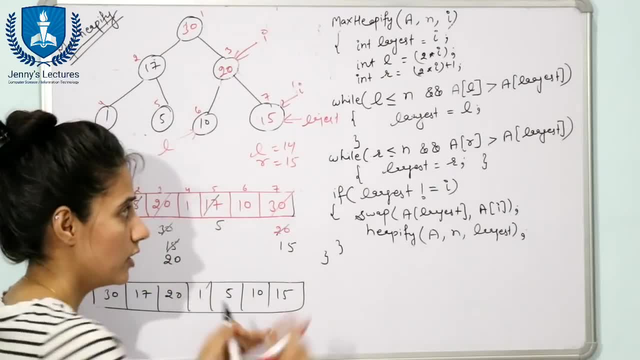 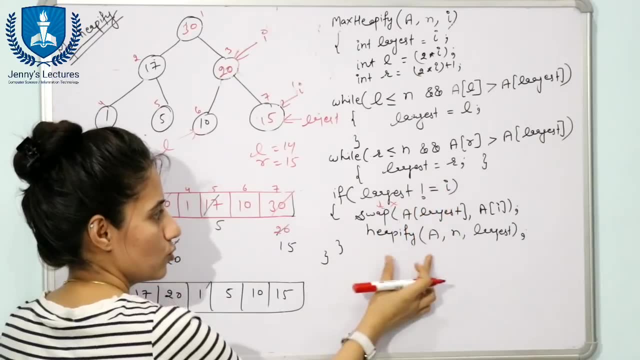 Largest, not equal to, i Fine, Because control will not go to this loop. Control will not go within this if condition, Because this condition is not true. So then hippie phi method will not be called. Now we will stop to call hippie phi method. 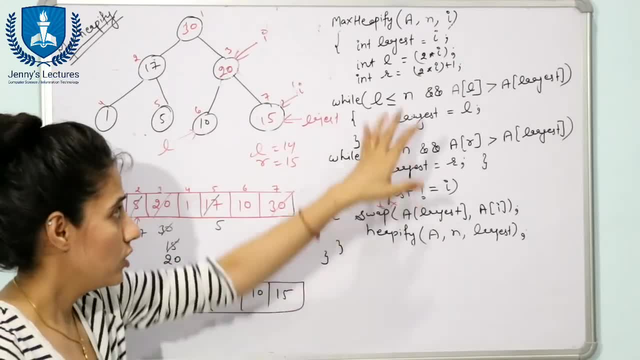 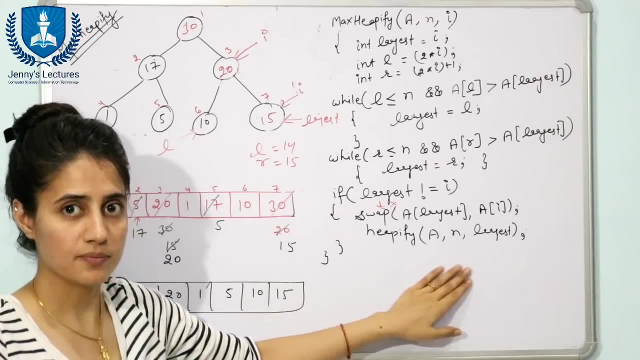 Because we have reached at the end. So this is how max heap would be built using this hippie phi method And the time complexity using this is order of n In heap sort. you can use this hippie phi method And if you are going to, 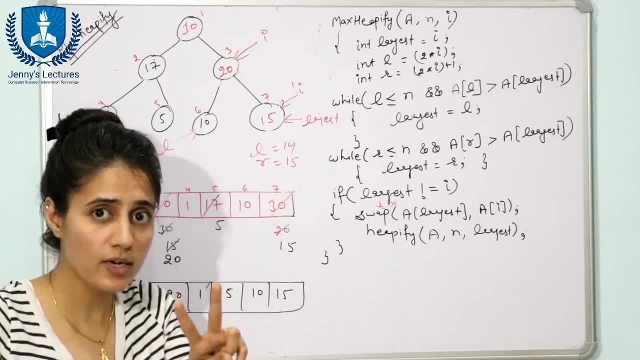 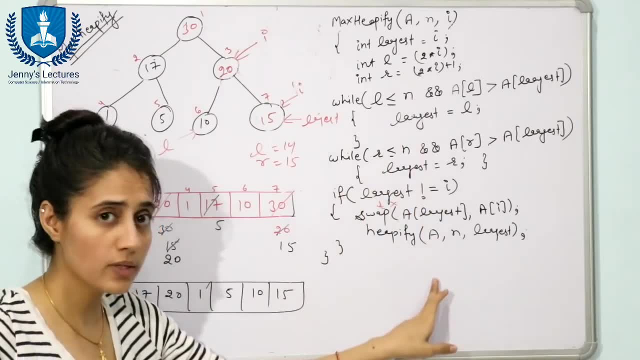 write down the code for heap sort. Then how you will write. two step would be there in heap sort: First, building of max heap. next, deleting- In building also, you will call this method. Second, in deleting also, you will call this method. Now how to write down that code. 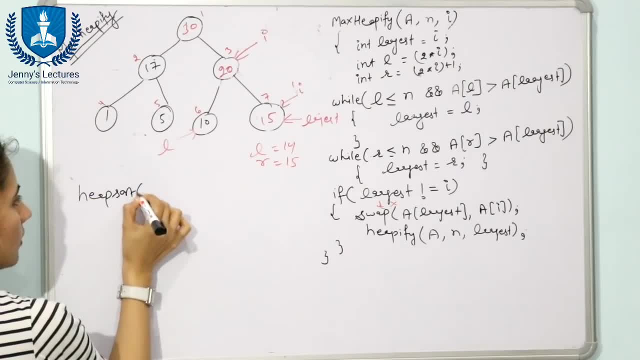 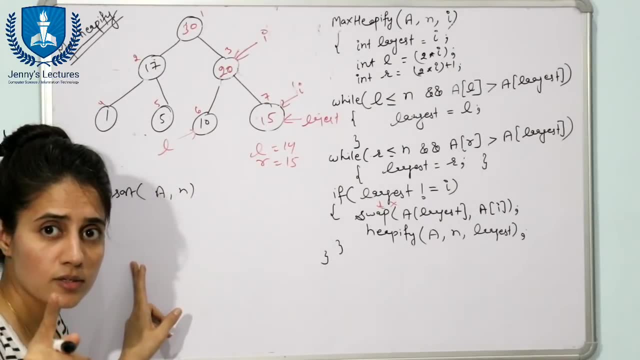 So now you can write like heap sort array. you can pass here array and total number of element. And first step in heap sort is build a max heap. For building max heap Here you are going to call hippie phi method. I have already told you from: 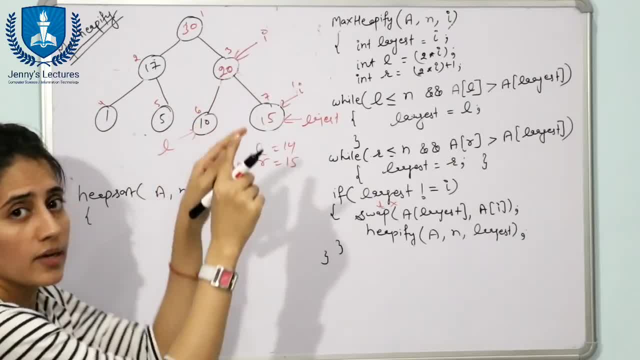 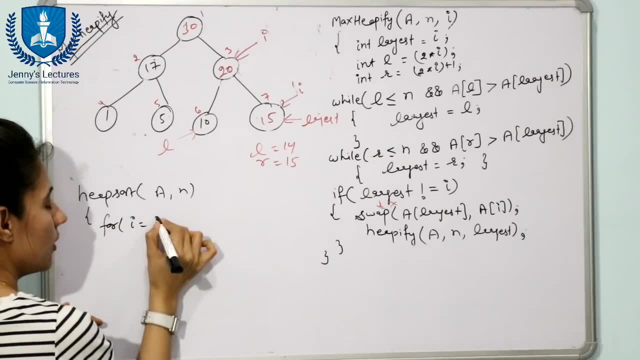 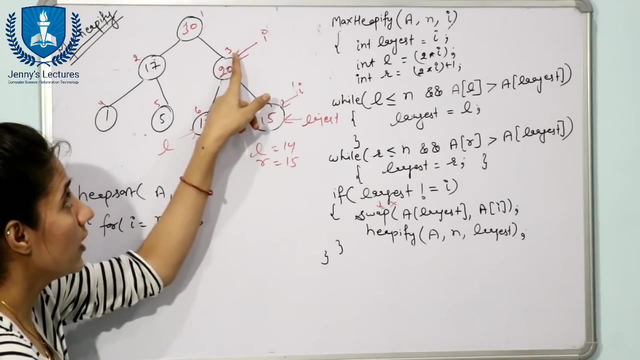 n by 2. From the non leaf node which is at largest index. So we are going to write a for loop, for i is equal to n by 2. i should be greater than we are going to call, first of all at 3, then 2 at 1, till we reach to the. 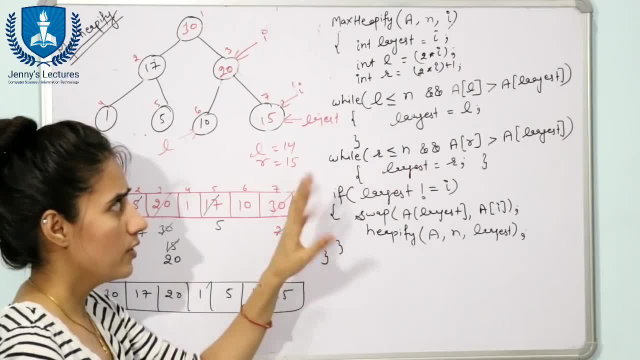 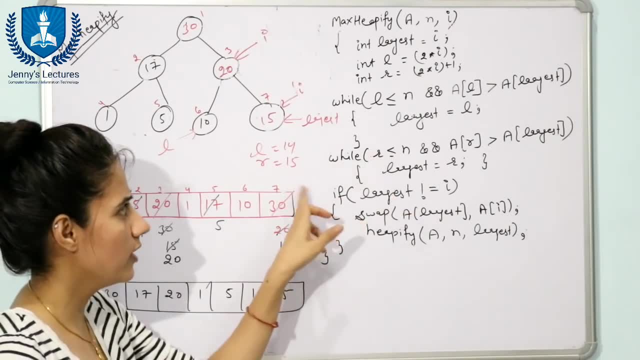 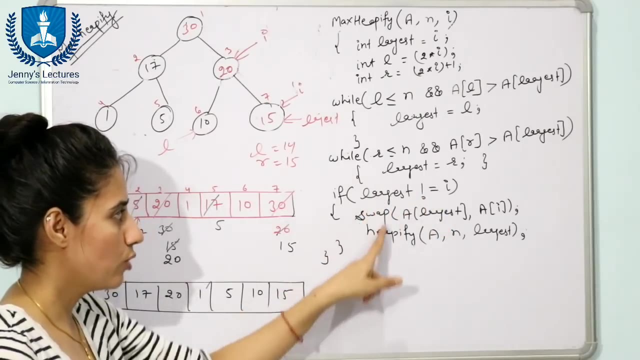 15. now check: is 14 less than equal to 7? no, this condition is not true. control will not go to this row. is R value R value 15: 15 less than equal to this n? no, this condition is also not true. so here we'll check: largest not equal to I. so that condition is also not true. no, swapping would be done. and now? 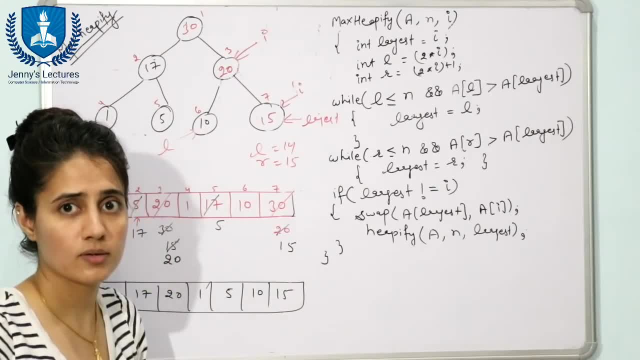 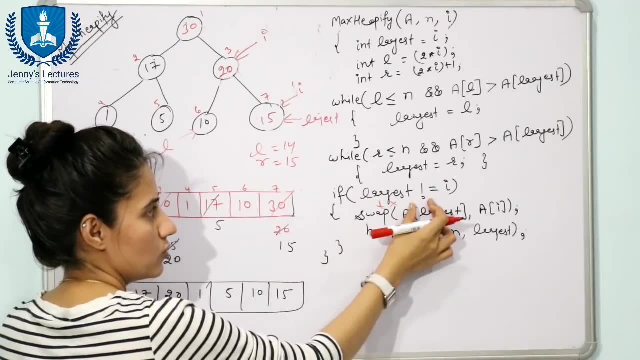 this is done, going to. we are not going to call this heapify method. fine, because control will not go to this loop. control will not go within this if condition, because this condition is not true. so then heapify method will not be called. now we are going. we will stop to call heapify. 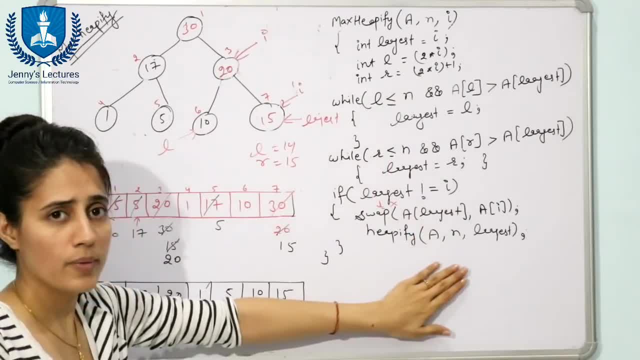 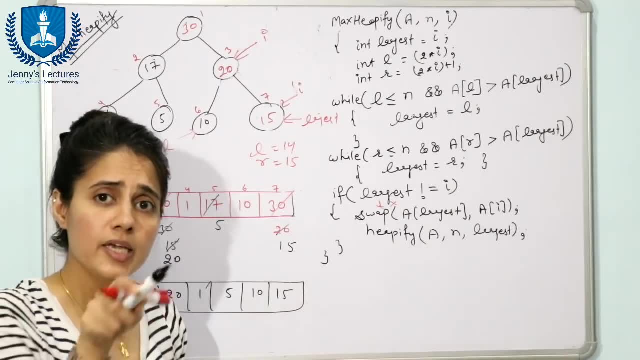 method because we have reached at the end. so this is how max heap would be built using this heapify method and the time complexity using this is order of n in heap sort, you can use this heapify method and if you are going to write down the code for heap sort, 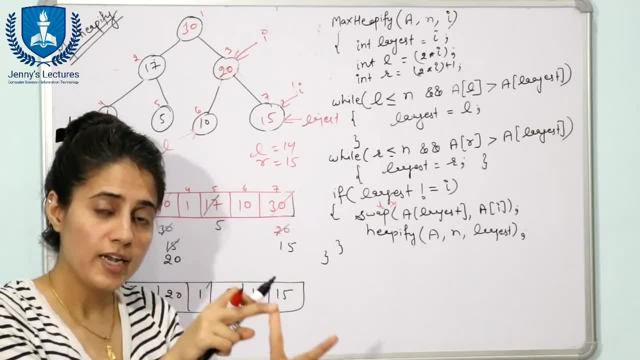 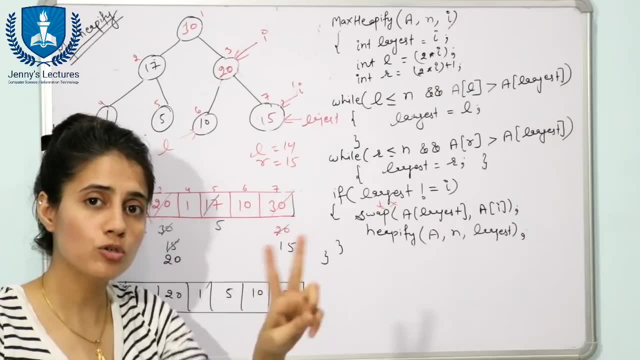 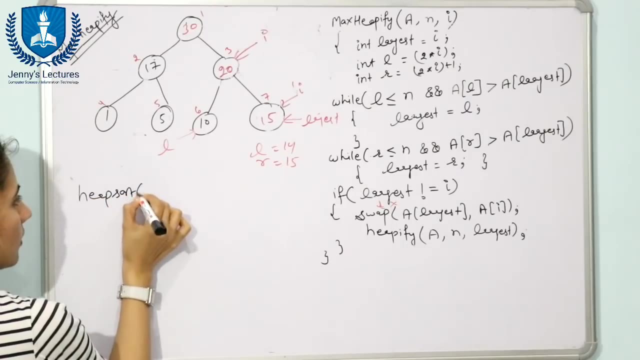 then how you will write- two step would be there in heap sort: first building of max heap, next deleting. in building also you will call this method. second, in deleting also you will call this method: now how to write down that code. so now you can write like heap sort array. 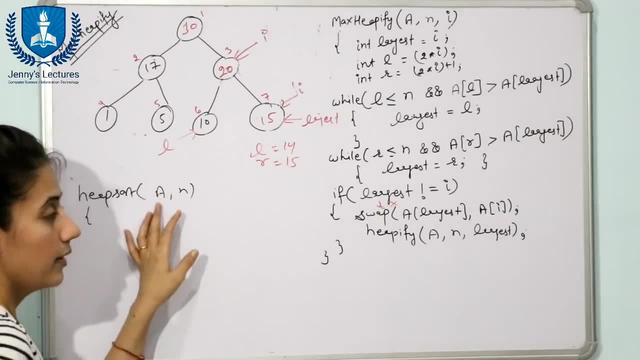 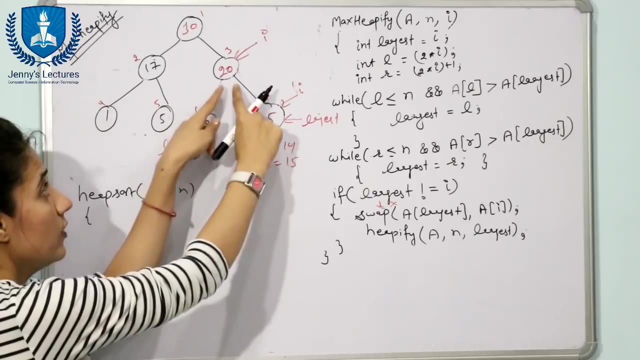 you can pass here array and total number of elements and first step in heap sort is you just build a max heap in build for building max heap from where you you are going to call heapify method. i have already told you from n by 2, from the non leaf node, which is 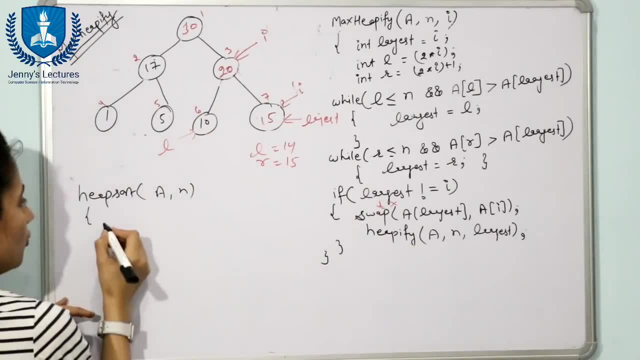 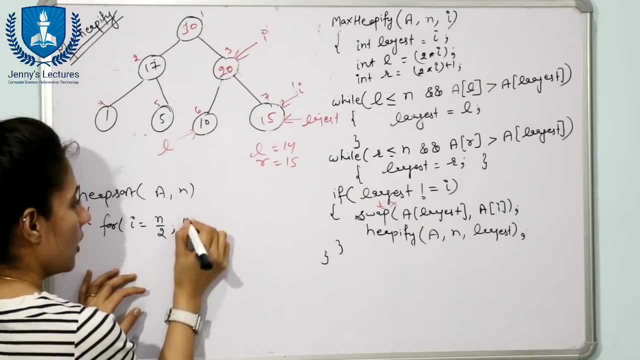 at at largest index. fine, so we are going to write a for loop, for i is equal to n by 2. i should be greater than we are going to call, first of all at 3, then 2 at 1 till we reach to the end. 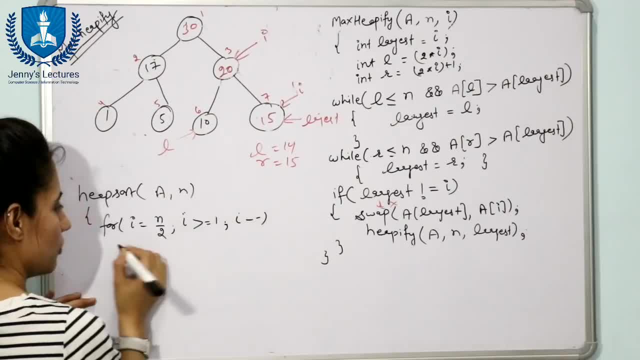 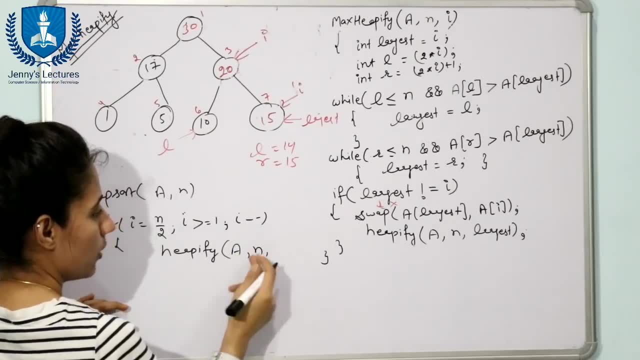 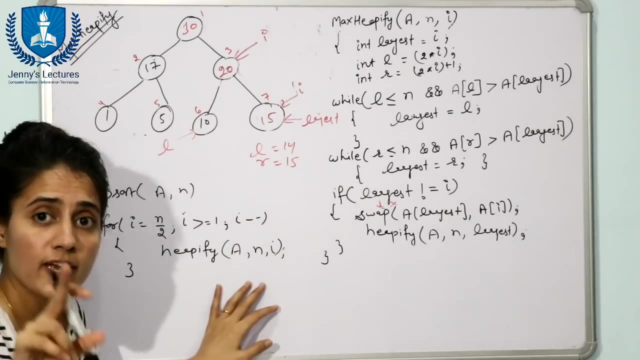 i should be greater than equal to 1 and i minus minus. here we are going to call this method heapify method array. we are going to pass this n and we are going to pass i right now. this, this step, is just for building now. next is deleting. fine, now deleting would be. 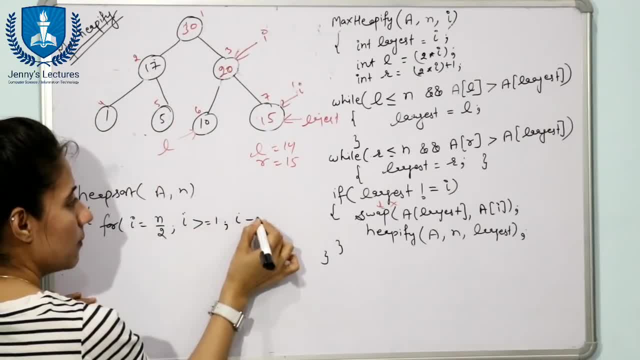 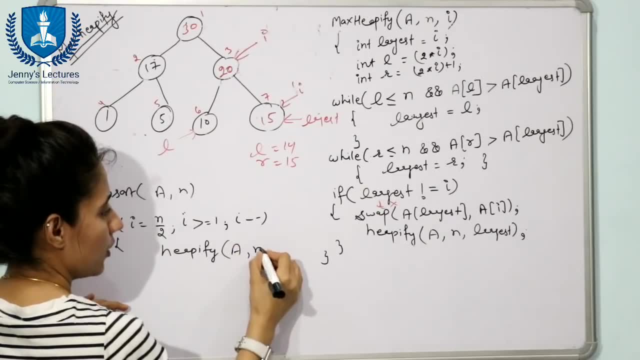 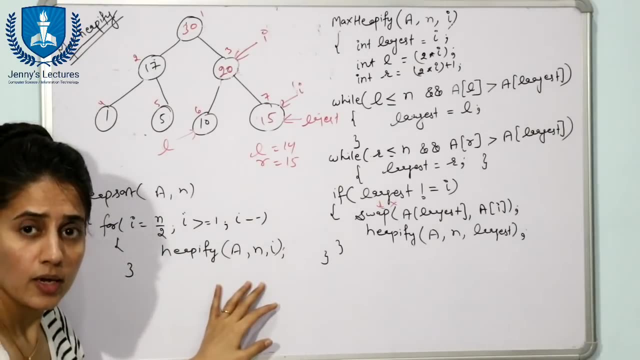 end, i should be greater than equal to 1 and i minus minus. Here we are going to call this method hippie phi method Array. we are going to pass this n and we are going to pass i. Right now, this step is just for building. 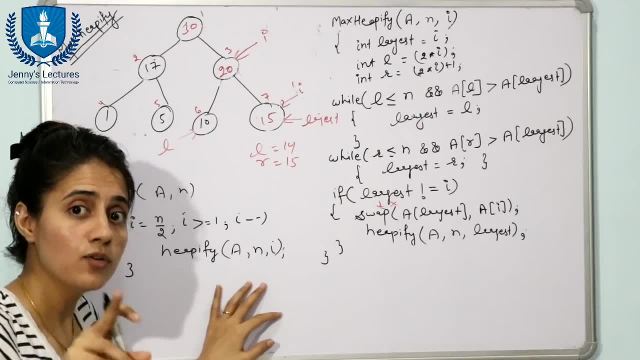 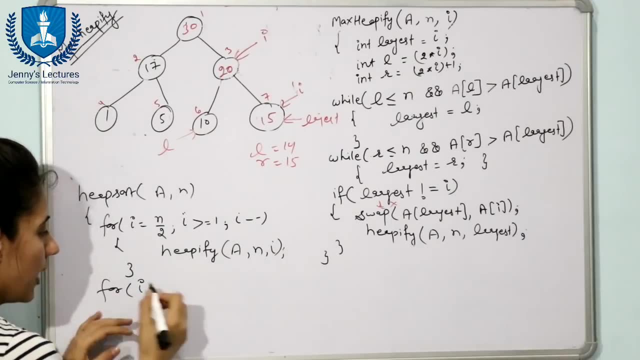 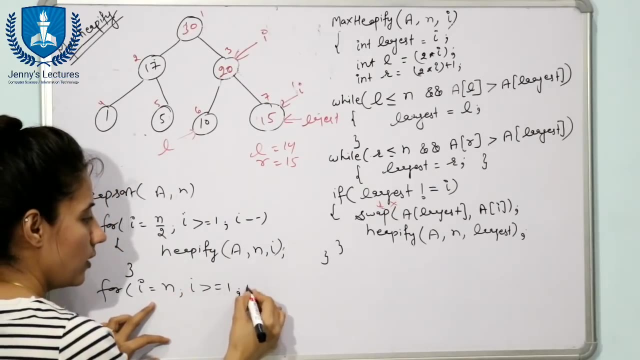 Now next is deleting. Fine, now deleting would be done from the root always. So now we are going to call one for loop again, And this: i would be n, i should be greater than equal to 1 and i minus minus. So here see this. 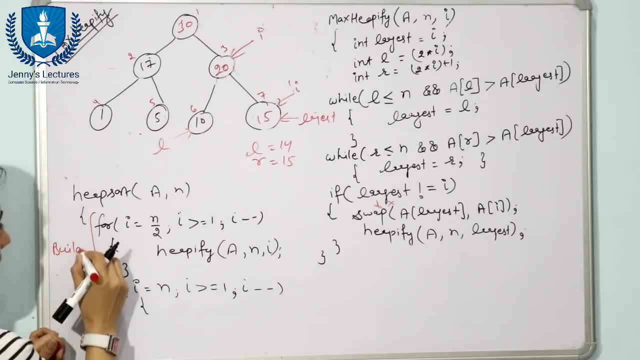 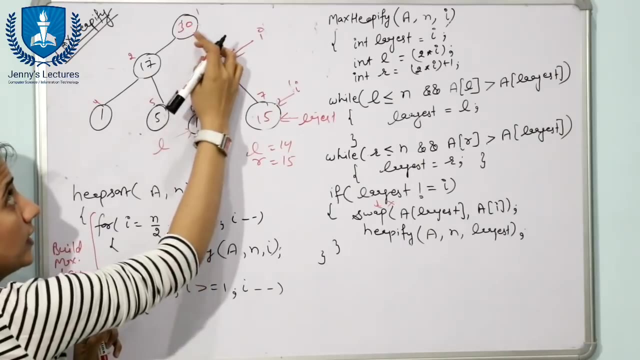 this step is what? build max heap, this for loop, right. And after that next step is what for deleting element from max heap? fine, So for deleting, when you delete element- suppose we are going to delete this 30, then what we have done, we are going to swap. 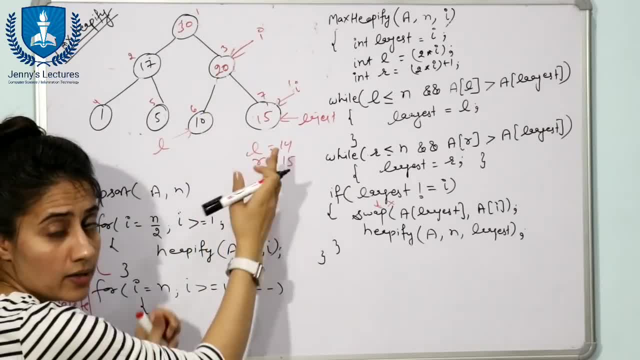 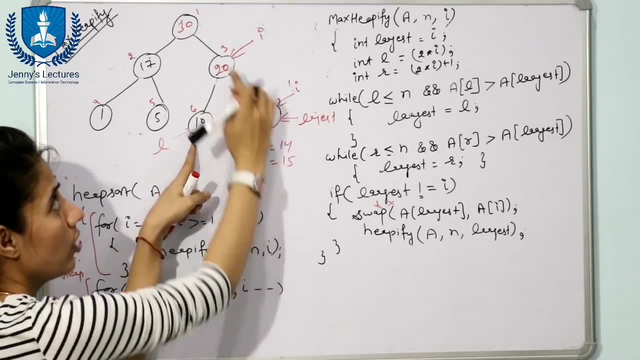 this element here, only Fine. and the array array- the heap size would be reduced to minus 1, and the last of the array- this space is free now. now we are going to. the deleted element would be shifted to here, only Fine. so here you can write, we are. 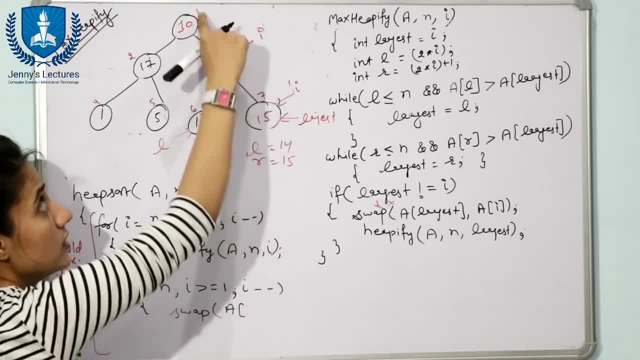 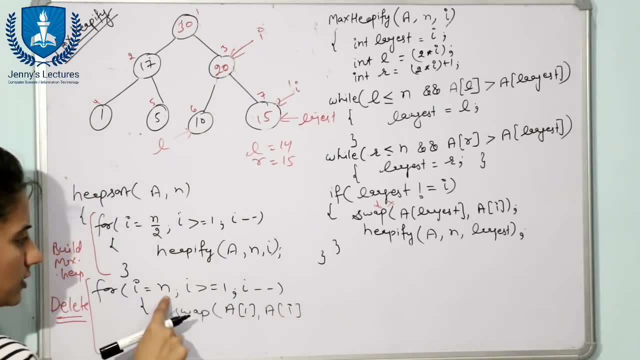 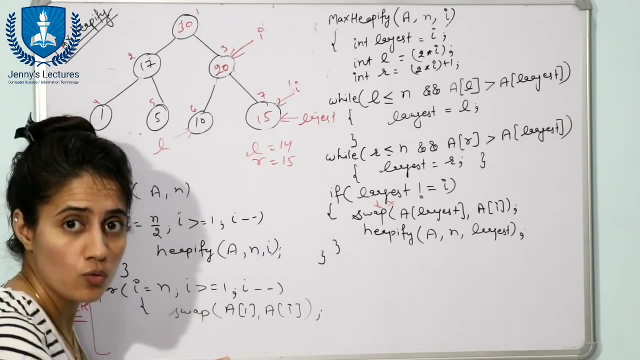 going to swap array of first, this element, with array of i, because i is n, so n n means the last element. Fine, and after swapping? after swapping, what we will do, we will check: is this still satisfying max heap property? if not, we are again going to make it max heap. 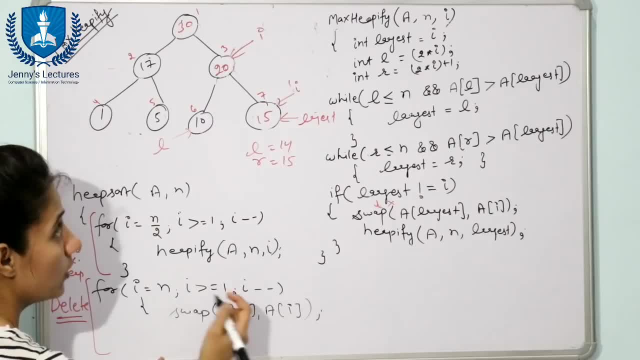 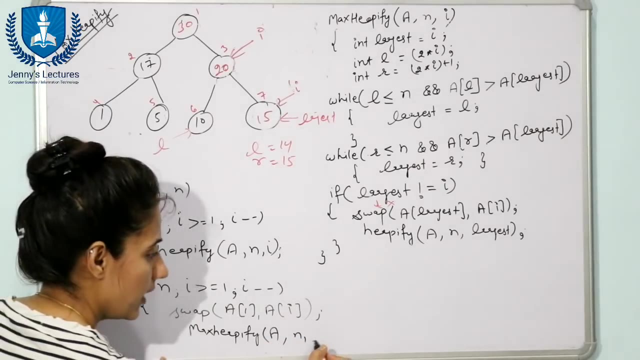 by calling this heapify method. So now here also we will call: see here we have taken name max heapify. so i am going to write here max heapify. so here also i am going to call max heapify. on array, a number of elements are n and here 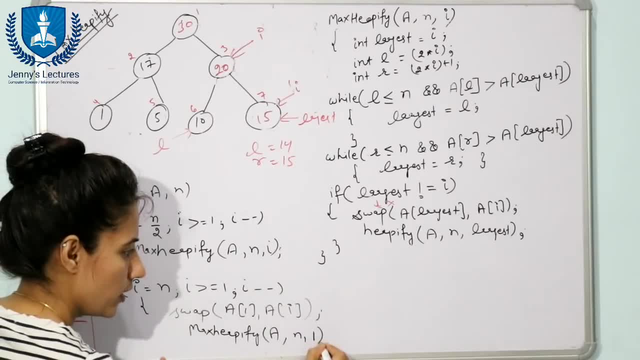 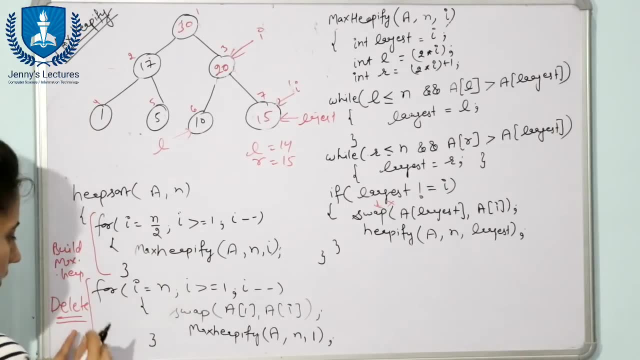 the i value, i value would be passed. what here we are going to pass? 1. and this step is for deleting and after that you are going to close this heap. so this is what heap sort is here. 2 questions are there, i know. i hope you know that. 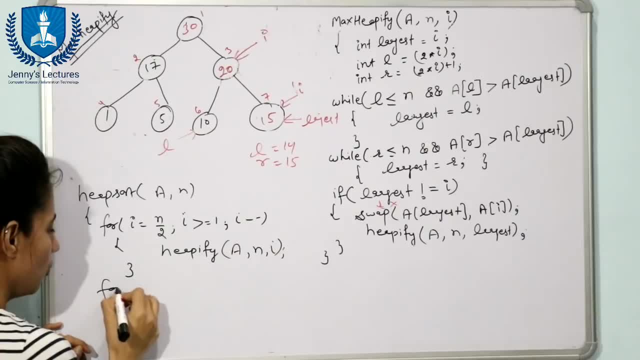 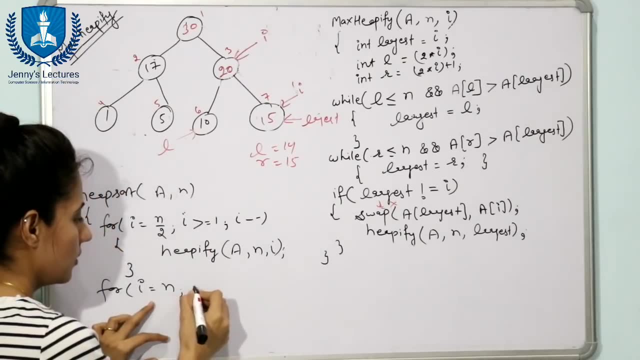 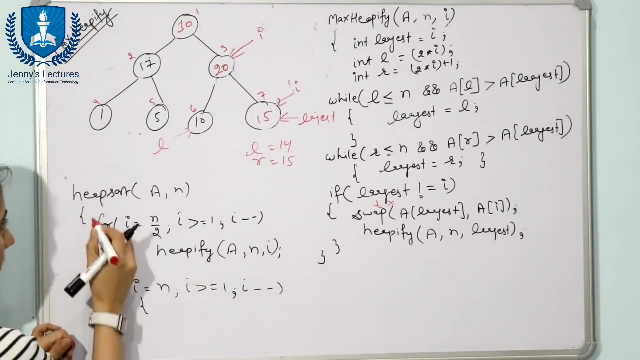 done from the root always. so now we are going to call one for loop again, and this i would be 4, n, i should be greater than equal to 1, and i minus, minus. so here see this: this step is what build max heap, this for loop, right, and after that next step is what for deleting. 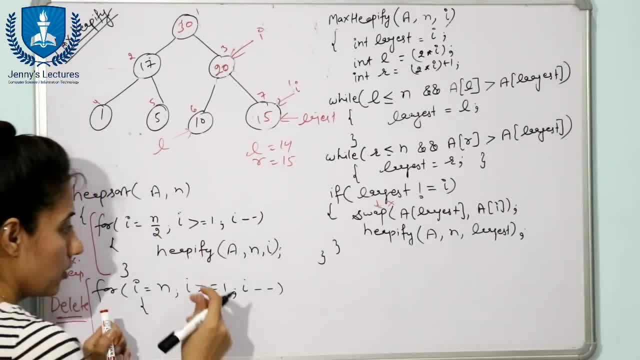 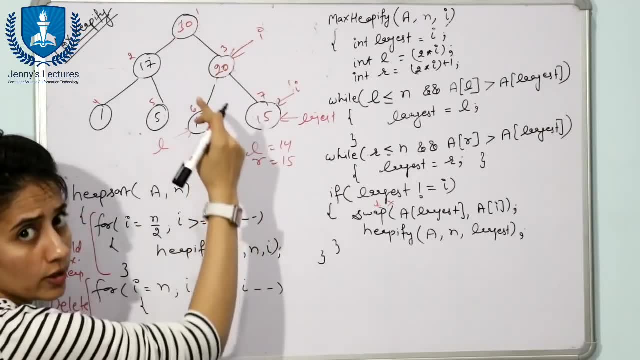 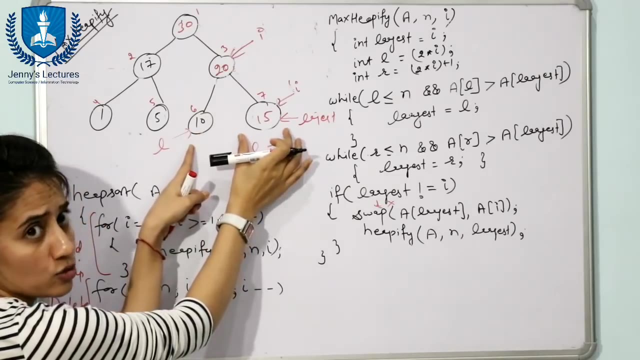 element from max heap, fine. so for deleting, when you delete, when you delete element, suppose we are going to delete this 30.. what we have done, we are going to swap this element here, only fine. and the array, the heap size, would be reduced to minus 1 and the last of the array. this space is free now. now we are going. 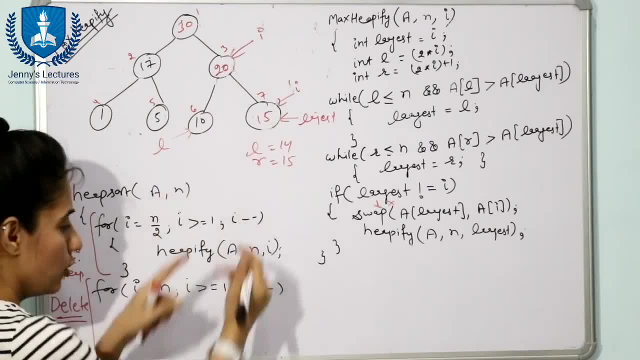 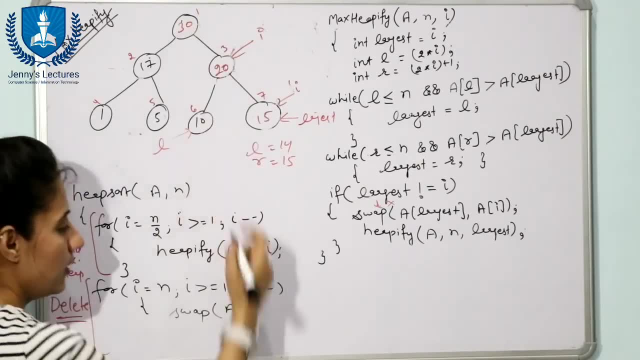 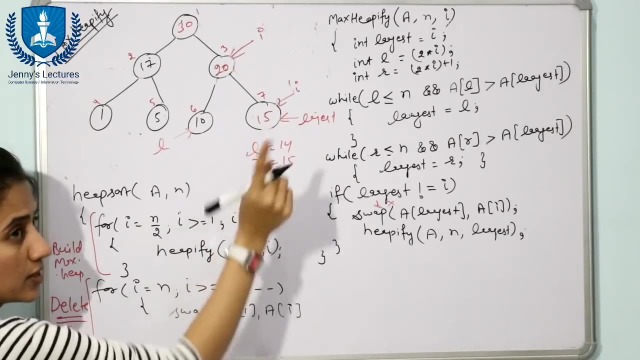 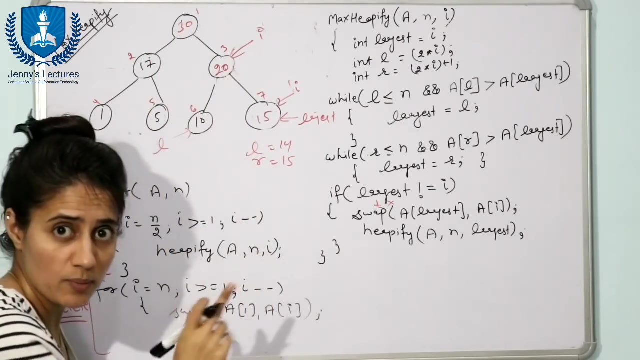 to the deleted element would be shifted to here, only, fine, so here you can write: we are going to swap array of first, this element, with array of i, because i is n, so n, n means the last element. fine, and after swapping, after swapping, what we will do, we will check. is this still satisfying? 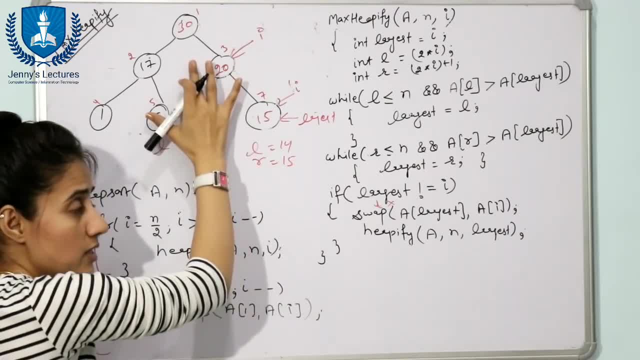 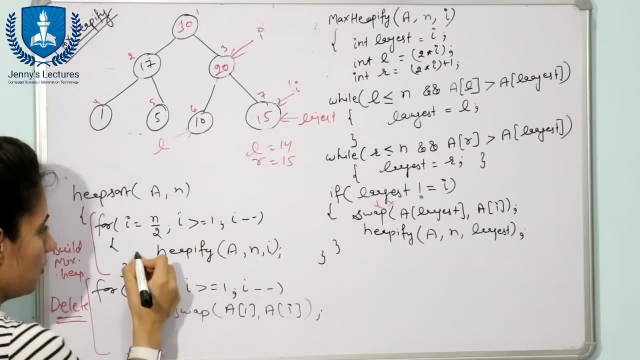 max heap property. if not, we are again going to make it max heap by calling this hippify method. so now here also we will call: see, here we have taken a max hippify, so i am going to write here: max hippify. so here also i am going to call max. 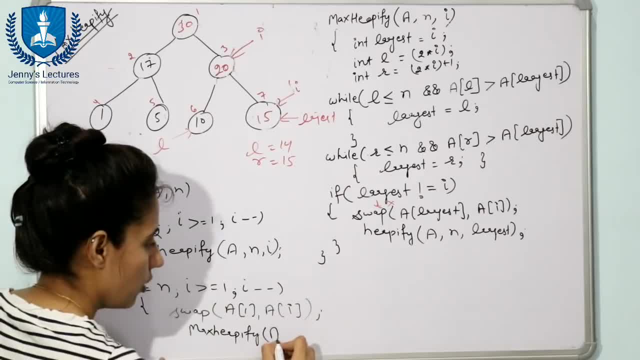 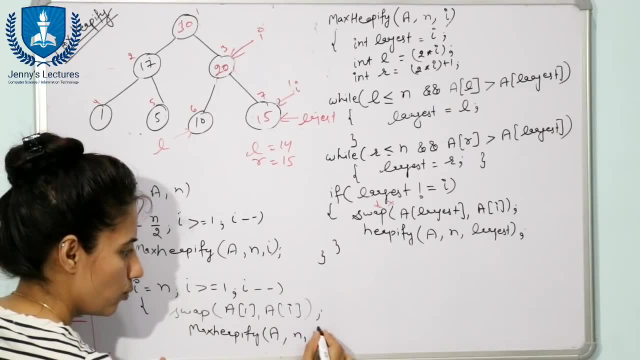 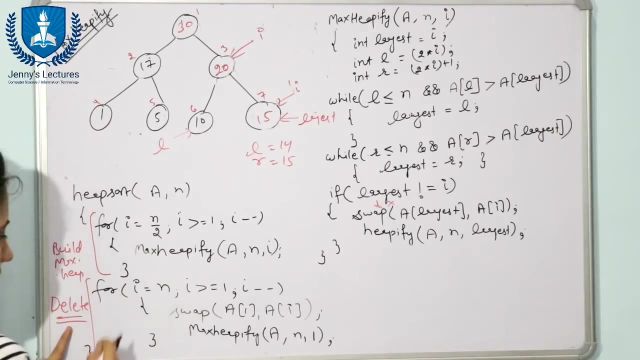 hippify on array. a number of elements are n and here the i value- i value would be passed. what here we are going to pass 1 and this step is for deleting, and after that you are going to close this heap. so this is what heap sort is here. two questions are there. i know that. i hope you know. 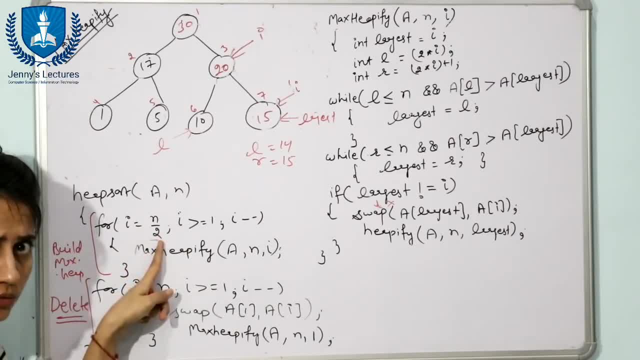 that why i am going to start this build this loop. so i am going to write here max hippify. so here also i am going to call max hippify from n by 2 in building of max heap, but this for deletion also. i am going to start this loop from: 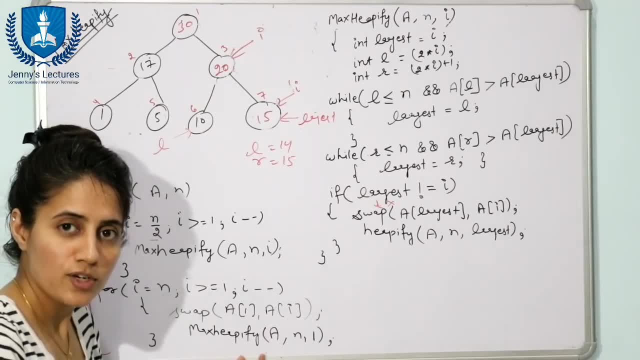 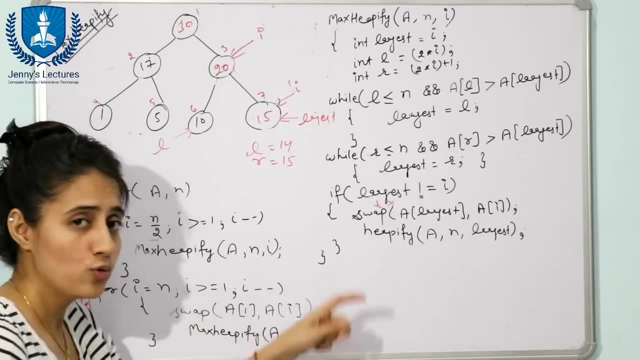 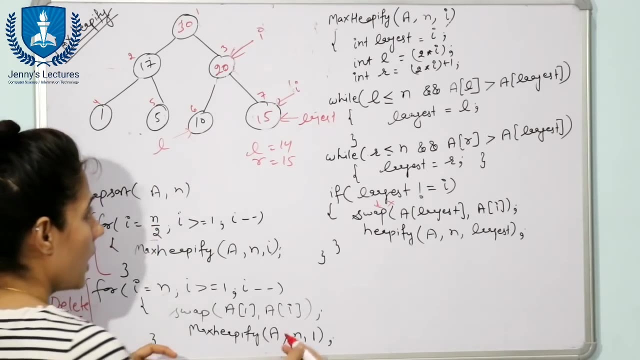 n and here i am going to pass one only so here. pause the video, try to find out the answer, and if you get the answer, then please tell me in the comment box. okay, here i am going to discuss why this- we are going to start this loop from n and why this is here one. okay, see here. see after. 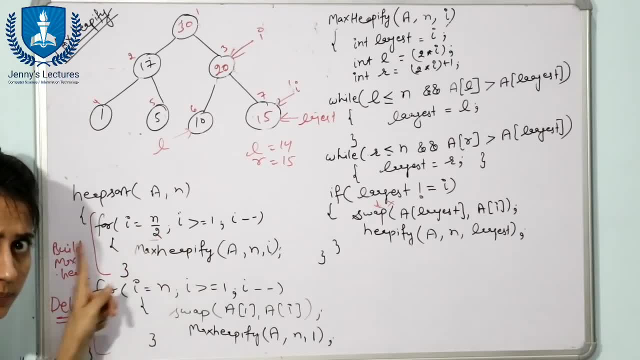 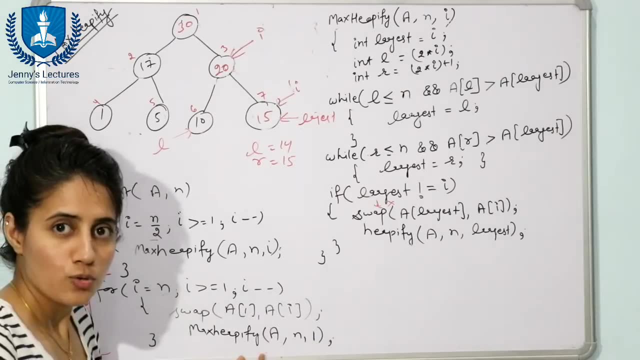 why i am going to start this loop from n by 2 in building of max heap, but this for deletion also. i am going to start this loop from n and here i am going to pass 1 only. so here, pause the video, try to find out the answer and if 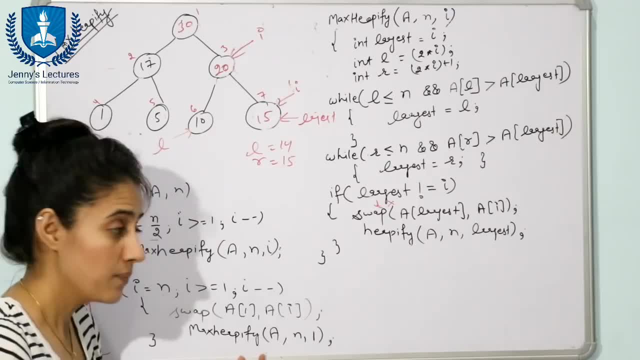 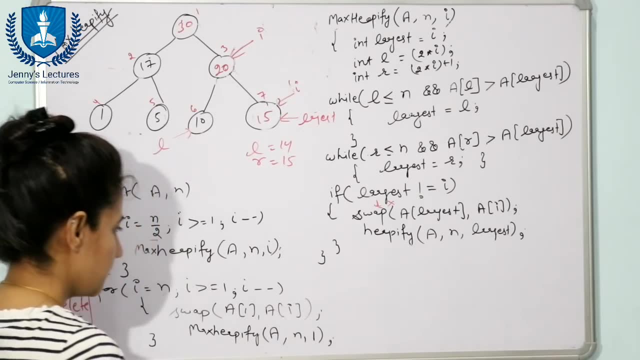 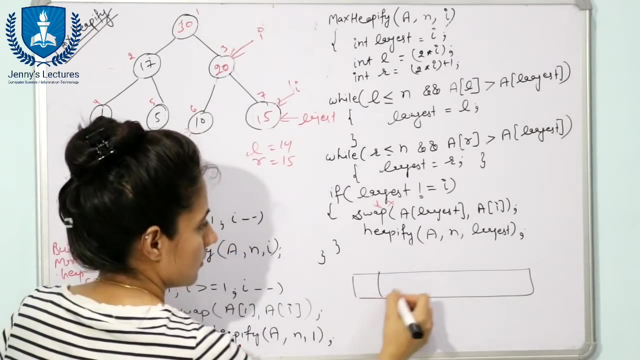 you get the answer, then please tell me in the comment box. ok, here i am going to discuss why this. we are going to start this loop from n and why this is here 1. ok, see here. see: after building of this max heap, the array would be something like this: 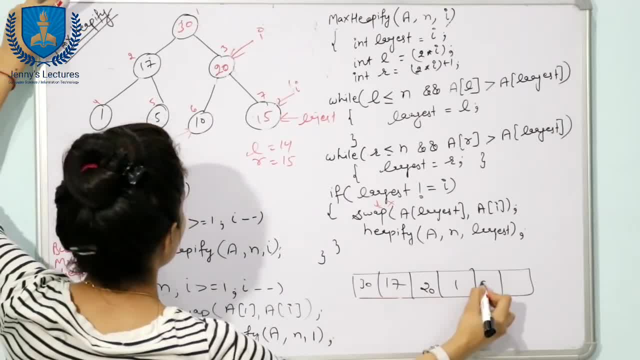 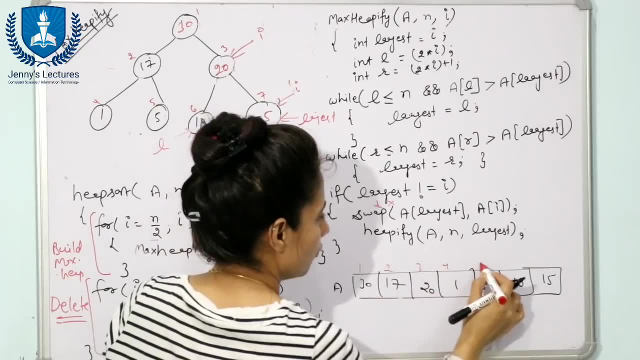 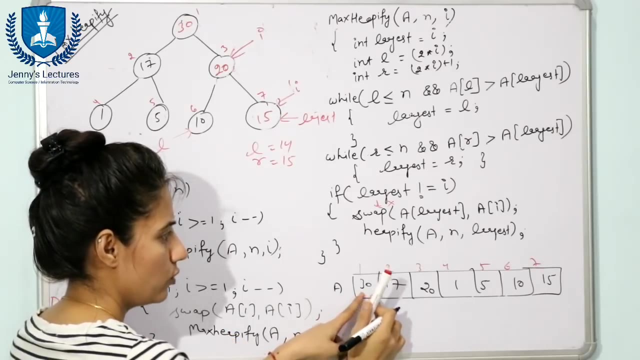 here is 30, 17, 20, 1, 5, 10 and 15. right index is 1, 2, 3, 4, 5, 6 and 7. now we are going to delete the data now, in deletion, what we will do, we will swap what we will. 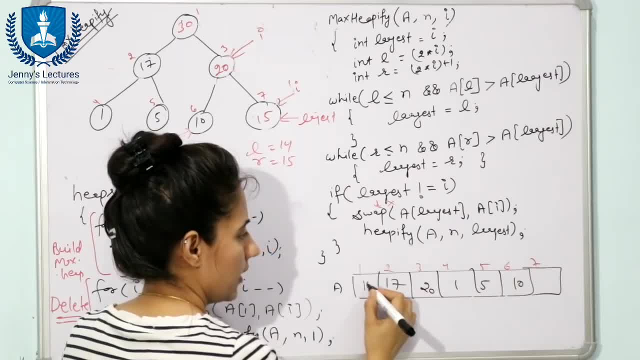 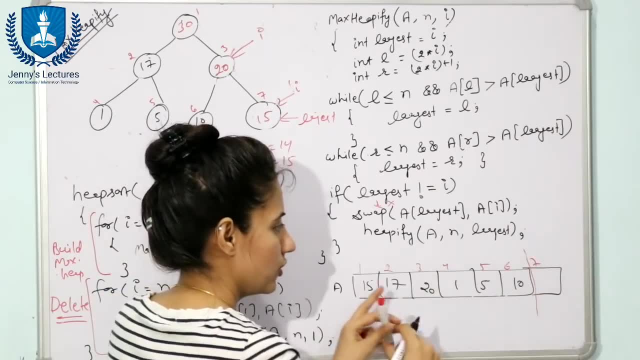 delete 30 from here. the last element would be shifted here now. now the heap size is from 1 to 6 and this, this, is the blank space. so i am going to. we are going to shift 30 at this place, right? so that is why the swap is there. 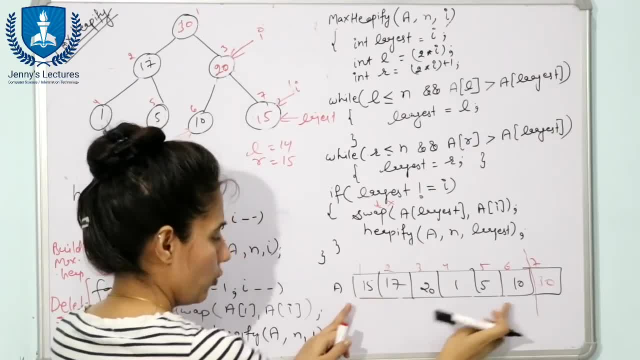 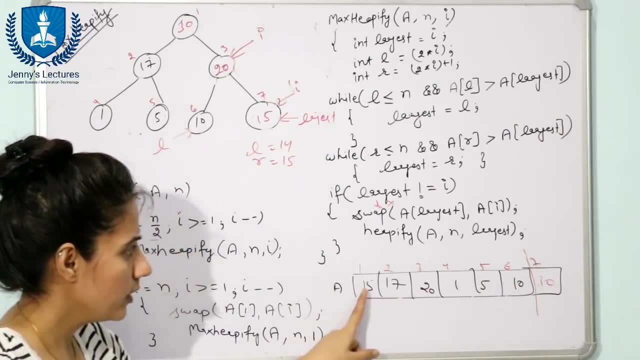 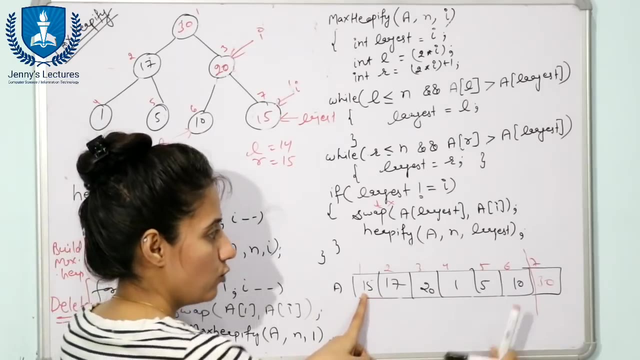 now, now again. if again we are going to call this heapify method, fine, after heapify method, next largest element would be here at first place. it means 20 would be at this place. now, now again, you will delete 20 and 20 would be stored. 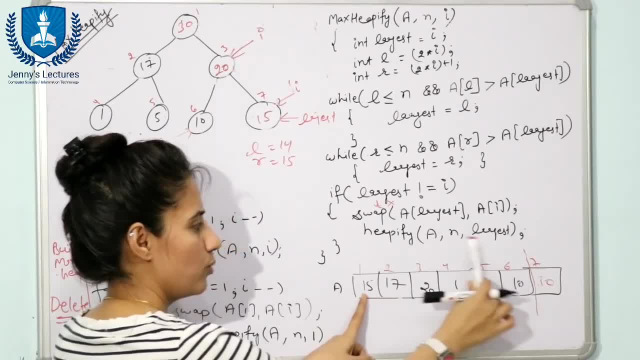 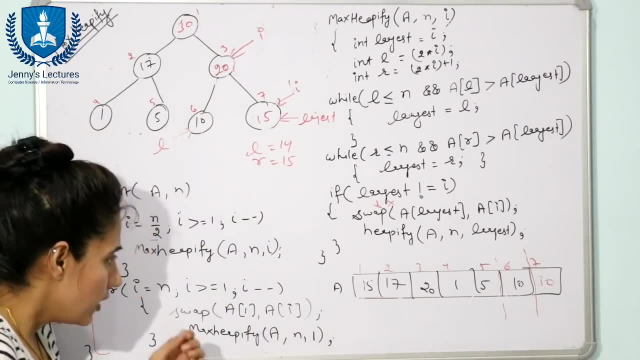 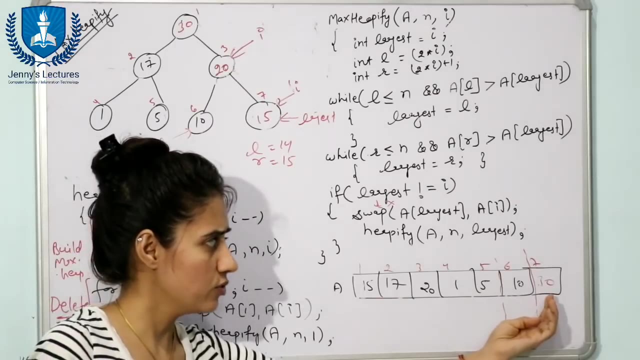 here, and the element which is there at the last position would be shifted here, and again the size would be reduced. ok, so now, that is why i am going to start the loop from n here only because here the size is to be reduced, from here only first. 7. 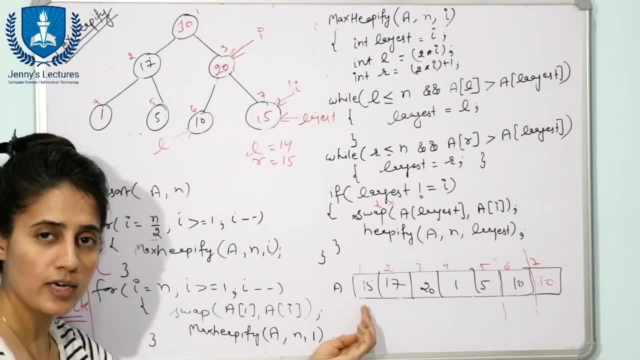 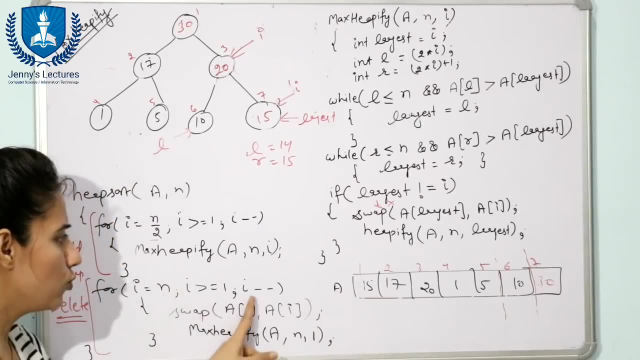 then 6, then 5 and till we reach to 1. we are going to delete data till we reach to 1. that is why i am going to start this loop from 1. if you start this i from 1 from 1, then what you will do? you will do i minus, minus. 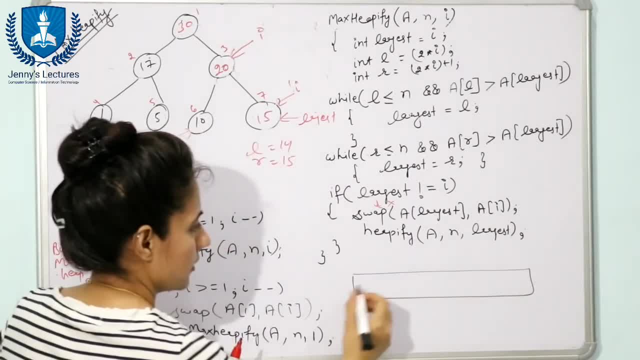 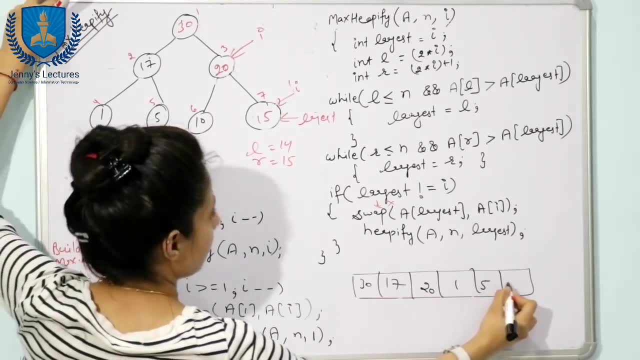 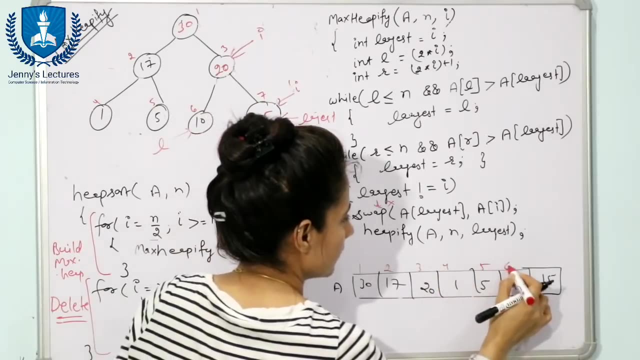 building of this max heap. the array would be something like this: here is 30, 17, 20, 1, 5, 10 and 15. right index is 1, 2, 3, 4, 5, 6 and 7. now we are going to delete the. 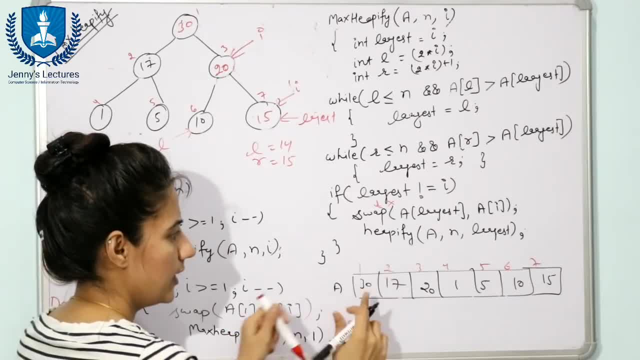 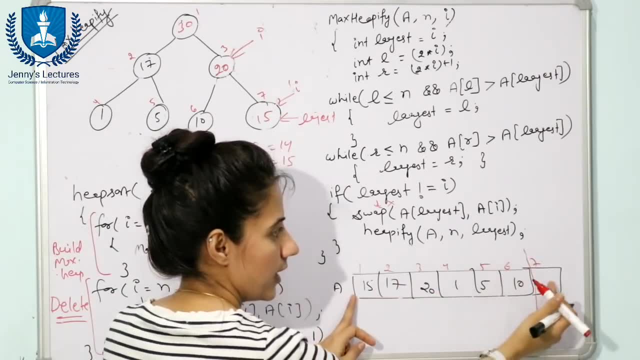 data. now in deletion, what we will do, we will swap. what we will delete: 30 from here. the last element would be shifted here now. now the heap size is from 1 to 6 and this is the blank space. so i am going to, we are going to close this loop. this is for deletion of the heap size, so i am going to, we are going to. 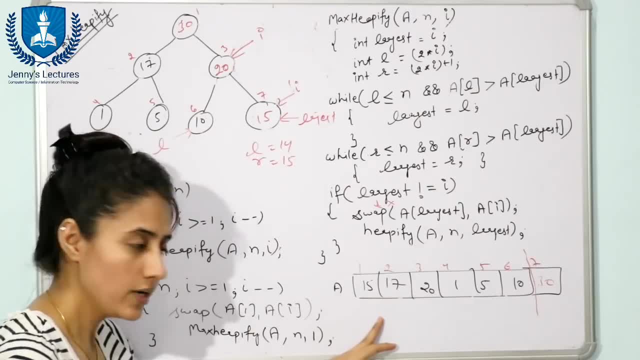 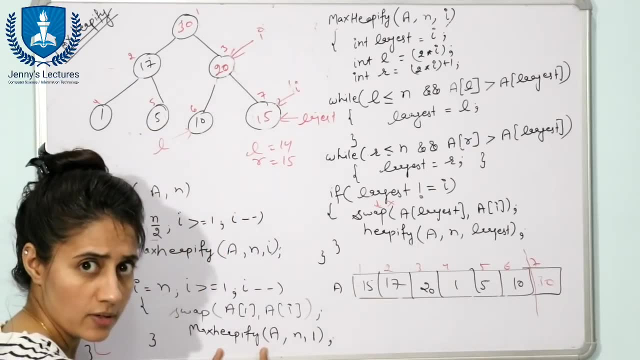 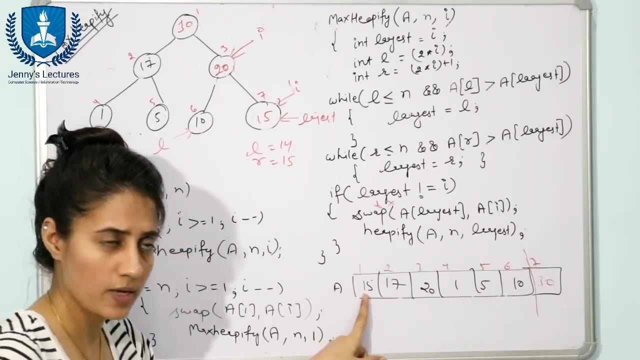 shift 30 at this place, right. so that is why the swap is there now, now again. we- if again we are going to call this cp5 method- fine, after hippie phi method, next largest element would be here at first place. it means 20 would be at this place now, now again, you will delete 20 and 20 would. 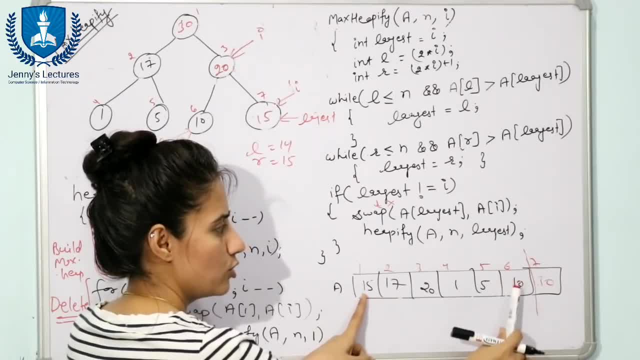 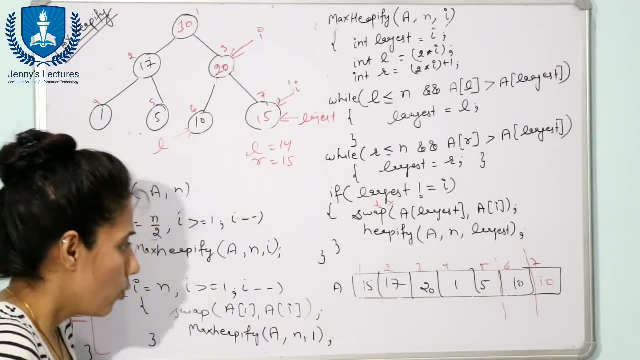 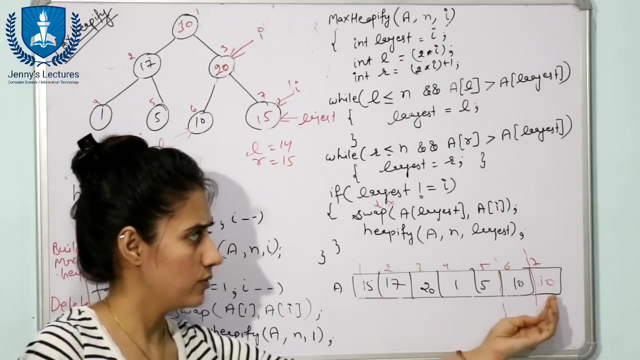 be stored here, and the element which is there at the last position would be shifted here, and again the size would be reduced. okay, so now, that is why i am going to start the loop from n, here only because here the size is to be reduced, from here only first seven, then six, then five, and till we 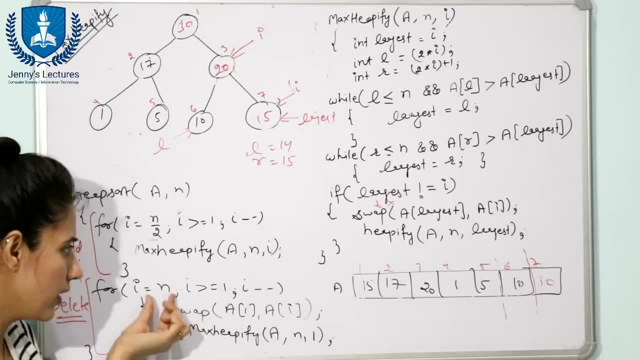 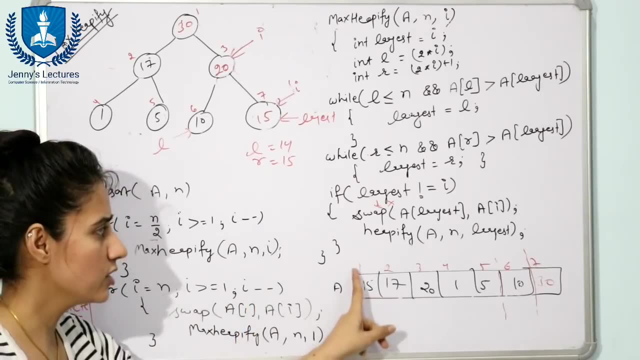 reach to one. we are going to delete data till we reach to one. that is why i am going to start this loop from one. if you start this i from one, from one, then what you will do, you will do i minus minus. then next time i will be two, next time i will be three. so from here you are going this. 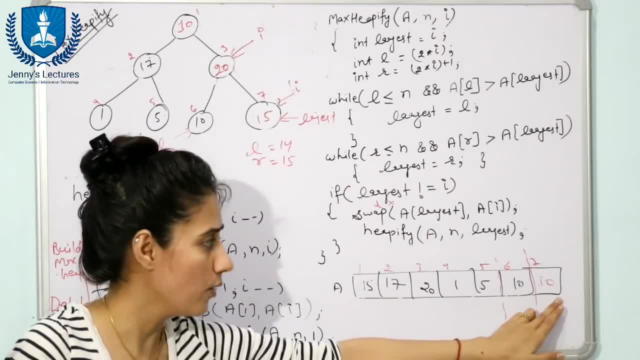 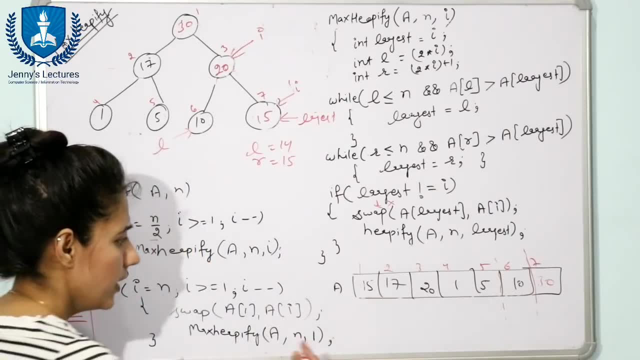 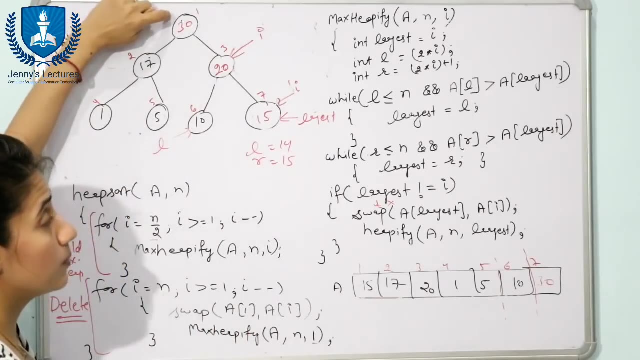 side. no, but in deletion you have to do what you have to reduce the size from array heap size. from this side we are going from right to left. fine, and now why we are going to pass one here? because always we are going to call this cp5 method, at this place only. 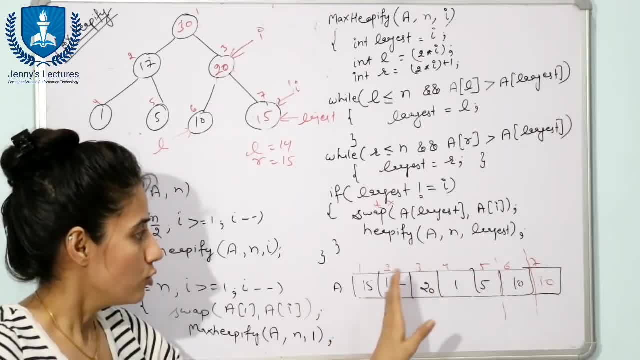 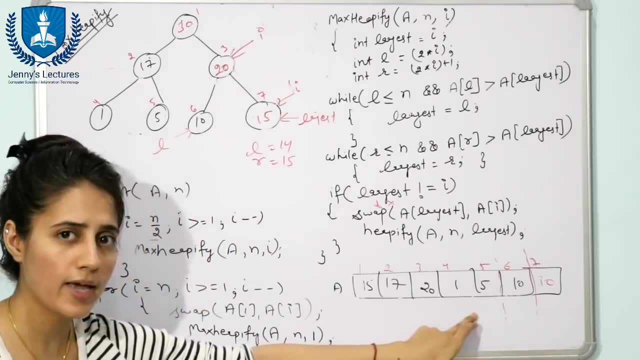 then next time i will be 2, next time i will be 3. so from here you are going. this side no, but in deletion you have to do what you have to reduce the size from heap size. from this side we are going from right to left. fine, 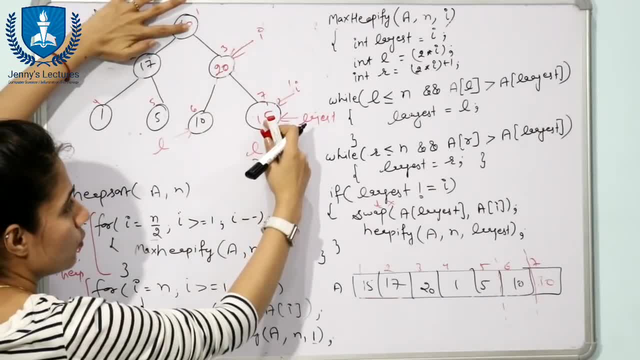 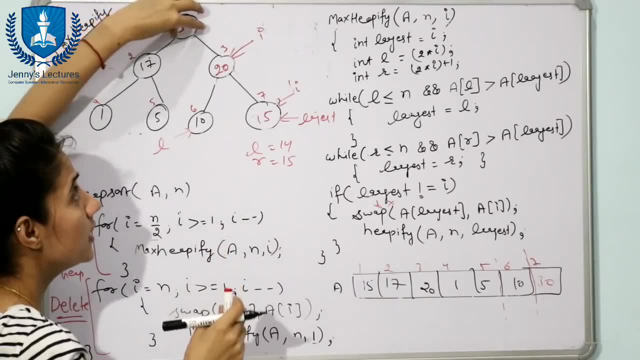 because if you delete this 30, then you are going to pass. you are going to place 15 here and you will check: because of this 15 is it violating maxi property. so now we are going to heapify method on here only on the root node only because always we are going to delete data from.